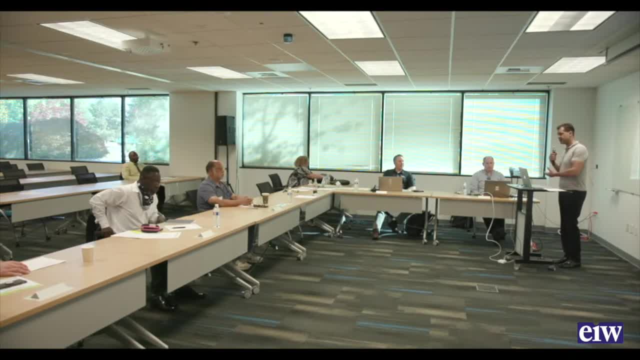 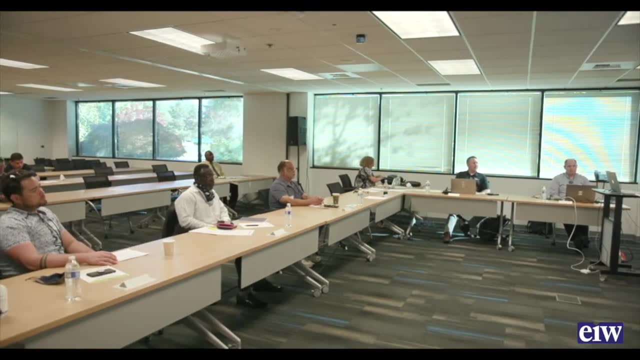 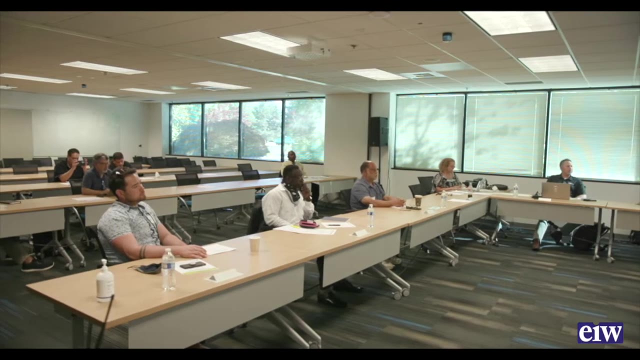 We also want you to see the best practices that companies like Hoffman has been able to master over the years, And they've been very successful in public contracting, And to me, there's no better example that we could use to give us access and tools that will help us navigate through future projects. 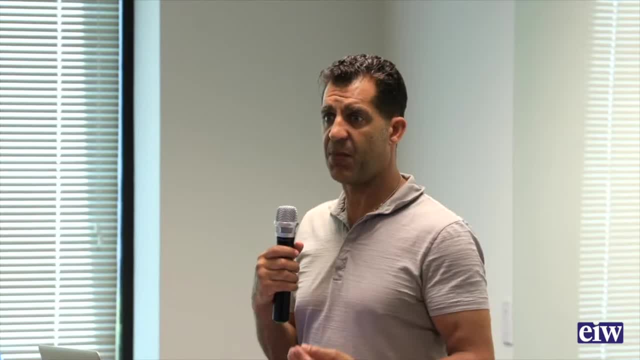 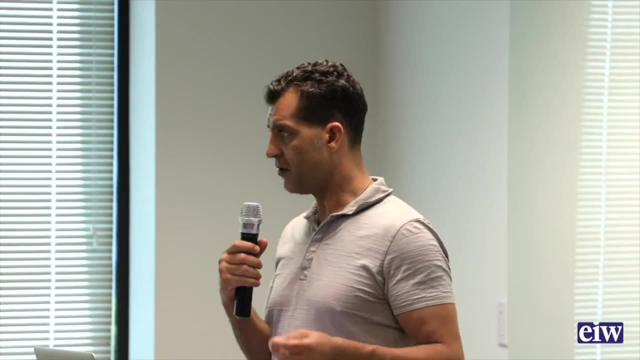 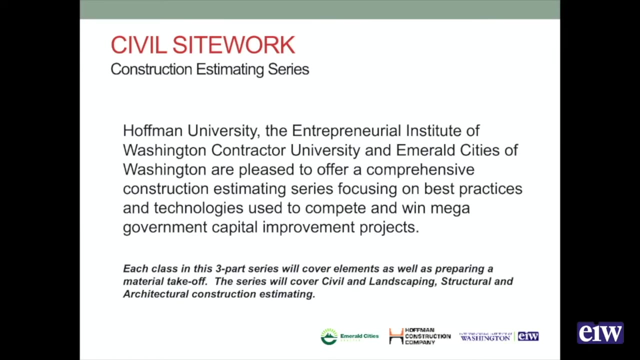 Those of you that aspire to be general contractors, this three-part series is going to be spot on for you. Those of you that want to have a better understanding of other trades, not just the trades that you specialize in, this three-part series is going to be great for you. 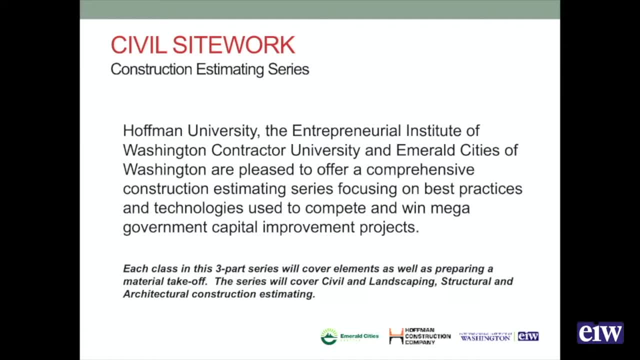 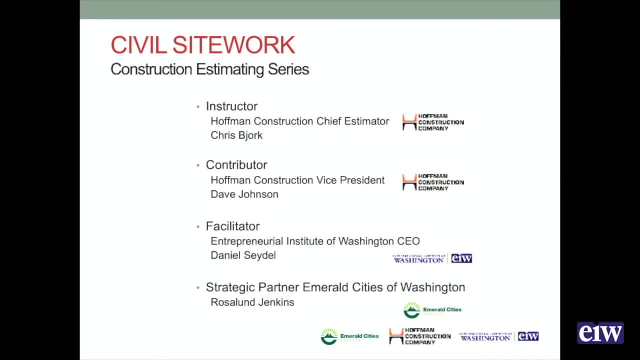 It's also going to be a good resource for you that specialize in those certain elements. And so today we're going to be focusing on the civil side, On the civil side of construction. Obviously, we are joined today with our instructor, Chris Bjork, who's going to be introducing himself. 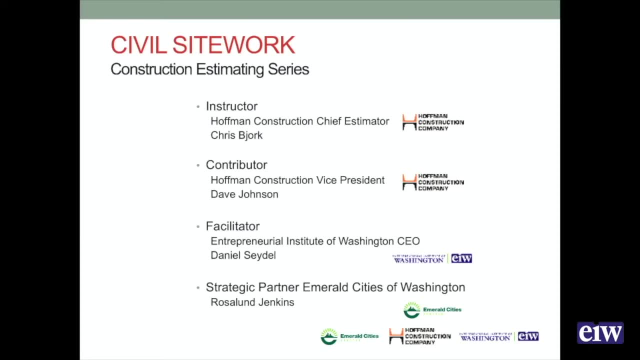 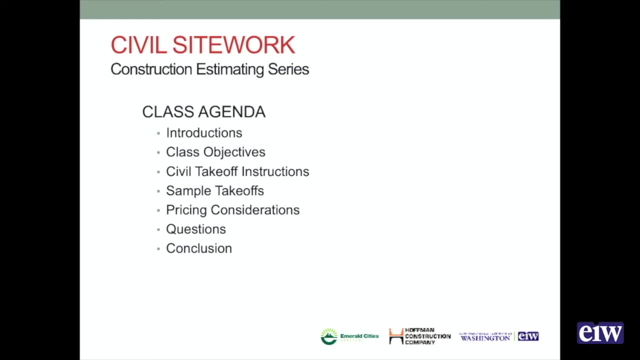 He's been a great asset for the Entrepreneurial Institute of Washington, which is another partner that we have. that, put this, made this all possible, And again we'll hear from Rosalind Jenkins. Our agenda is as follows. We're going to be doing our introductions and our class objectives. 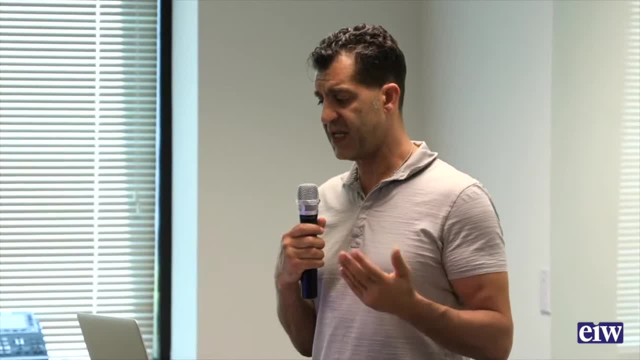 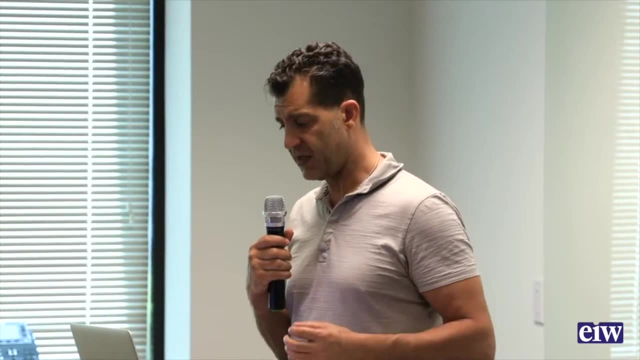 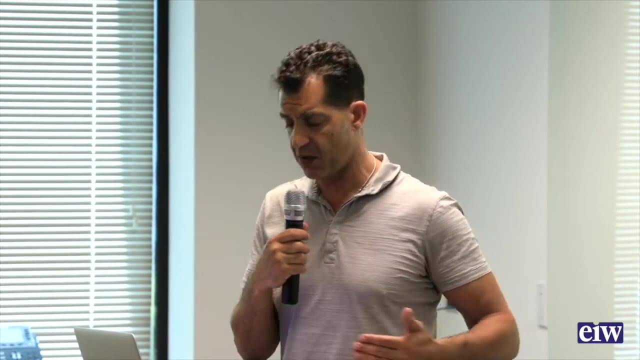 We're going to go over the civil takeoff instructions And then we're going to go through some sample takeoffs. We wanted to really personalize this so you could see how we go through the estimating process step by step, And so we're excited to be able to share these best practices with you. 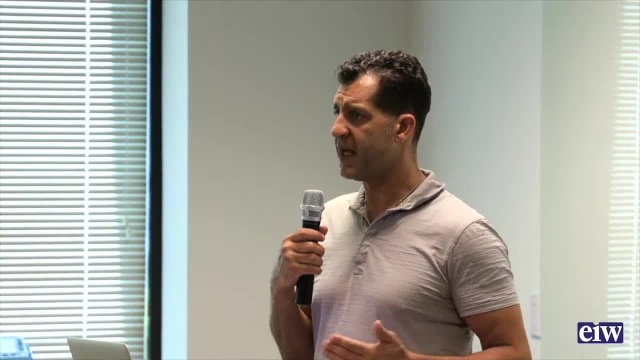 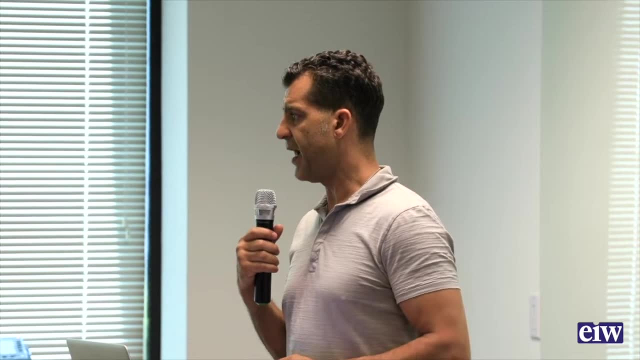 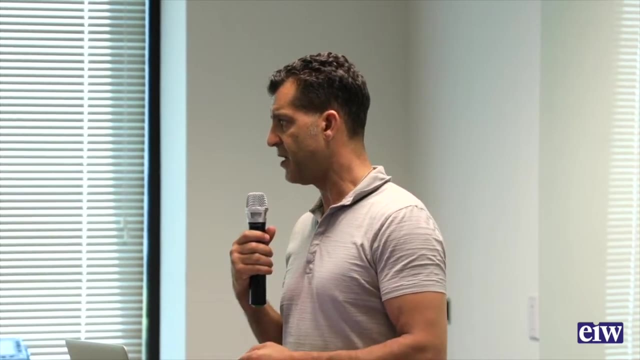 And again, because we have such an intimate group, we're going to be able to have time for Q&A. Those of you that have joined us electronically, we're going to ask that you raise your hand and develop questions in the chat. There's also a survey in the chat. 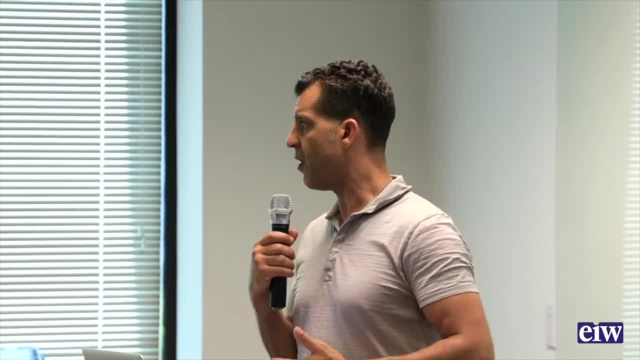 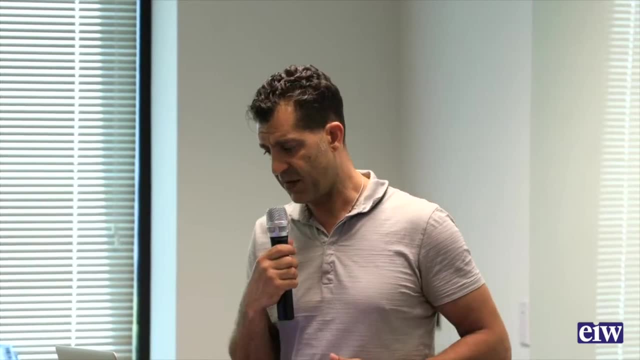 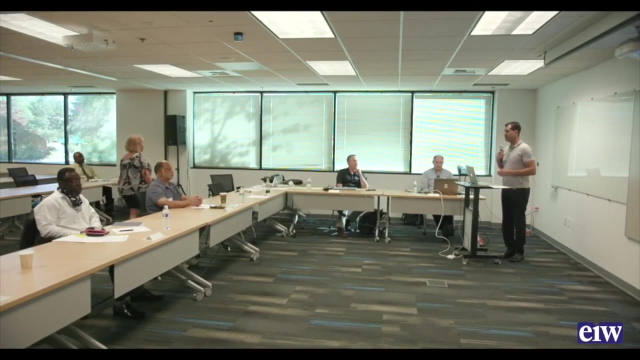 And we would encourage all of you that, if you're involved in the Zoom, to participate in the chat so we can quantify and analyze that information. I'm going to just tell you a little bit about myself and then we will get into the show. 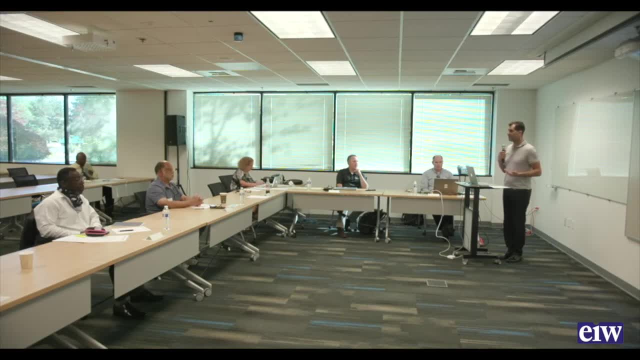 Again. my name is Dan Seidel. I'm the founder of the Entrepreneurial Institute of Washington. I also run Platinum Group Business Development, Construction Management and Community Outreach Minority Business Advocate. Over the years I've been blessed to develop projects. 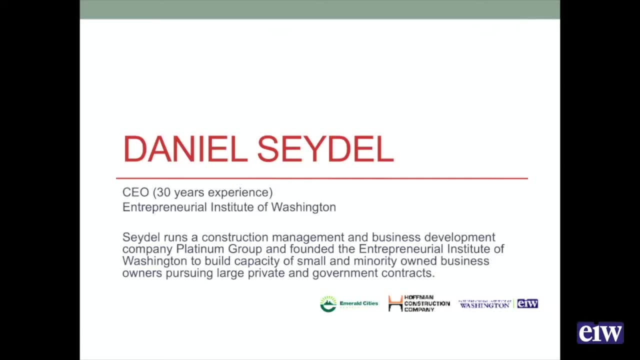 I've been blessed to develop partnerships and relationships with firms like Hoffman Construction And over these years I've felt like that exposure was good and beneficial for me and my career but would be even more beneficial if I could share those experiences, if I could share those lessons and best practices with all of you. 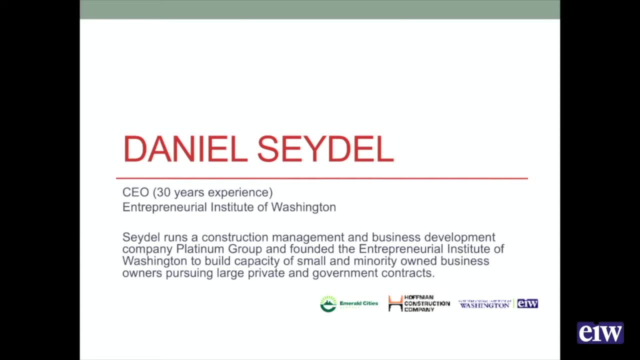 And again, we're televising this class because we want to be able to share those experiences with all of you. We want to be able to share it with as many people as possible And again, this is through the great contributions and efforts of Hoffman Construction. 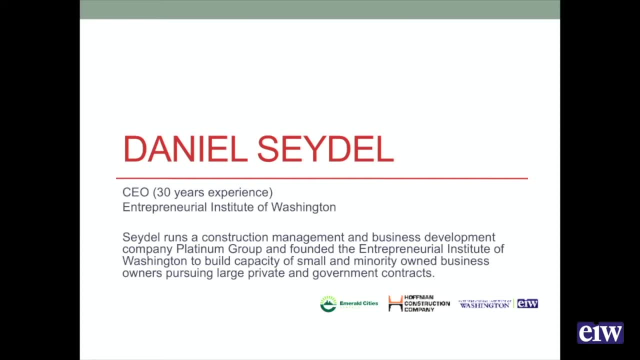 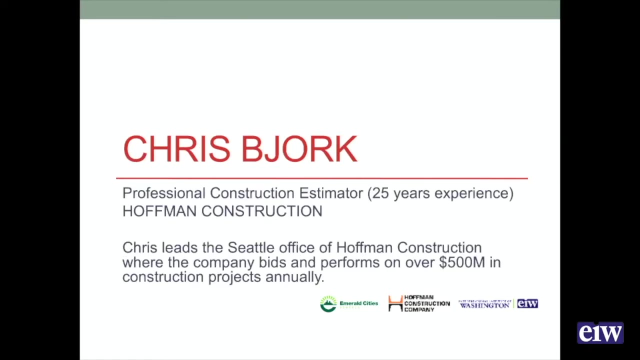 And again, we couldn't be more grateful for their efforts. So, again, my interest is really helping prepare our small businesses to accelerate their growth and development, And we see government contracting as being a resource. I'm going to go to the next person that we have in our presentation. 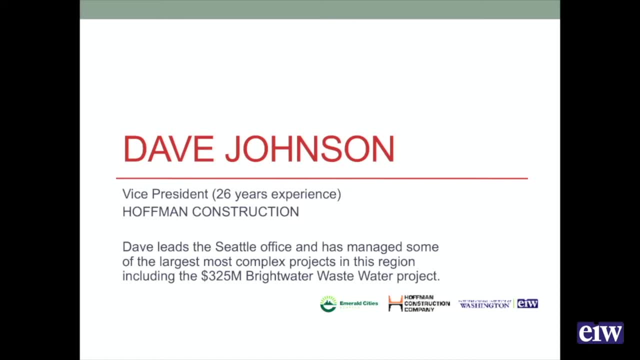 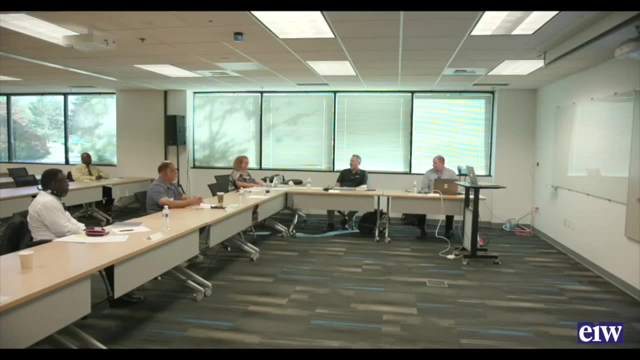 And that is Dave Johnson. And Dave, please go ahead and introduce yourself. I'm Dave Johnson. I'm Vice President with Hoffman Construction And I've had the opportunity to work with Dan for the last 15 years trying to help develop partnerships and mentorships with businesses around the area. 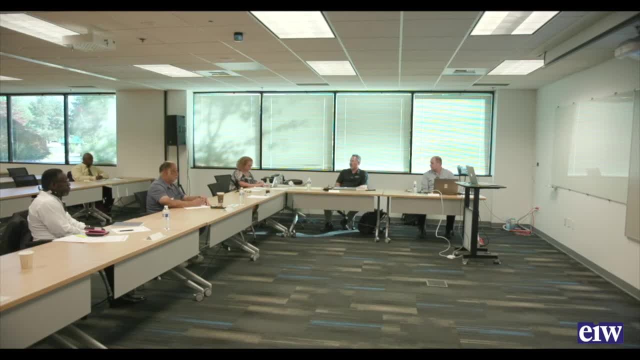 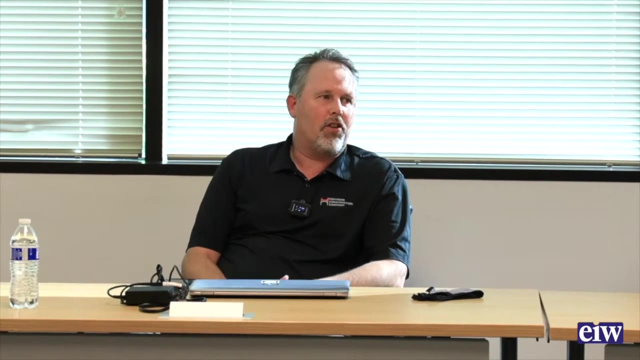 and help to figure out how we can encourage others to be successful on our projects, And so it's been a great opportunity for us to develop networks and partnerships with folks to do that, And so this series is just another example of things that Dan has helped us with. 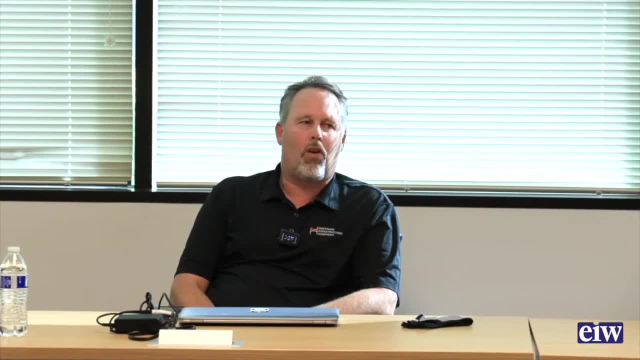 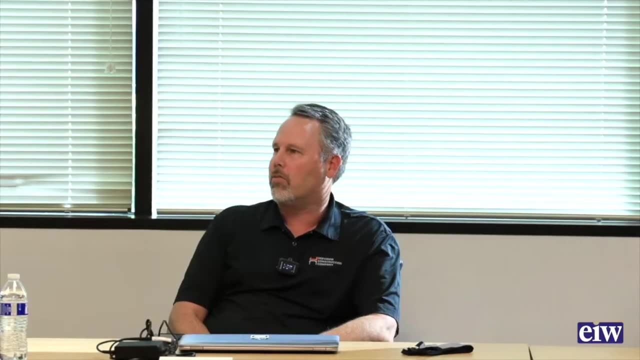 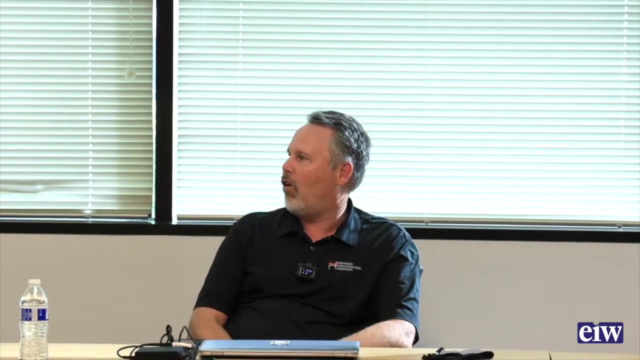 to figure out how we can improve people's skill sets at different aspects of construction, And estimating is one of them. that obviously is an important part of being successful with construction, So I'm glad that you all are here and online And thanks for participating. 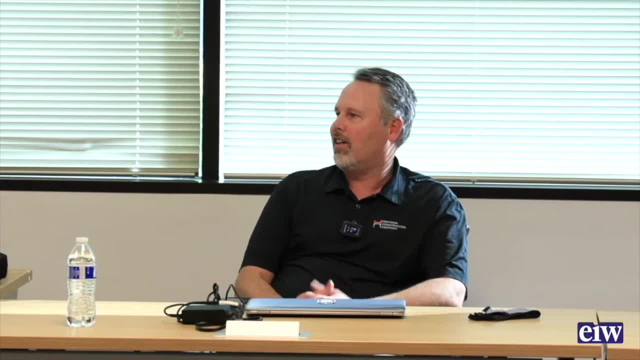 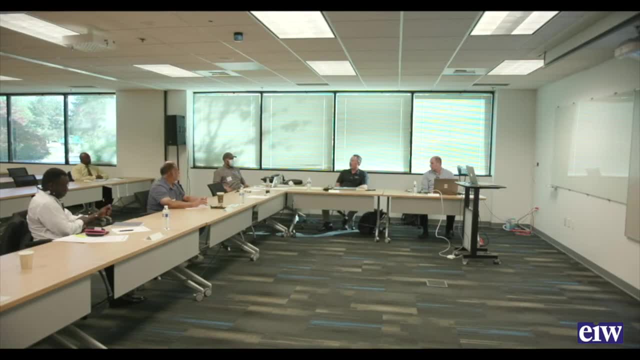 And, frankly, this is just one building block on being part of a successful business, And we'd love to help get on our projects as well. So that's another networking thing that we'd love to do too, to expand networks with people. 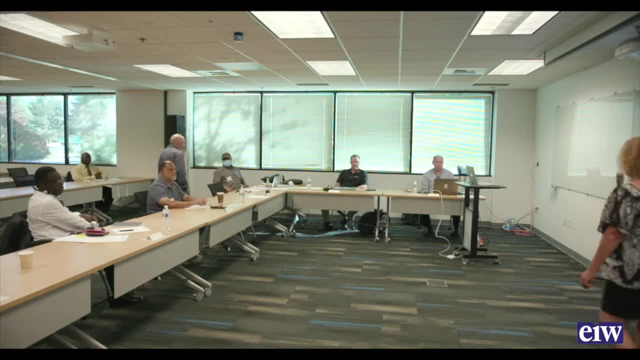 Thank you so much, Dave. Thank you, My name is Rosalind Jenkins and I'm the Economic Inclusion Manager for Emerald Cities Collaborative of Seattle, And thank you so much for the people who are Emerald Cities e-contractor graduates and participants for joining today. 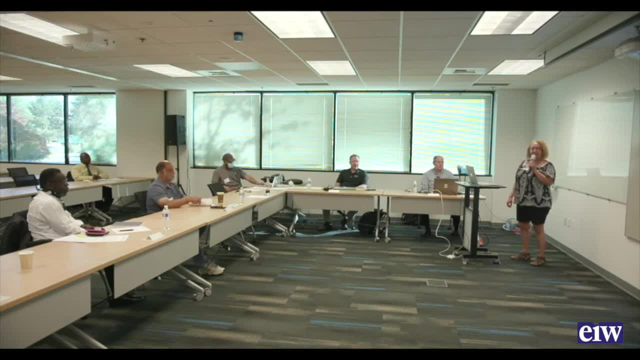 We have people from the states of Massachusetts, the state of California and, of course, our friends in the Seattle-Tacoma area and the state of Washington, And we're going to have a brief poll, But before we do, let me just mention. 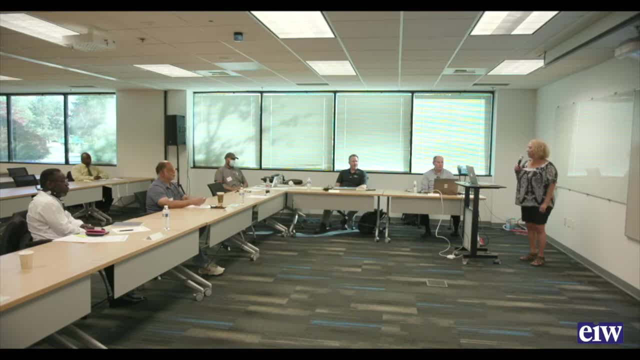 that Emerald Cities works at the intersection between equity and the clean energy implementation and exemplary building, And we're just delighted for this estimating training tonight and happy that you all participated. We're going to have a very quick poll so that we understand who's with us tonight. 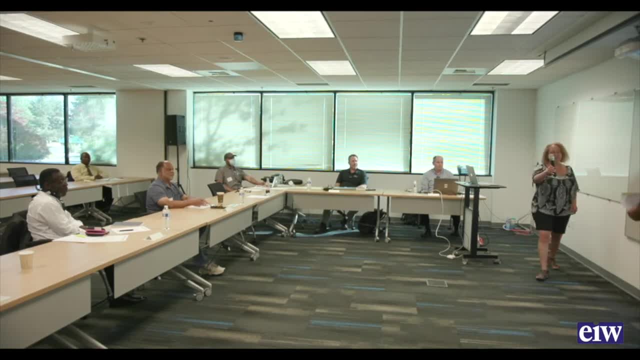 Thank you so much, And I would be remissed if I did not take a special moment to recognize the great production team that we have here today We are. our video production is being done by an Emmy Award winning producer, Cooper Visual. 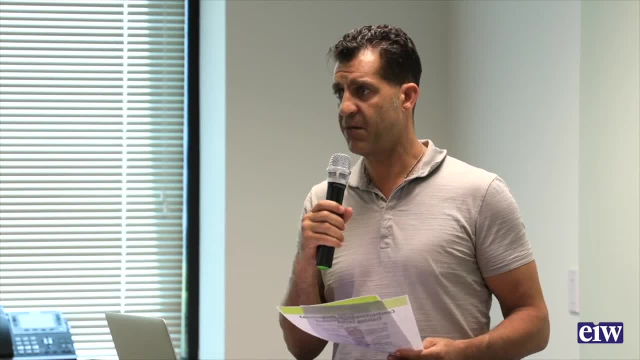 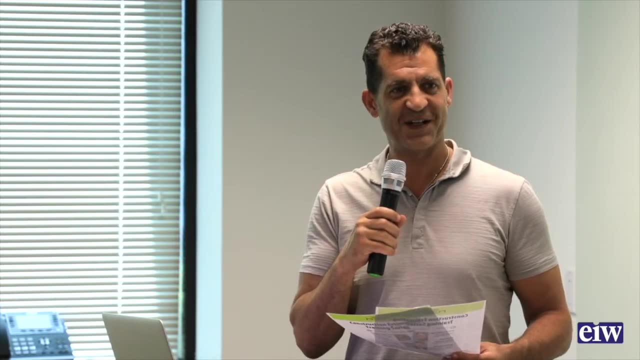 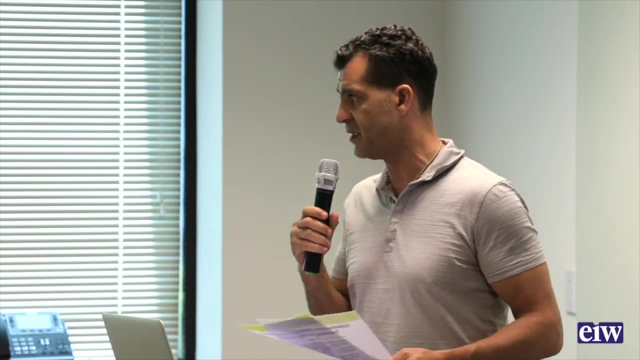 Travis Cooper is here and we're real happy to have him a part of this production- And, of course, our 35-year veteran community photographer Tabor 100, extraordinary member and the secretary of the Entrepreneurial Institute of Washington, Keith of Flywright Productions. 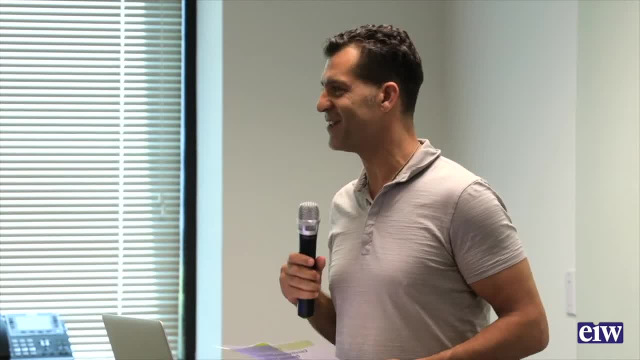 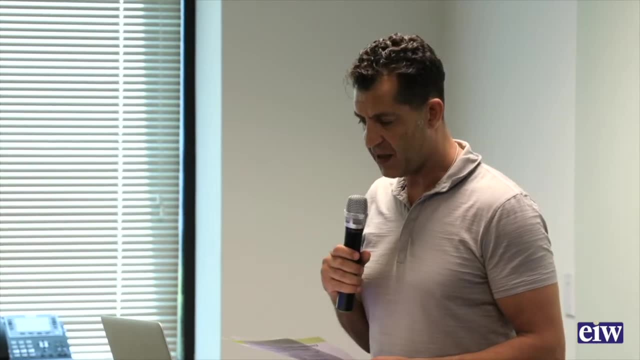 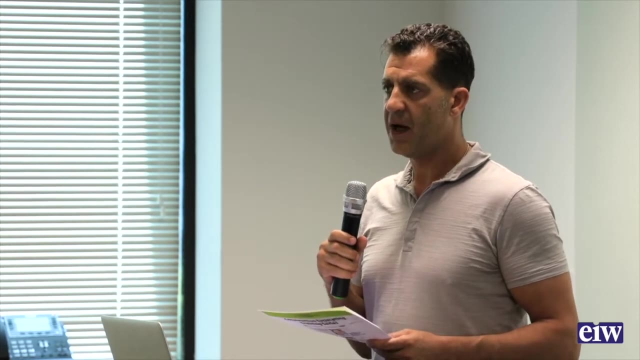 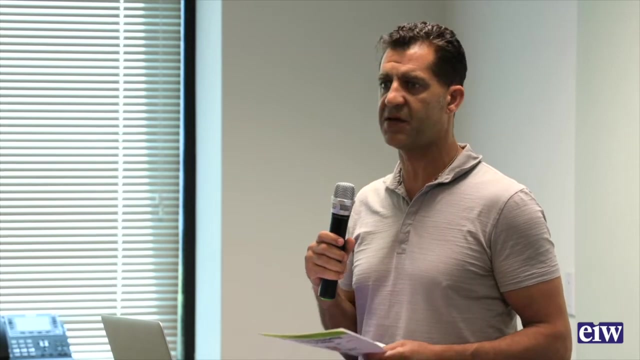 Let's give them all a hand if you can. And, last but not least, the star of this show, the man who really is responsible for helping analyze and quantify some of the most complex, sophisticated, largest megaprojects in this region. 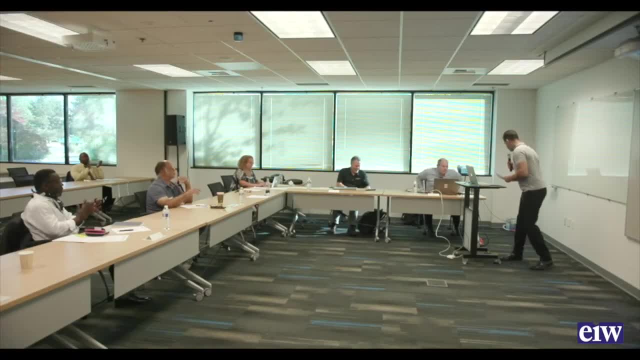 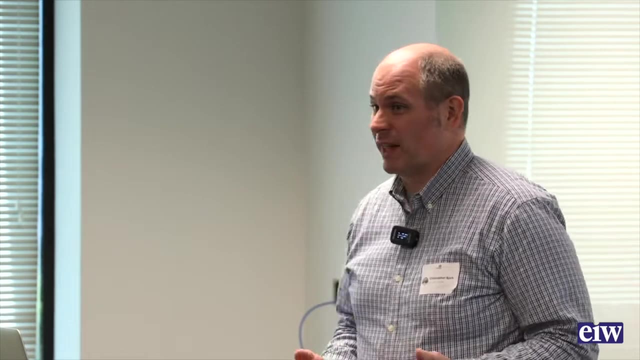 Let's give a warm welcome to Chris Bjork. Thank you so much. Thanks, Dan. My name is Chris Bjork. I am the chief estimator of our Seattle office at Hoffman Construction. I've been with Hoffman 26 years, most of that spent in estimating. 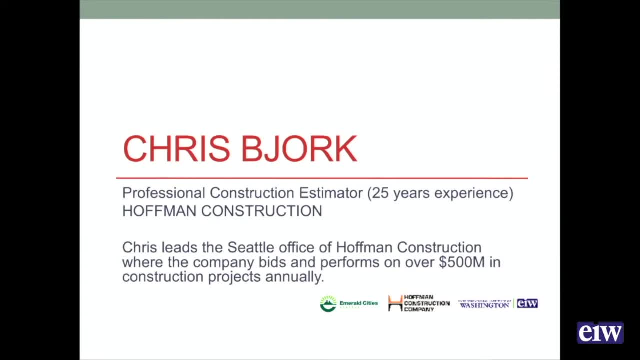 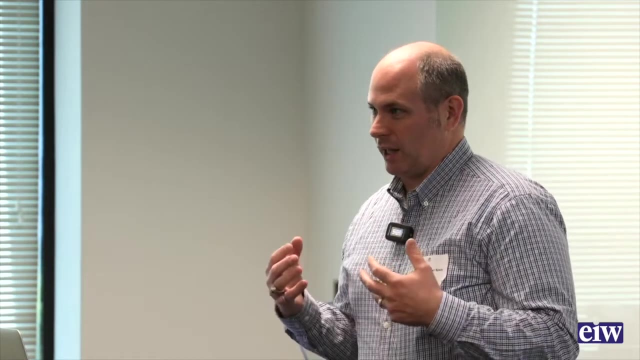 I've gotten to been fortunate enough to look on work on all sorts of types of projects, from bright water wastewater treatment plant to the space needle, renovations to molecular engineering. I get to touch a lot of different types of projects and that allows me to get a lot of different experiences. 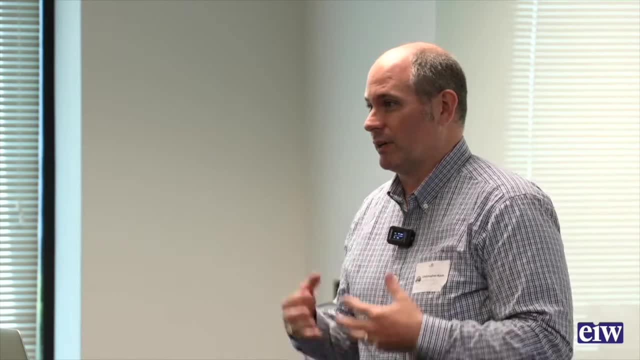 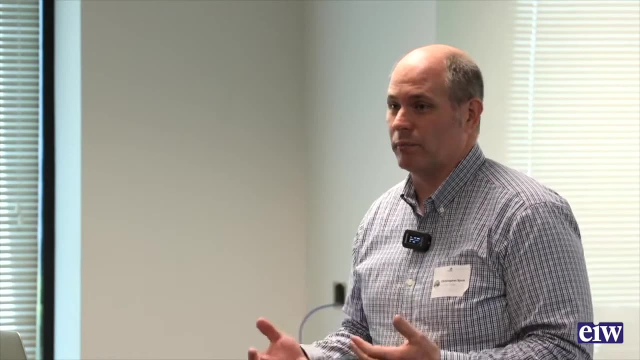 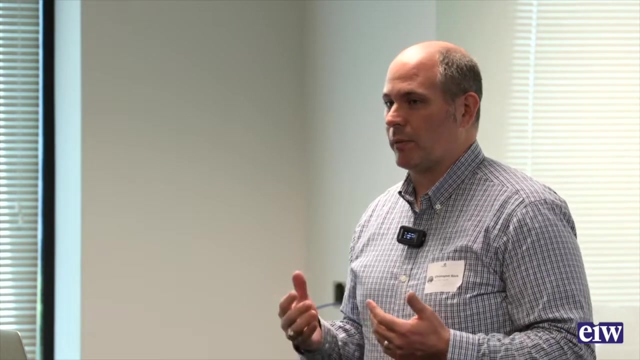 which I get to impart and use this training to help make people better at estimating, And that's really the goal. I've worked with Dan many times. This is, I think, the third in the estimating programs that we've done And I really it's all about making people better and getting more skills. 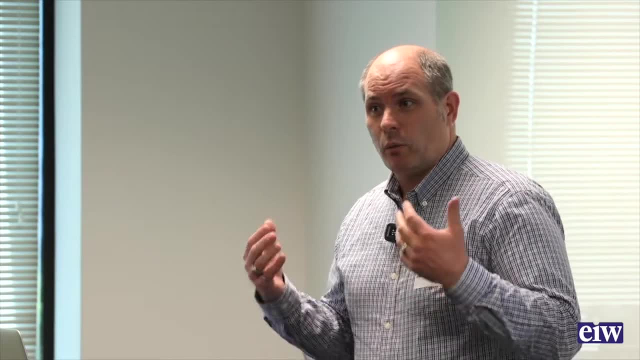 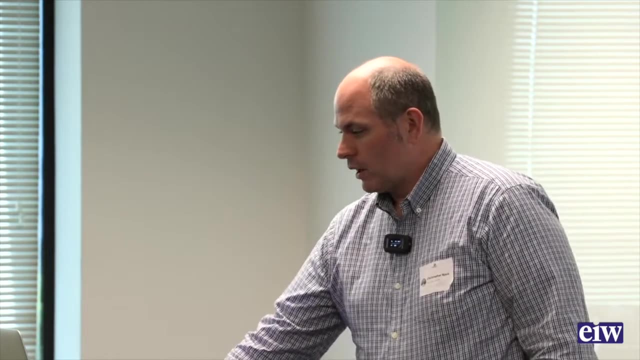 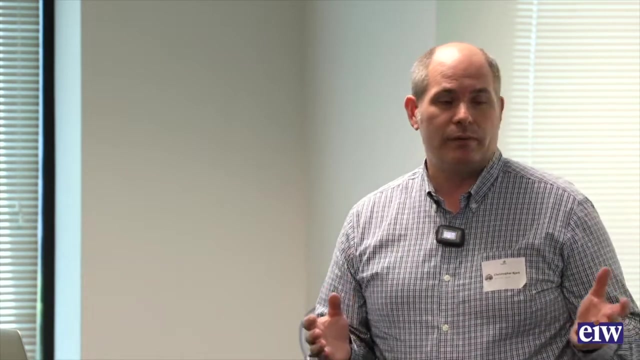 and giving you an opportunity to kind of get into my what I think and how I look at a project so that you can get that perspective. What we're going to talk about tonight. we're going to look at civil site work. We're going to look at takeoff and pricing techniques. 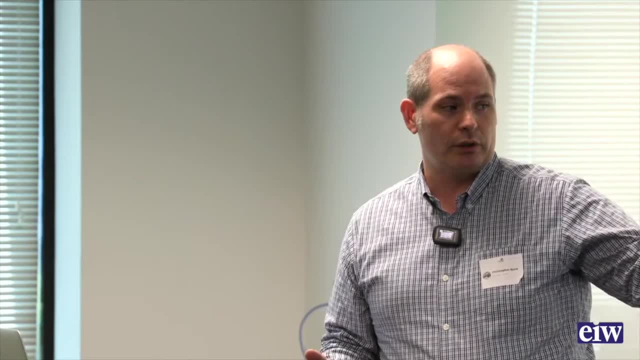 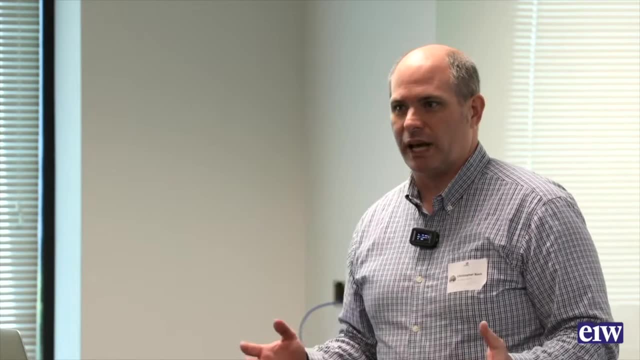 We're going to cover demolition and abatement, We're going to cover earthwork utilities and construction Paving base courses And then we're going to have some section where we talk about some of the other elements, more specialty items about civil site work. 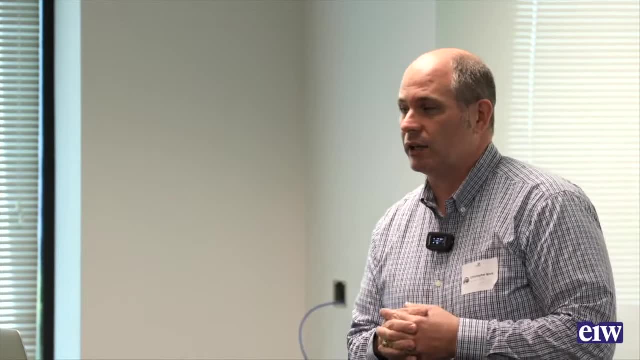 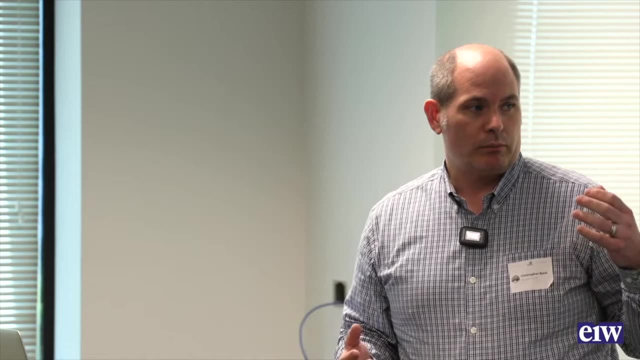 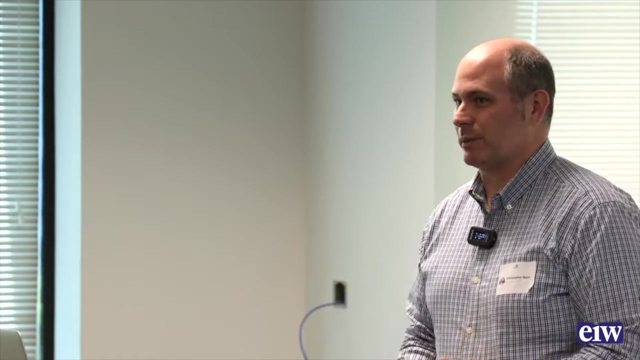 So we'll start off with demolition and abatement, And we're going to talk about both building demolition and site demolition. But before you start talking about demolition, there's always one activity that always goes first, and that's abatement- Hazardous material abatement. 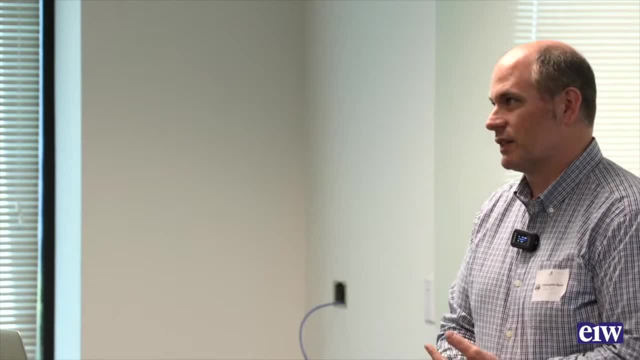 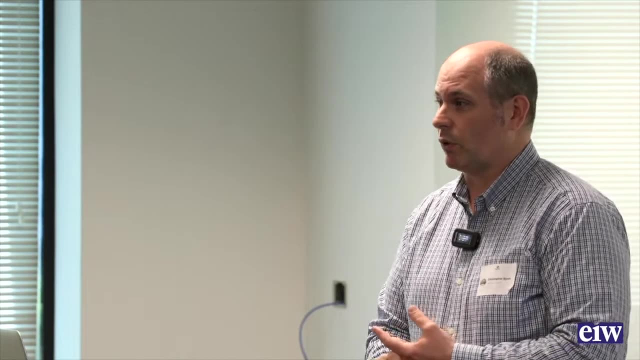 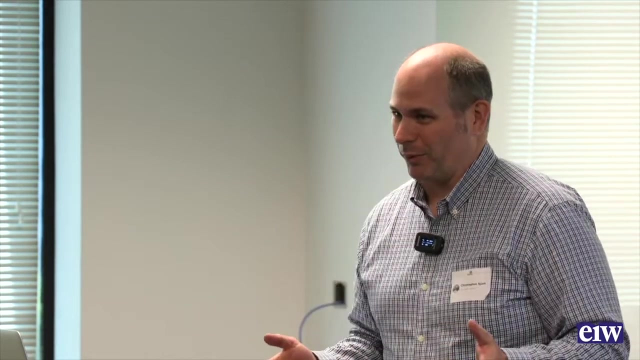 So you want to get asbestos out of a building. It's the lead out of a building, The CFL bulbs, making sure that you have all that, those hazardous materials, safely out of a building before we get in and start doing the work. The great thing about that is that there's usually always a hazardous material report. 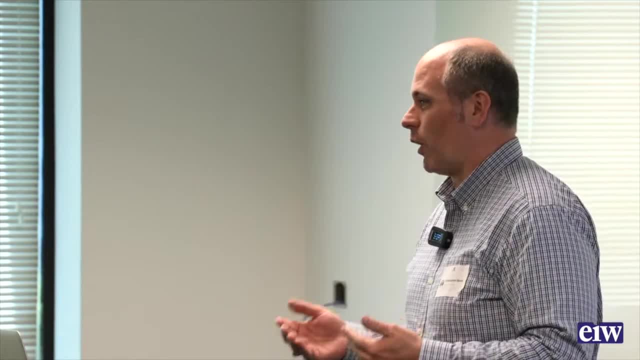 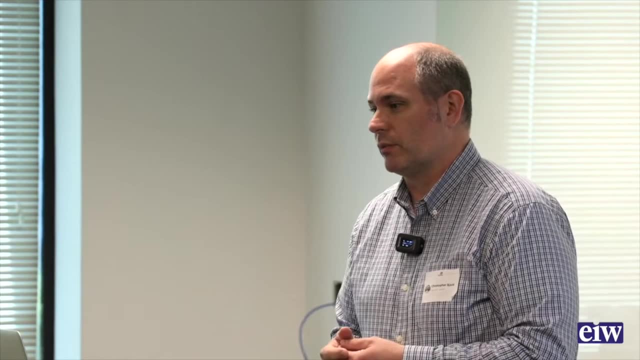 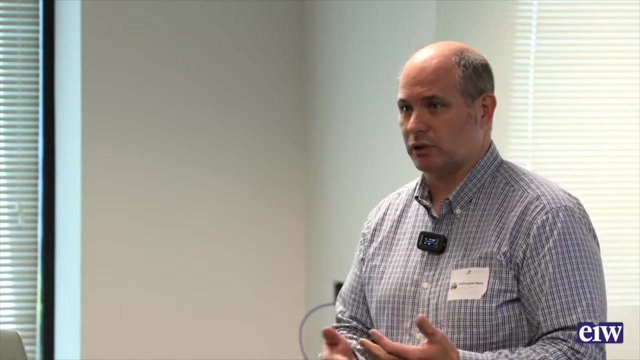 And in those hazardous material reports it will actually tell you quantities of materials from a survey that they do. You can rely on those materials. You should always check with the demolition drawings and any drawings that they have provided in that report as a back check to make sure that there's not maybe an error in the report itself. 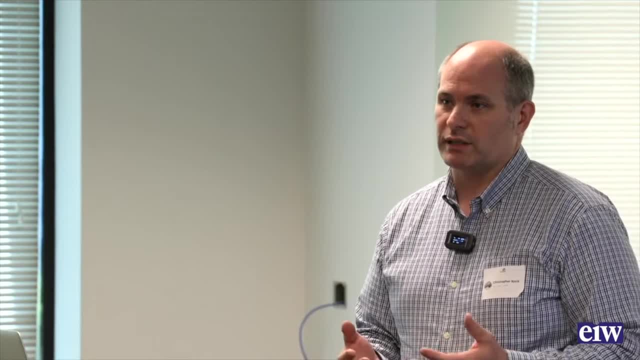 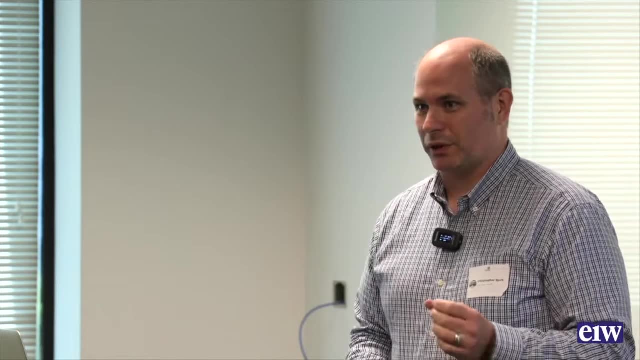 But you can rely on those quantities and that's a great advantage. The things that you need to know about hazardous material abatement, if you're looking at it, are the things that aren't in the report, And that's the access. 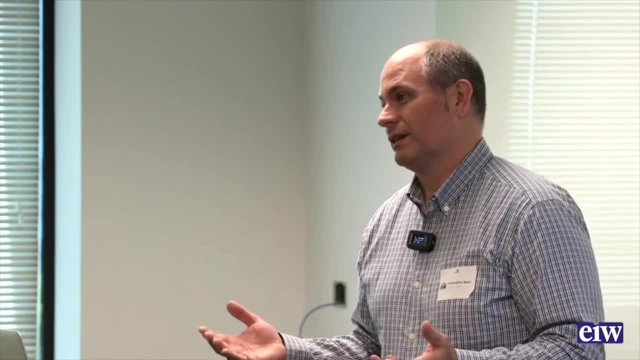 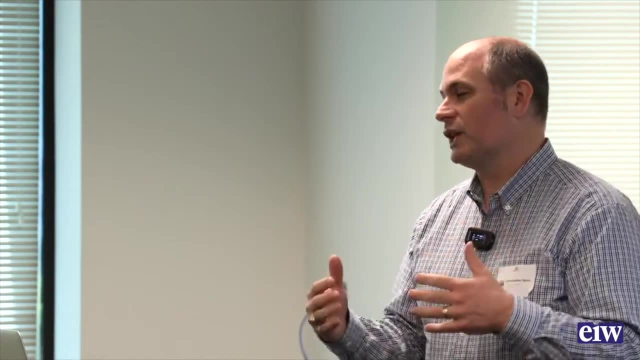 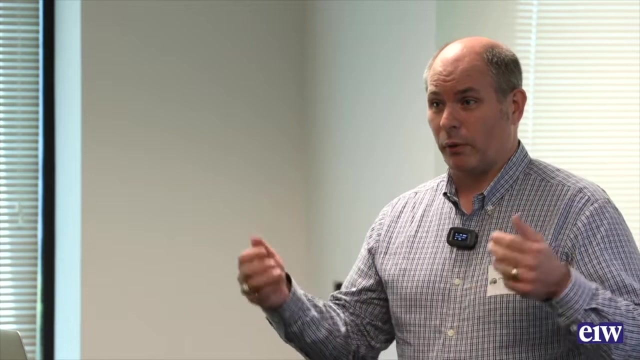 What do you have to do to get to the abatement? We actually had a job where we were going through abatement. He had a precast façade project built in the 60s so the fireproofing for the attachments of that precast façade had asbestos in it. 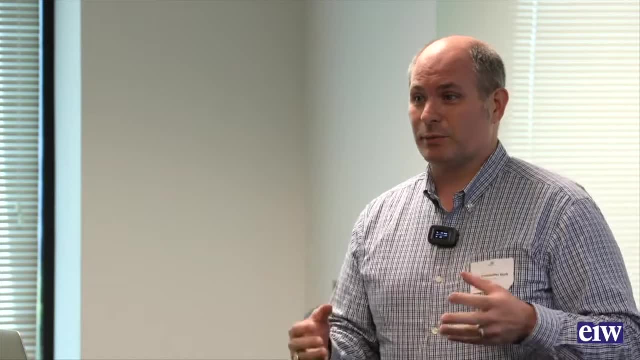 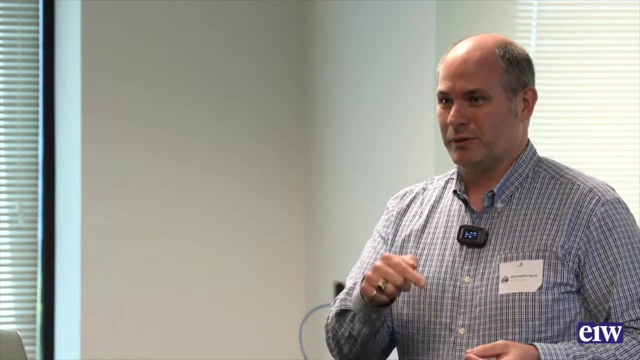 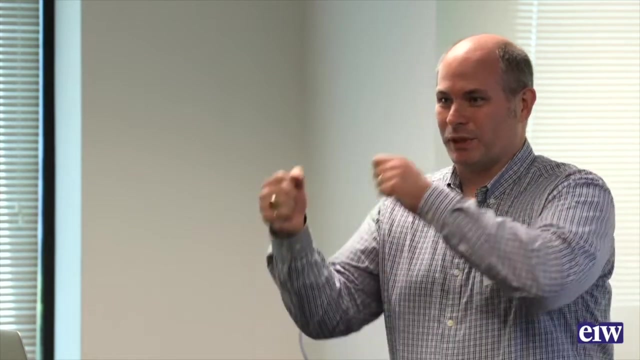 You needed to get in there and abate it. The attachments were behind a column on the perimeter. The only way to get to the attachments to abate the fireproofing was to take the precast panels off. They were off of the building, abate and then put them back on the building. 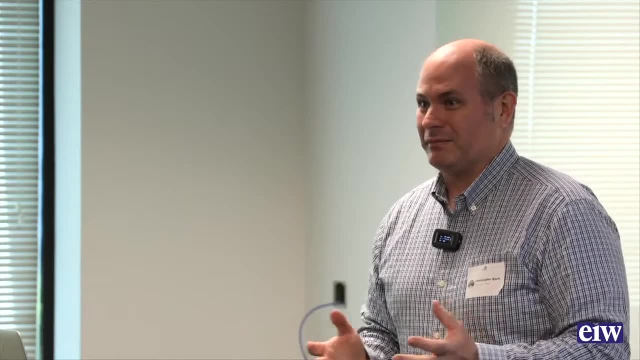 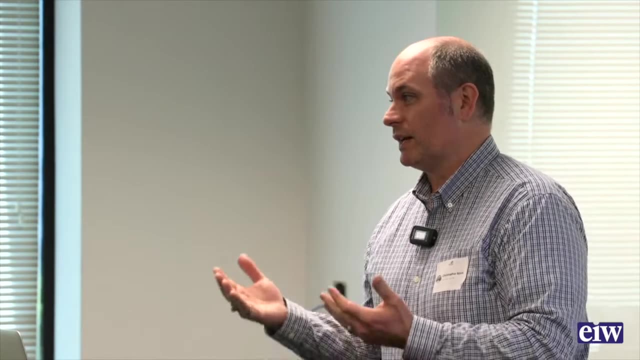 That's not on a drawing, That's not on a hazardous material report. So you have to be able to look at the work you need to do and what access you have to get to it, to make sure you realize some of those logistical things. 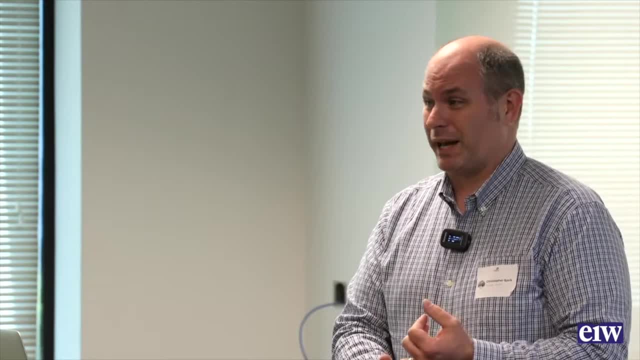 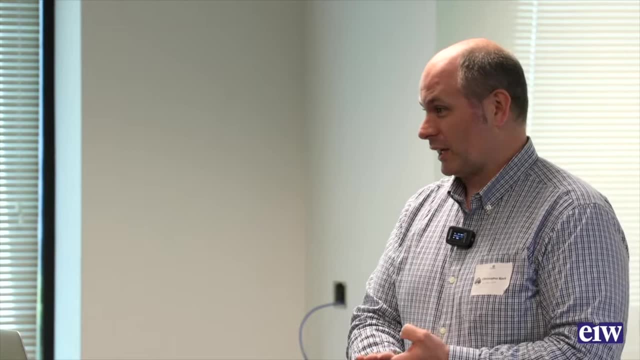 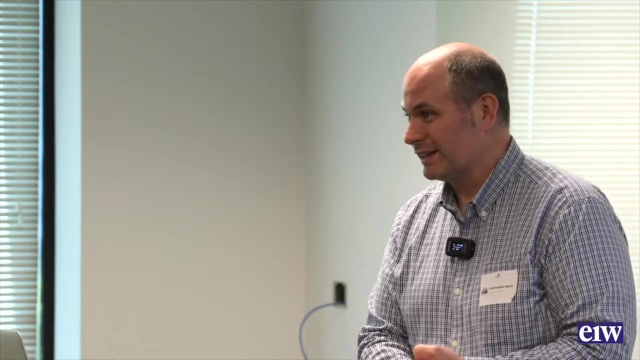 Because paying for a crane, taking off a precast panel, having outside access to fireproof and then putting the precast panel back on, that's a lot of cost that if you didn't realize that you needed to do, it's not something you want to find out after the fact. 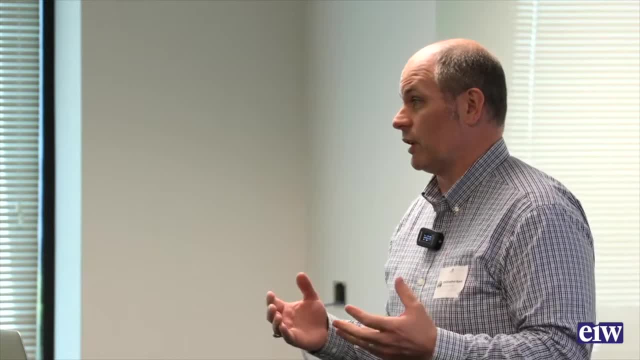 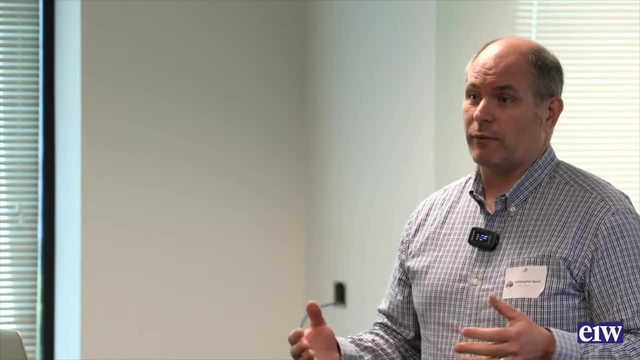 But you also need to coordinate with the demolition too, because demolition and abatement really go hand in hand And oftentimes, as a general contractor, we want to have both of those scopes in the same contract, because we want that coordination happening at that intimate scope. 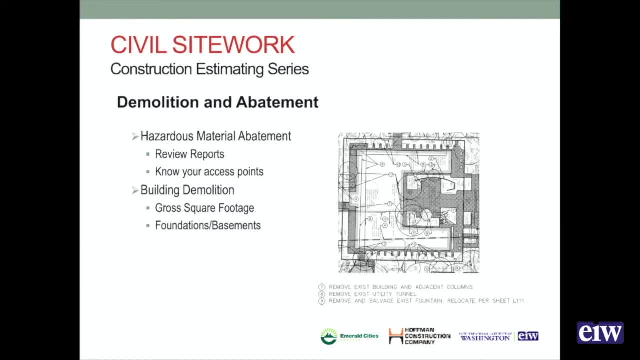 Subcontractor level, where whoever's doing the demolition can make sure that they coordinate with what's abated and whoever's doing the abatement can coordinate with what needs to be demolished before they can go in and do the abatement, and that there's a coordination there. 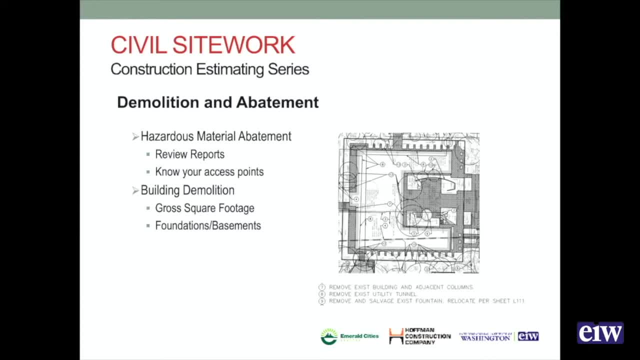 to make sure everybody's working as efficient as possible. Moving on to building demolition, that's where we're taking a whole building and we're taking it all down. The way that I look at it, the way that I look at building demolition, is by the gross square foot of the building. 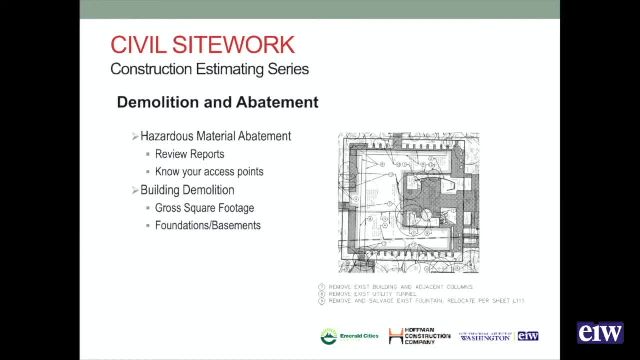 So take all the floor areas and add them all up and that's how much gross square footage you have. That tells a lot about what the kind of volumes you're dealing with. And then you have to really look at what type of how are you going to demolish the building. 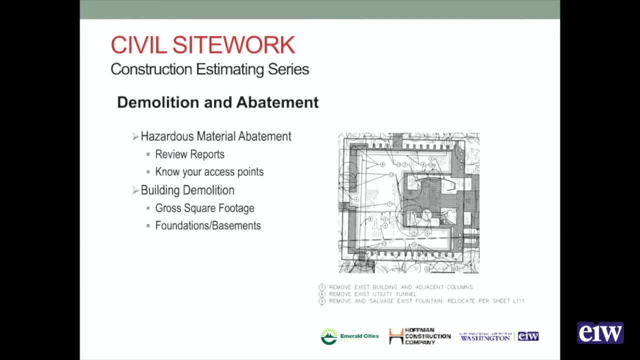 Are you going to do an implosion which is on the very high end of what works? What are you going to? take an excavator and put claws on it and systematically take it down? The cost for building demolition it can range from $5 a gross square foot. 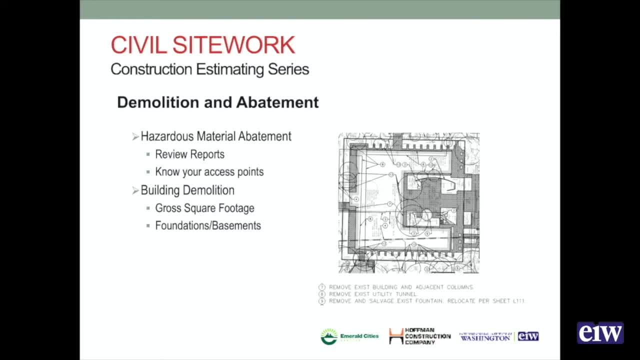 up to $20 or even higher, depending on what work you have to get done. The other key thing about building demolition- if you're looking at building demolition- is: what are you going to do with foundations? What are you going to do with basements? 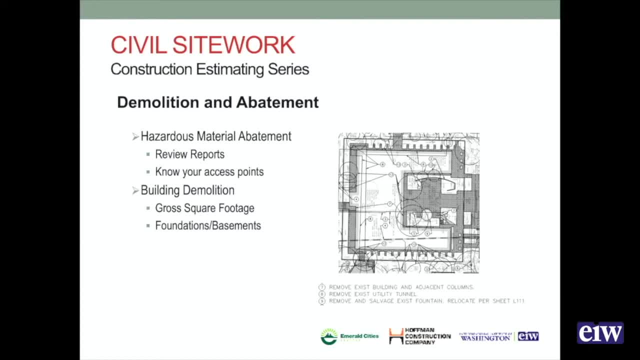 Because if you have to pull out the foundations, that is going to be a big deal, because pulling a footing out of the ground is a cost. It takes cost, it takes equipment to really do that And if you're going to, you might grind them in place. 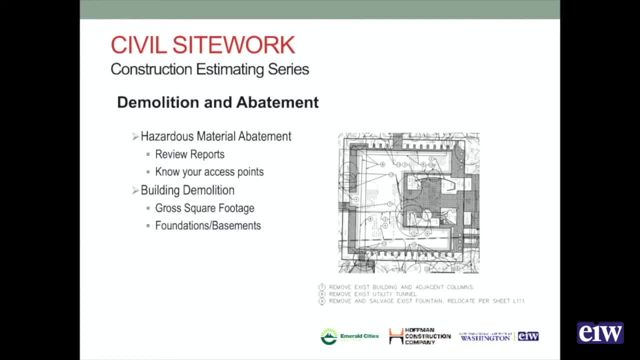 That's a common thing. where you take concrete, you grind it in place, use it as fill. If you're going to, if your building has a basement, you need to know: do I need to brace the exterior walls as I take the building down and suddenly there's not? 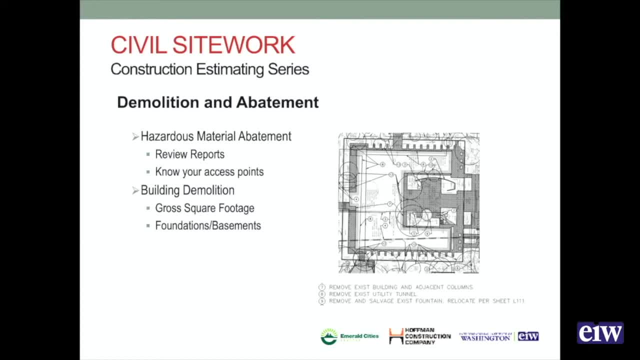 a slab on top of it that's holding the building down? Are we going to leave the wall, the top of those walls, up? Are we going to leave the basement in place? Are we just going to sometimes you leave the basement in place? 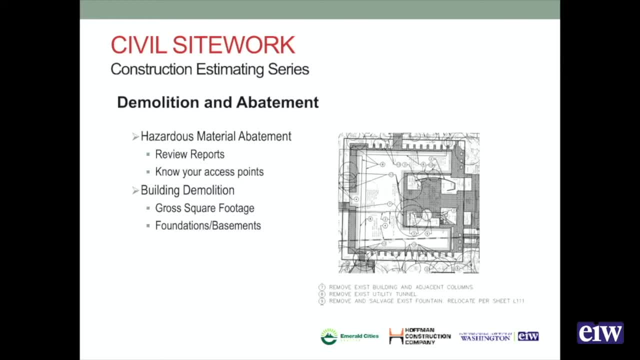 and you cut holes in the slab to allow water to get through and then you just fill the basement up with gravel. Those are things that will be on the documents and it will tell you what work you need to do, so you can take into that into account. 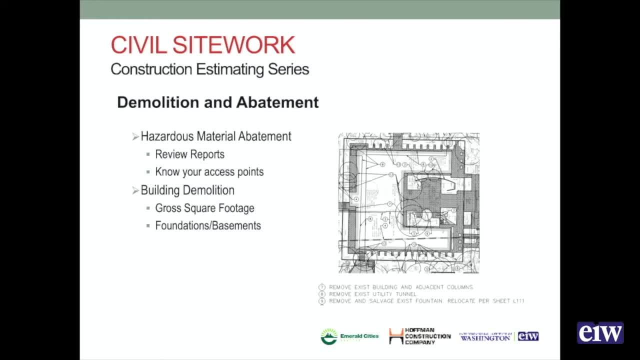 when you prepare an estimate and what that's going to cost Chris. one other thing that we've been caught on before is abatement, where the report says, hey, you need to take care of, say, paint of some sort, but it doesn't necessarily say what you have to do with that. 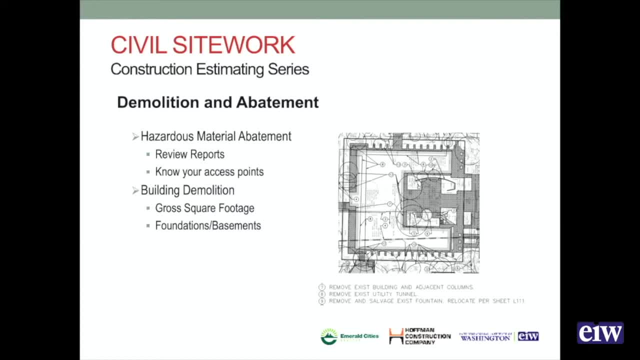 And we had an instance where you're demoing walls as part of the demo contractor and it has lead paint on it And it may not be lead paint to a point that you have to peel it off and abate it, but that still lead paint to a point. 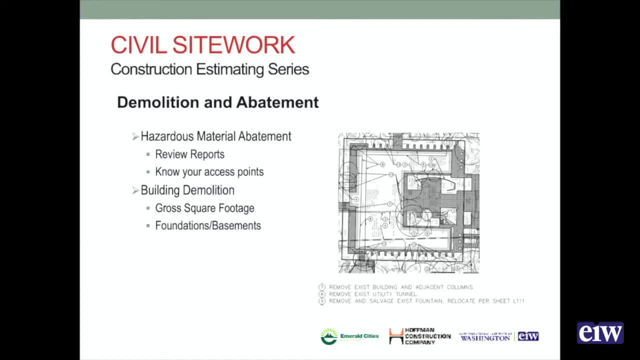 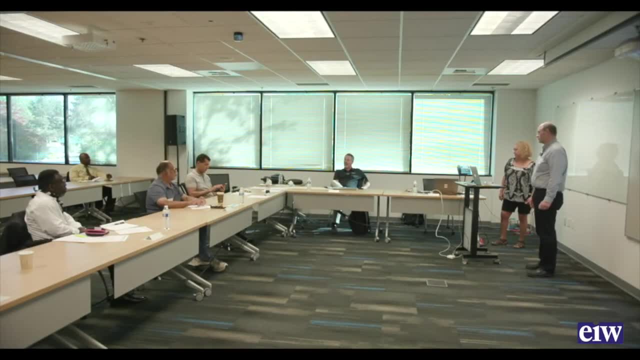 where it has to get taken off to a higher quality landfill And at that point you're paying an extra premium for that. It's a gotcha that it's not Exactly Well. that's a great point too, especially with dealing with the abatement. 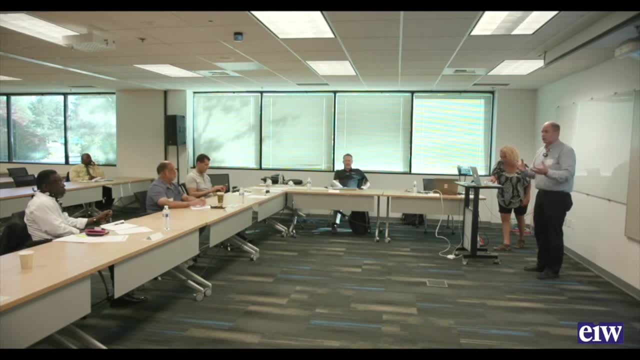 or this would go into contaminated soils, which is related to the hazardous material abatement. You need to know what level of contamination that you have so that you know where you need to take it And in certain levels of contamination, could be taken as far as Umatilla Oregon. 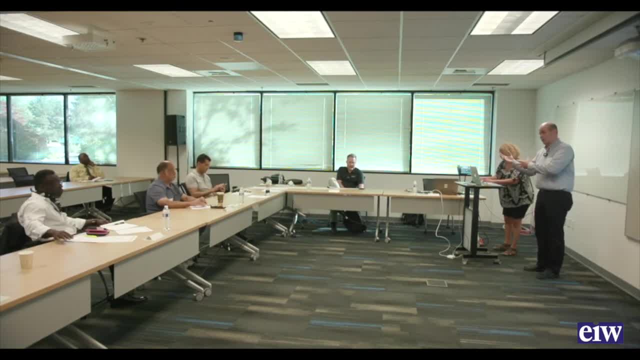 because they're at a higher concentration and that's where the facility might be. Some are low enough concentration where you can still take them to the landfill, But you need to understand what that is so you know where you need to take them, because where you need to take it. 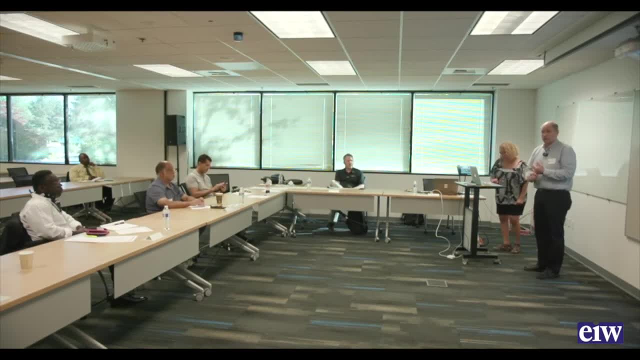 is going to affect how much it's going to cost, both in transportation costs and the cost to the tipping fees, that you have to drop off the material at the site. How about, Yes, If I were your environmental consulting company, my job would be to try to save you money. 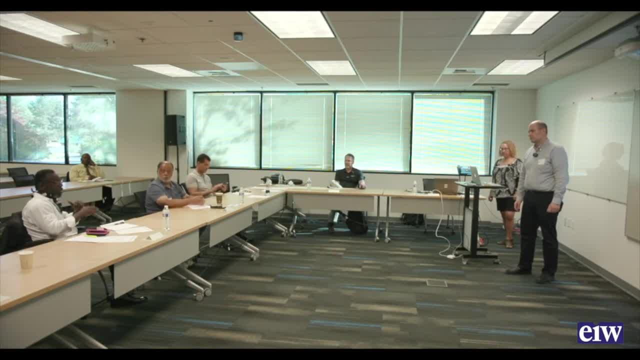 And so before I go in and say here's the report, I would make sure you would have a T-clip, knowing that all the material that you have is below a certain hazardous material percentage. And because it's below that percentage, I can save you money. 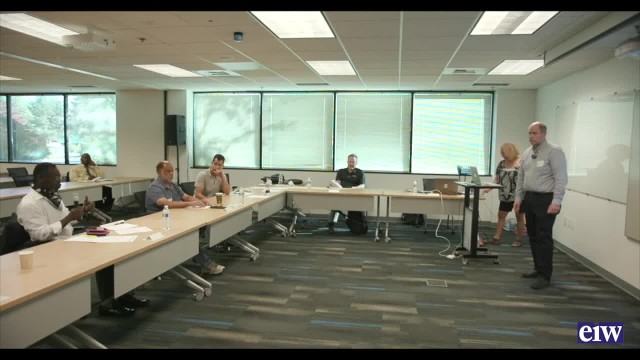 And if it is a problem for us to remove asbestos-containing material in between another material, we can always encapsulate and still save you money, Absolutely. So that's the name of us as a subcontractor is to help you save money and help us all become successful. 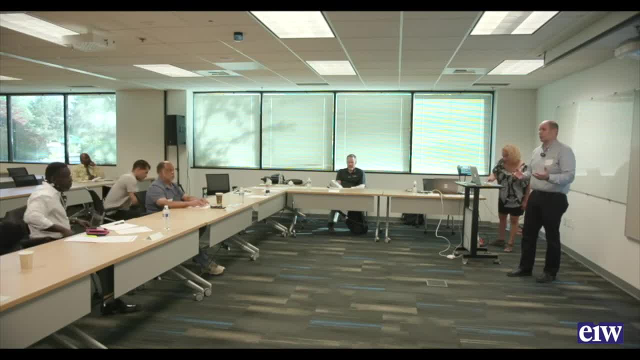 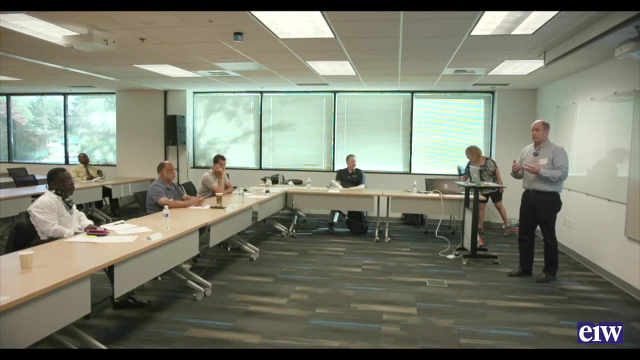 That's a great point. Sometimes, with hazardous material abatement, there are other ways to encapsulate it where you don't have to necessarily abate it, And that's a great point that sometimes you need, Even once construction has started. don't be afraid to. 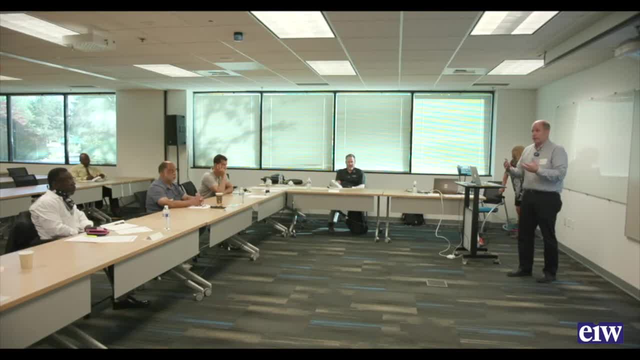 If you see a way to save money that provides the same level of quality at the end of the day, Those are things that we take into account even once we start construction on, Because that's a value to not just us as a general contractor. 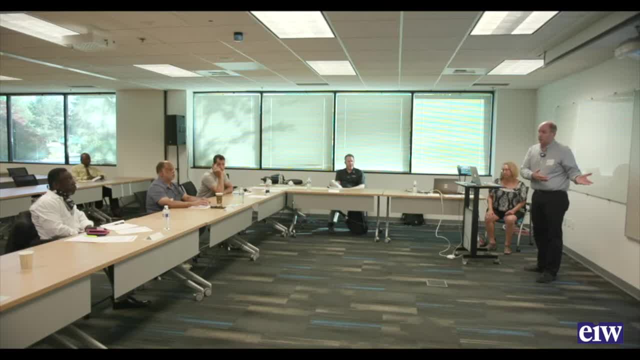 but it's a value to the client that we're working for as well. When we can think, Think of a better way to do it that saves money, provides the same level of quality. that's a win-win for everybody. Moving on to types of demolition: 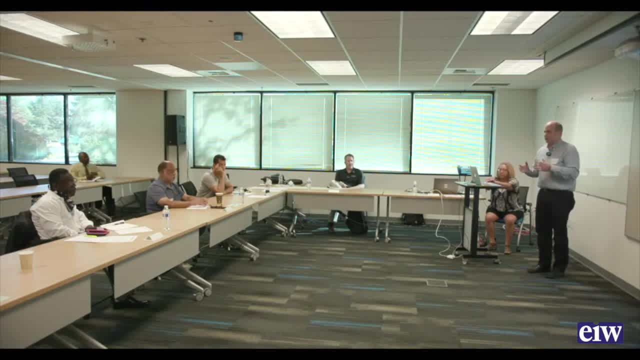 selective demolition. This is more of the surgery demolition. It's going in you're. You might be taking Demolishing a floor, you might be demolishing a room. This is where there's a key quantification of scope that you really have to have. 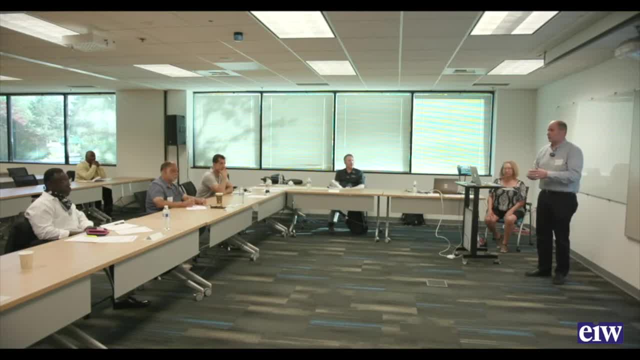 Here's where you will have demolition drawings, Floor plans that show what walls are going to be demolished, what ceilings are going to be demolished. You'll have keynotes that tell you exactly what scope needs to be in work, because they will tell you exactly what needs to happen. 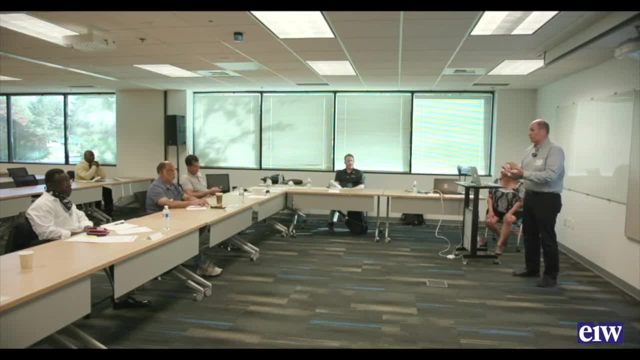 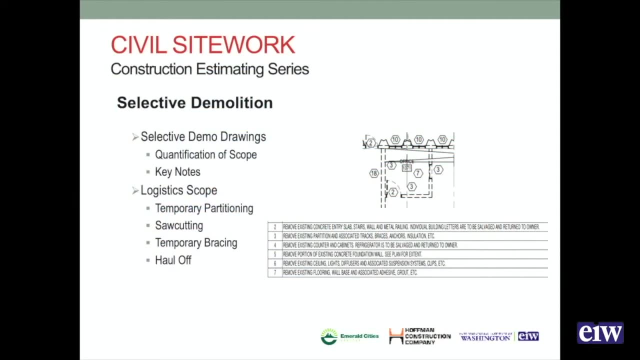 Salvaging something needs to. You need to take some care when you remove it so that it's in good shape when you give it to the client. But it also tells you. You might have one keynote that has some dashed lines around it. That keynote tells you what scope of work. 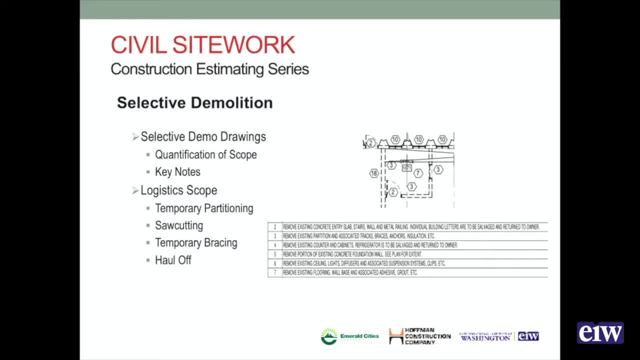 needs to be done with it. A lot of things with selective demolition are making sure you know your logistics. Think of how you're going to do the work when you do it. Demolition always has temporary partitions. Oftentimes you are in an occupied building. 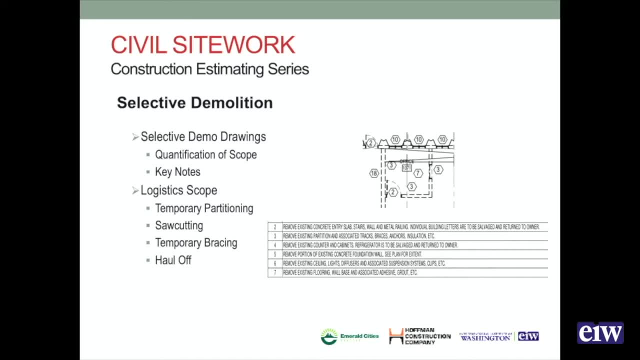 You may be in a hospital where you're doing temporary demolition, so you need to have that secure perimeter so that dust and debris don't go out into the hospital, but also so The people who are supposed to be in doing the work have a safe place to work. 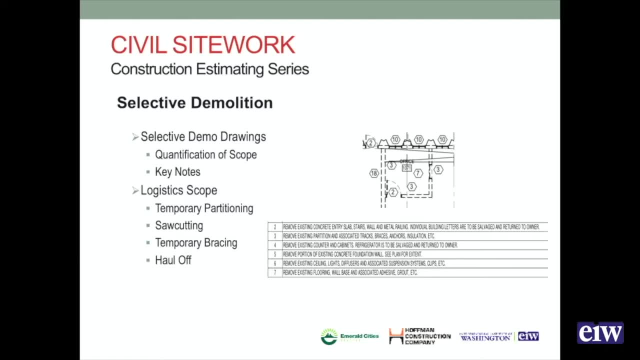 and the people who are not supposed to be in the work area are stayed out of the work area and don't go into a place where they could be in danger. That cordons off that area. but you have to think about what work and what your sequence of demolition is. 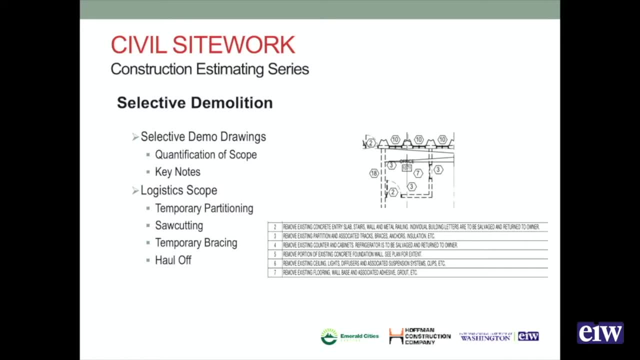 to make sure you move those partitions and set up the partitions so you have a secure perimeter. Saw cutting is another thing that isn't always shown on demolition drawings, because you may have a 30-foot long concrete wall but you're only going to demolish. 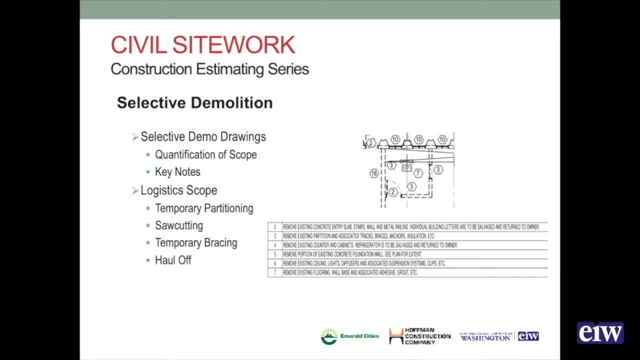 the middle 10 feet of it. It will most likely show you demolishing that 10 feet, but it won't tell you that, hey, you need to put saw cuts on either end of that demolition zone. So you have to look at that. 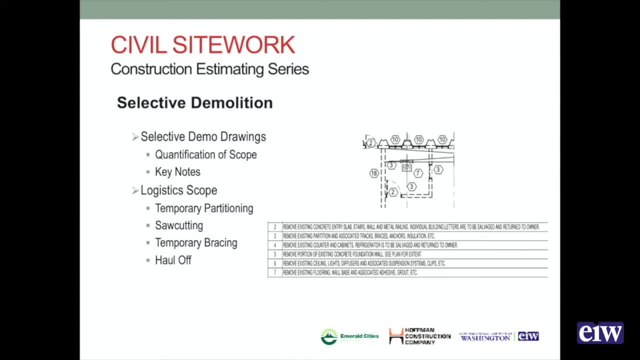 and know what your means and methods are to perform the work and what your means of doing that are. Temporary bracing is another thing. We've even seen projects where you have to demolish a bearing wall, so a load-bearing wall- in a building. 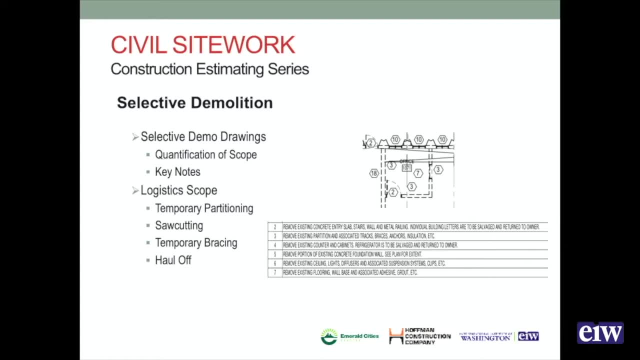 Well, to do that, you need to know that I'm going to need to put some shoring on either side of that to make sure that, as I demolish this wall, the load that it was carrying has another path Until someone can come in. 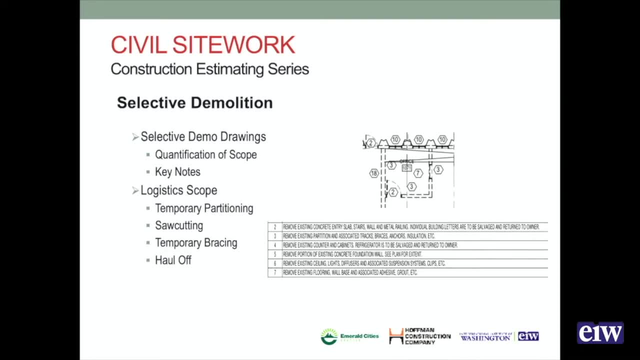 and put in the replacing structure for it. Those are things that are means and methods, so they're not always necessarily shown on the drawings. There may be a note that says, hey, you need to shore this, but they won't necessarily tell you how to do that. 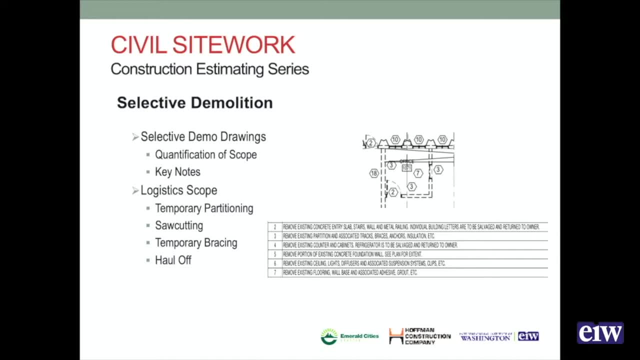 So the means and methods are things that you need to think about when you do a demolition takeoff on what's the most efficient thing, Because sometimes, if you have a large enough area on a ground floor, it may be the easiest thing to do to go in there. 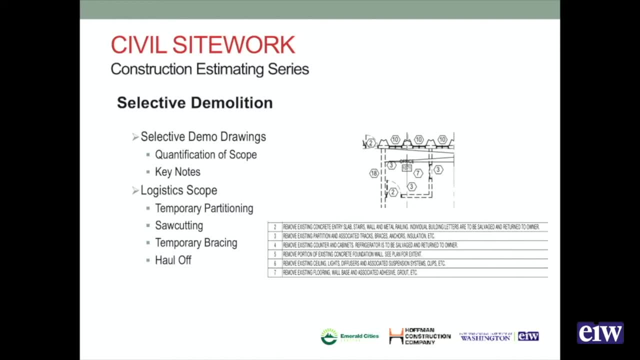 put a temporary partition on there and go in there with a bobcat- if the bobcat can be supported on the slab- and just start knocking things over Once it's all safed off, and if you don't have load-bearing walls in there. 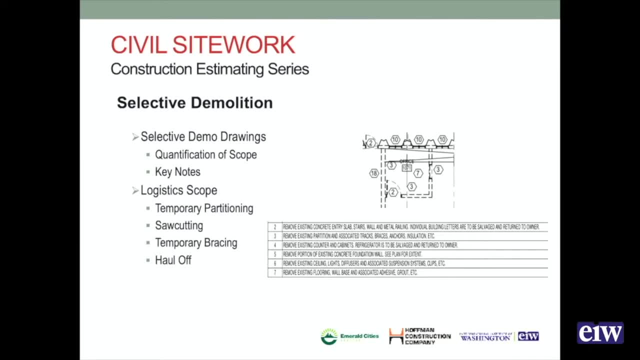 that may be the most efficient way to get the materials out. Last thing that you need to be concerned about with selective demolition is your haul-off. So you're going to need to load all this debris out and either put it into a dumpster. 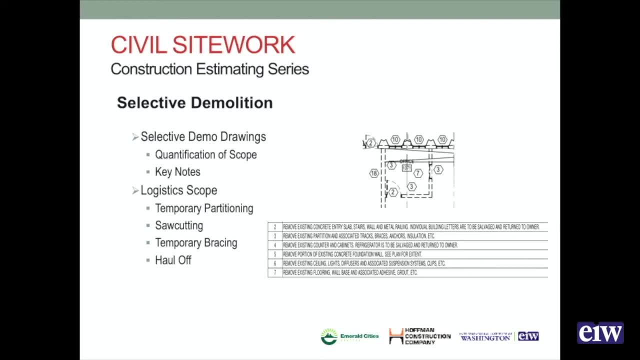 and maybe you're fortunate that the general contractor is going to pay for the dumpster and have it hauled off. Maybe it's a large enough scope where you need to provide the haul-off as well. So that means you need to know how much things weigh. 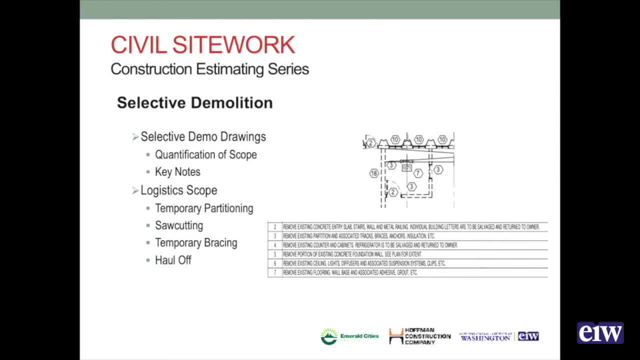 There's a number of different ways that you can find out how much things weigh, because what does a drywall do? What does a drywall partition weigh? You know, pounds per square foot. Well, if you look at trade publications like the Means Guide, 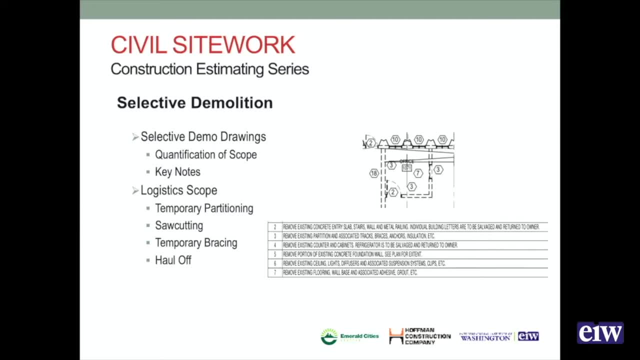 or a local one that's called the Guide. they actually do have weights per square foot for some of these demolition materials and what these construction materials cost. I actually use the AISC, the American Institute of Steel Construction, Their design manual, which I got years and years ago. 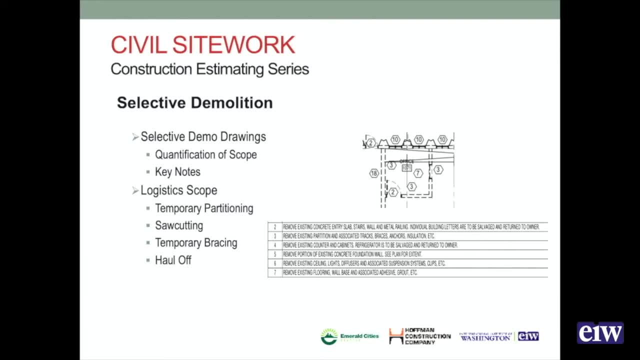 of all the things in the back of the steel design manual. it has weights of drywall partitions, soil, different types of soil, CMU walls. It has all this extra information in there. that is incredibly useful because once you know the weight of everything, 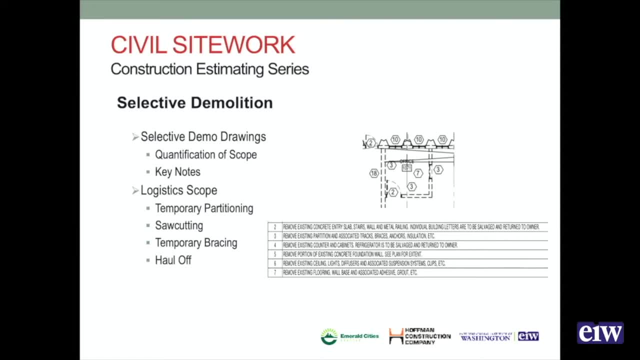 then you really know what it's going to take to both haul it off and then to get it into a truck, drive it to someplace, and how much of a tipping fee I'm going to have to pay at the landfill to dump everything. 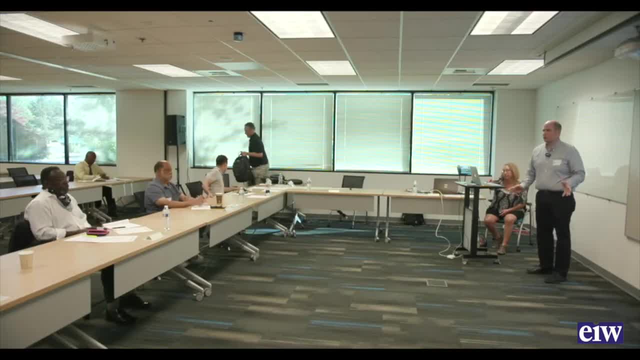 The next, the final part of demolition is site demolition. So this is where we're doing everything on site, where oftentimes there's a. I always see a little confusion on. you know site demolition. what's site clearing? Because you'll see them used interchangeably on jobs. 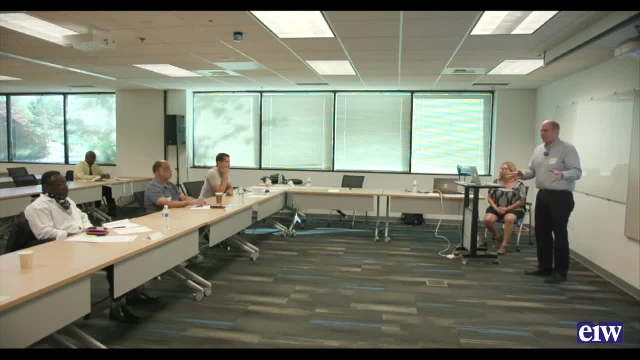 For this presentation. site demolition, in my mind, is hardscape, It's paving, it's curbs, it's, you know, benches, pipe, bollards, those kind of hard materials there. Site clearing is your landscaping, it's your vegetation removal. 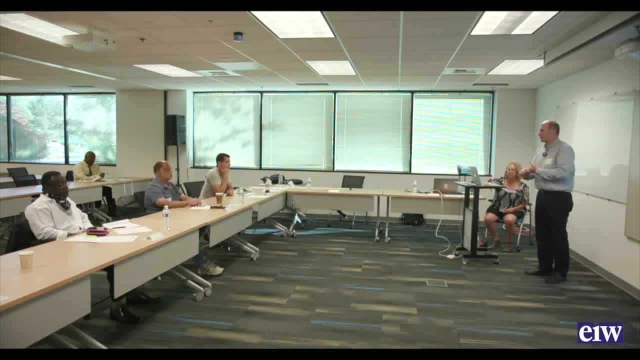 it's stripping off topsoil. it's taking down trees. if you need to, Scopes that you will typically find are paving. So you look at paving. look at the area of paving that you need to demolish. How many lineal feet of curb? 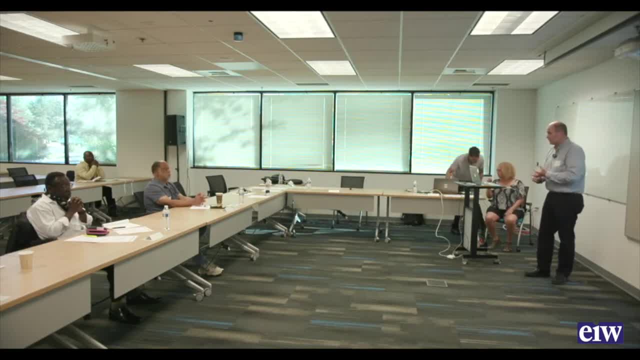 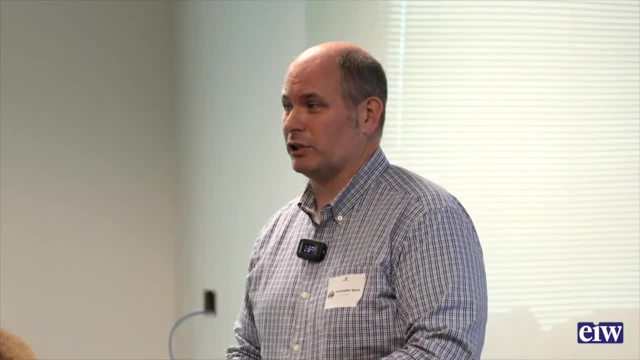 are you going to demolish Walls, you'll need to know the area of the walls and sometimes that takes a little bit of work to do because oftentimes on a site demolition drawing they will show you the length of the wall that needs to be demolished. 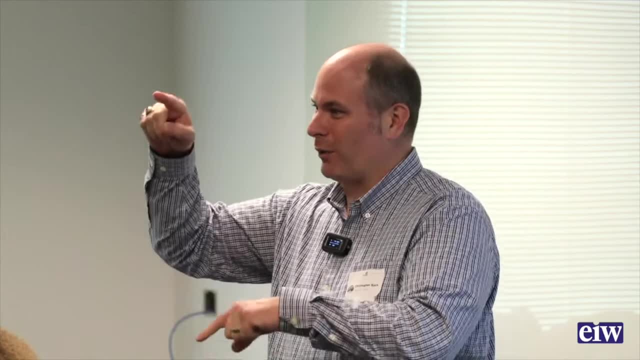 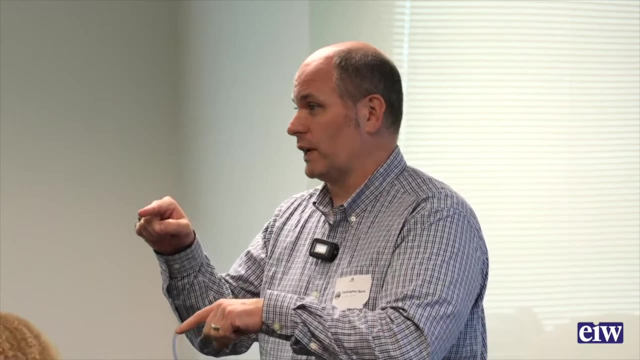 But you need to go to the existing site survey to find out how tall that wall is and actually piece together the dimensions and the elevations off of the site survey. The other thing to always remember about a wall is that they usually have footings. 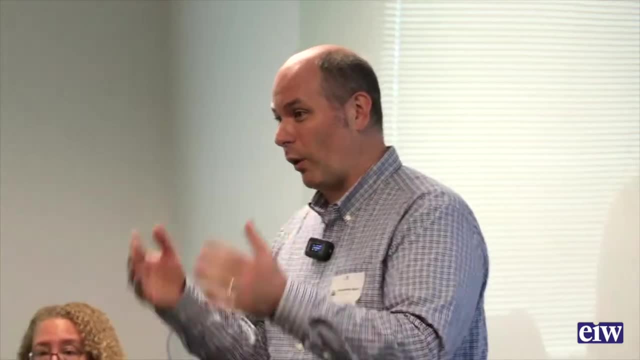 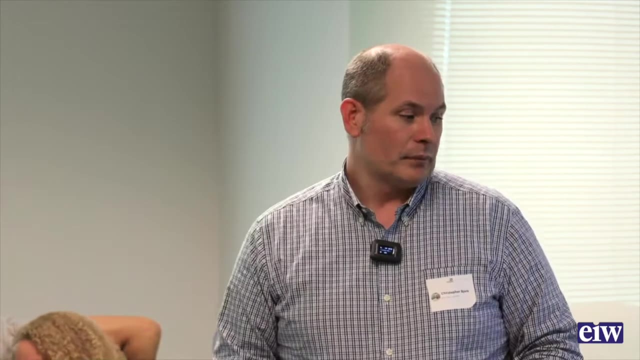 So realize that there is more than just the wall that you're going to have to demolish. There's usually a footing underneath it that you're going to have to take and demolish as well. Site furnishings are counts. How many benches do you have? 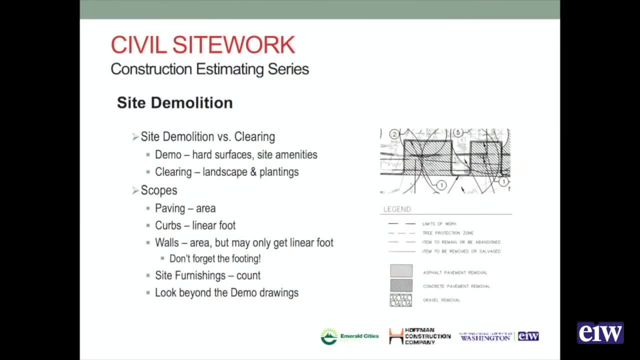 How many pipe bollards do you have? How many site railing do I need to remove? The key thing that I've always found with site demolition is to really look beyond the demolition drawings, And it's not uncommon where I overlay an existing site survey with, say, the grading plan. 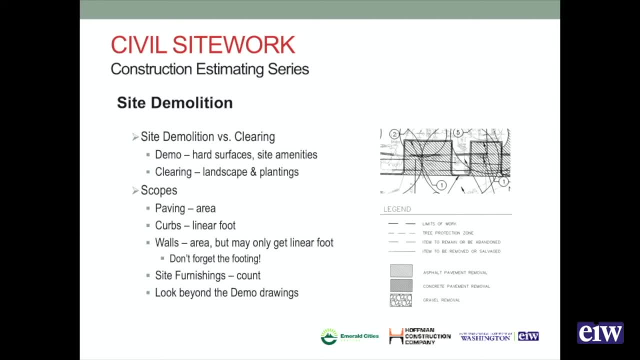 and find out that the actual paving that needs to be demolished might be two or three times as much as shown as on the site demolition drawing, because you're grading over the top of existing pavement And you don't actually necessarily see that until you overlay it. 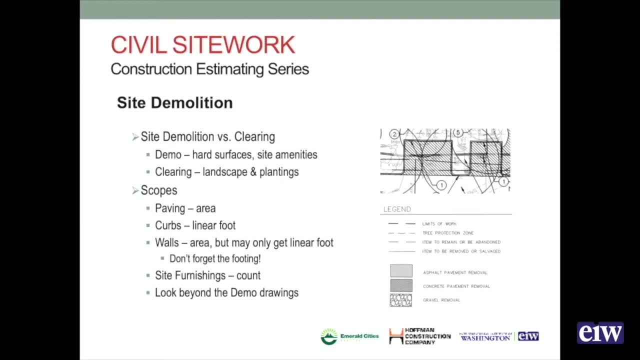 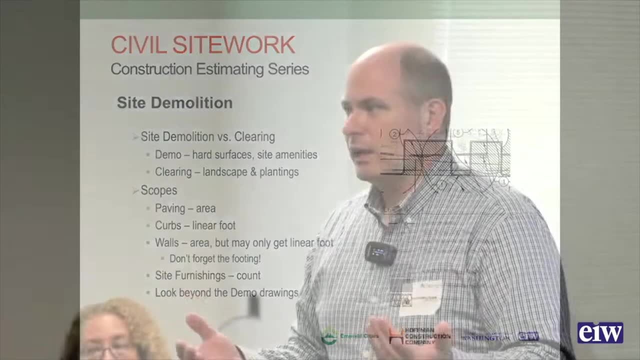 And some of that time is that there's just often so many little parts and pieces and they're in light faded print on the site survey that they don't make it over into that site demolition drawing. But you need to be able to look and overlay that. 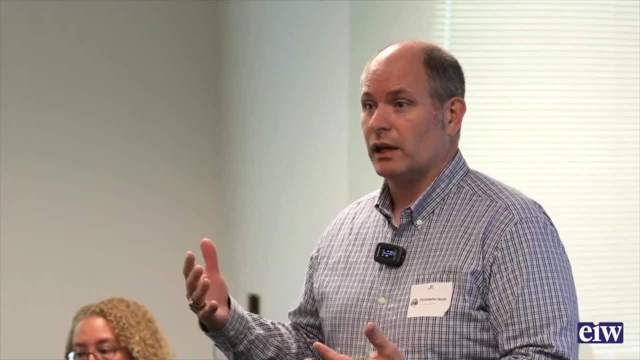 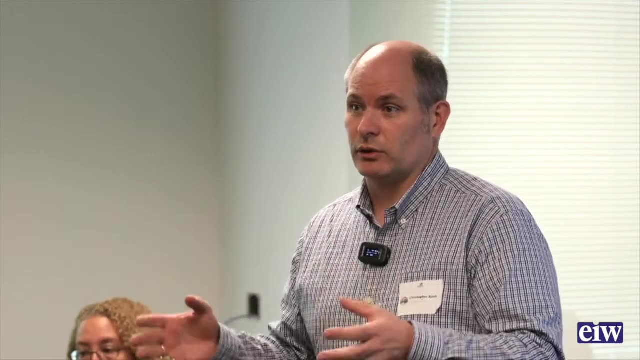 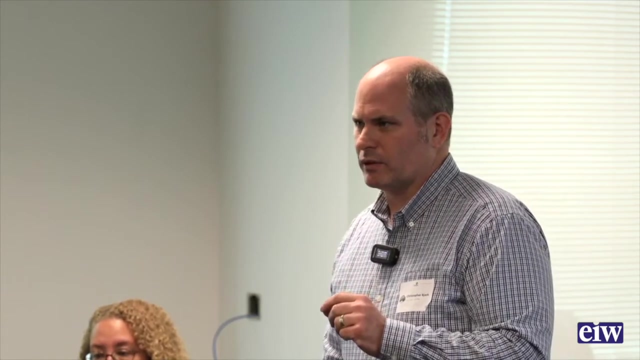 and see what work needs to be done from the actual grading drawings and paving drawings that you're doing, where they show the area of work that you're actually getting into and doing that work. That's the key thing that I would say. with site demolition, that is the most frequent thing that you can get burned by. 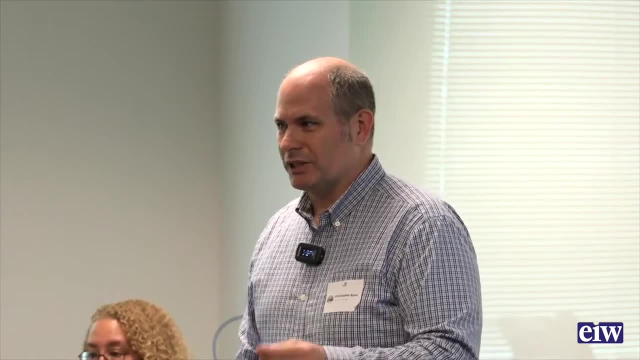 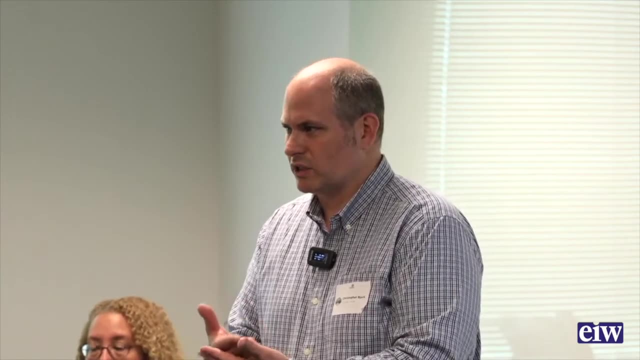 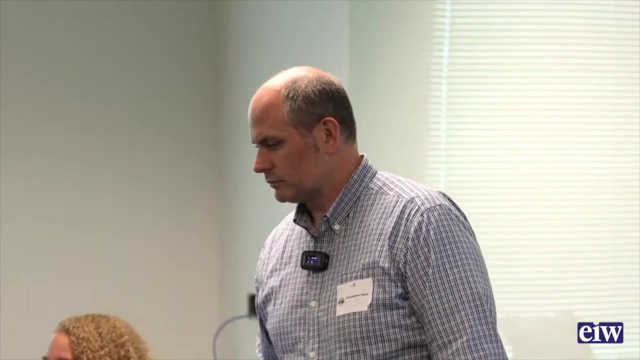 is that something is shown but it's not really shown. So you just have to do the work to overlay those drawings and see where those limits of actual work are and how that compares to what you have on an existing site survey. That brings us to earthwork. 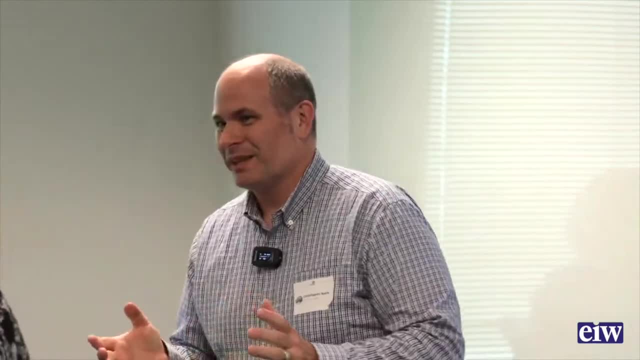 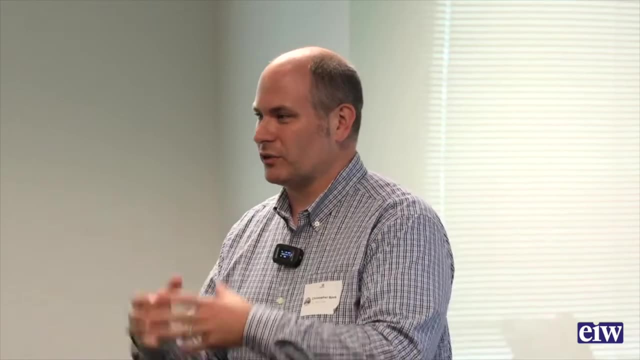 So the first part is the site clearing. That's the first activity that always happens in earthwork And that is: are you going to need to take down any trees? Those are in each count, because a tree can take you a couple thousand dollars to remove. 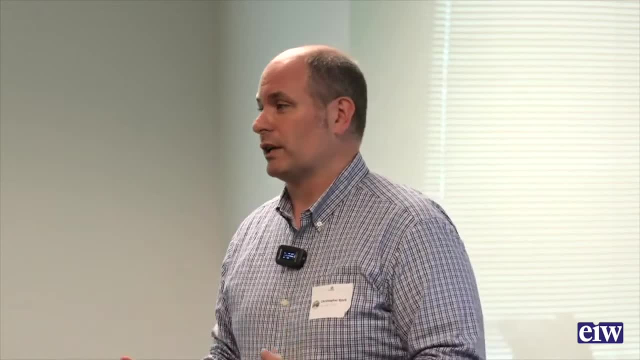 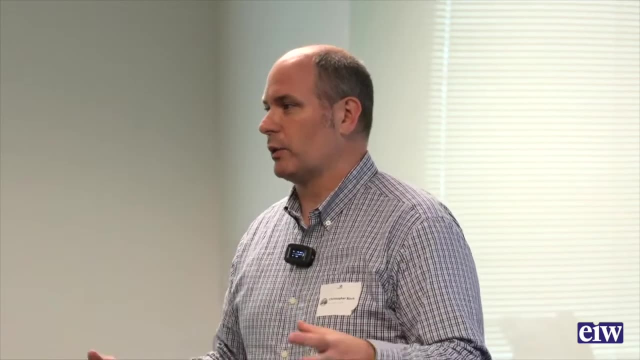 It depends on how big the tree is. It's your clearing and grubbing, getting the brush out. We look at that as on a square foot basis and making sure that we know that. what area do we have to clear, because you'll take a piece of equipment. 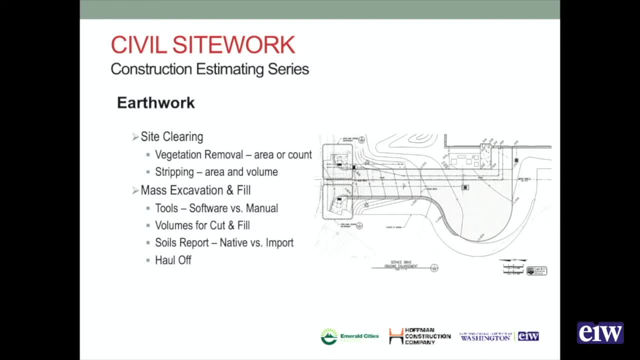 and scrape that off. The final piece of that is your stripping. So that means if you read your soils report. so whenever you start talking about earthwork, always read your soils report because that will tell you a lot of information. It will tell you how deep you need to strip topsoil off. 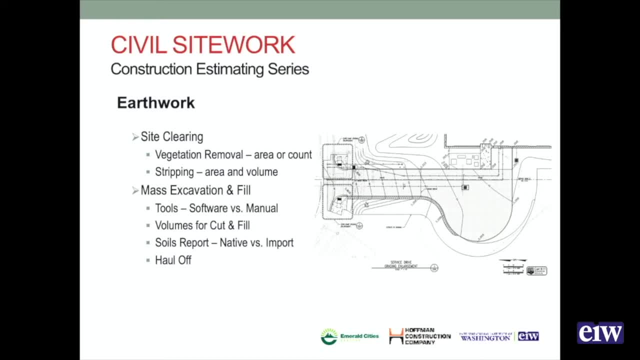 That's only in your landscape areas. You don't need to strip that off where there's paving. But it could be anywhere from 6 inches to 18 inches, And so you need to take that soil off, Because it's the organic material. that's really not suitable. 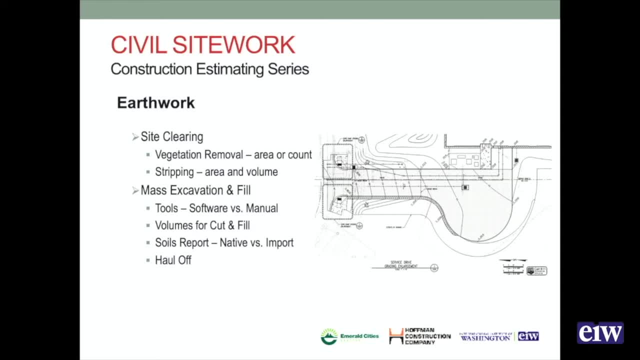 to be used as structural backfill, And then you need to know what you're going to do with it. Are you going to stockpile it on site so that it can be reused as topsoil? Is that allowed? You need to know. 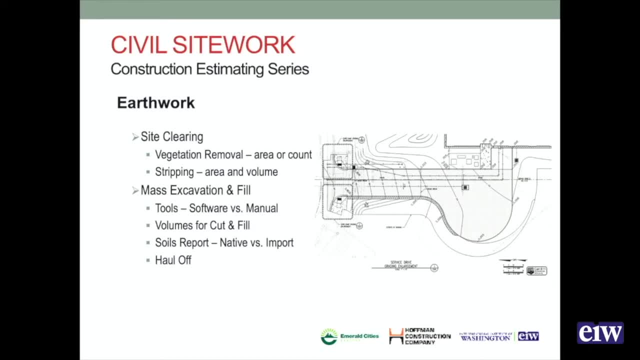 The soils report will let you know, Or you need to possibly ask a question. They may allow that but they may not have mentioned it in the soils report. You might be able to use it for landscape forms Or you may need to take that soil off. You may need to haul it off site and take it to either a landfill or some other place where you can deposit dirt, And so then you need to know what's that going to take And where am I going to take it. How long is it going to take for me to get it there? 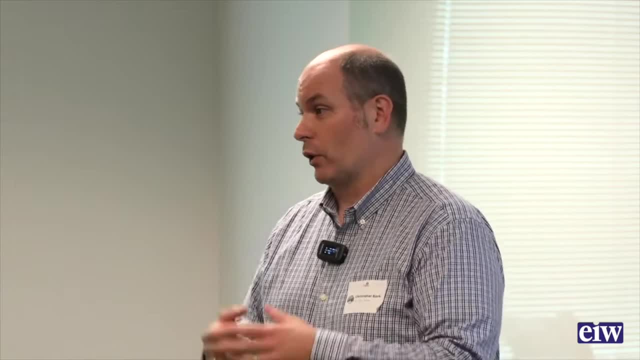 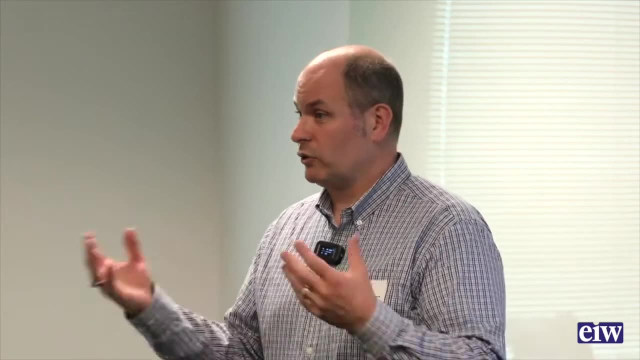 And what's it going to cost for me to drop it off there? Now, if you are doing the earthwork yourself, you may have another site, another project that could use that. Well then, that's something you can think about On both the project you're looking at and the other project. 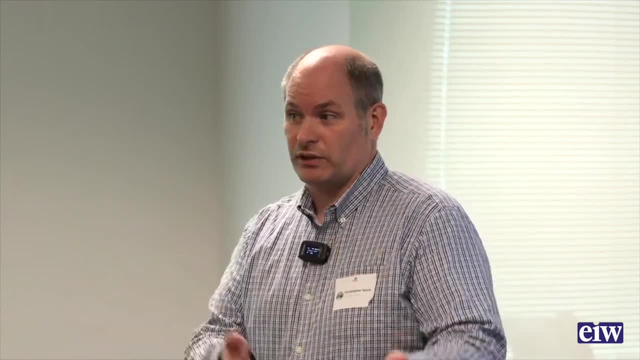 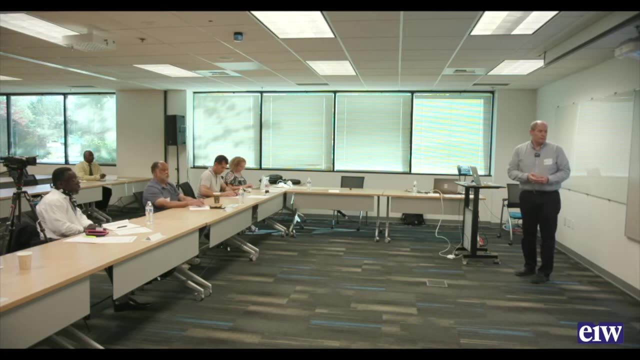 and ways that I can save money. If this soil is suitable to be used at another site, well, that's an advantage that you might have The way. yes, The soils here in Washington State- at least my experience- were finally lead, arsenic, cagnum in the soil and heavy metals. 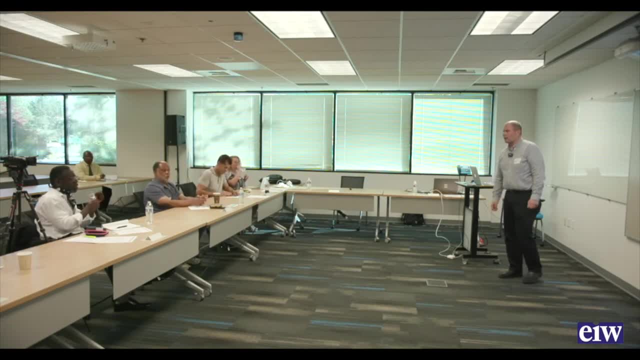 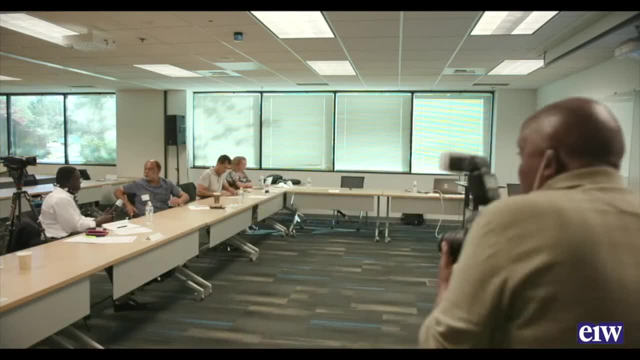 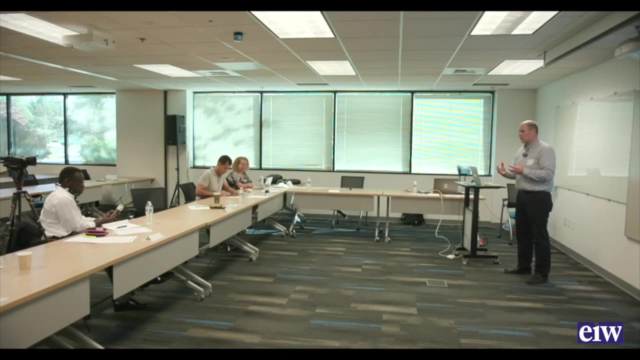 Where are you guys taking that? There are different places. There are sites locally. Really, it depends on what the level of contamination is. It may be a local or regional landfill site. It may be on the other side in the eastern Washington. 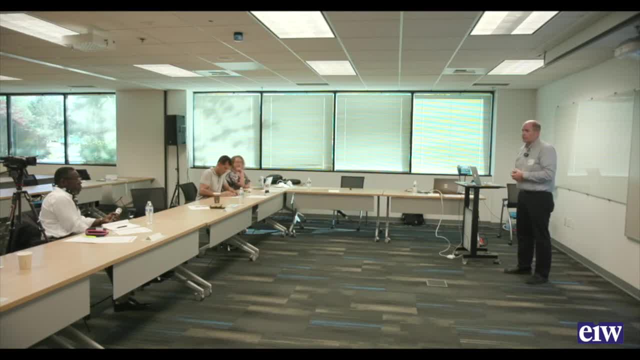 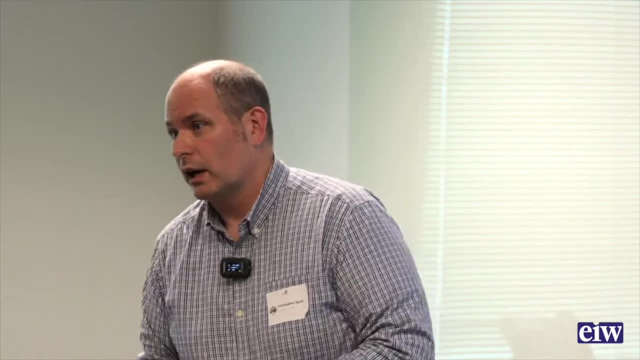 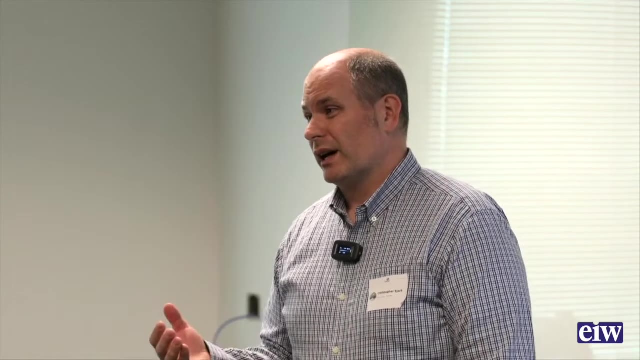 It may be as far as I've had. contaminated soils need to be taken as far as Umatilla, Oregon, which is a ways away, And usually that's by train. it takes to get there And it just really depends on what the levels of contamination are. 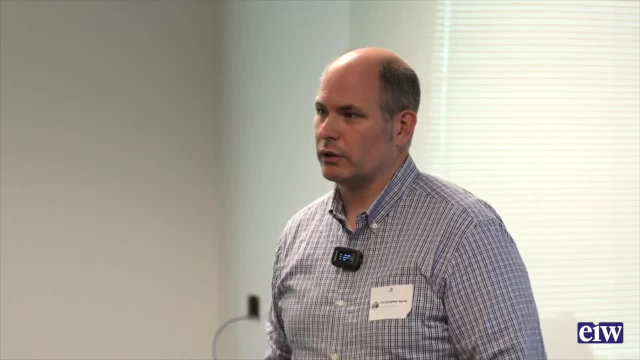 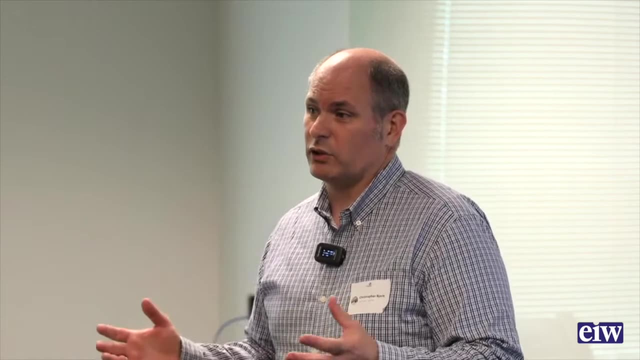 because that's what tells you where you can take it. Some landfills actually can take a certain level of contamination, Some can't, So you just need to work with those landfills. Off the top of my head, I don't know all the different landfills. 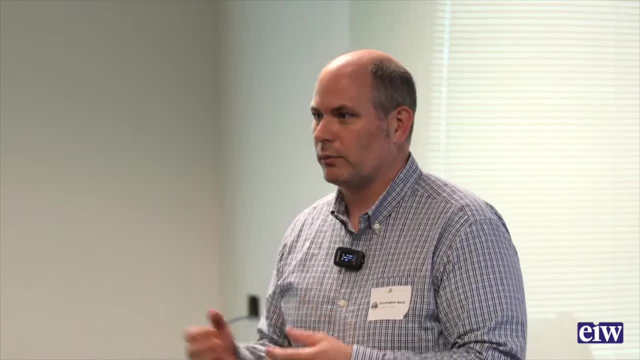 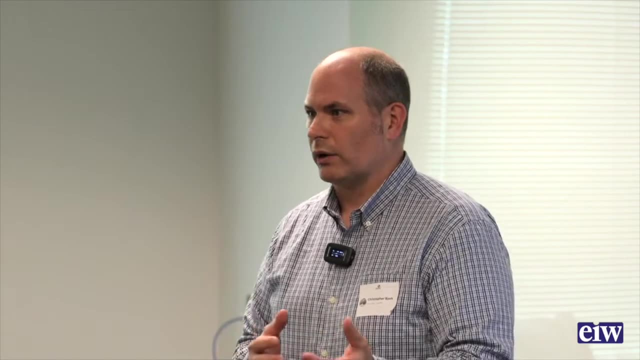 I usually rely on our earthwork partners to let me know, hey, where do you need to take this, And so I can figure out. what kind of a round trip is that going to be? Is it something you can take with a truck? 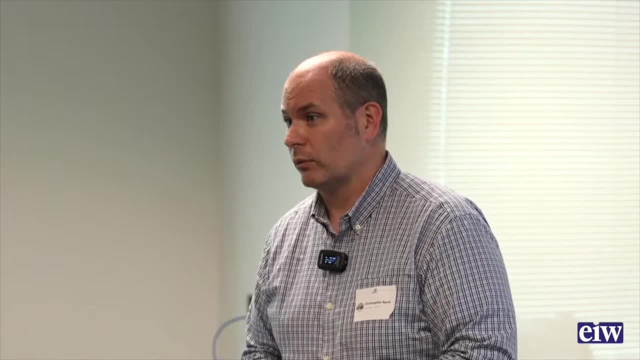 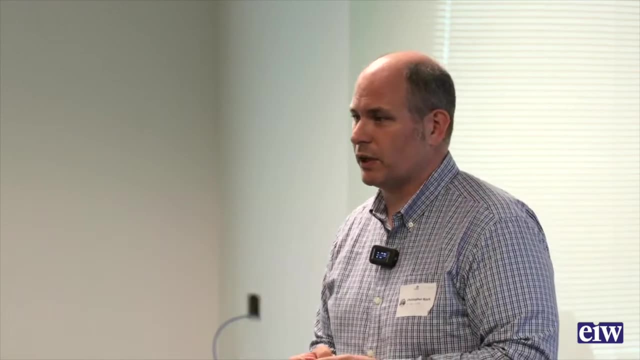 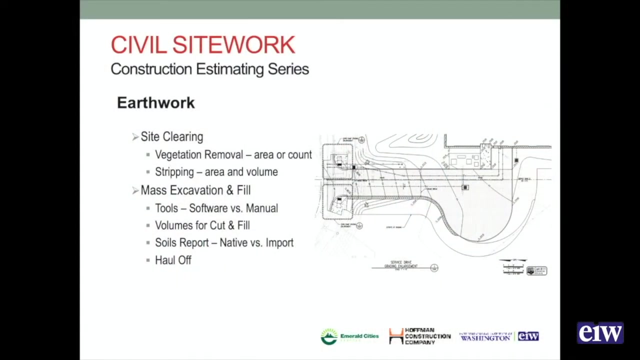 Is it something you need to think about in a different type of transportation method? Then the first types of excavations. the first type of excavation that we talk about is mass excavation, And that is really molding the site. What it's not is it's not digging out footings. 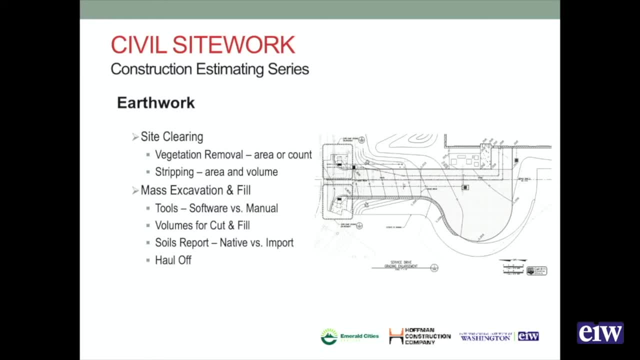 It's not digging out basements, It is grading the site and making sure that the overall grading plan is achieved and you get to those final grades. So you'll have cut and you'll have fill. And the way that you quantify this, what I use is I use a computer program. 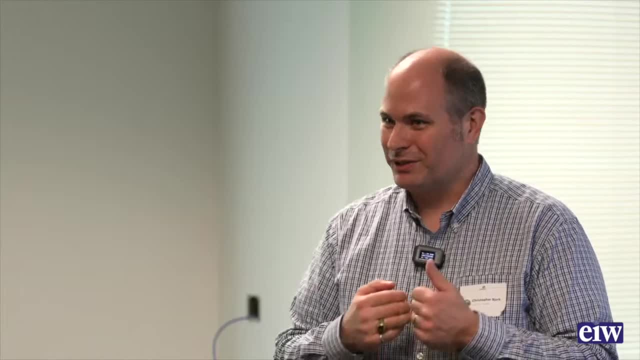 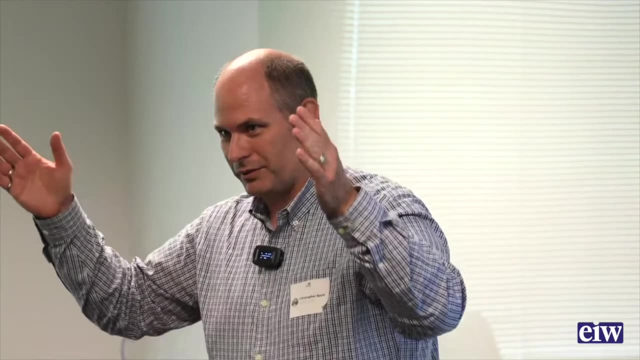 But if you don't have the technology- and back when I started you still sometimes had to do this and we were taught this- the way that you quantify this is you take your grading plan and you actually draw two scale squares on your grading plan. 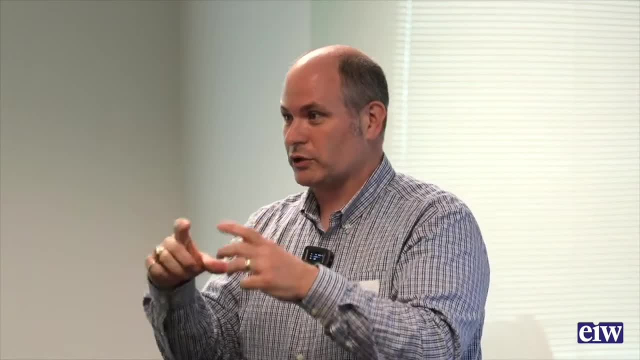 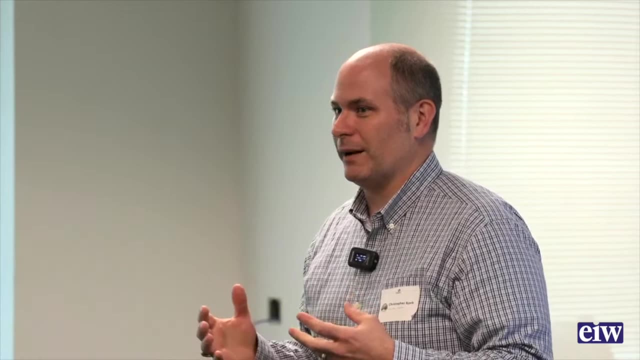 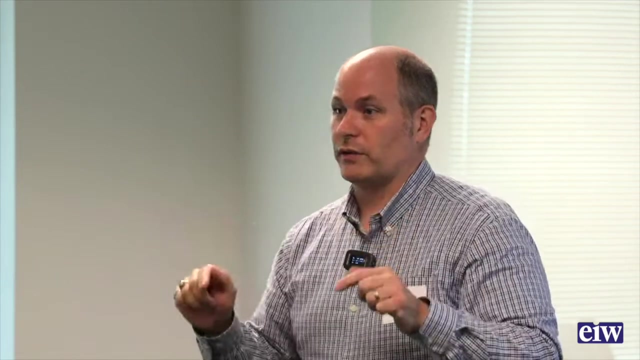 and you pick the four corners of each of those squares, So they may be 10-foot squares, They may be 100-foot squares- It depends a lot about how big your site is- And you figure out what the four corners of the final elevations are. 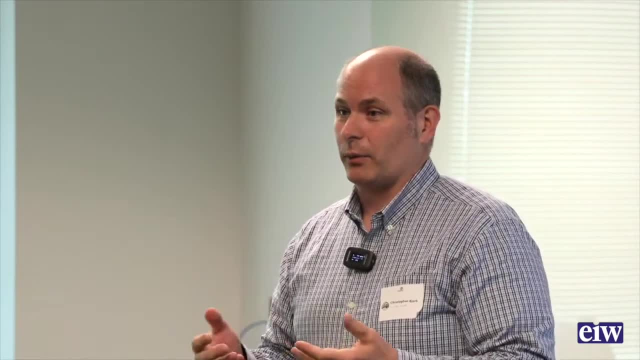 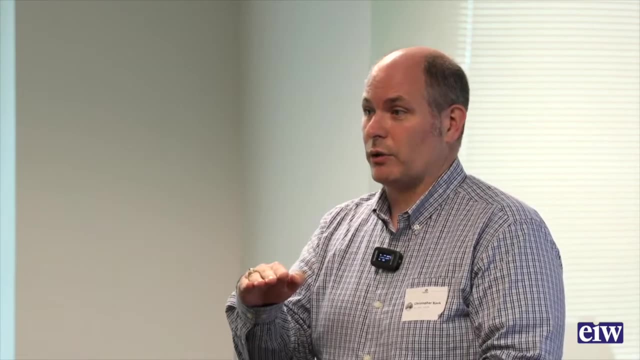 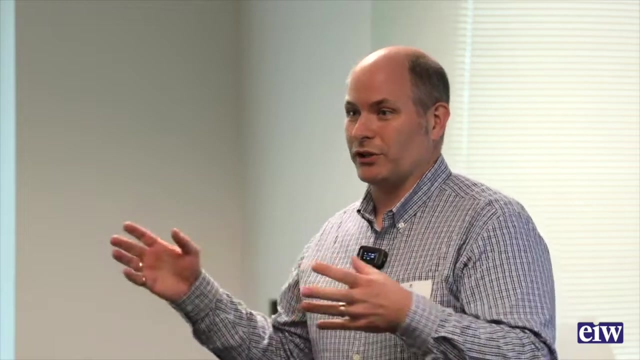 and the four corners of what the existing elevations are And you figure out your average finish grade and your average existing grade And that will tell you whether you have a cut situation where you're taking dirt out, or you have a fill situation. You add up each of those squares and then you have a total of cut and fill. 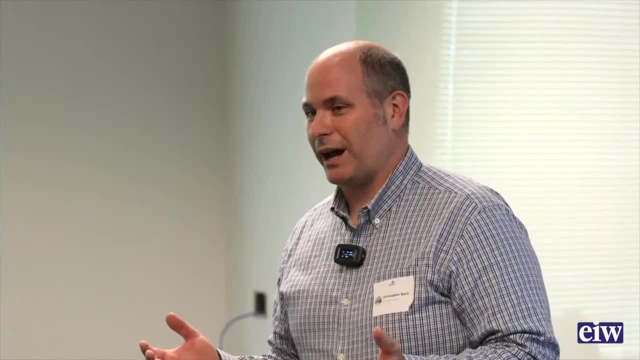 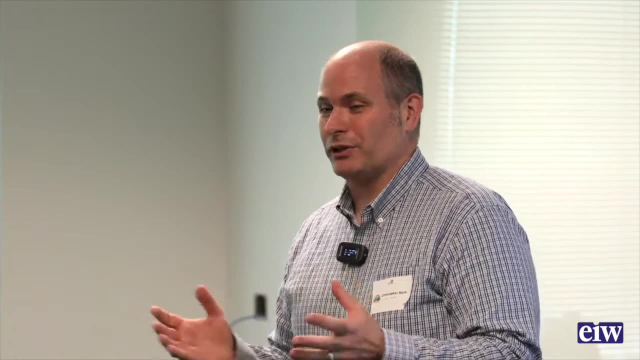 Now, that can be very time consuming, But if you don't have access to a computer, that's the way that you have to do it. And how big do you make those squares? Well, it depends. The smaller you make them, the more accurate you're going to be. 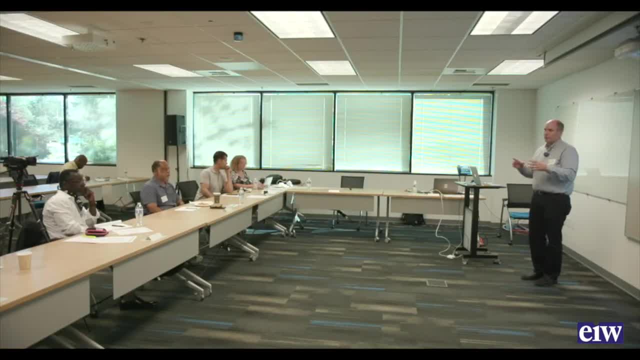 But it's going to take you a lot longer to do it. So you have to really gauge, and that's going to really be dependent on every project. Luckily, there's a lot of great software out there that will compute all this for you. 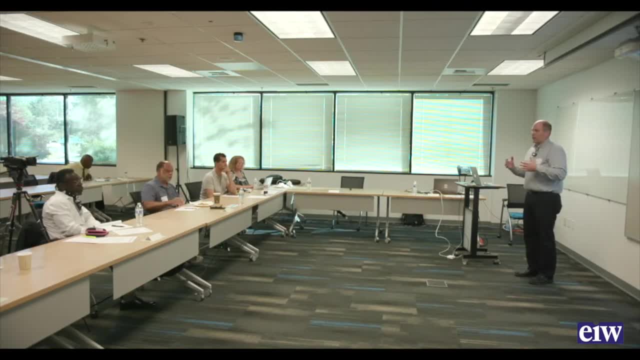 And the software that we use, you can actually import. If you've got the drawings, it will actually bring in a PDF of those drawings And you can trace the existing contours, trace the final contours And then you hit compute and it will actually tell you what the difference is. 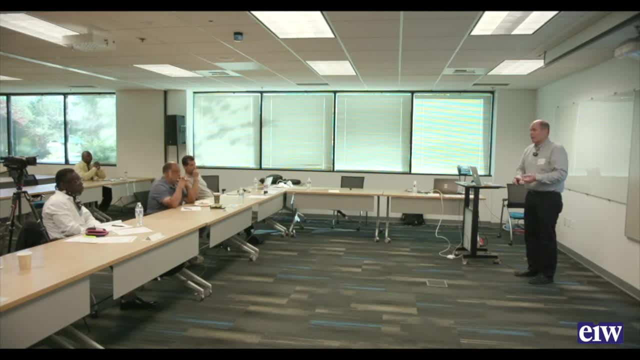 what those volumes are, tell you how much cut, how much fill you have. It will allow you to actually do maps of where your cut and fill are, And some of the great things about these is that they're pretty powerful because you can plug in what your stripping depth is. 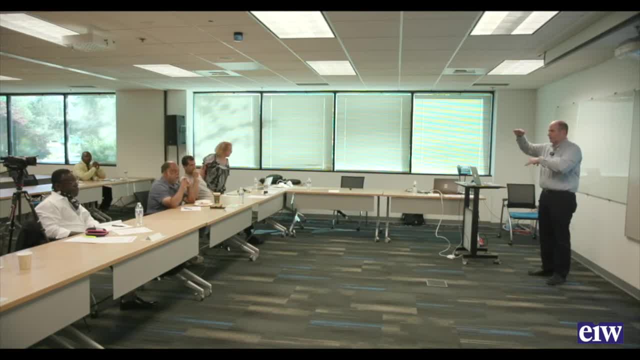 So that tells you that it automatically is going to take if you're starting at elevation 100, but you're stripping a foot off. that means it's going to take a foot off when it starts running its calculations And it's going to tell you how much stripping volume that you have. 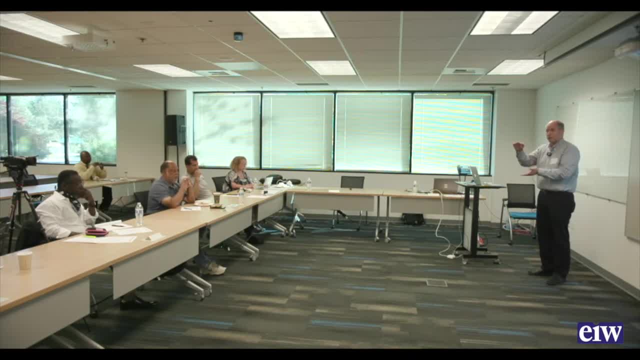 so the cubic yards of stripping volume. But then when it starts computing, when you're cutting fill, it's going to tell you cubic yardages factoring in have already taken off a foot of soil off of this, which means that your quantities are going to be more accurate. They can. also, when you have paving sections, it will. actually you can put in your paving sections and your depth, so your six inches of concrete and maybe six inches of gravel underneath of that. Or if you're in a landscape area, if you've got 18 inches of topsoil you have to put in. 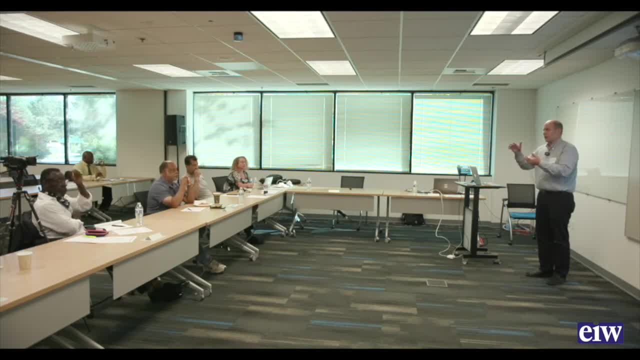 you can put those areas in and put those sections in and it will actually lower your final grades. so to make sure that you have an accurate, a truly accurate look at how many yards of cut and how many yards of fill you have, When we do cut and fill, we use cubic yards. 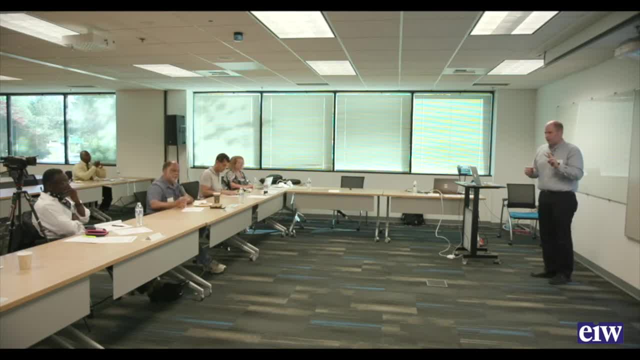 It's volume. But there's two types of cubic yards you're going to use when looking at this. There's bank cubic yards, or neat cubic yards is what they sometimes call it, and that's what the volume is in the ground before you disturb it. 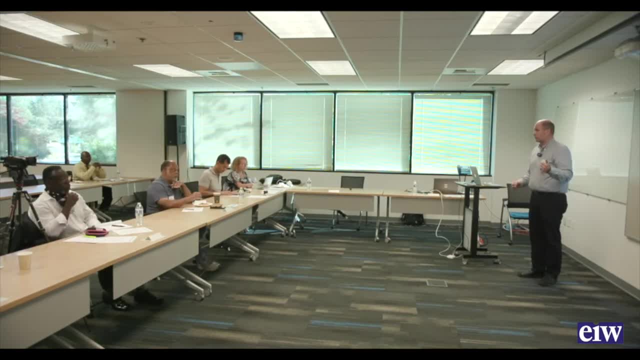 And then there's truck cubic yards, or sometimes it's called loose cubic yards, and that is what that volume is when you disturb it. So when you dig dirt out, it expands, It swells, And if you bring in import gravel in, and then you have to compact it and it's going to shrink. So if you order exactly one cubic yard of gravel and put it into a three foot by three foot by three foot box and compact it in there, you may be as much as only fill it up about two-thirds full. Because once soil is disturbed it's got air voids in it and that makes it expand. So what are those swell and shrinkage factors? Well, the standard rule of thumb that I use is 35% in and out. That's really highly dependent on what type of gravel or soil you have, because it can be as low as 20%. It could be even lower than that if you have really a big rip-rap type rock where you don't have a lot of fine soil in between it, so there's not a lot of compaction, that can actually happen. 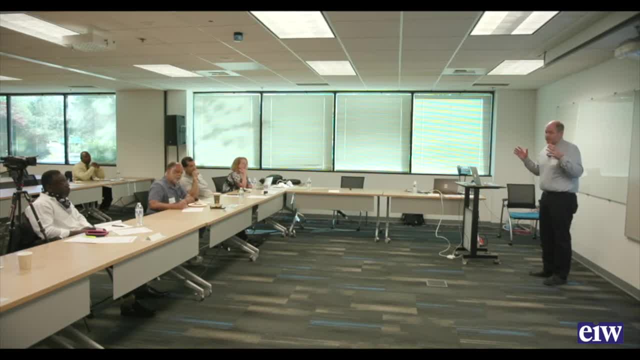 But it may be 35% because it's got a lot of compaction. that can happen. The best way to find out what the exact percentage is is to actually talk with the questioner or the quarry that you're dealing with, because they know their material the best. 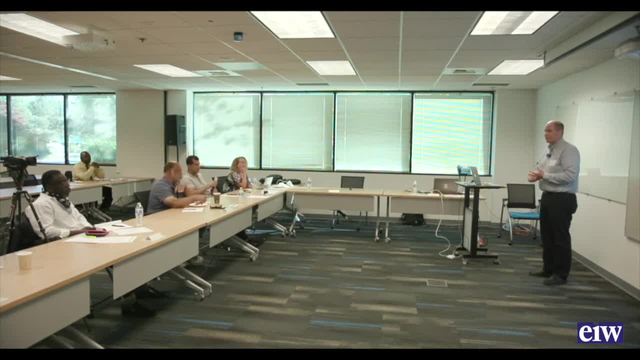 And they'll be able to know: hey, how much do I need to figure if I'm trying to achieve 95% compaction or 90% compaction? You might talk with the geotechnical engineer as well. They may know something about that as well. because they've done studies on that soil as well. But rule of thumb anywhere from 20% to 35% is usually a very good rule of thumb for shrinkage and swell factors. Another thing that you need to know about is looking at the soils report. 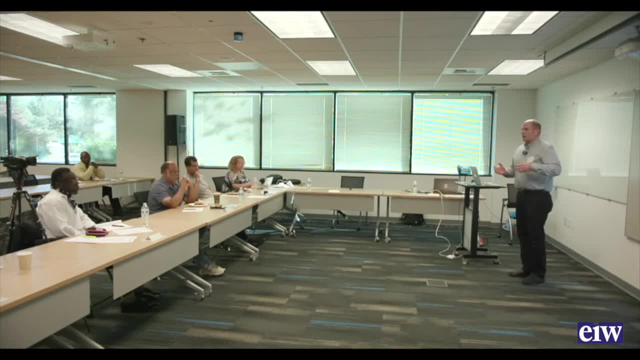 is native fill versus import fill. When you read the soils report, it will let you know whether the existing soils are suitable to be reused as structural fill or what they can be reused, as They may be able to be reused as landscape forms. 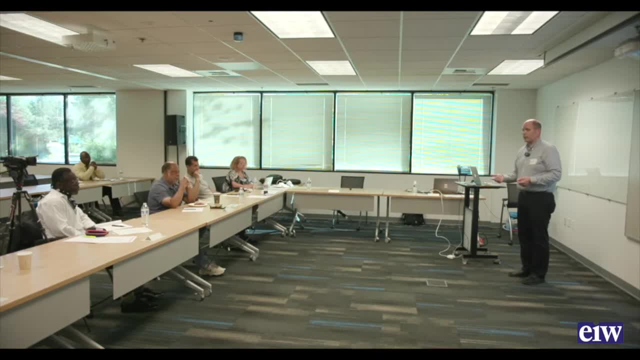 They may be able to be reused as structural backfill. If they can be reused as structural backfill, you can stockpile that on site. You may have to tarp it and condition it and make sure that you take care of it, But that means that you may be able to take that soil. 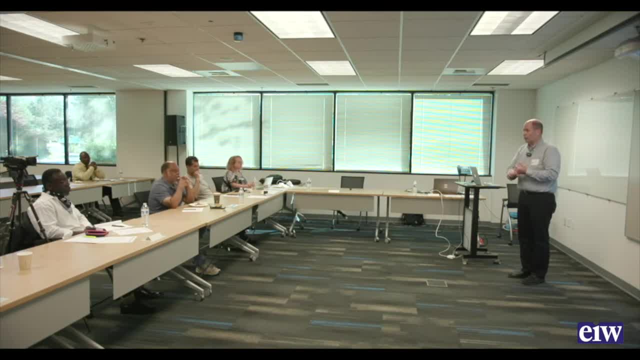 and then use it to backfill footings, backfill walls or put it as fill underneath the building. if your building is under a fill area, If it says you can't use it, then you know you need to haul that. You need to haul most of that off. 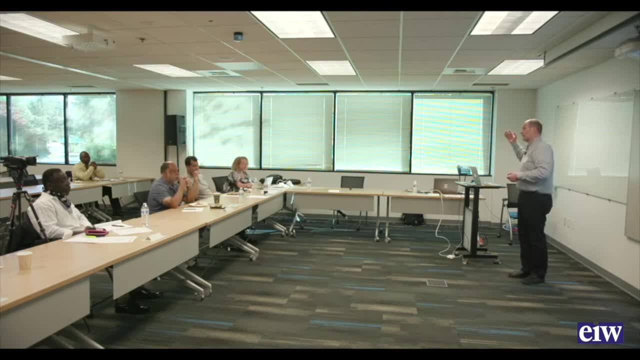 and deposit it somewhere off-site, And then all the fill that you need for the site you'll need to bring in, and bring in as either an engineered structural fill or a gravel. It depends on what the actual conditions are and what the drawings actually call for. 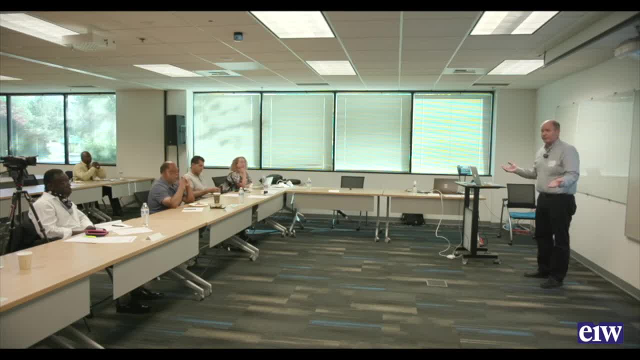 It's an important thing to know, because import costs a lot more than native. If you've got native fill, you're not paying for the actual material itself, You're just paying to handle it. So that's really important to look at your soils report. 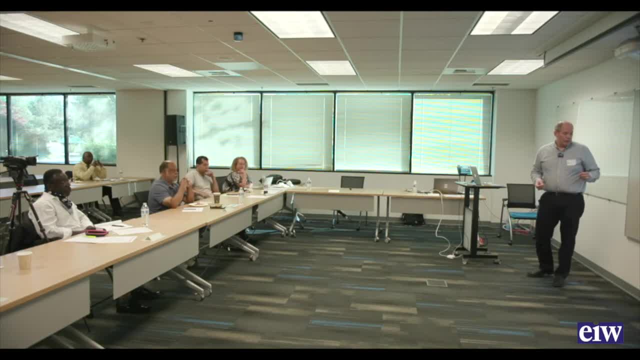 to find out whether you can use that. The other thing is haul off And, just like everything else, you need to know where you're taking the material. Do you have a site that's a half an hour away or do you have a site that's a three-hour round trip? 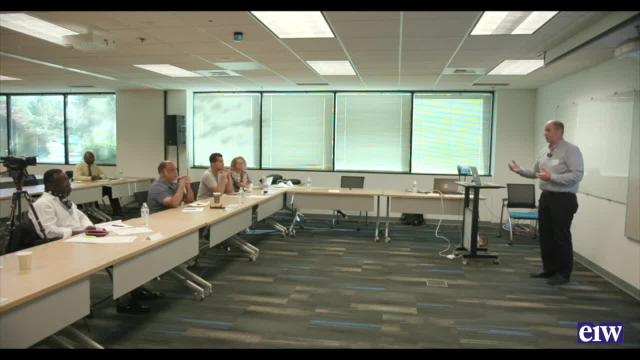 That's important to know because you have to pay for the trip there And if it takes longer it's more money. So you need to understand that. You need to understand, on the import cost, where you're getting the material from so you can understand how much is that going to cost. One thing about buying rock from a quarry: oftentimes they will sell it to you, or quote it to you, in tons, as opposed to cubic yards. Soil can weigh anywhere from 85, 90 pounds per cubic foot up to 120 pounds per cubic foot. 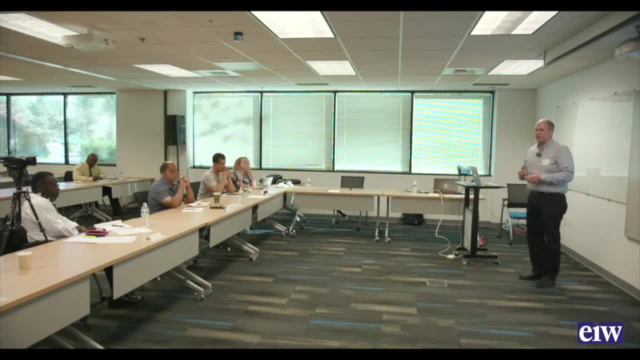 So the best way that you can do that, and you can really figure out what that specific soil is, is to talk to the quarry. They will know what the pounds per cubic foot of that material is. What I usually do, though, is I usually just say: 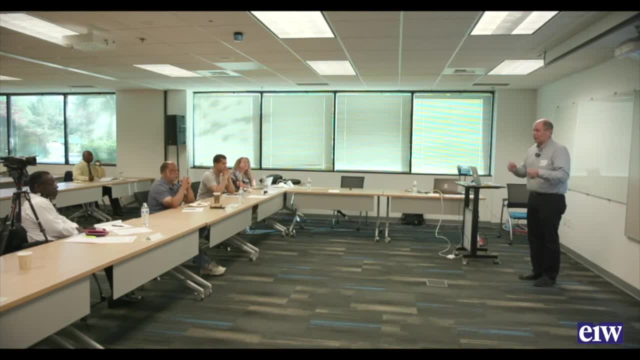 I need X amount of cubic yards, whether I tell them it's either truck yards or bank yards, and I'll let them figure it out, because they know what it is and they're used to people having to companies ordering things by the cubic yards. 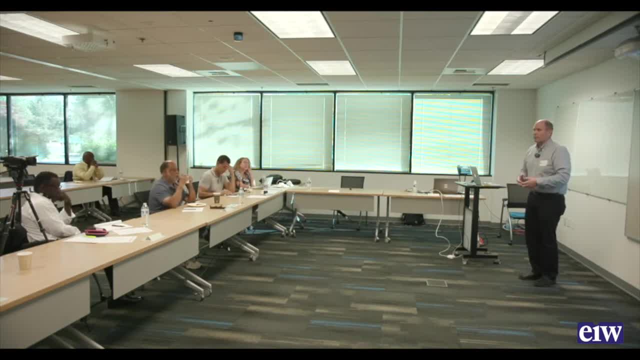 but then figuring out what that tonnage is? because they have to figure out the cubic yards anyway, because the loads of the truck are measured by cubic yards and not by ton. So work with the quarry If you're looking at buying material and that material when you purchase it. 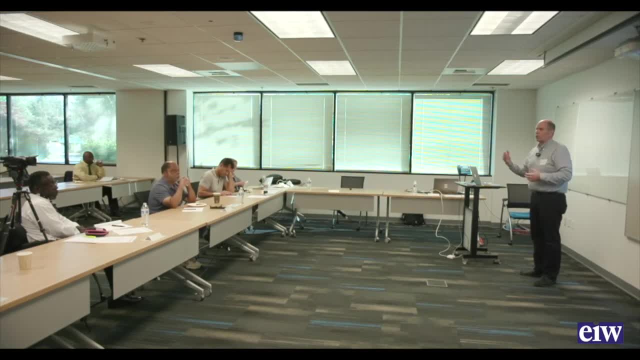 make sure you talk to the quarries to make sure that you get the information. If you're getting a quote from them, make sure that they understand what you're looking for. Are you looking for a quote per cubic yard or do you already know what it's going to weigh per ton? 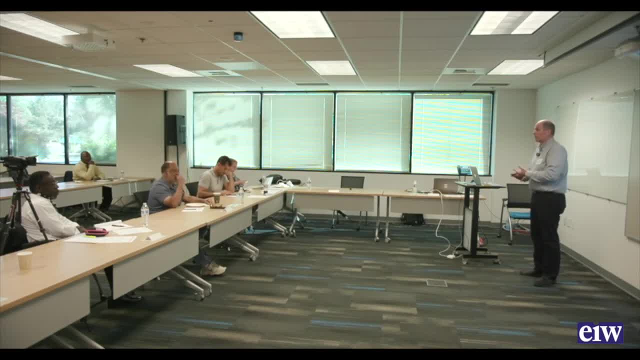 and you want it per ton. Make sure that you talk with them and they understand and communicate what it is that you're expecting and what it is that you expect out of them. The next part of excavation is your structural excavation. That's where we're digging out basements. 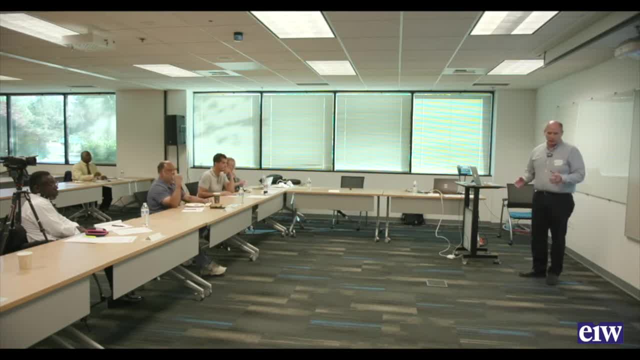 we're digging out footings and that's where we really look at a more itemized, surgical type of excavation, Where we need to think about how we're excavating it. Do we have side slopes which are clearing that out so that the soil doesn't cave in on you? 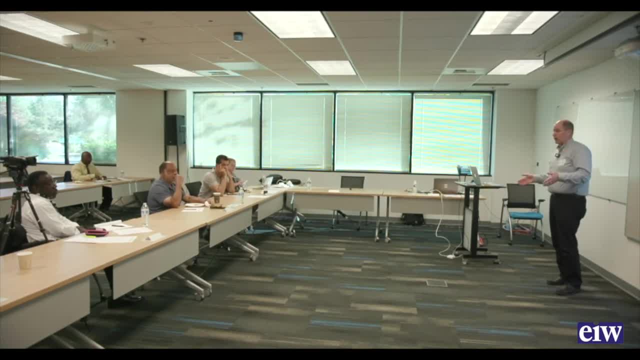 Are you doing a basement excavation and are you shoring That logistics? you need to understand that, because that's a different volume that you're going to be taking out When you look at excavations and whether it's a footing or a basement. 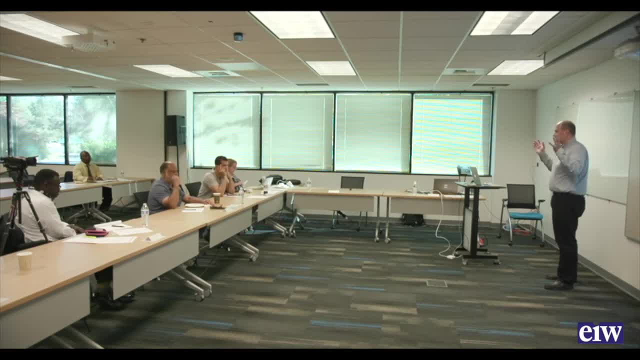 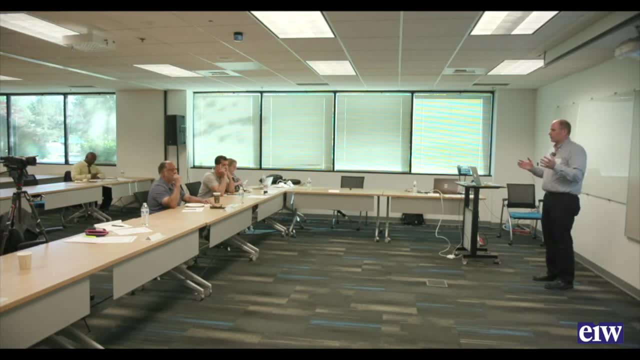 if you're talking about actually side sloping the excavation, then the way that you look at it is: you're dealing with volumes. You need the volume of excavation, you're going to need the volume of backfill that goes back in there and you need to know the volume. 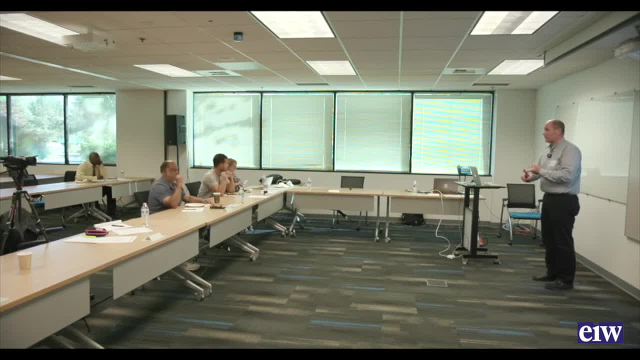 of whatever it is that you're putting in there, whether it's a footing, whether it's a basement. So the way that we figure out the volume of excavation is: we'll take this trapezoid here. Now, if you're looking at a footing, 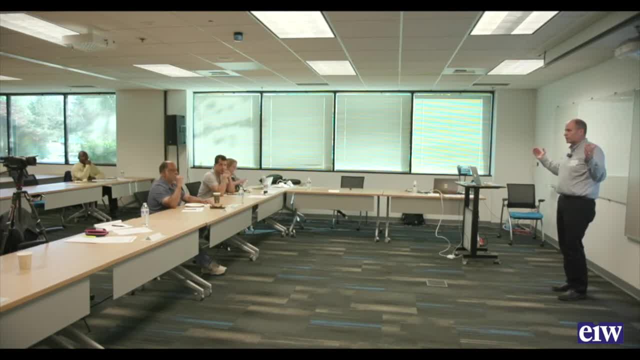 you're going to want to start that trapezoid a couple feet off of the edges of the footing, because whoever's going to come in and build that footing needs some space to put formwork in. They're going to need some space to get a person in there. 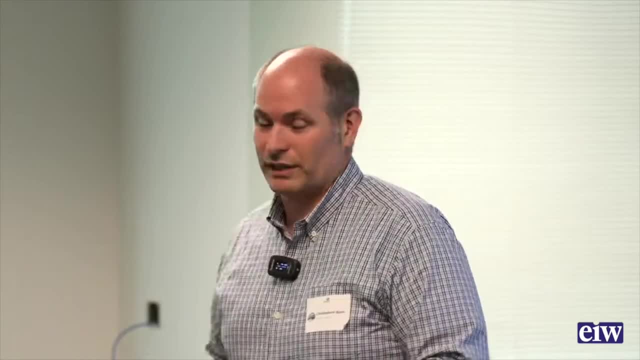 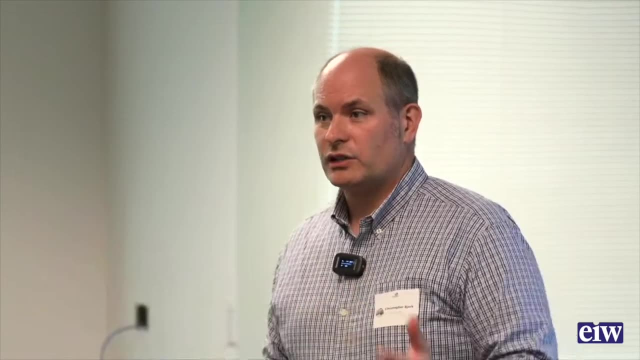 and to put in some kickers to make sure that formwork's braced off. So usually that dimension is about two feet, So you figure two feet around the edge, slope it up at a one-to-one. Now, that's the typical. 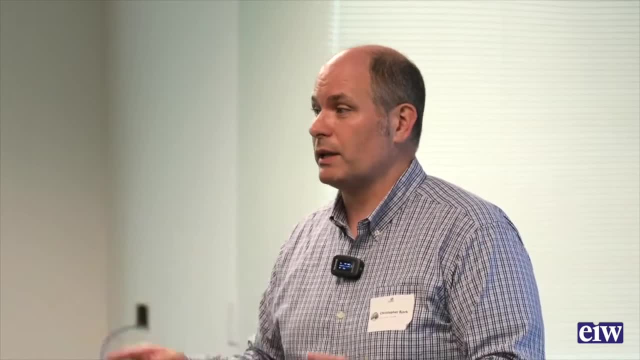 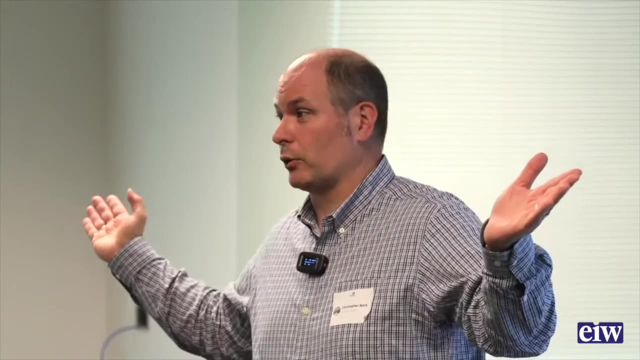 The one-to-one is typical. Always look at your soils report, because certain soils may be able to withstand a three-quarters to one, or they may need to be more at a one-to-three-quarters, where you actually have a shallower slope and they're taking more earth out of it. 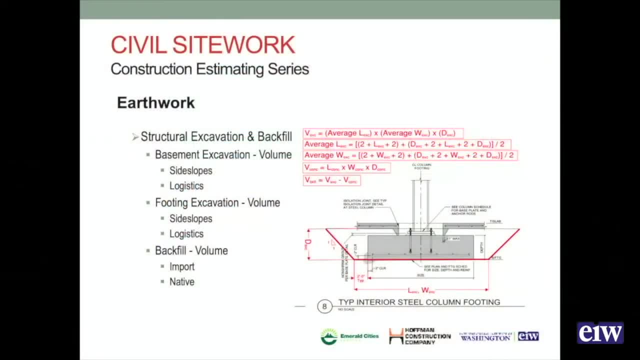 But you take your average length, so average of this length and that length, average width, same dimensions, by your depth of excavation and then divide by 27.. I don't have that up there, but always remember to divide by 27. 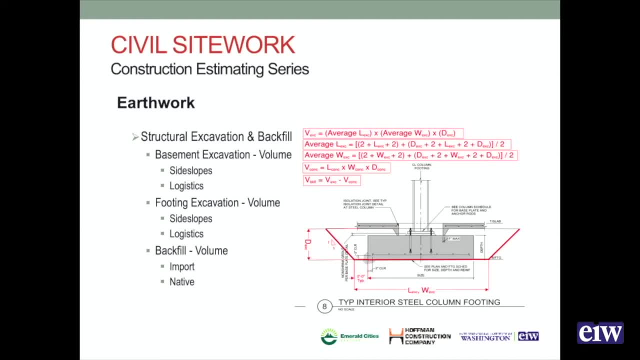 because that converts you from cubic feet to cubic yards, And that's a real important conversion factor when you're dealing with feet, because all your dimensions are going to be feet, and when you need to get it into cubic yards As far as the volume of concrete. 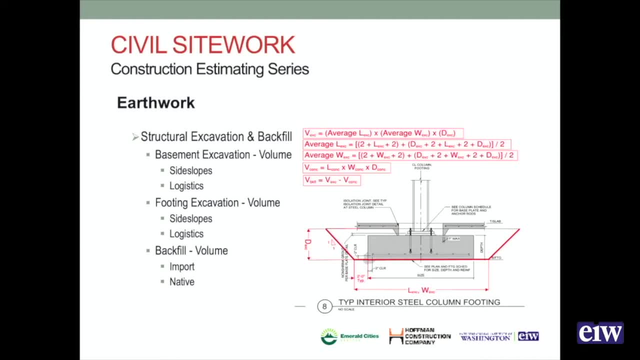 you'll know what the footing size is. That'll be shown on a structural drawing that it's going to be a 10 by 10 by 2 feet footing. You can compute that volume: The difference between the volume of excavation less the volume of the footing. 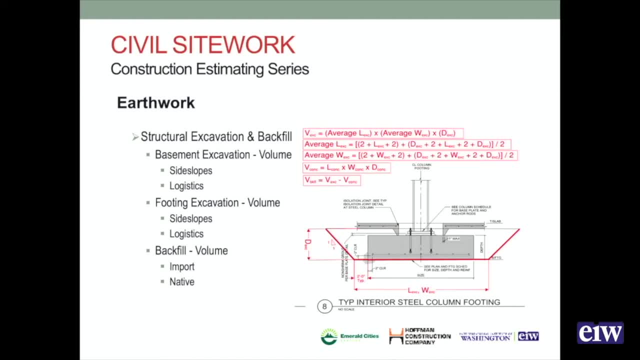 is how much backfill you need, And then so, like mass excavation, with backfill you need to know whether it's you can use the native or whether you need to bring in import- One thing that oftentimes you will see too on projects: 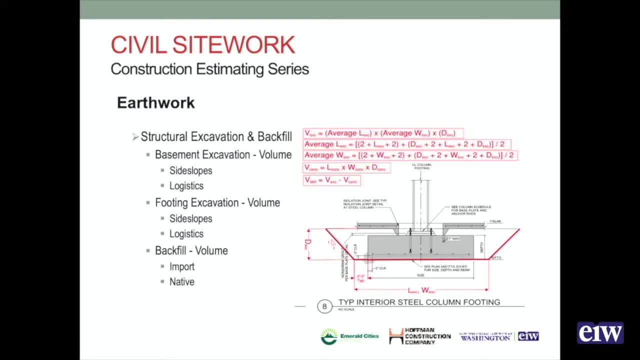 is what they call neat cut excavations, And this is particular to foot footing. So this is kind of the what I need: to coordinate with a concrete subcontractor and the general contractor to see if this is a possibility. So neat cutting a footing means that you dig the whole. 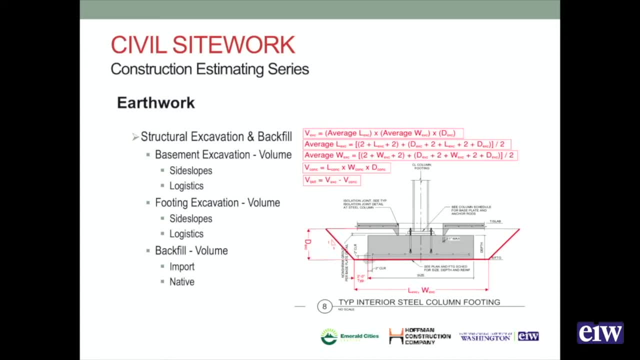 the excavation for the footing- not exactly where the dimensions of the footing, but maybe a couple inches outside that footing- and you dig it. and you're able to dig it vertical because it's shallow enough where the soil can support the cut. And then the concrete subcontractor. 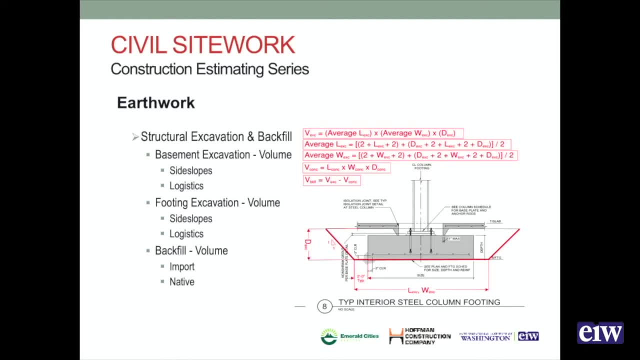 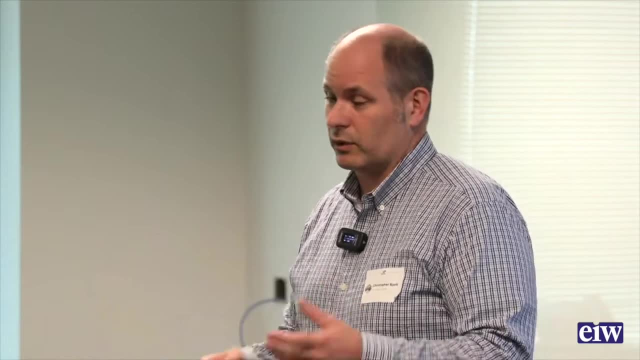 will come in and pour the footing. They won't use any formwork, They'll pour it right up against the earth And that can save a lot of money. A couple of cautions with that is first you need to know you can't necessarily assume that. 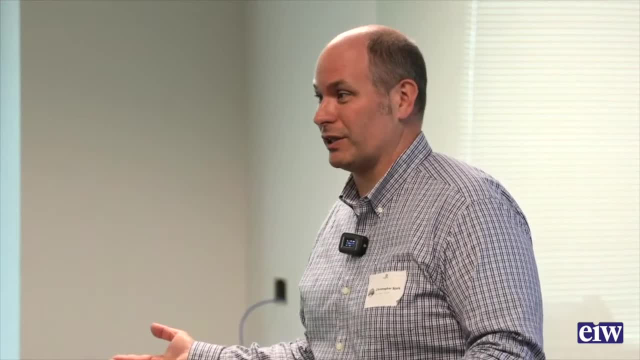 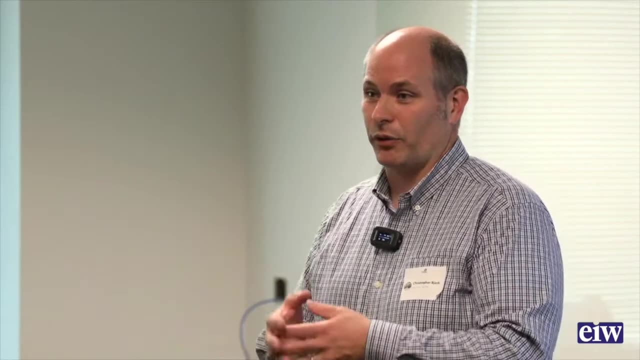 you need to make sure that that's what the concrete subcontractor is doing, because if you're the excavator, you don't necessarily have control over the concrete subcontractor, So you need to make sure that you're both on the same page. The other thing you need to know is: will the structural engineer allow that? Because sometimes the soil conditions are such where the structural engineer says, no, I don't want knee cutting of a footing. Also, is your client going to allow it? Because certain types of projects the client is going to want to rely? 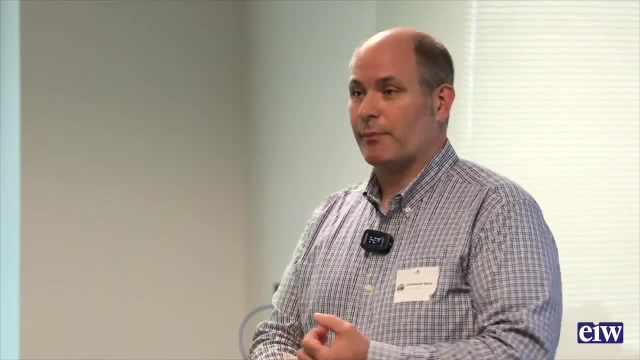 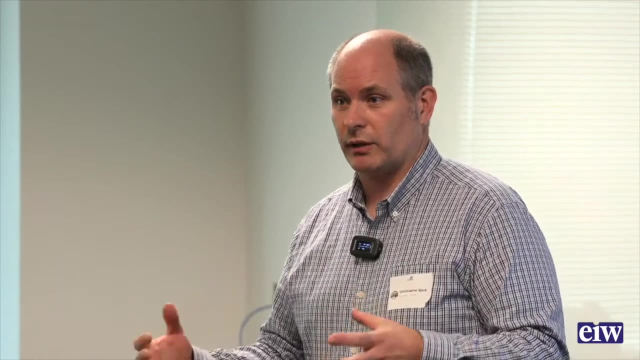 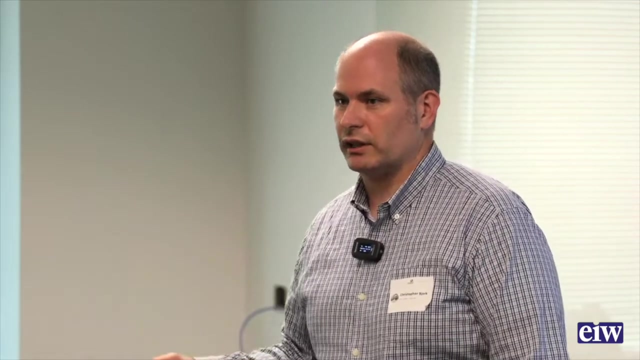 on exactly where those footing lines are. If you are a lab building, building a lab building and this is the ground floor and you have labs on that floor, that first person researcher that comes in may want everything a certain way. the next researcher that comes in, they may have to run new mechanical lines. 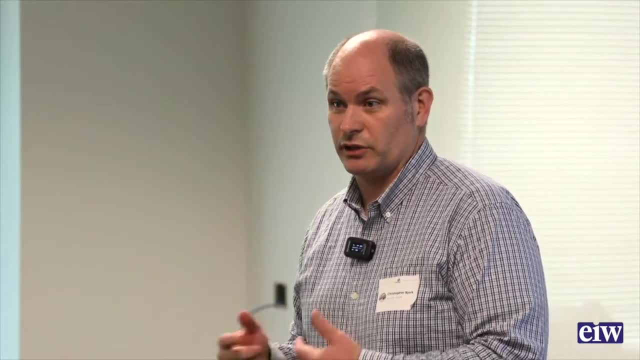 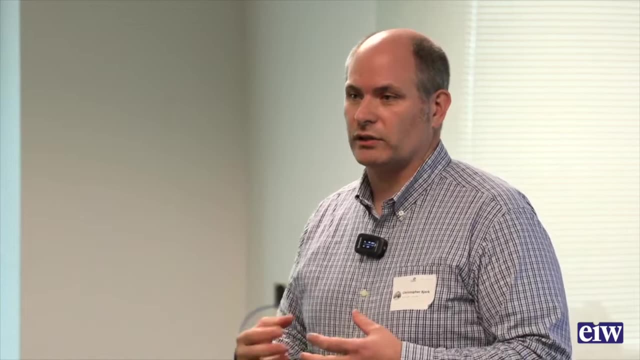 underneath the slab. because of the type of research that researcher is doing, That means they may need to saw, cut the slab and run those lines, and the clients don't want to suddenly open up a slab and find that suddenly now they have to do some demolition work. 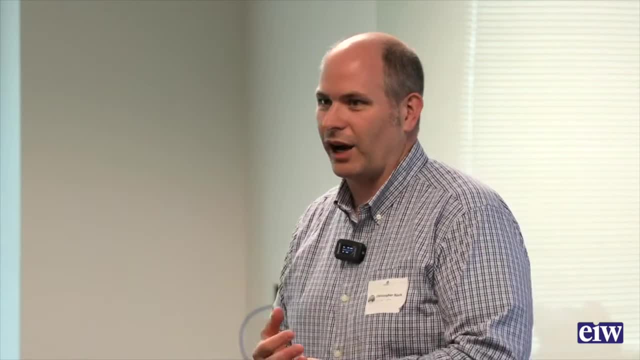 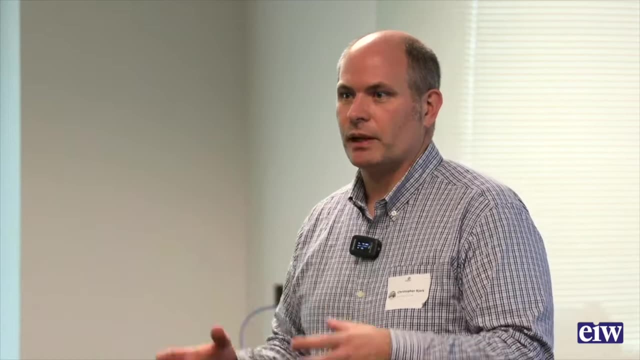 of a footing just to get a line in. It's an unexpected cost that they don't necessarily incur. so they want to make sure that I'm not even going to run the risk you're going to form these up and make sure that they're all exactly how they need to be. 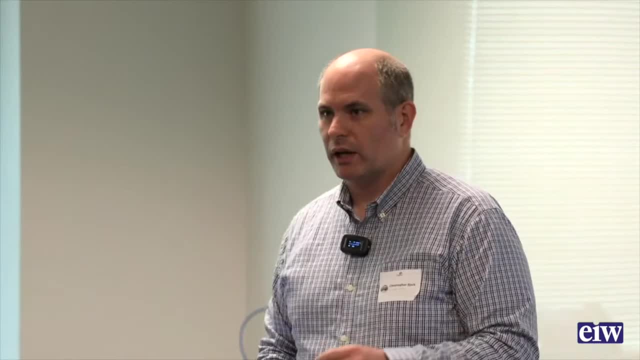 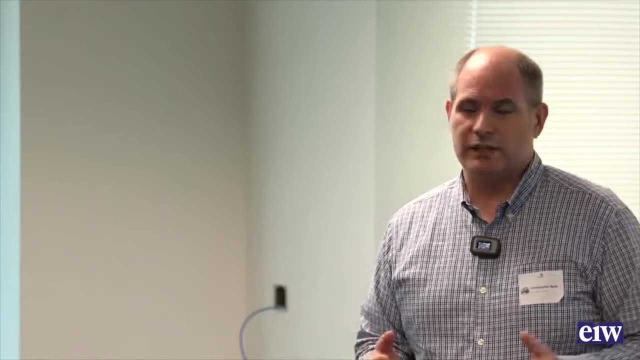 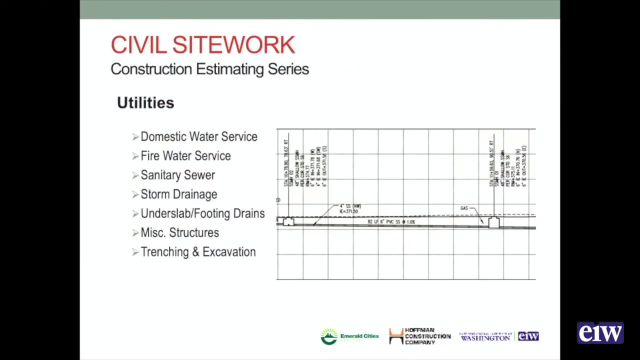 So that's just one thing to make sure that you are aware of if you go into a knee, cut footing situation. Next, key piece of site work and civil site work are utilities. What types of utilities? Domestic water, fire water could be sanitary sewer, storm sewer. 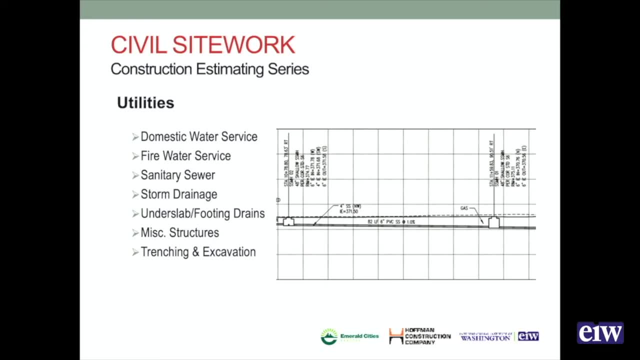 gas also. this falls into under slab footings and under slab drains. Often times if you're in a wet soil condition, you might have an under slab drain to take ground water from underneath the slab. Most all projects have a perimeter footing drain as well. all covers in here. 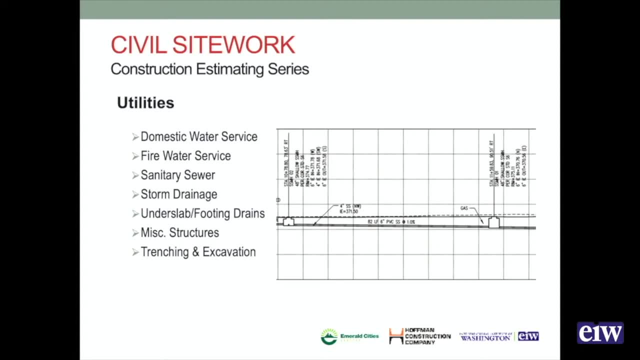 What you need to know here is: you take that off by lineal footage. by material type. so is it PVC pipe? is it perforated PVC type? is it ductile iron? is it steel? and by size, is it 8 inch pipe? is it 6 inch pipe? is it? 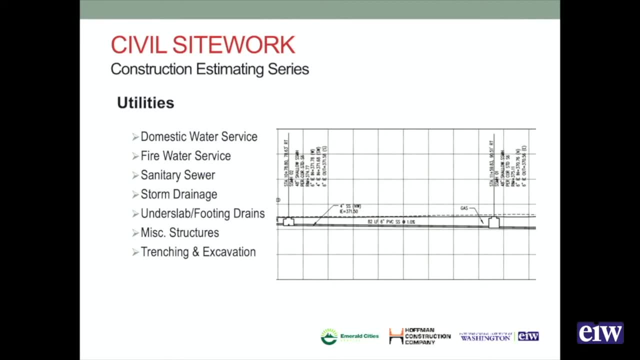 24 inch pipe. If you're looking at a treatment plant, you may see a 108 inch pipe or even larger pipes than that. It's a big cost difference between a 108 inch pipe and an 8 inch pipe. So then you have the pipes. 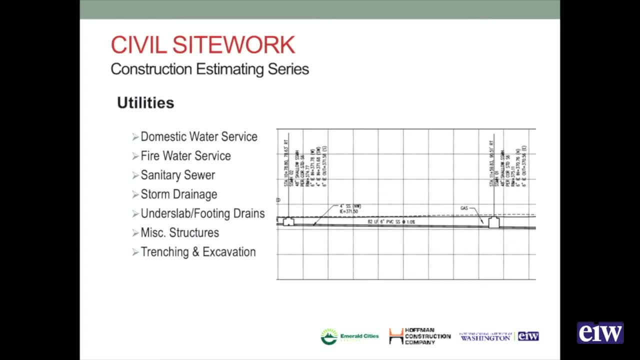 those are going to have fittings, because pipe only comes in certain lengths, so you're going to need to make sure that you understand how those fittings work. You may have Y's where the pipe splits or two pipes come together. you will have 45 degrees in elbows that you 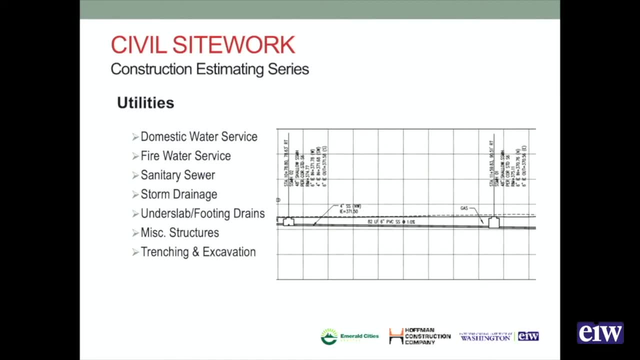 need to take into account for your quantities, then you'll also need to know the miscellaneous structures. So miscellaneous structures, that's manholes, it's cleanouts, it's vaults, it's back check assemblies, valves, meters, and with meters, are you providing it and are you? 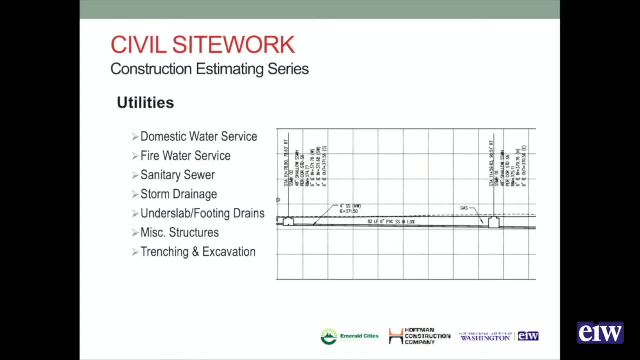 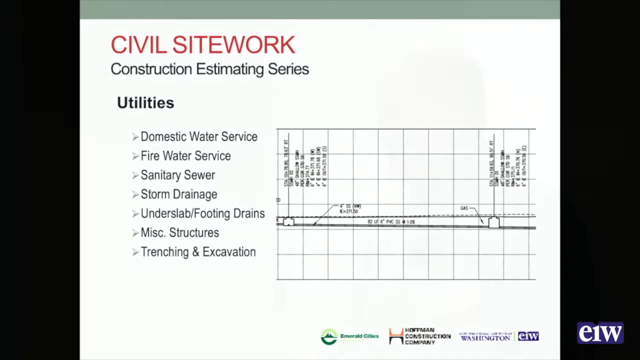 paying for it or is the utility paying for it? Sometimes the utility will pay for it and bill the client direct. You need to know that information because it affects what your estimate will be. And then there's the trenching and excavation that goes with all this. And that is, you take a section and are you going to shore it. How deep is the excavation? That can be anywhere from 2 feet deep. Water lines in general are very shallow. Sanitary sewer and storm sewer lines can be very deep. I've 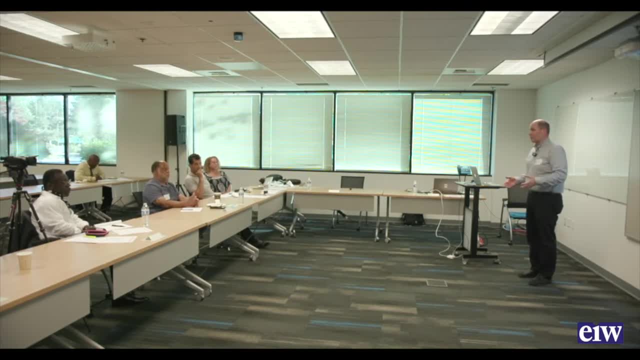 seen even on small projects, where they get to be 20-30 feet deep. So if that's a 30 foot deep excavation, you need to know how you're going to shore that, Because that's a dangerous situation if it's not shored, and it's a lot of money. 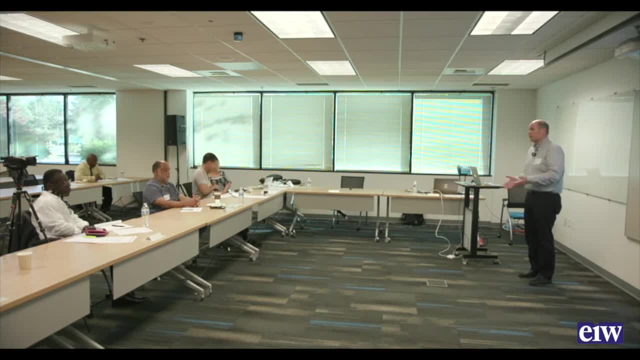 to you may not even be able to physically have the room to side slope and cut the back and lay it back. We're going to do a sample storm drain takeoff so you can get a really good depth about how you look at that later on in this. 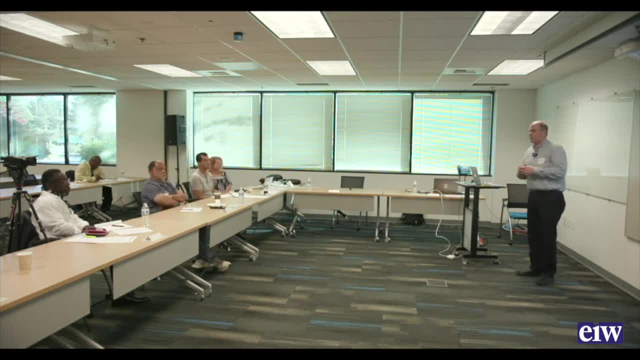 Paving and base courses. So paving, you're looking at asphalt. Flexible paving is asphalt, permeable asphalt: We look at that on an area basis by the thickness, Similar to- I will say similar to gravel Asphalt companies. if you're buying asphalt they'll 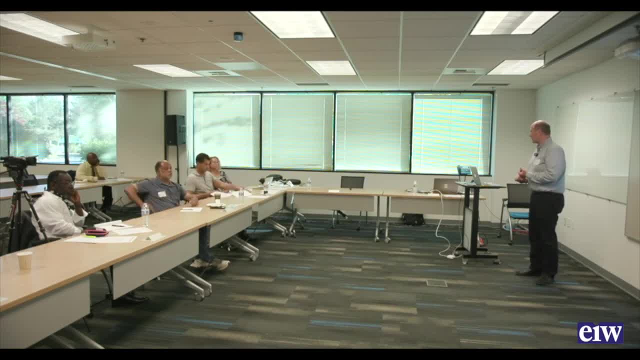 want to sell it to you by the ton, But they will be able to tell you what the area, how much it weighs per ton. So you can either get that quantity or, if you're hiring, you're not doing the asphalt work yourself, you're hiring somebody to. 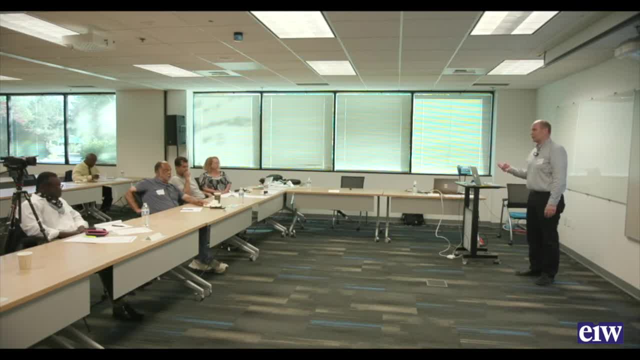 do the asphalt. If you tell an asphalt company, I've got two inch, I've got 40,000 square feet of two inch hot mix, standard hot mix asphalt, they'll be able to tell you: okay, figure X, dollars per square foot. 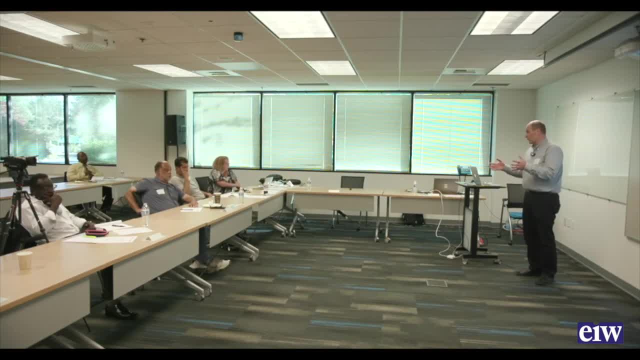 And they may quote you just as a unit cost, like that, because they may not have the plans available to them. They may quote you as a lump sum, because they do have the plans available to them. They may want to just quote you as a unit price, just. 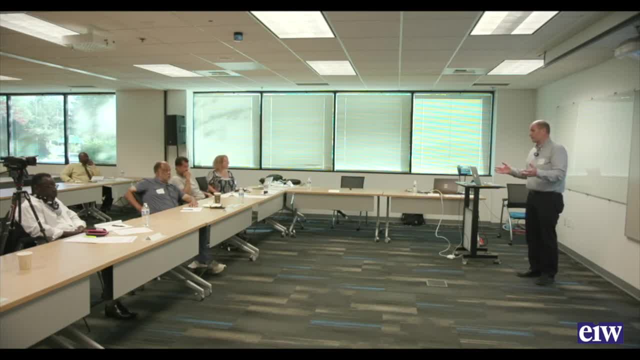 because they may be unsure of what's the actual end result is going to be and they want to work on a more of a unit cost basis as opposed to a lump sum basis. Yes, There's no cleaner way to use a material, because asphalt is basically a petroleum product. 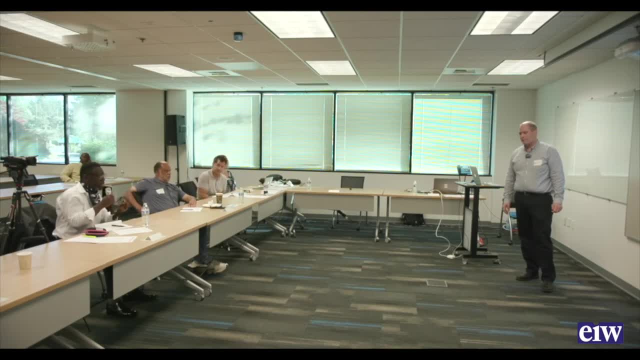 and you have to put it on hot and greasy and it's doing its thing, and it's raining. We're in a rainy state, And so we're always setting up either caps on sewer lines or some sort of erosion control. What do we do for this material? 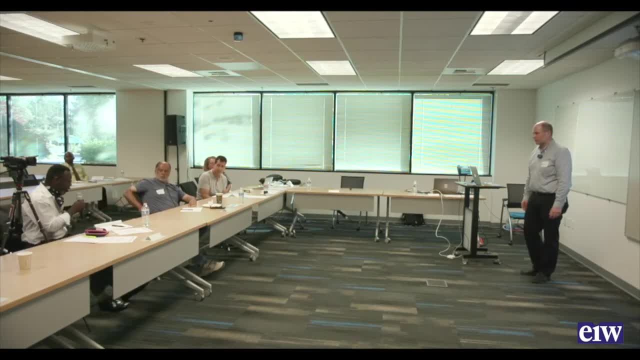 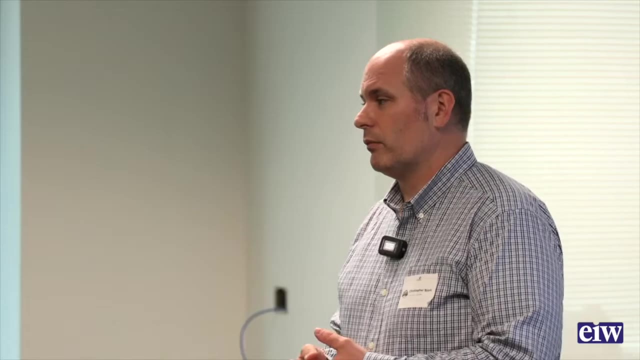 because we're always saying we want it green. Are we concerned? Well, there's a couple different things. To start with, asphalt is not the only paving solution. It's used frequently because it's an inexpensive paving solution. It costs a lot less than concrete. 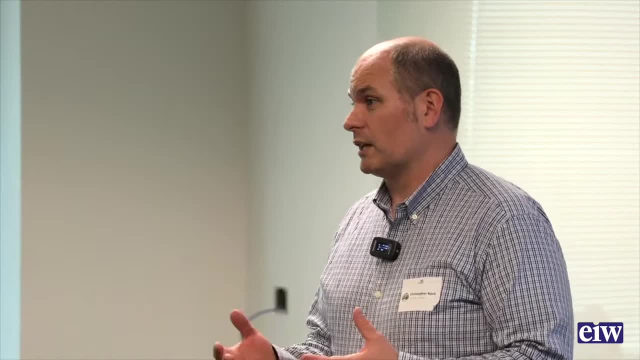 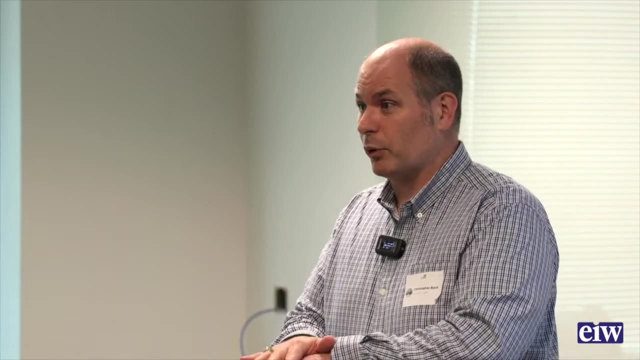 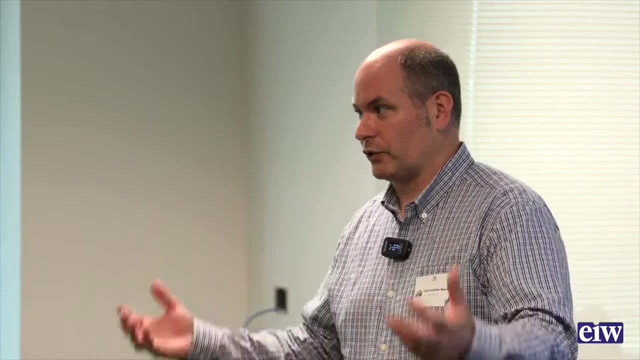 but in order to mitigate some of the problems with asphalt- aside from the petroleum issue is that it's a hard surface, It's an impervious surface, So you have to provide catch basins and you have to provide storm drain and infrastructure for that, And now you have runoff. and extra runoff. instead of infiltrating the soil like it would be in nature, It is now running into a sewer, and now you've got that cost and that environmental impact. They do have a permeable asphalt, though, where you can put that down. It costs more than regular asphalt. 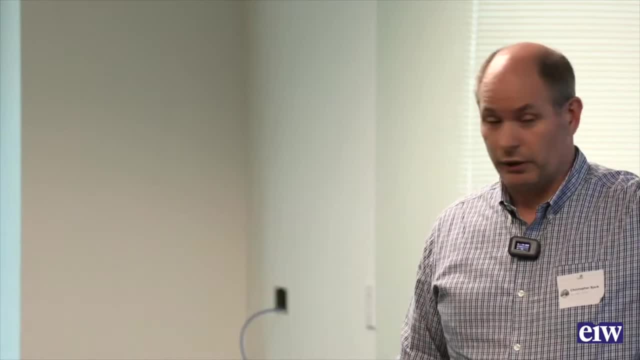 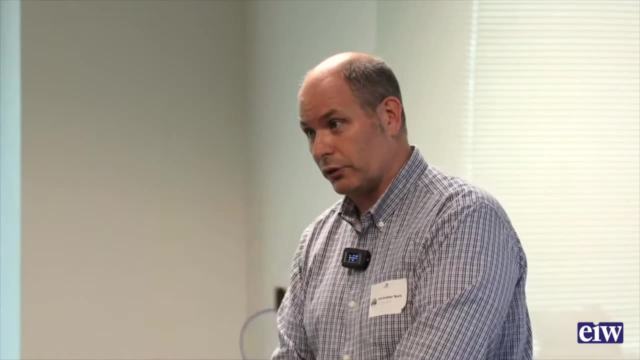 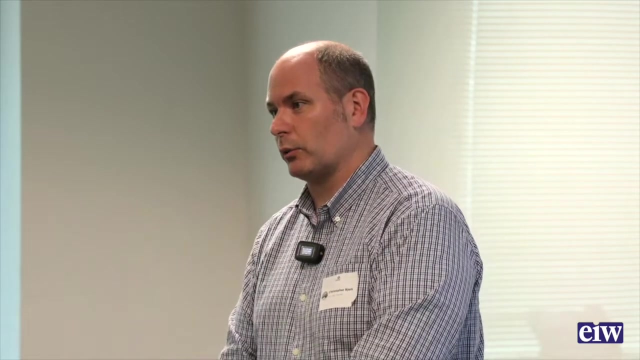 So it's something that you would need to know as far as materials and types of asphalt paving that you're working with, But it allows the water to actually infiltrate through that, so it's actually a lesser environmental impact because the water is now going back into the ground where 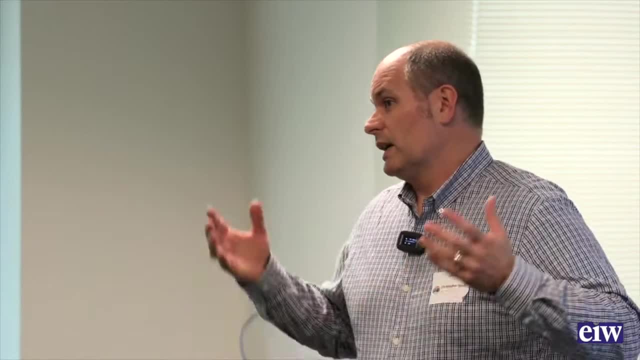 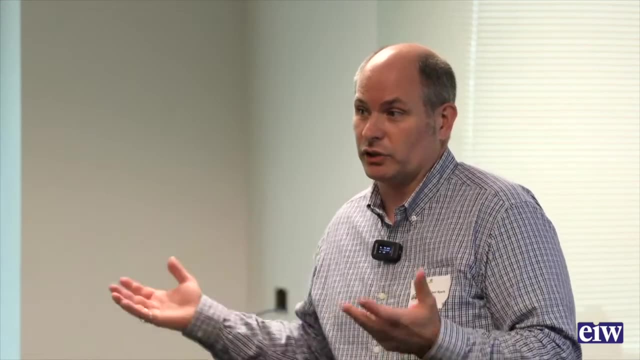 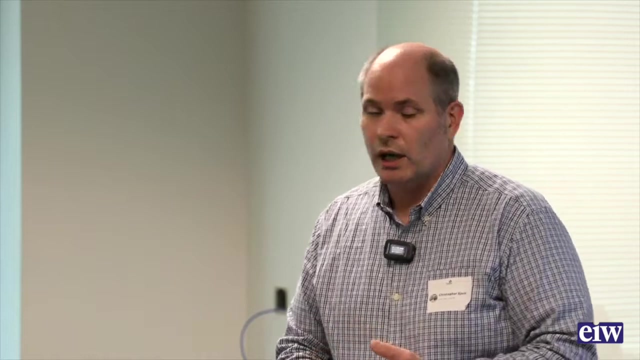 it wants to be. It just costs more. but outside of switching materials, then that's the best solution. as far as switching materials to, whether it's a concrete material or a permeable concrete material, They have a permeable concrete material as well. There's also other. 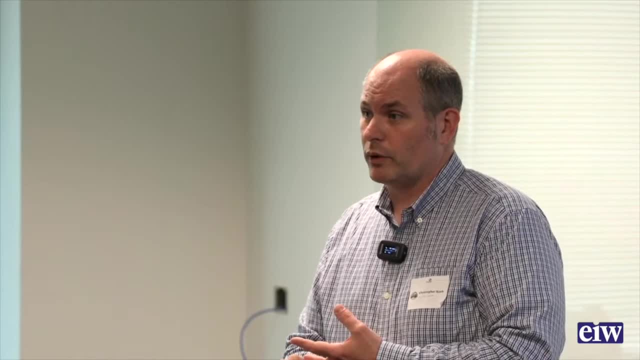 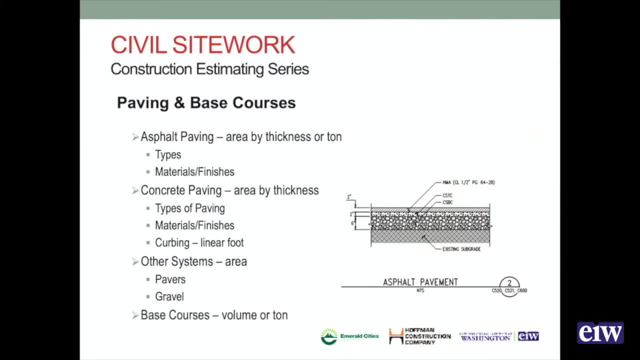 systems like a paver, systems that can allow water to get through as well, that have some lesser impacts. No matter what you put down for paving, there's going to be some kind of environmental impact, because concrete takes natural materials to make, There's an environmental impact for concrete. 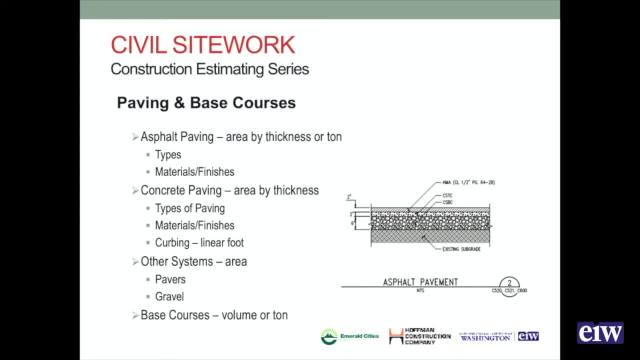 There's an environmental impact for brick pavers or stone pavers, But it depends on what your offsets are, because there's costs associated with all of them as well. There are projects that do have permeable asphalt on them. There are projects that have permeable. 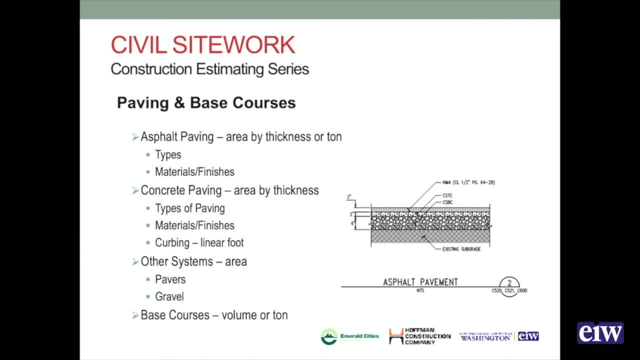 concrete on them. There are concrete paving projects. There are paver projects Sometimes, often times- and this kind of gets into this- other paver systems. There's Grasscrete, which is a paver system that often times they use in a landscape area. So it's a series of 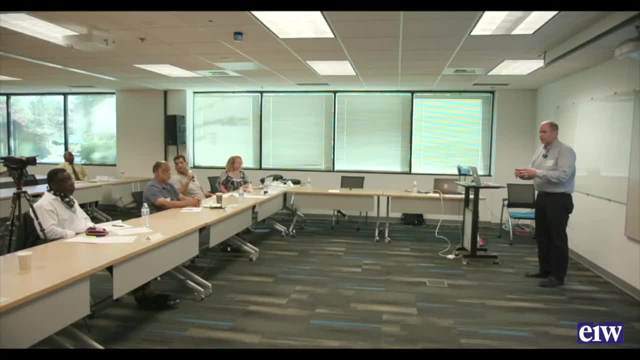 hollow, like precast pavers that you put in that allow you fill with topsoil and it allows grass to grow through them. So you still have a landscape area but it allows for, like a fire truck to drive on it, So often times for a fire lane to. 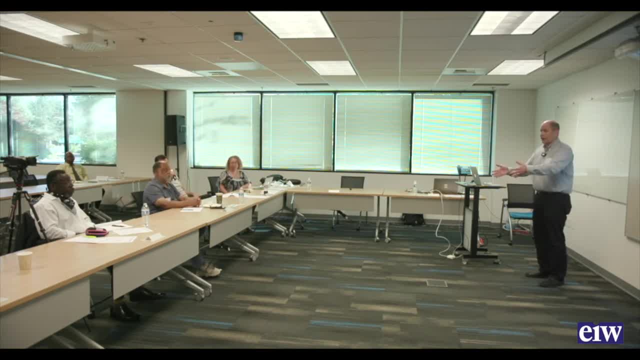 for access to a building in a landscape grass area. they'll put in a Grasscrete area so that they can still have the pristiness of soil and landscaping there without having to make the hard without and have that but still have that hard surface. Yeah, Tim. 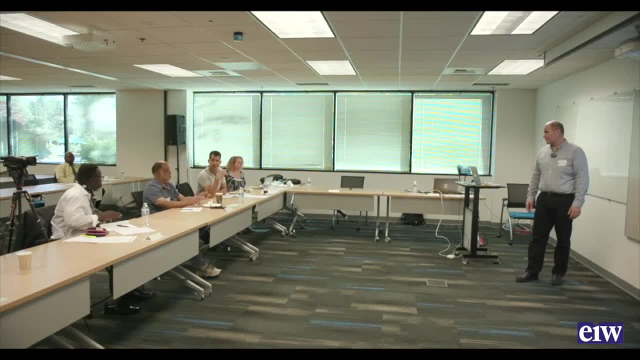 a lot of times you'll find, especially in Washington state, the evergreen construction standards really apply in the housing side, especially multi-family, and so you'll see a lot of pervious solutions within their site plans. The most often place where I see pervious concrete or pervious asphalt is 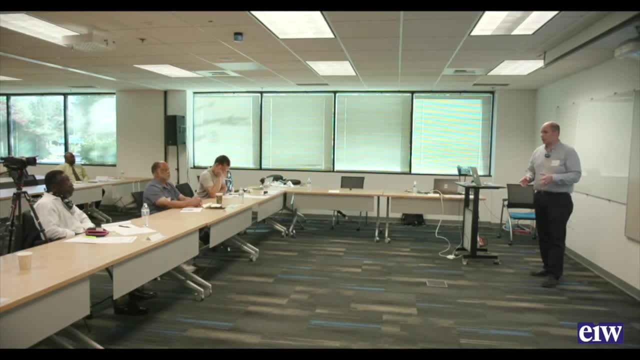 in sidewalks and actual walk surfaces as opposed to parking lots and drive surfaces, because the, if it's not maintained properly, it can. it will not wear as well as standard asphalt or standard concrete and it's going. if you're driving vehicles over it, it will get more wear and tear. 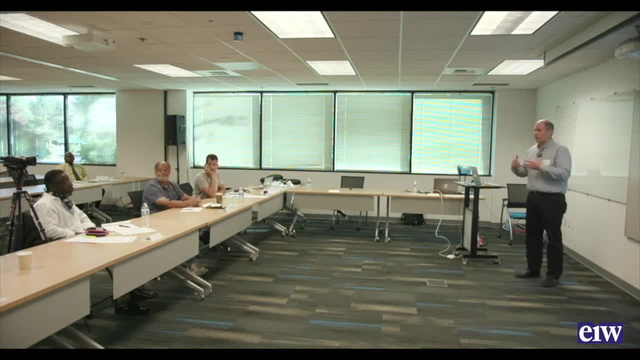 than on it, and plus you can get dirt and debris and stuff into some of those voids that allow the surface, the water, to get through the surface. but concrete paving is the same thing, is area by thickness, but you need to know what kind of finishes you have on it. so 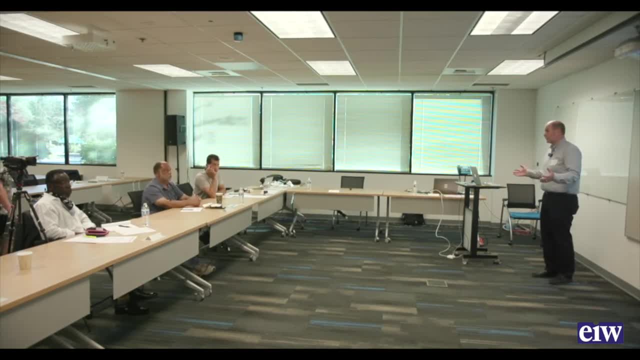 do you have a standard sidewalk finish? Is it a vehicular paving that maybe has more of a raked finish? Is it a plaza where you've got a decorative stamped or saw cut finish? Those are all factors that are going to cost more or less money. 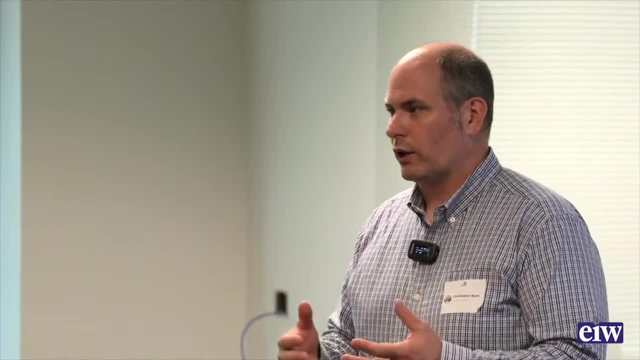 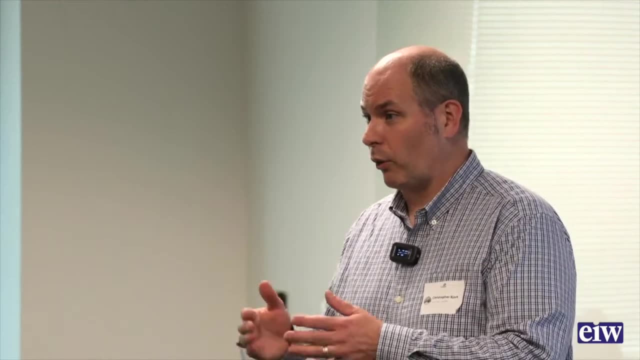 so you need to factor that into what work you're being done. Expansion joints: you need to know where your expansion joints are and where you're going to break up the pores of the concrete, so that you know how much labor you need to put into it. but concrete paving. I'll price out cost per square foot, depending on what that thickness is, and curbing the curbs are going to be priced per lineal foot. but you need to know what kind of curb is it. is it a standard curb? is it a flush curb, where the top of the curb 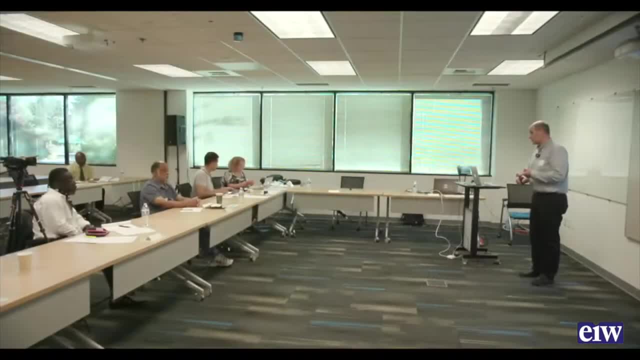 is at the same height as the paving or is it a curb and gutter system? because curb and gutter is going to cost a lot more than just a standard curb and even VSCLV details will have that curb and gutter actually as a often times as a two pour. 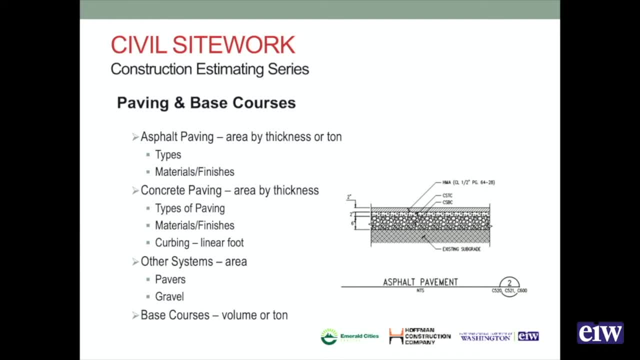 activity. so you pour the base gutter and then you come back and pour the top of the curb too. so you need to understand what those details are, that it will affect your pricing. and then those other systems that we talked about are brick pavers, concrete pavers. 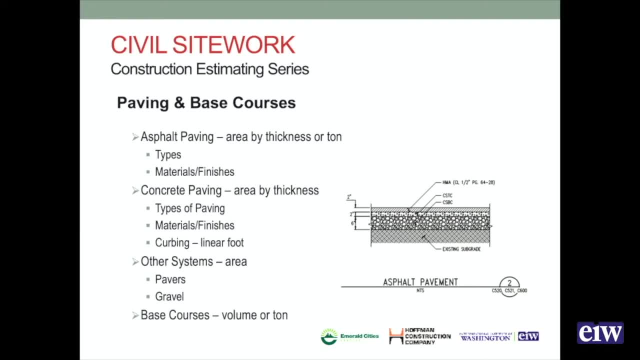 stone pavers with pavering systems. you need to know what the details are, because they can be sand set, they can be mortar set and that depends on: are the joints? are you filling them with sand or are you filling them with mortar? what's the base course? 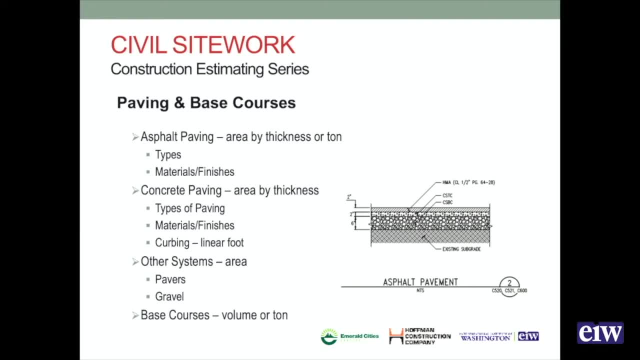 are you setting on a sand leveling course? are you actually pouring a slab underneath it? because if they're on a vehicular setting, you may actually need to pour a structural slab underneath that those pavers, in order to have the right area and the right depth to support. 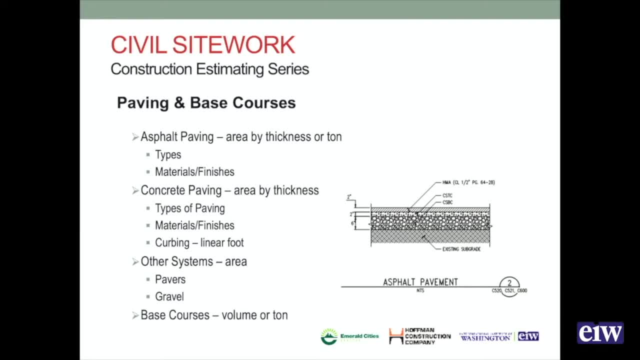 the vehicular loads and then base courses you need to know are: what's the thickness and what are you putting in there? now this example here is a section of asphalt paving and it actually has here a two inch top course, which is usually about an inch and a half minus. 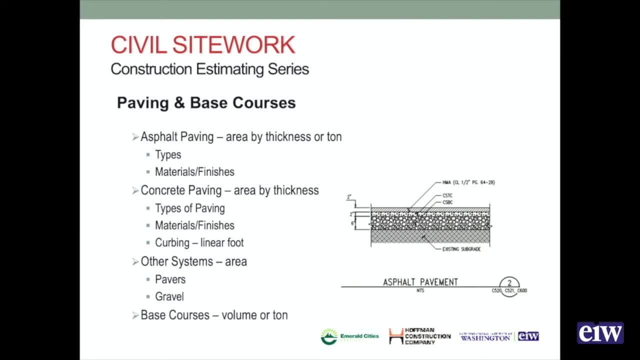 gravel. I mean not an inch and a half, but a half inch minus gravel and then a six inch base course on it, and that's usually a three quarter inch minus gravel. so two different types of gravel, that's two different activities. you also need- you've got an existing subgrade. 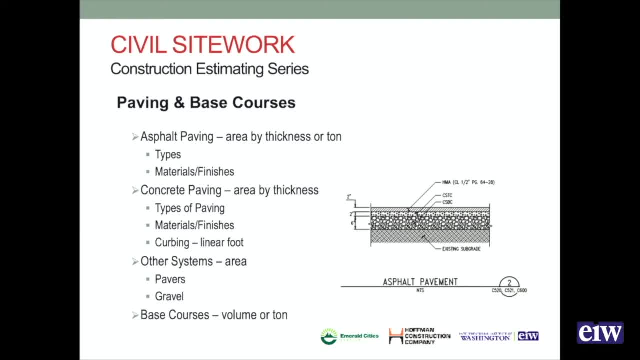 so you need to think about what am I going to do to make sure. am I going to proof roll that, or do I need to spray down a basically a commercial grade roundup to make sure that any kind of plants don't grow through that, because sometimes those are called. 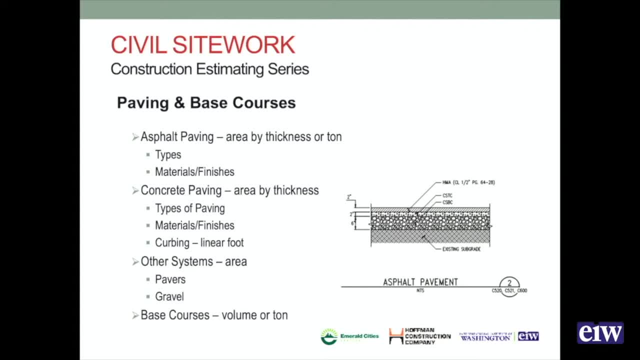 out to put a vegetative inhibitor there to make sure that you don't have a weed start suddenly start making its way through your asphalt paving. you may put down a fabric as well. those will be called out on your section details. so that brings us to the other side elements, the kind of the specialty. 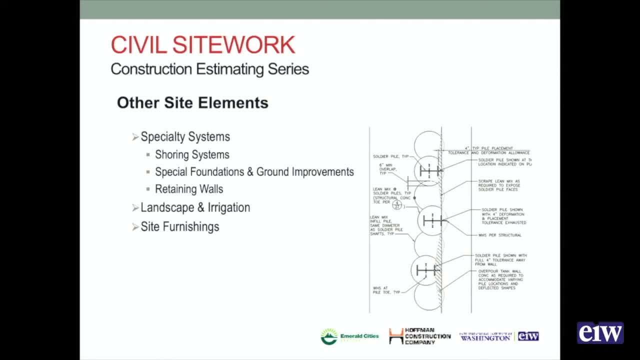 systems and I'm not going to go really in depth here because these are really more specialty systems. but if anybody wants to, you know, send Dan and I a lot of emails that you want to do another class on these. I'm happy, happy to do that. but these are like. 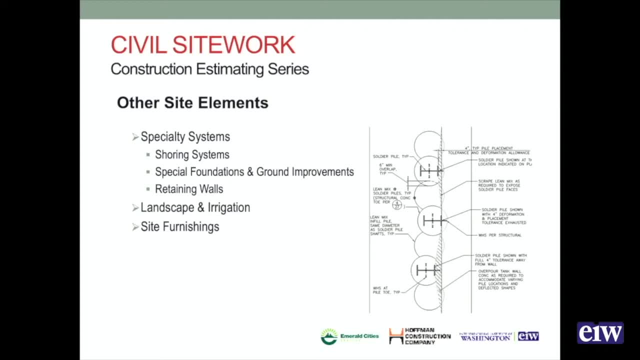 shoring systems. the example here that you see is a secant pile shoring system where you actually drill concrete shafts with steel beams in them to create a basically a wall, frequently used in a situation where you have water. so this is off of one of our 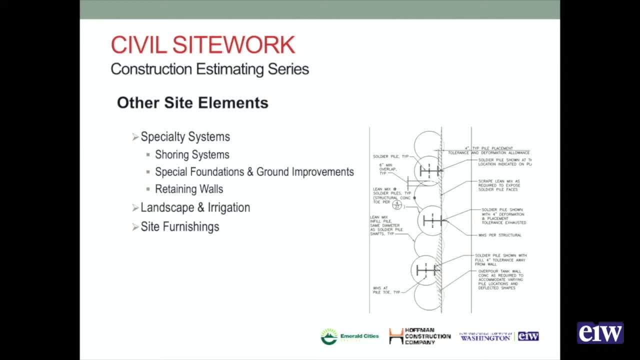 CSO projects that we built. so it's basically a giant water basin right next to Lake Washington. so you drill those down deep and they're deep enough where they can act as a cut off wall to prevent the water from the ground water from coming back into the. 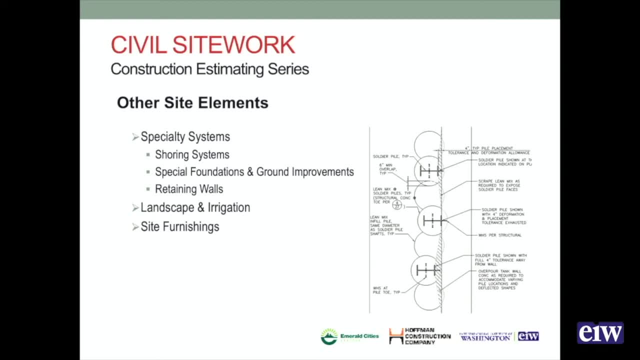 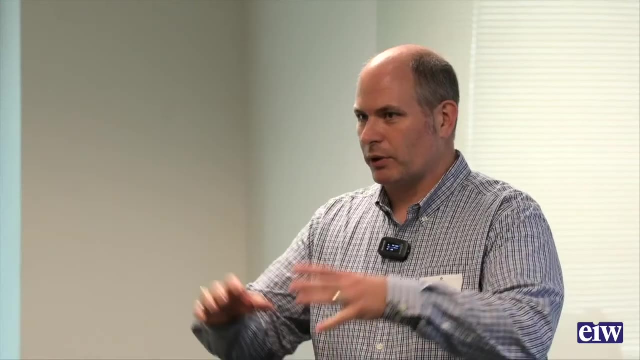 excavation, but there's conventional soldier pile and lagging systems. there's soil nail walls. it also would talk about specialty foundation systems, so piling, drilled shafts, micro piles, ground improvements like stone columns that you have to put in to basically shore up and increase the density and compaction and the bearing capacity. 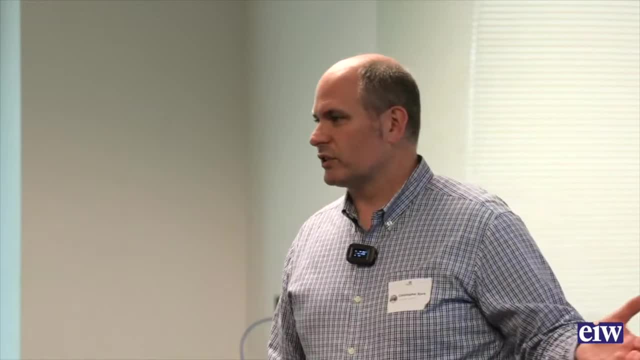 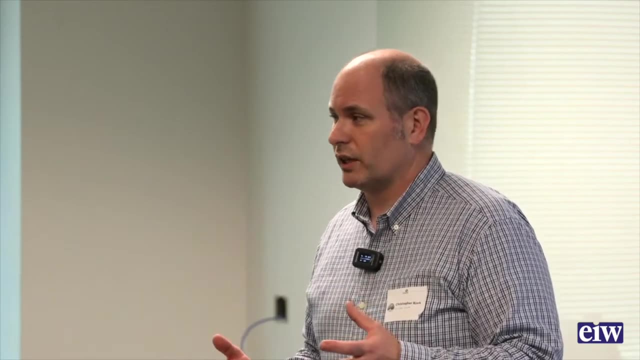 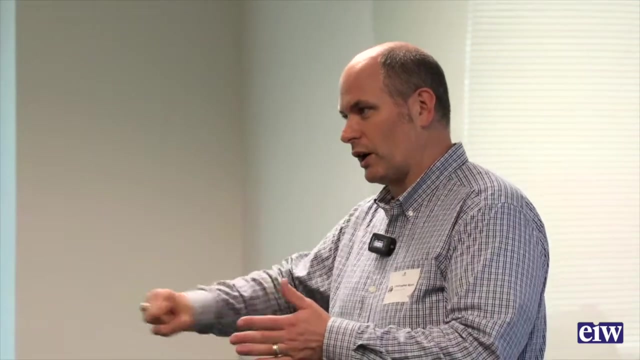 of the soil itself, retaining wall systems. so that can be as simple as a concrete retaining wall. it might be MSE wall, which is mechanical stabilized earthwork, so that's a wall where you actually build up the wall and put tension rods into the soil as you build it. 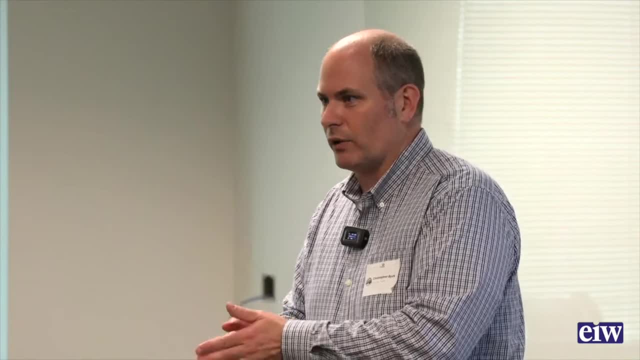 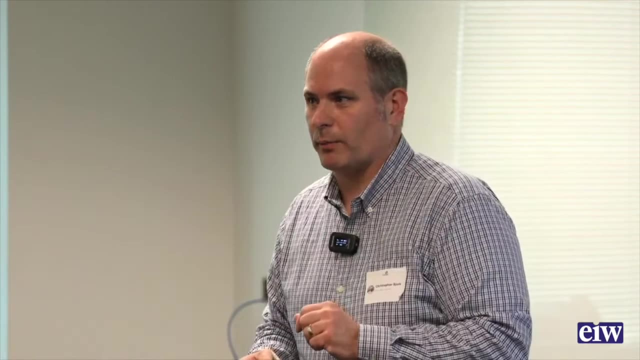 and they'll often times have facing on it whether it's a precast base or sometimes a shotcrete base. but it's another way to do it. you'll actually see if you drive up I-5 and you look at the thin wood length that is being built. 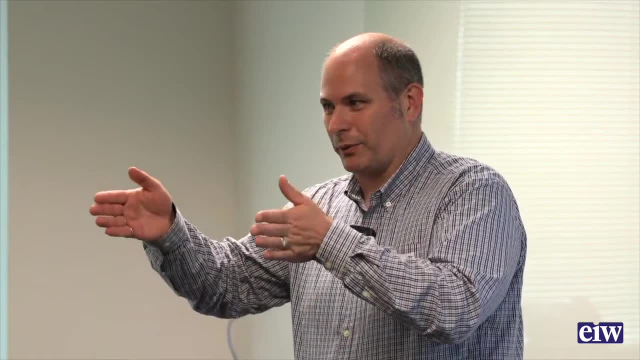 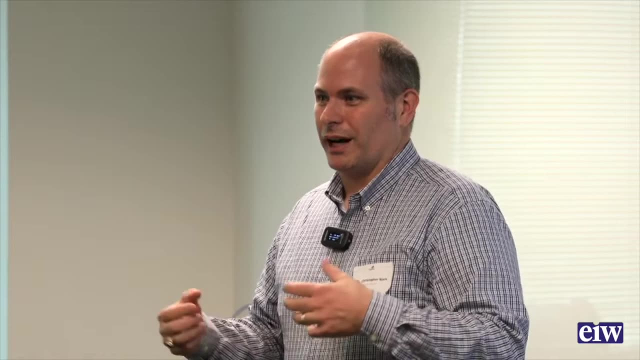 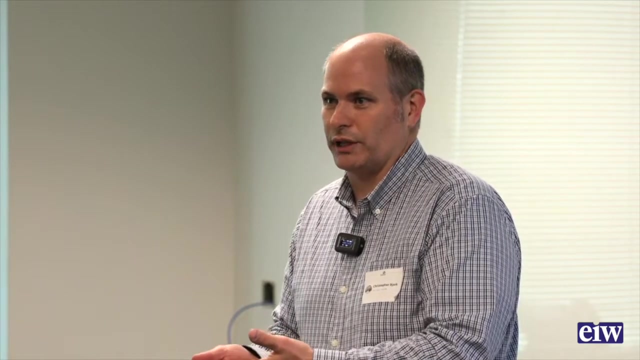 you see some of those walls that have where they're building the ramps and they've got little precast panels on either side of an excavation. those are mechanic MSE walls. they're tensioning those panels off each other to make sure that you have a structural retaining wall. 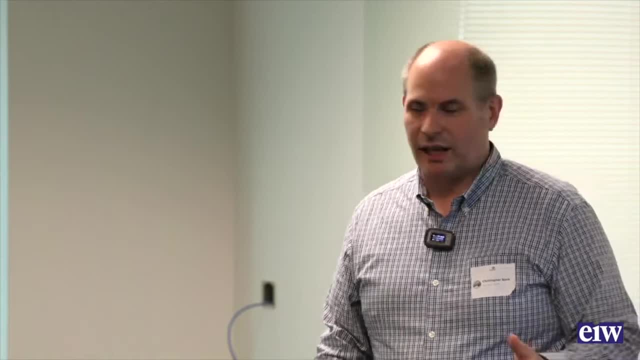 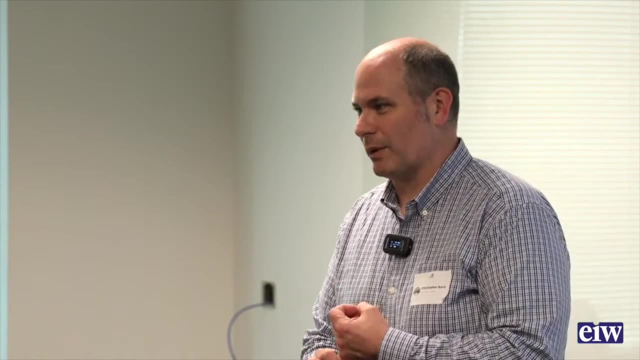 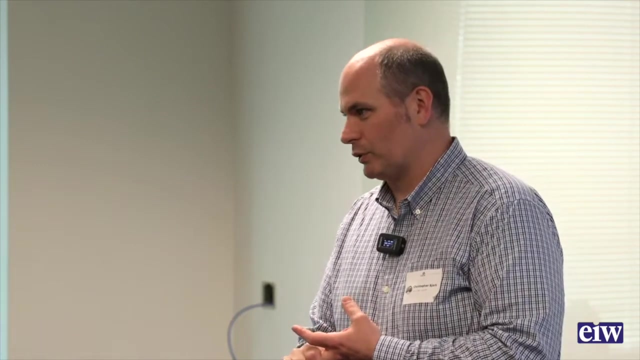 there other side elements, landscape and irrigation. now, landscaping is pretty straight forward. they'll tell you on the drawings what type of plants and how many of them. they'll tell you areas where you need to put hydroseed. they'll tell you what depth of topsoil. 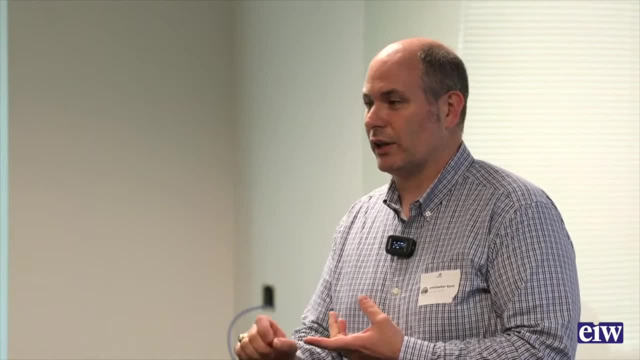 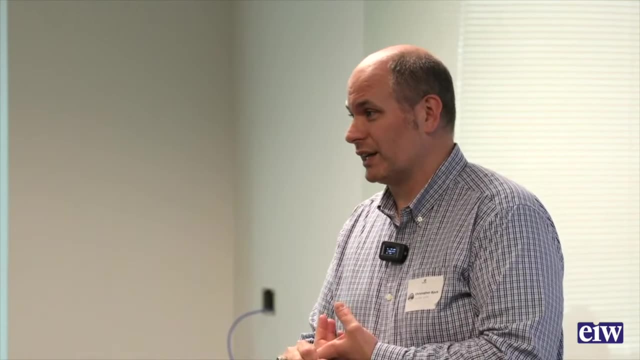 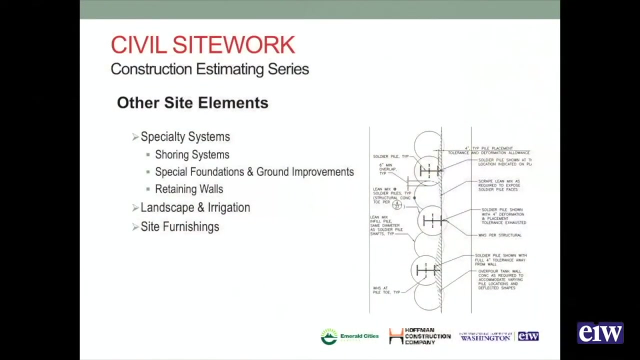 to put in and where to put it. they'll tell you, and usually it's a chart in the drawings. they'll tell you what kind of trees and, on the irrigation side, they'll show you where all the heads are and they'll show you where your main lines are. 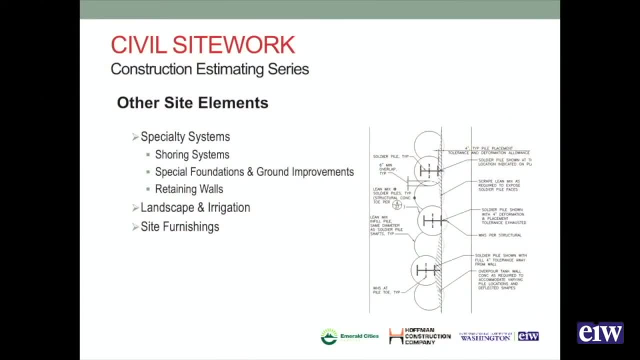 and where you need to put sleeves underneath paving furnishings. those are each counts. how many benches do I have? how many pipe bollards do I have? those things? you can figure out those labors, the labor to install, that fairly easy specifications will tell you who they want to buy that from. 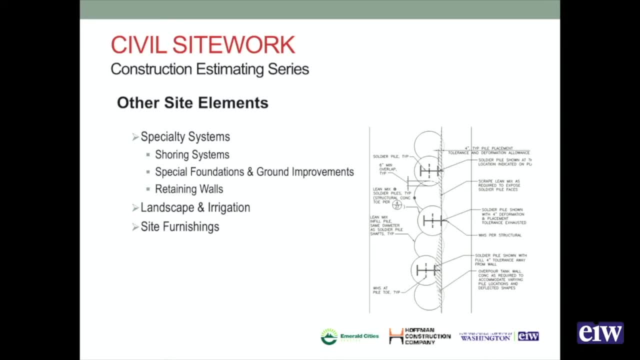 you can call that vendor up and get a quote- sometimes some of the vendors that are right online. you can actually just go online and fill out a form and within a couple days they'll email you back with the quote or they'll call you and start talking about it. 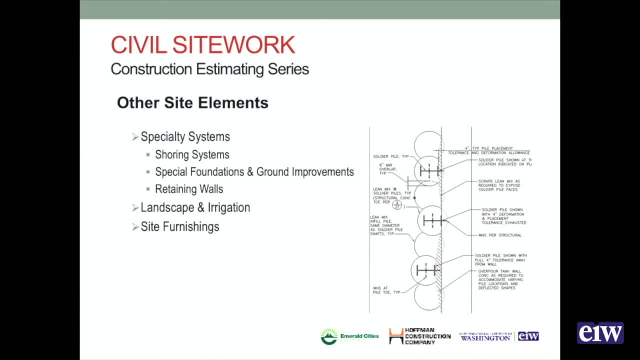 those are really the kind of specialty systems that you see a lot in site work, but they don't really come up necessarily as frequently, but you need to be aware of them as far as how they interact with excavations, because if you've got a shoring system, 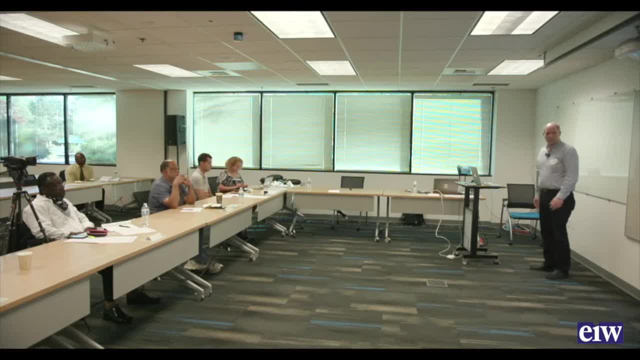 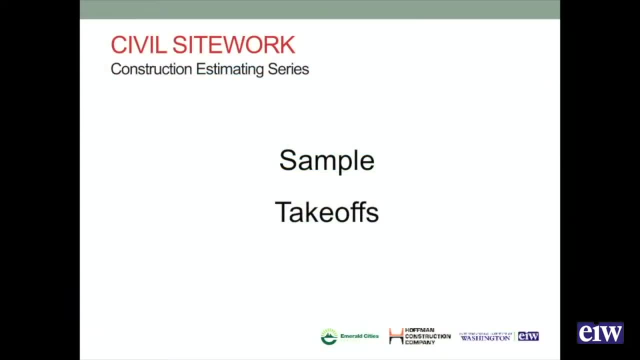 that's going to affect how you do an excavation, how you price an excavation. so that brings us to our sample takeoff section. so we're going to do three sample takeoffs. I'm going to do them using some of the screenshots that I've done, but very systematically. 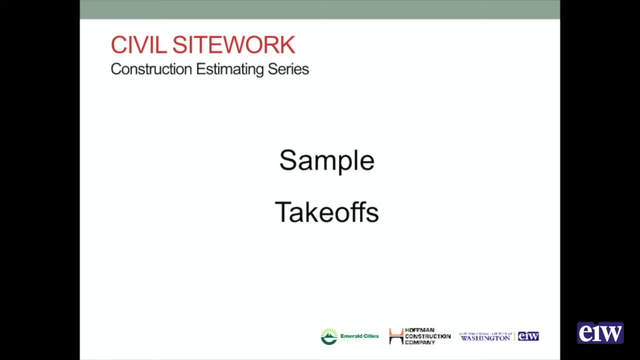 I've taken these off using Bluebeam software, which is a great software to use. you can do with the PDFs. it's very proactive on how to take things off. there are a number of other different softwares out there, whether you use OST or something else. 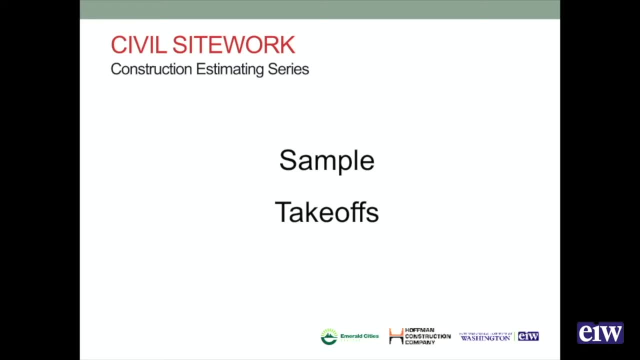 even if you're using a scale or a wheel. for those of us who remember using those items, it's the same methodology. now I just use the computer technology to aid and help me to do it faster. so we're going to start off, we're going to do a sample of 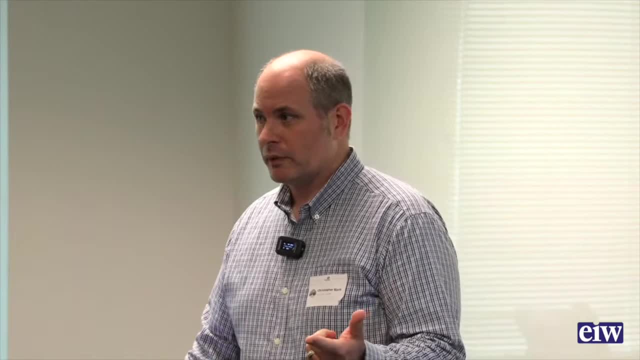 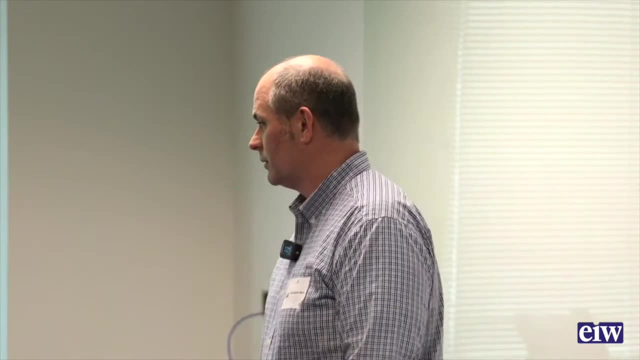 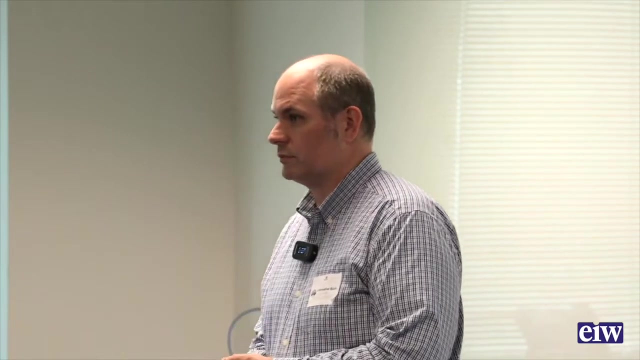 demoing a room, then we're going to look at a storm drain, and then we're going to look at an asphalt paving area. quick, before we move forward, just a quick round of hands. what kind of software programs are we using right now? so raise your hand if you're using. 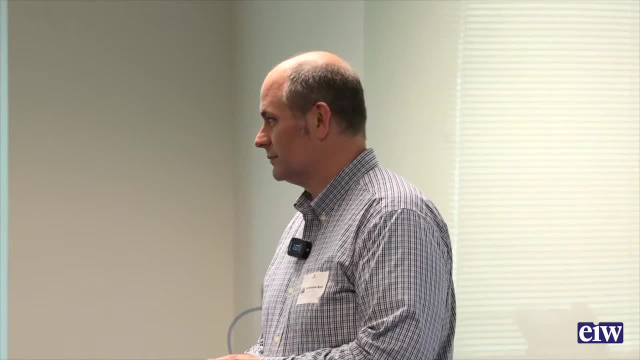 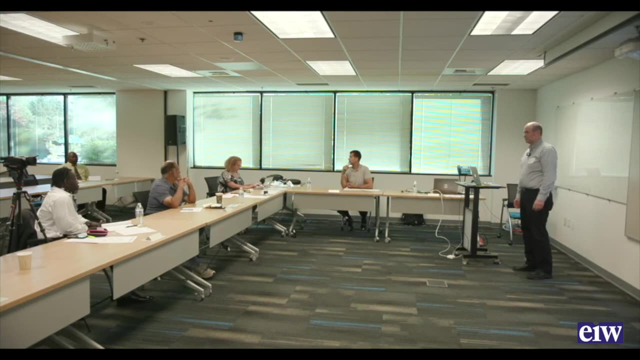 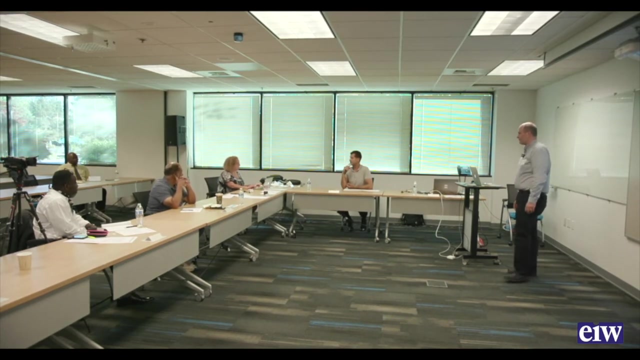 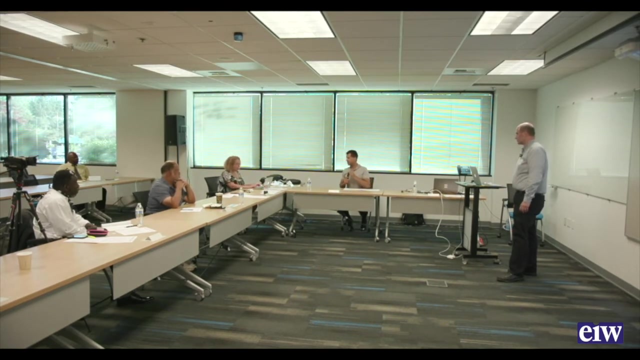 Microsoft Excel: ok. Bluebeam: ok. RS Means any other applications that you may be using. ok, what kind of responses are we getting in the chat? ok, wonderful, wonderful. I'll be curious to see if there's any other conversations in the discussion. sorry, no, no, that's great. 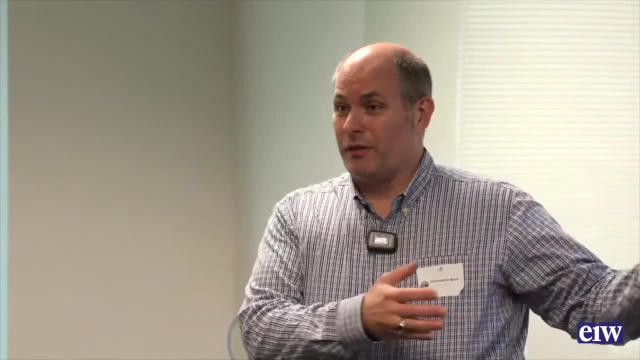 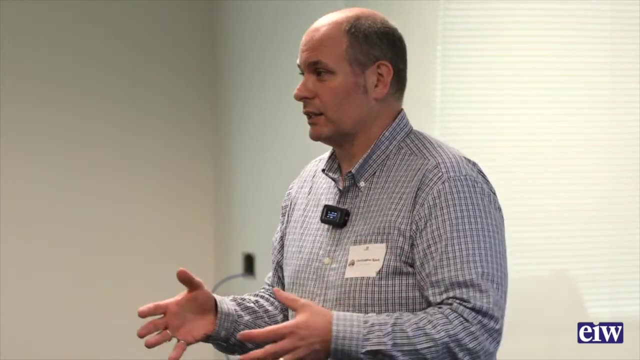 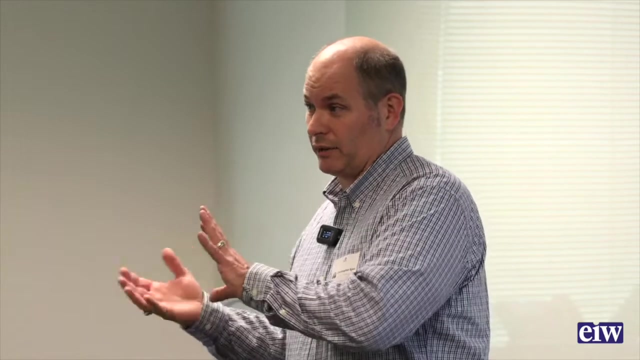 and just to piggyback a little on what Dan was saying and add to that the summaries I have, when we get to a summary and actually the pricing information we're going to use, we're going to use Excel and while we have a software estimating software program, 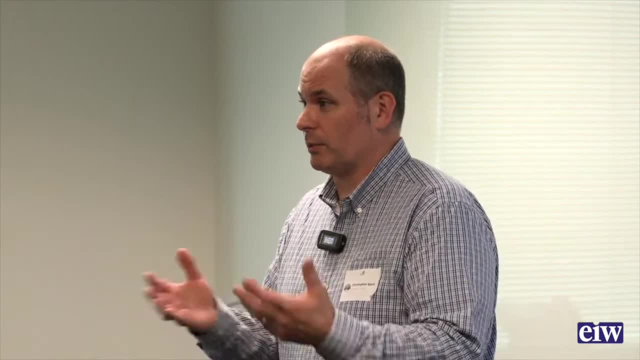 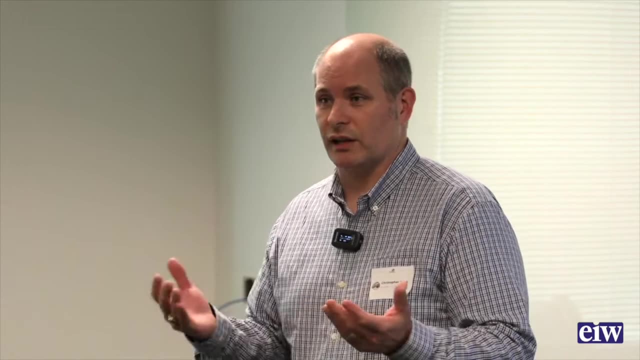 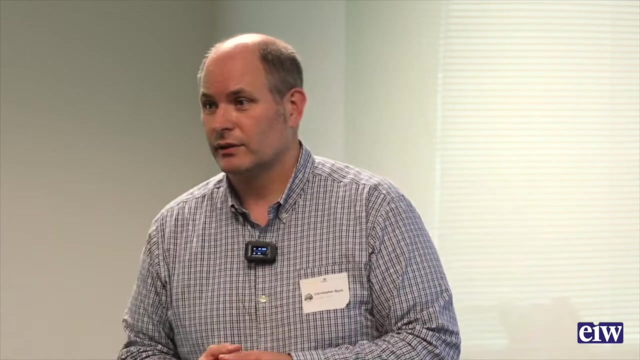 we actually take that data and export it to Excel because Excel is a lot easier to manipulate. when you need to manipulate things- and Excel is a perfectly fine- we used to use Excel and it's a very flexible way to generate quantities and price things out. yes, so when you guys. 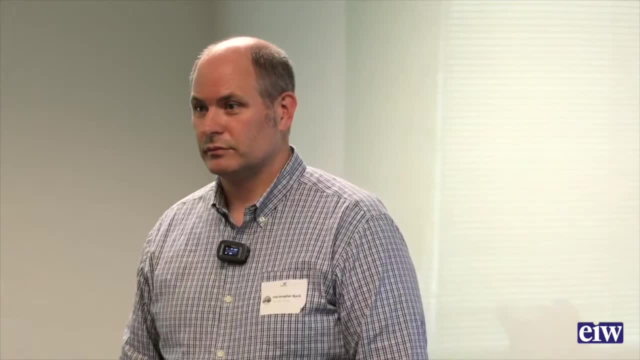 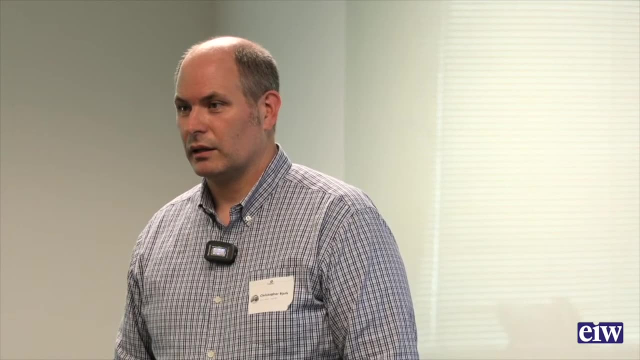 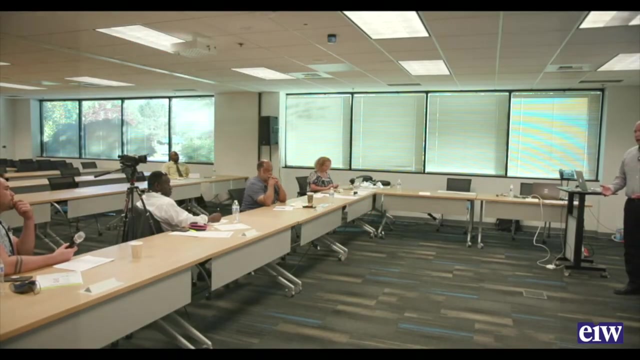 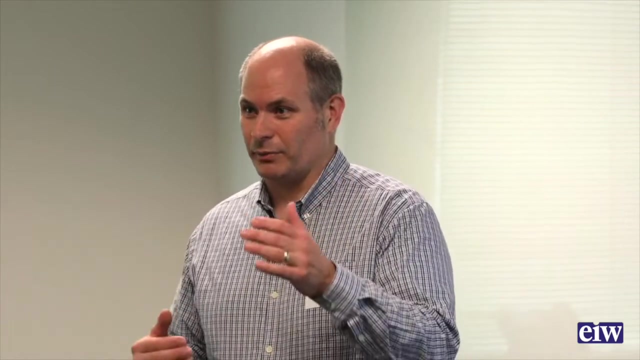 sell. do you actually get your own software, your in-house software, somewhere to make your to do your estimating? yes, so when I first started with the company, we used Excel, so we had a number of different Excel templates that we developed over the years and pricing guides and summaries. 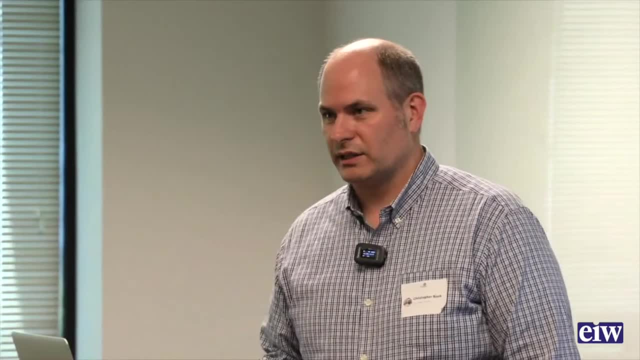 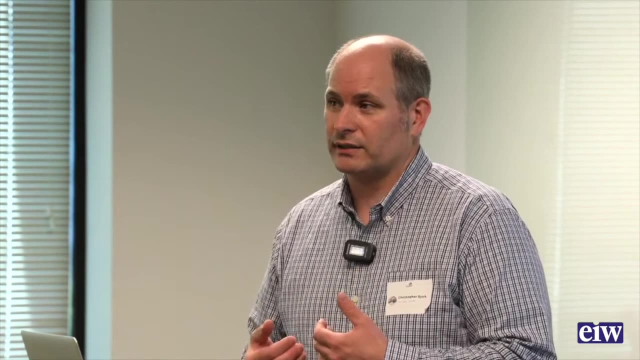 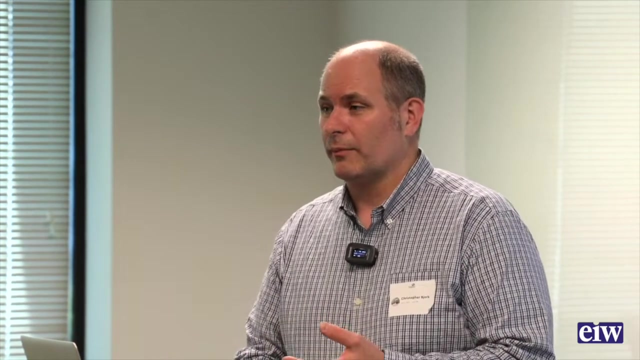 that we used. we then switched to estimating software. so we did a. we looked at different estimating softwares and there's a number. we use Beck's Beck Technologies Destiny Estimator, but there's Timberline, there's WinEst In8. there's a number. CostOS is another one. 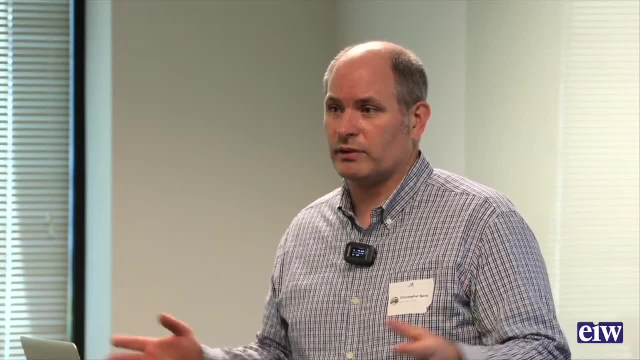 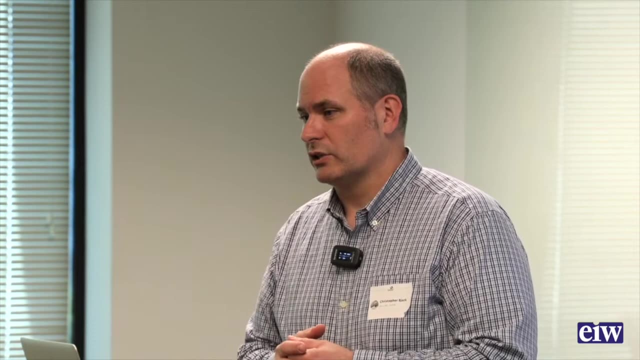 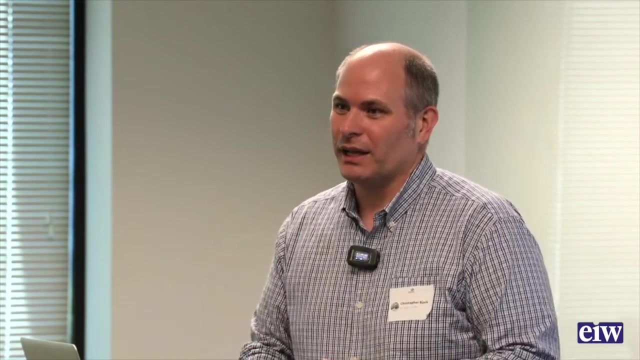 there's a number of other software programs. they all cost money, they all have different costs things, and so if you're looking at estimating software, which is a whole other, another topic, but it's important to test drive those things, those different softwares, to figure out what works best for your situation. 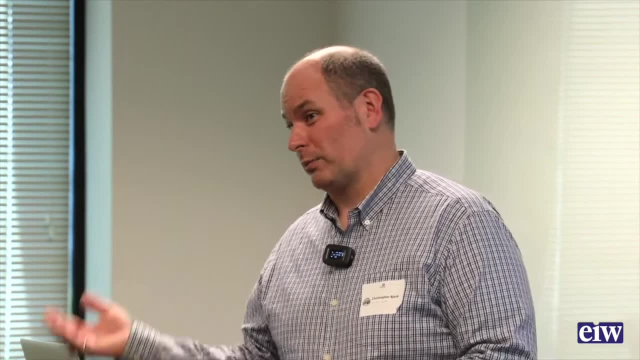 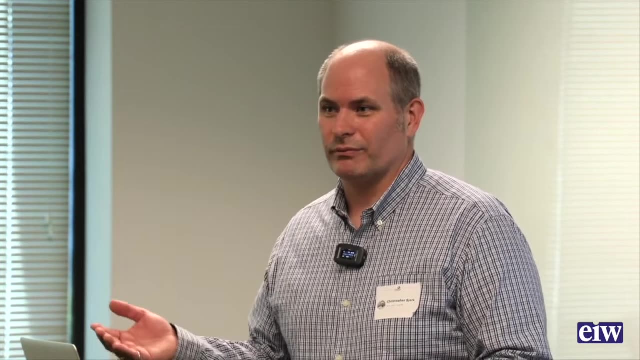 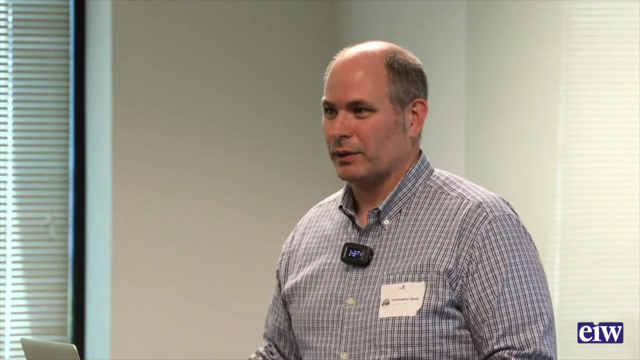 and both in what it provides and what it costs, because you may need something that doesn't need to have necessarily all the bells and whistles for what you do. so you don't need to pay for all the bells and whistles because some of them can get. fairly expensive, especially when you start tacking on maintenance, maintenance terms and support and service terms. that can start adding up into tens of thousands of dollars, depending on how many licenses you need. a lot of times you'll find that they have different modules that they want you to. 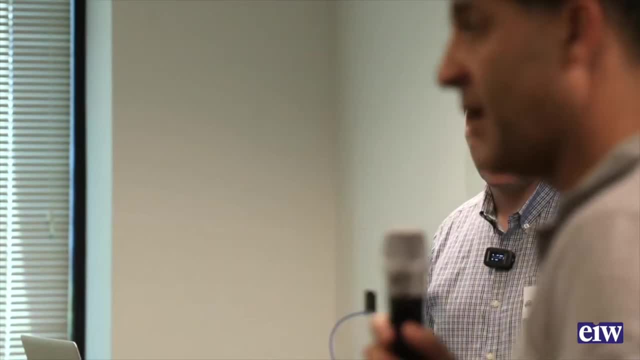 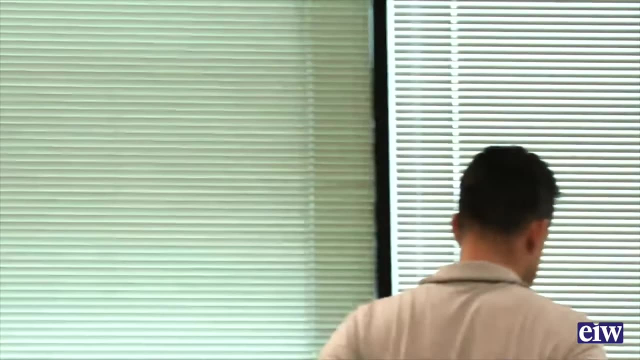 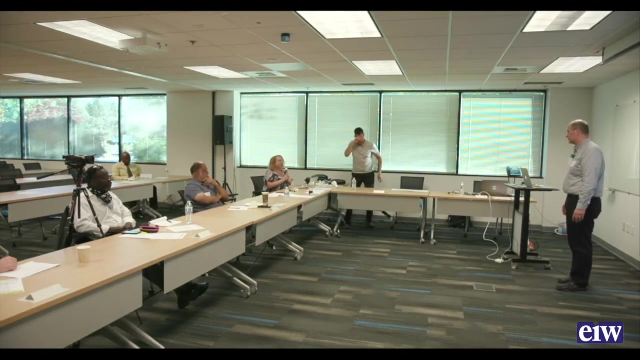 give consideration to, and then you also have to think about how well it integrates into your accounting system, and that may be also a consideration. please, Rosalyn, hang on, let me get you the mic. so at Emerald Cities, we have been wondering about how best to support e-contractor. 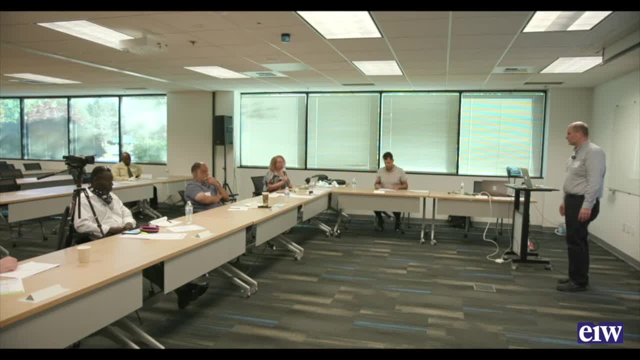 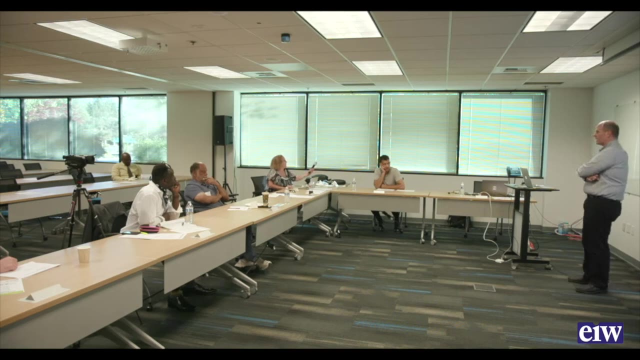 participants. maybe in bidding on larger work, is there a possibility that we could acquire one of these software packages and allow licenses to be shared by some of our participants to limit cost to them? you would need to contact the software companies often times- I know often times some software companies- 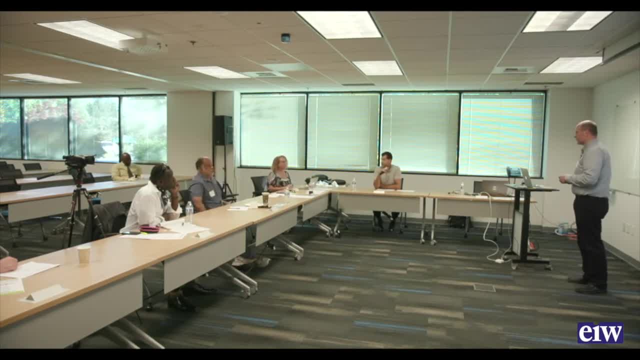 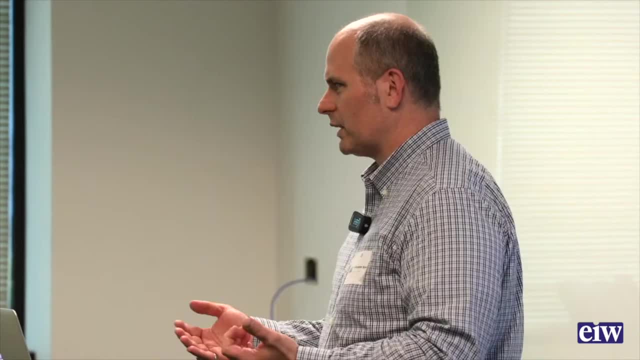 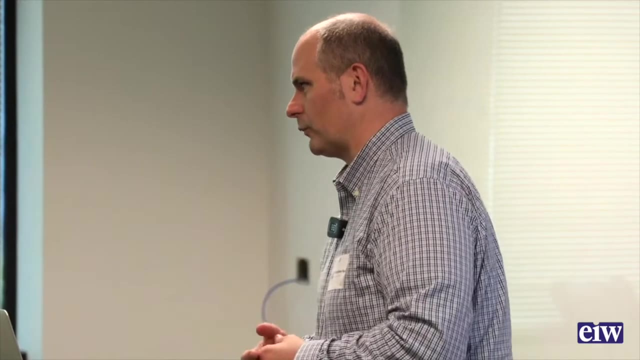 give a license to a particular person and they have to be named who that is. but you may be able to work something out on something like that if you have a limited amount of opportunities. that's something you need to get into a discussion with that particular software company. 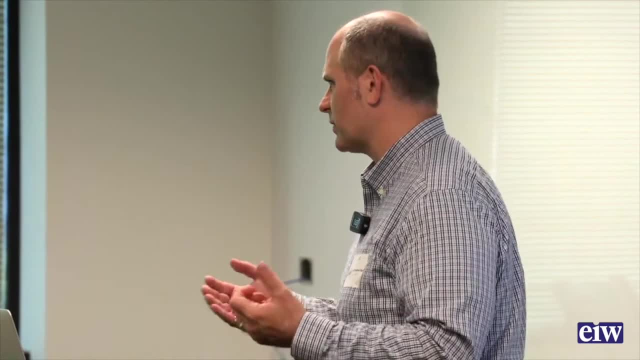 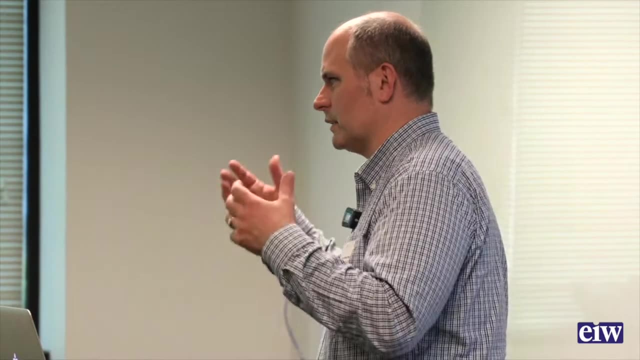 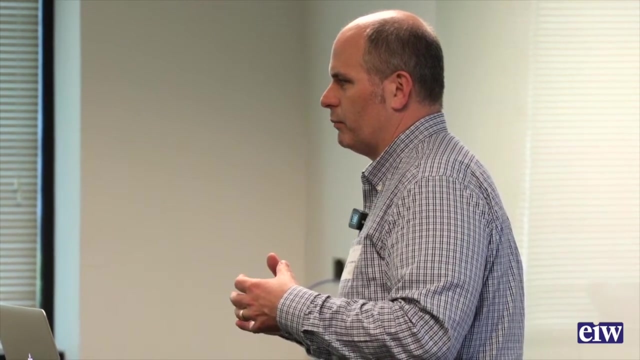 for certainly we have something like that with some of our other software, like the Autodesk, the BIN, the software Revit and Navisworks, where there's a set number of licenses that you can be used and every time you open up the program you check out a license. 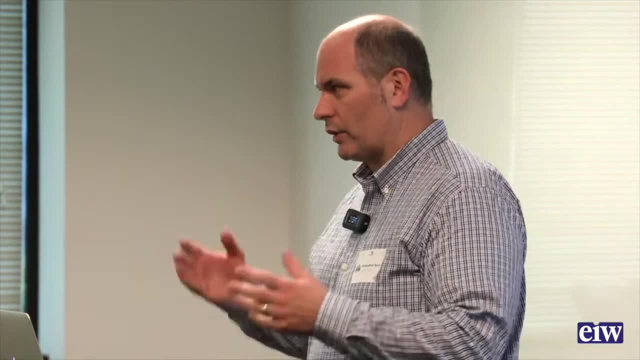 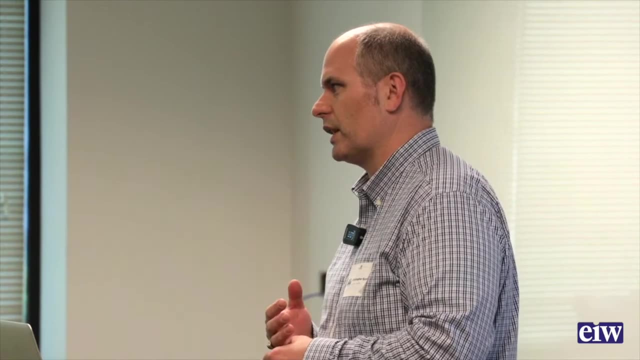 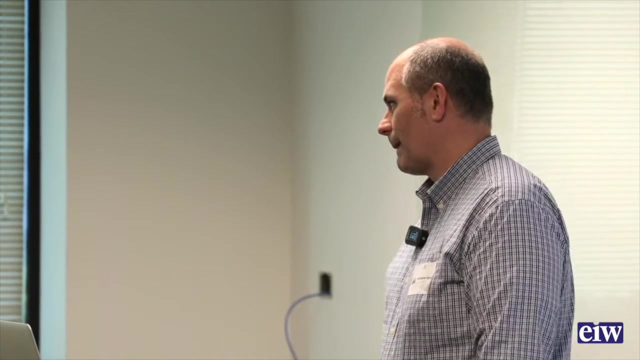 and if all the licenses are checked out, you can't open up the program. so there are opportunities there, I think, but you need to really talk to the software companies to make sure what their ideas are. yeah, that's a great question and actually we, the Entrepreneurial Institute of Washington, 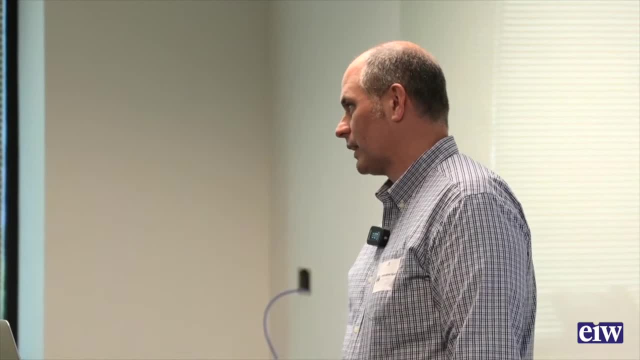 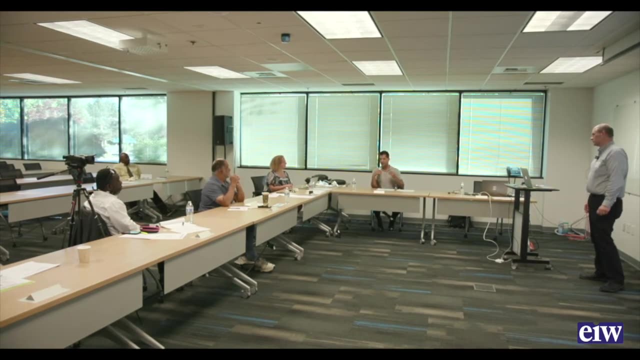 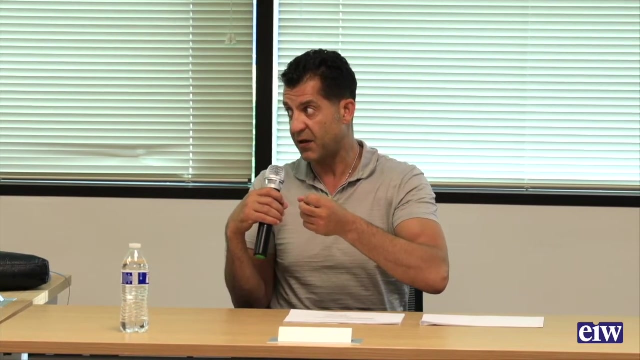 has ambitions of acquiring different subscriptions that will help enhance the members and small businesses capacity. the challenge is: we're working under the non-profit environment, which is helpful because they typically give us a pretty good price and also we have to do. we do, unfortunately, have to pay. 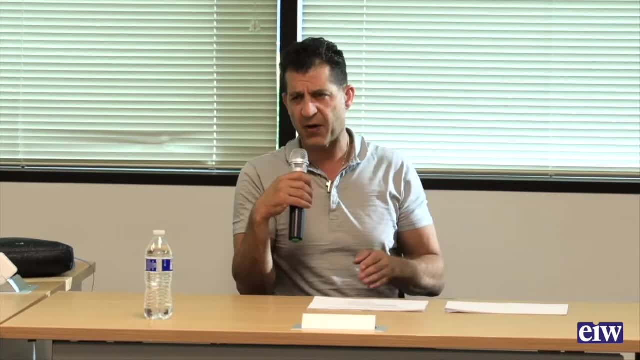 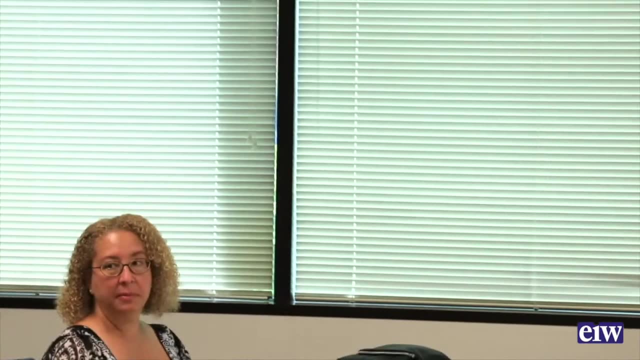 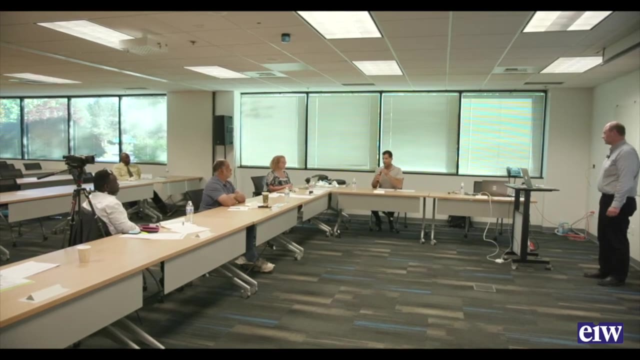 for those individual users. we're doing that currently with RS means, pardon me, as well as construction market data. Tim, I'm coming to you, ok- our sponsorship with Hoffman. I believe that's part of the evolution of the relationship. the other thing to think about, too, in terms of estimating software: 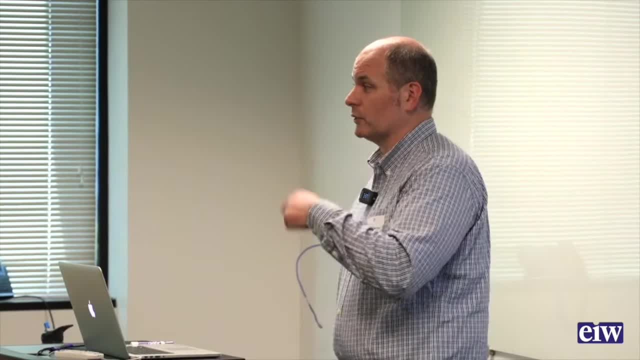 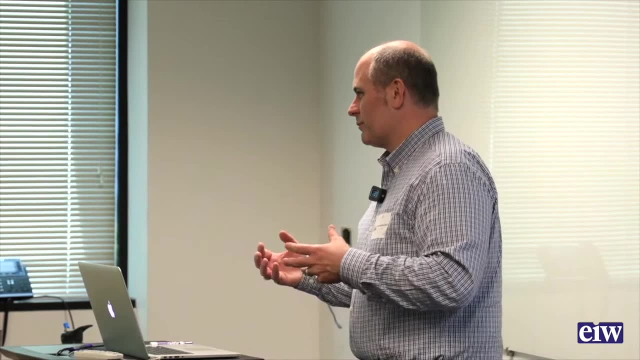 a specific estimating software program is: do the people who are going to be using it know how to use it? because there's a training involved with that and every estimating software in general. if you know how to operate one, you'll be able to figure out how to operate another. 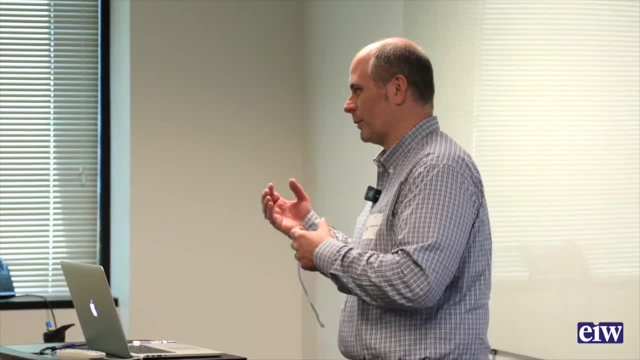 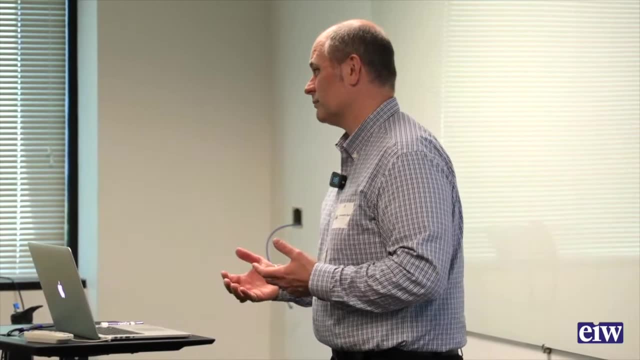 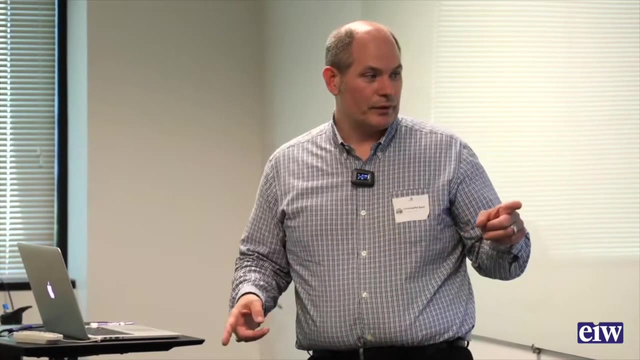 but they all work a little bit differently and some of them are more user friendly than others, so they're not necessarily always really intuitive on how to use them, and that's something you would need to think about. one thing for everyone: here in the classroom we have provided: 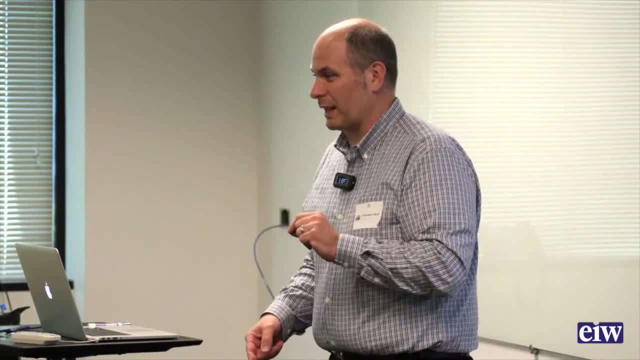 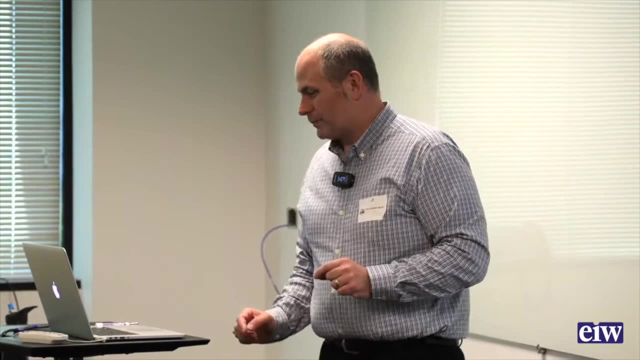 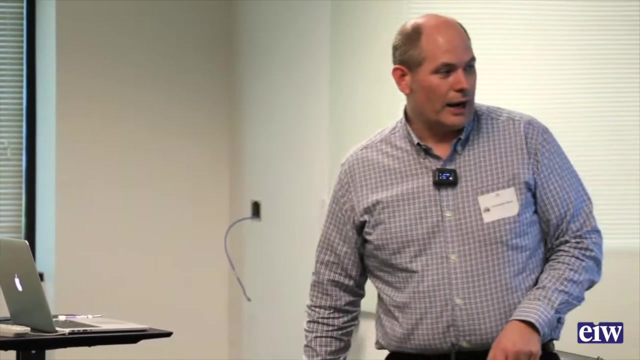 because I know some of this gets a little bit smaller for the people here. we have provided these sample take off slides for you so you can follow along and make sure that it's a little bit easier to read for you. so, starting off selective demolition, we're going to demo this room here. 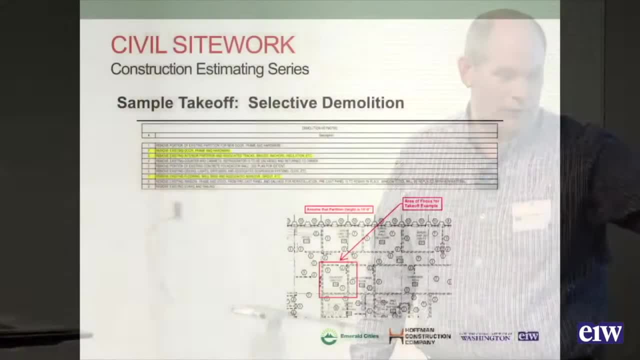 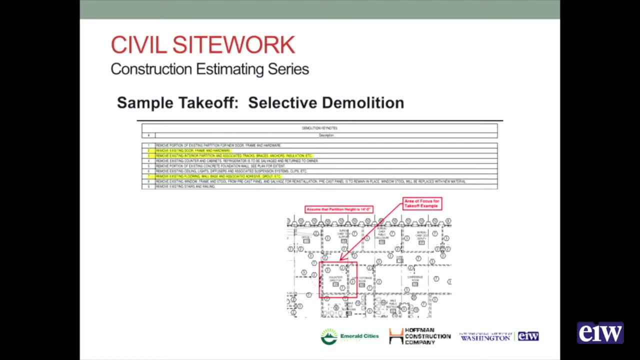 and if we look at this, we're going to assume, to make this easier, all the partition heights are 14 feet high, which is actually what the floor to floor height of the building is. but if we look at this, we've got three key notes. we've got note number. 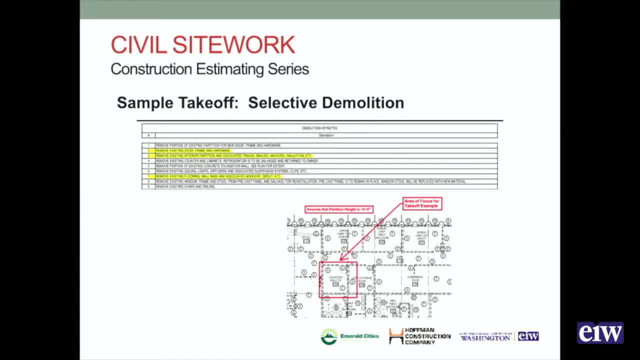 3, we've got note number 2 and we've got note number 7, so note number 2 says: remove existing door frame and hardware. 3 says: remove existing interior partition and associated tracks, braces, anchors, insulation, etc. and 7 says: remove existing. 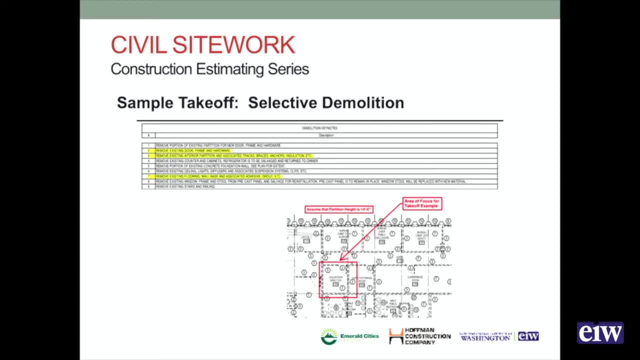 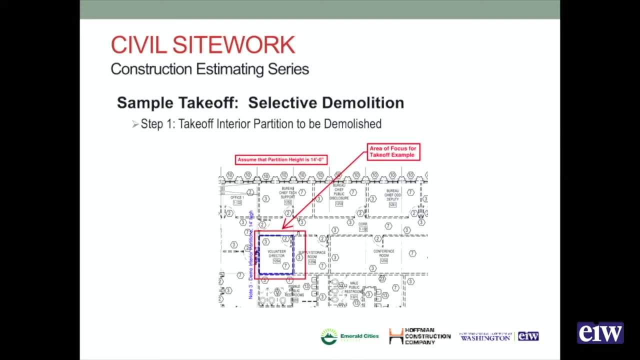 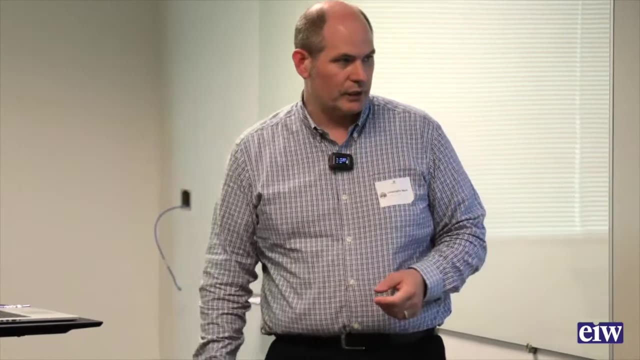 flooring, wall base and associated adhesive grout, etc. so you can see that the area that we're going to work in. the first thing we need to do is to take off the wall. we know that it's 14 feet high, so we'll take off the lineal footage of it. 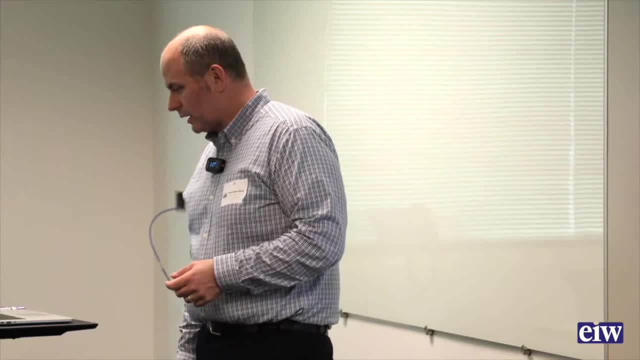 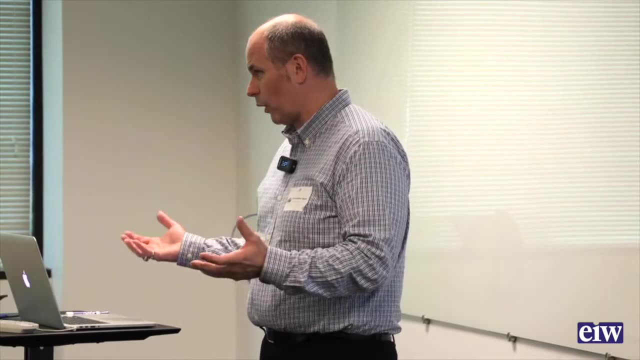 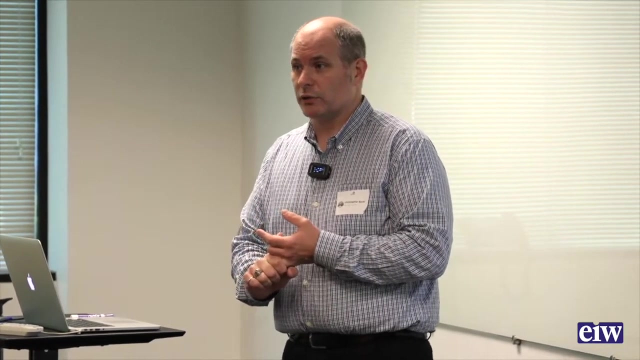 that lineal footage is about 40 feet, so that will help us to be able to generate footage of wall, which is what we need to both find out how much weight that we have for it and how much labor we need to use to demolish the wall. 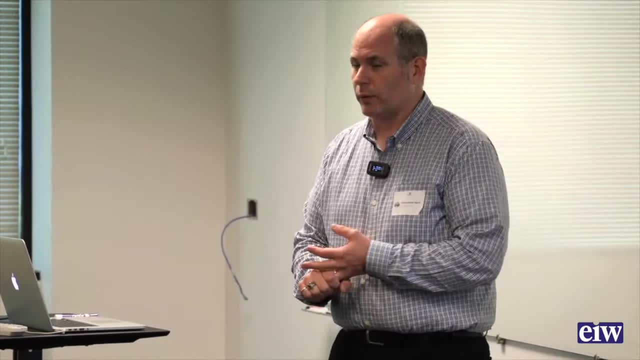 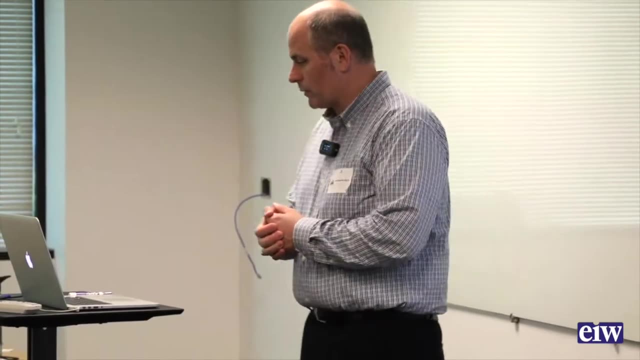 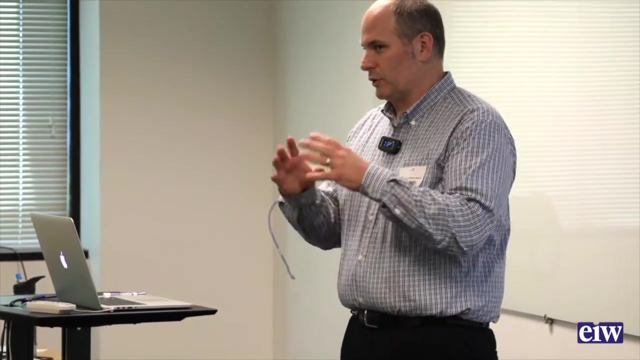 second item is to look at the interior door frame and hardware. that's an each count. we've got one each right there, so we'll note that in our summaries and then we will take off the flooring and wall base and one of the great things when you're using. 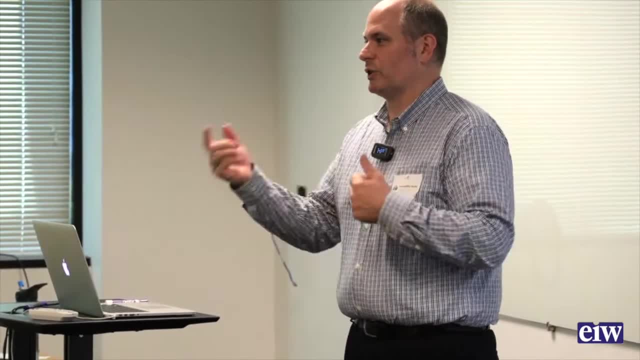 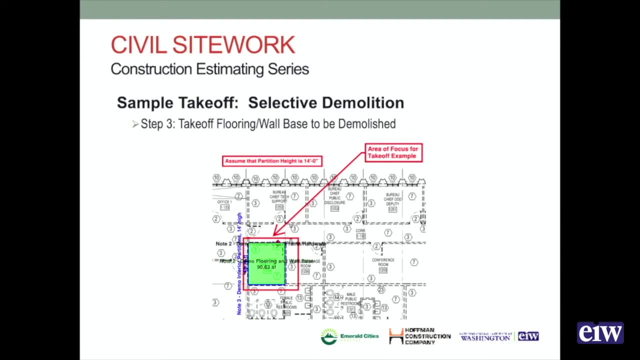 blue beam type software is that when you take off the area it tells you the perimeter as well, so you can use the area for the flooring and the perimeter to take off the wall base. so that tells us that we've got about 90 square feet of flooring and then 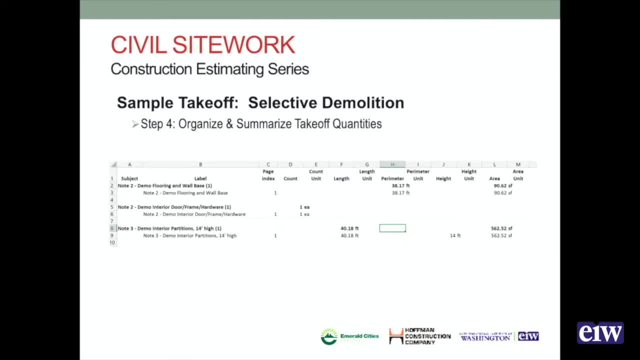 when we get to what the, if we move to what that blue beam summary is, it will tell us that we've got a perimeter of 38 lineal feet. so this tells us- and this is- I will caution this, because this isn't we're looking at- estimating and not 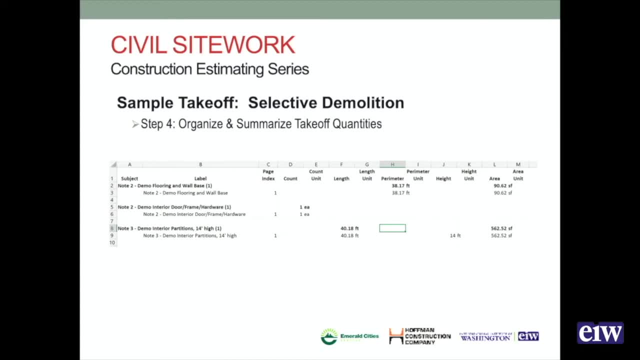 how to use blue beam. this is cleaned up a little bit to make it a lot easier, and that blue beam has a little bit of a process when you export your quantities into excel, on how to get them into something that's a little bit more readable. it's a straight. 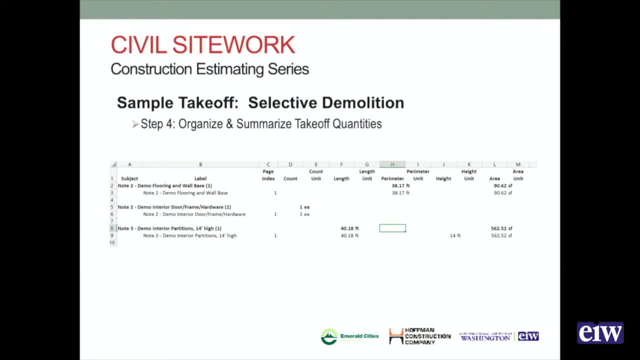 forward process. but there is a process with it. so there's what your quantities are. so you have your quantities in a nice summary format. so you understand what the work is that you're going to be pricing. now, Chris, really quick, go back one screen, and so, in this case, 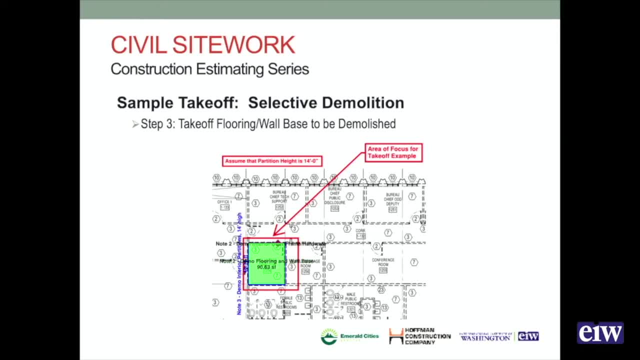 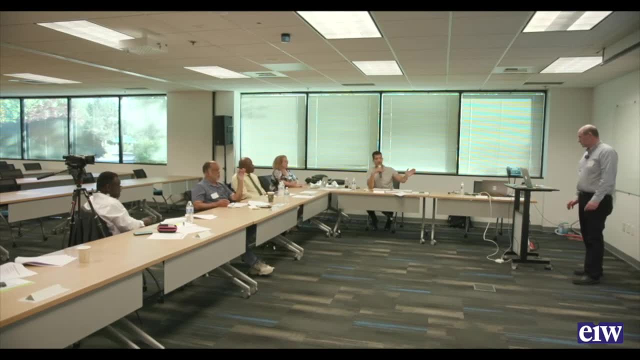 this is a one action. you decide that you're going to calculate the measurement, in this case for area. you identify what the scale is and then you click and you hold and drag over that area. so it's really kind of a one click or two click kind of action. 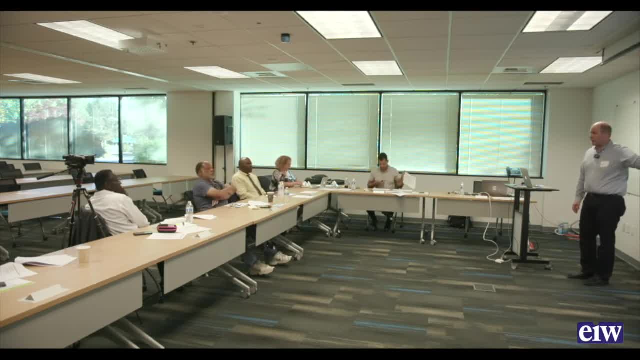 it can be so using blue beam. if you've got a nice square like that, you can click one corner and draw it to the opposite corner and it'll draw the square for you and compute the area and the perimeter for it. if you've got an unusual, 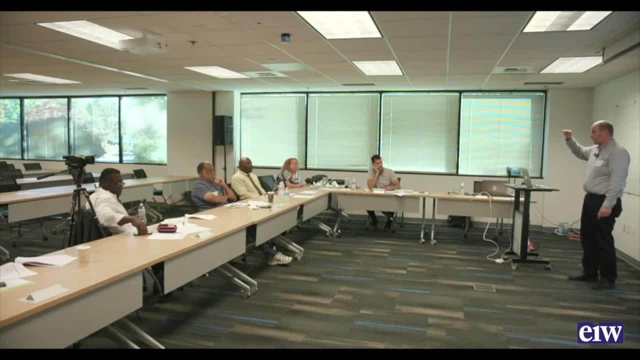 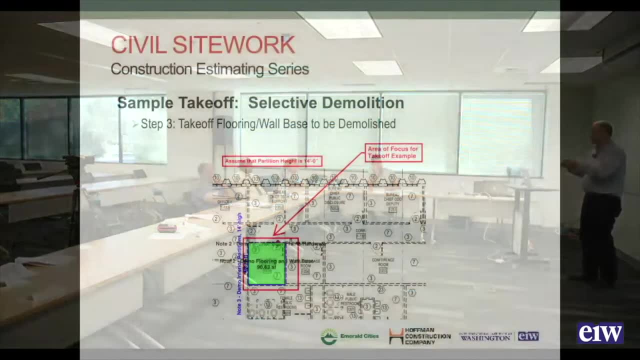 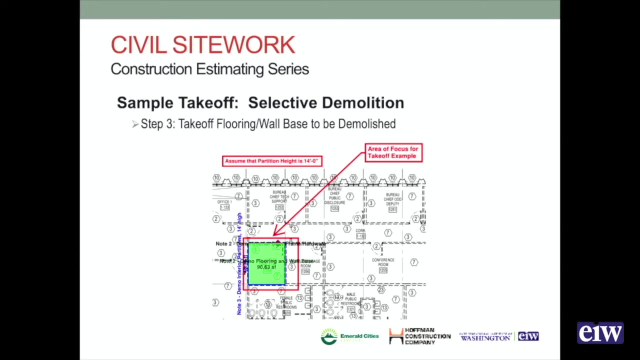 shaped area. you can click on each point and you can click around curves so that you can actually create that area there and it will still tell you the area and the perimeter. you can actually also take out areas so if you have a slab or an area with a hole in the middle of it, 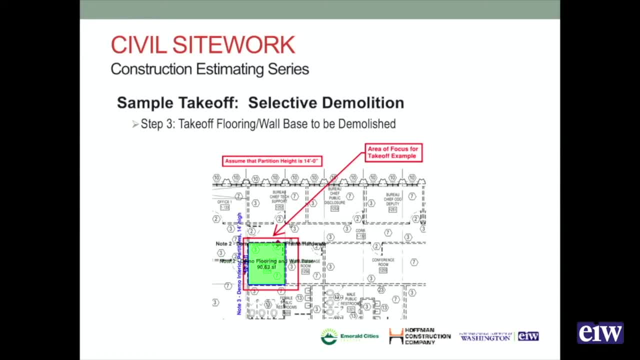 you can go back through and click on a button that will allow you to take out the hole. now, the caution with that is that it will compute the area without the hole, but the perimeter is the perimeter of the edges, so the perimeter will include the perimeter of that hole. 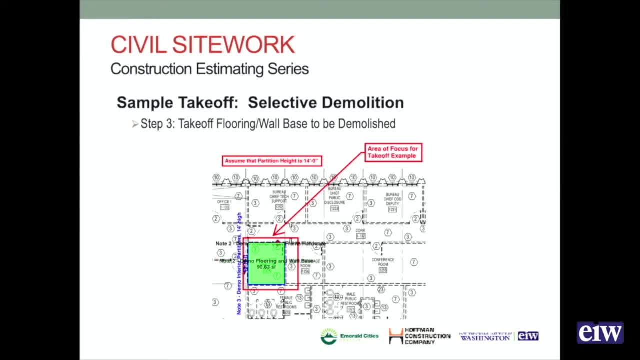 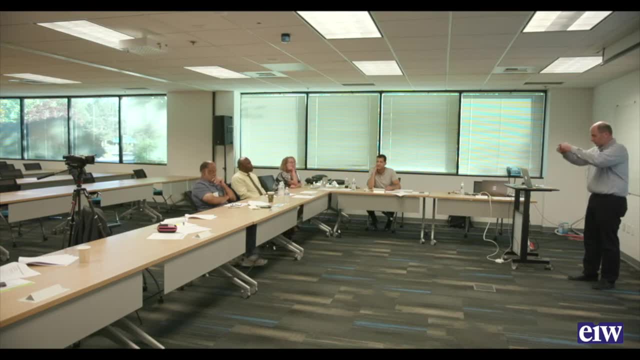 so it's something that you just need to be aware of when you do your quantities, because if you're looking at, say, a curve around the area, but you've got an area where it doesn't have a curve in the middle of it, on a paving section. 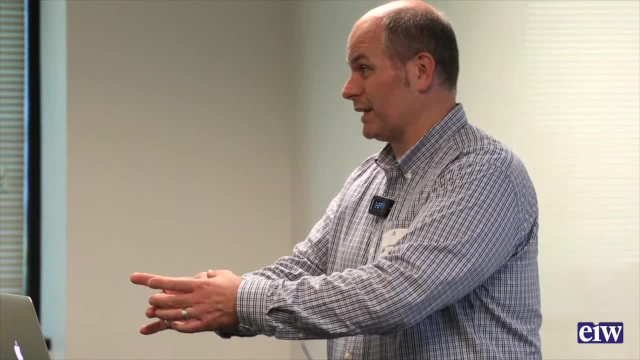 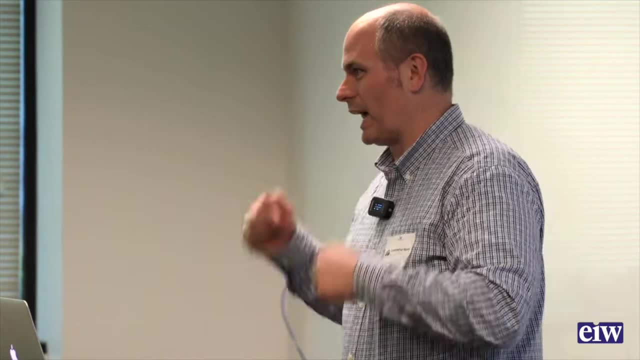 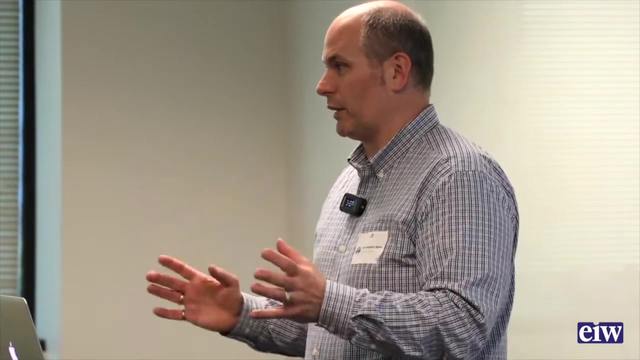 but there's a hole, say there's a landscaped area in the center of it. well, you might want to take off the edge perimeter in a separate action, because you don't want to put curve where you don't have curve. and if you just took the perimeter area? 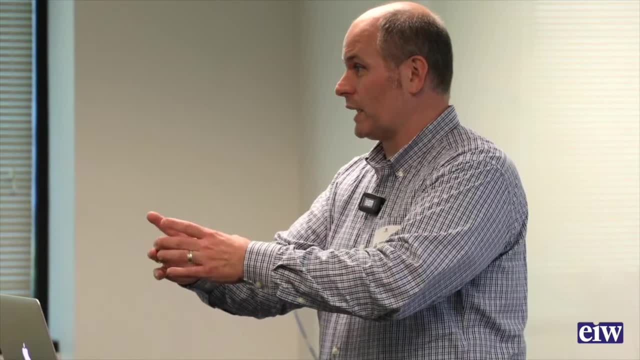 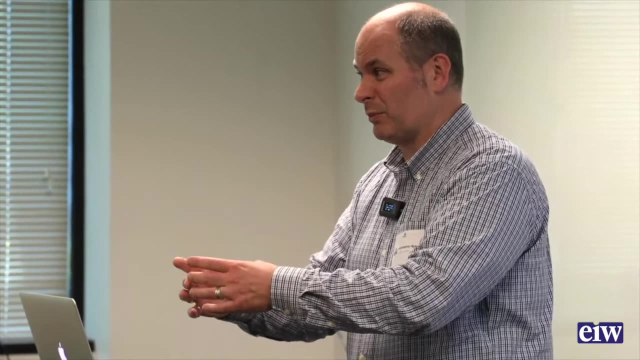 of an area with a block out in it, you're going to get to have that lineal footage of block out in there as well. and if you've got the lineal footage of block out in there and it doesn't have curve but everything else does, 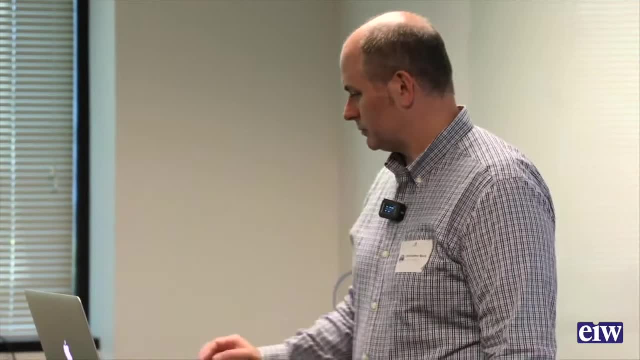 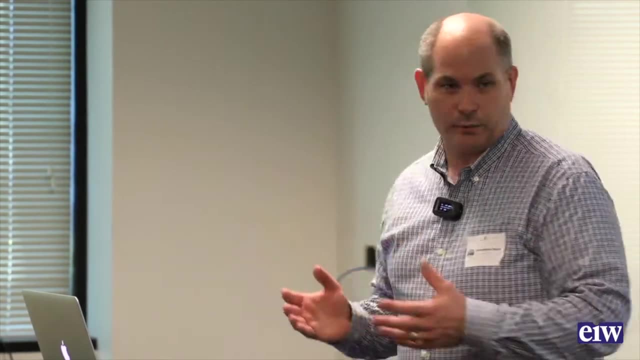 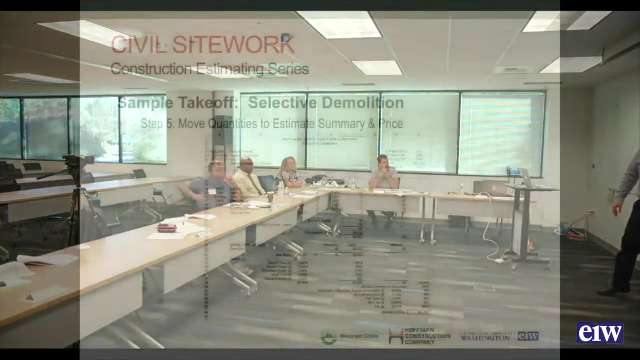 then you've got too much curve in your estimate. so then we will move on to what the estimate summary is, and this is how we really price out the estimates. so these, here's our quantities. there we've got our square footages, we've got our each counts. 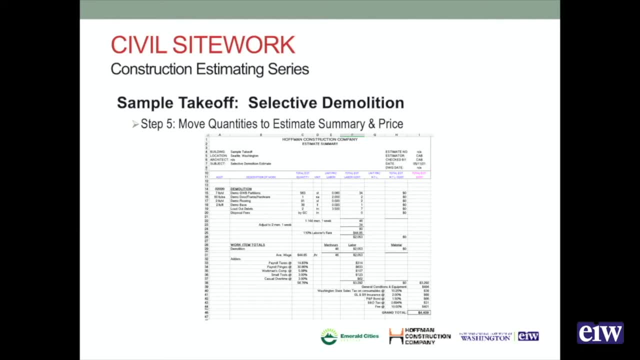 and over here we have. what I've looked up for me in my steel manual is the unit weights of the different materials that we are demolishing, so that I can compute that we've got two tons of material. we've got two tons of material to haul off. 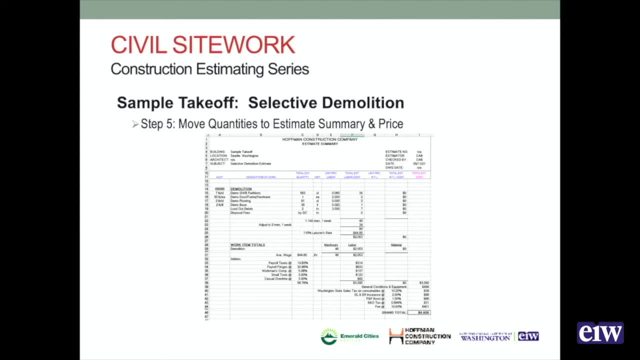 this particular job, the general contractor is going to do it for us, so we don't have to worry about disposal fees and tipping fees. but then we, to price it, we look at our productivity units, which are going to be: how many hours per unit do you have? 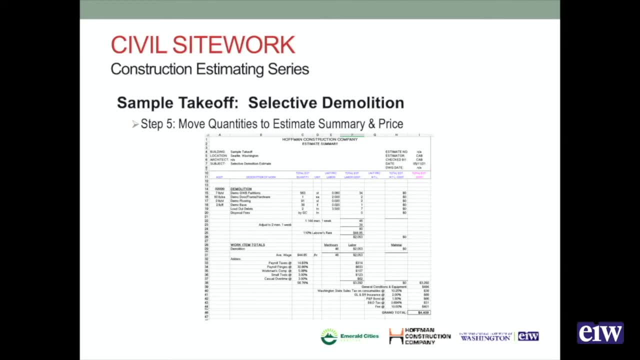 so hours per square foot hours per lineal foot hours, per cubic yard hours per ton for the haul off the quantity times, the productivity unit tells you how many hours total you have. you sum up the hours and then with this I've done a back check on this. 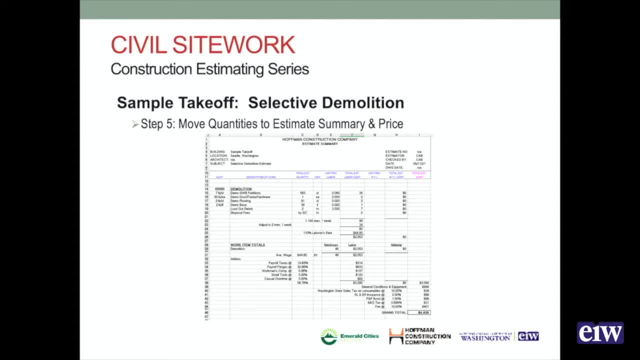 because if I see I've got 46 hours, and if I have 46 hours and I've got one week to do the work, that tells me that I've got 1.145 men or workers per week. well, I don't have .145 workers to put on a job. 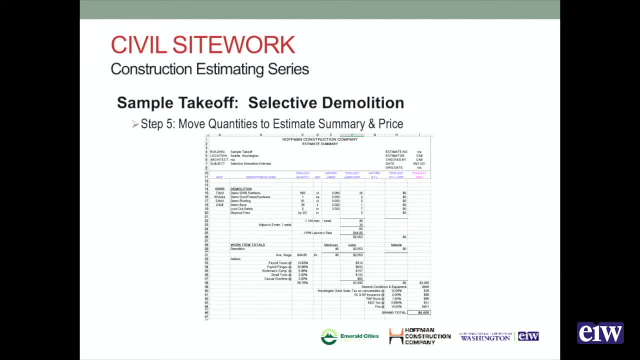 so in this case, I've said: well, I'm going to have- I'm really going to have- two workers there, because I'm not going to have one worker do the work. I'm going to have two workers do the work and they're going to still take a week. so I need to add some hours. I need to add 34 hours in there to bring it up to 80 hours so that I have two workers for one week. so once I have those hours, then I can figure what my wage rate is. so for here I'm figuring that. 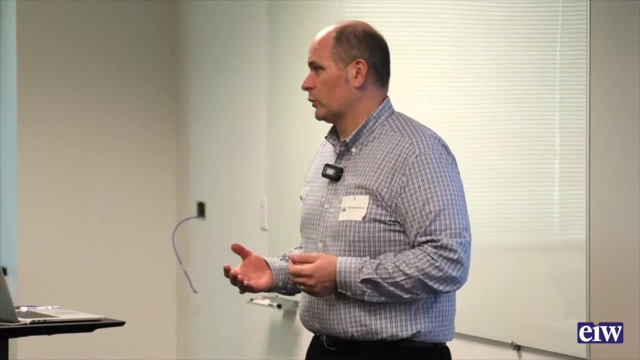 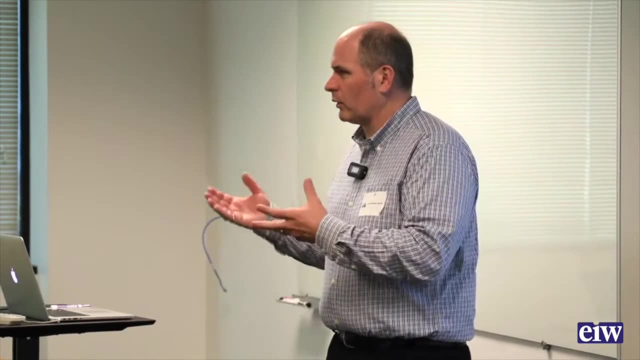 110% of a laborer's wage, because one of those workers is going to be a foreman and one of them is going to be a journeyman. so I need to factor in a little bit more in that wage rate and then I'll sum that up. 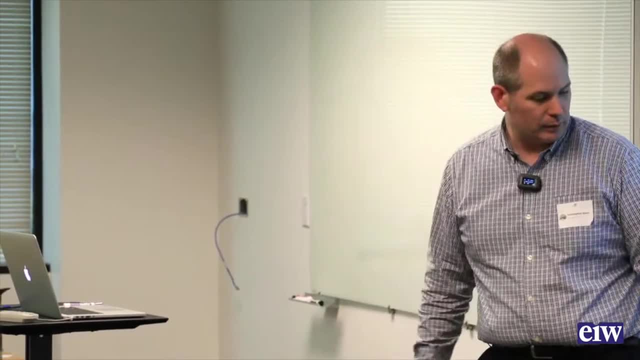 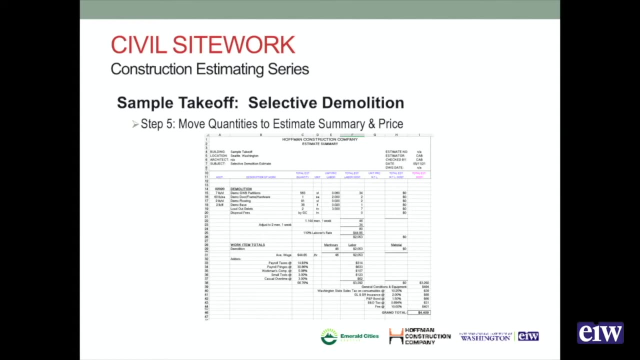 put on my labor adders, which we'll talk about later on in the project. but that's your tax, your fringe allowances for small tools, any kind of overtime allowances. sum that up and then put on your markups as far as your tax on your materials. 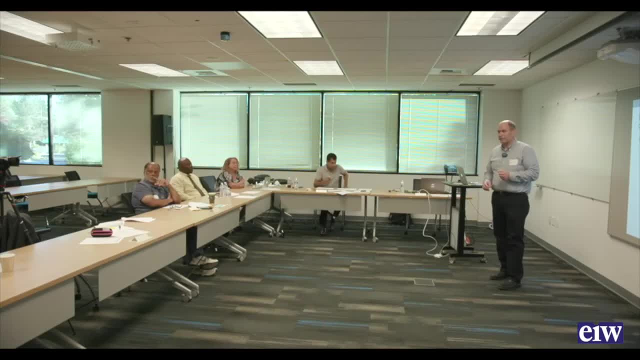 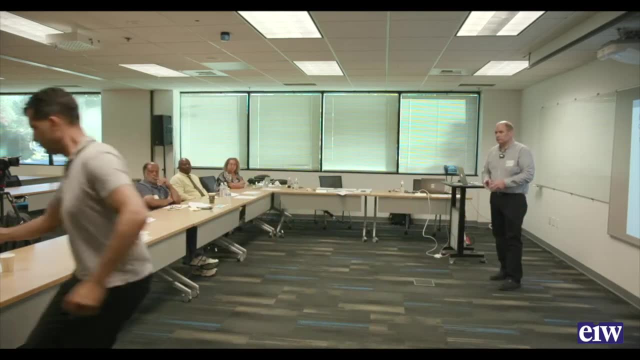 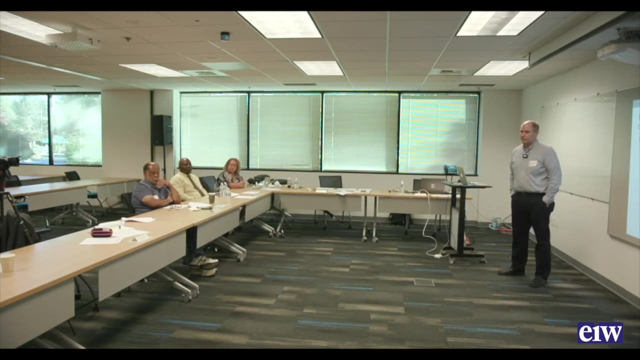 yes, and you're rounding up to 80. I mean, I guess what I'm asking is like: ultimately, how do you manage price when there's things that come up that you didn't expect? sounds like you're pretty thorough, but sometimes that stuff comes up you just take a hit on profit. 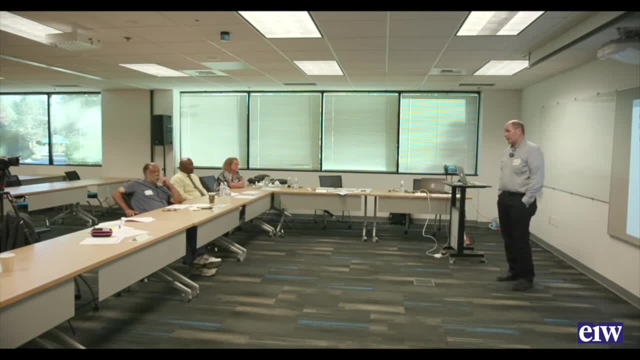 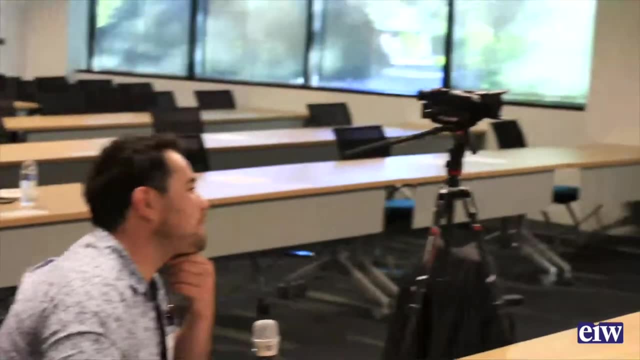 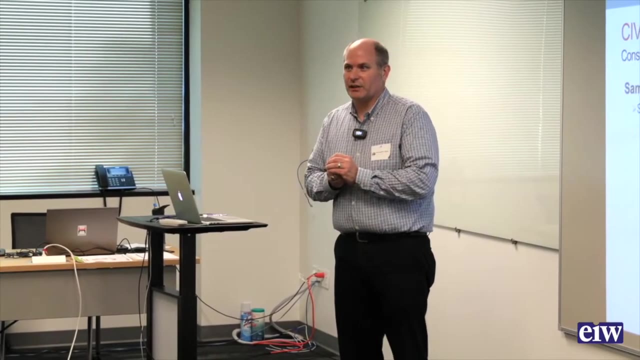 or do you basically? well, that ends up getting right down to a business decision, and so that's where you get beyond the science of estimating, get into the art of estimating. so, yes, I look at the project and if there's added risk there, I can do a couple different things I might. 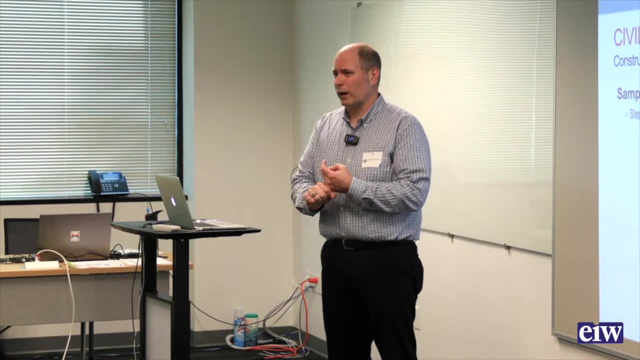 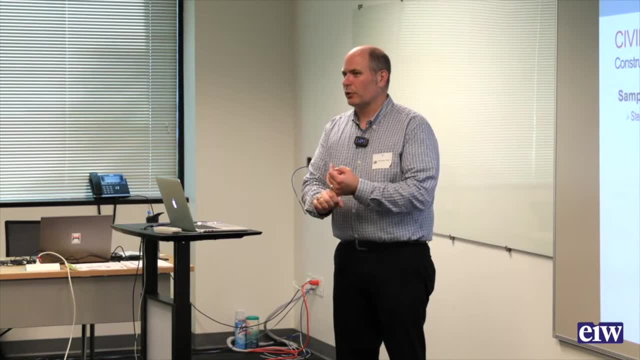 put in a few more hours, because I think I might need a few more hours here, because this is, I think I can do it for this, but I'm not confident enough in it and I don't think. and then I've got, or I might put in a little bit of. just a straight dollars for contingency in it, or I might increase my fee for it, because if there's more risk there might be more need to be more reward. at the end of the day. that all has to be weighed against if I'm bidding a job with. 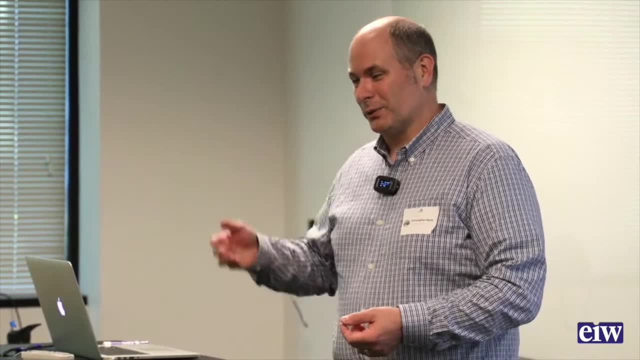 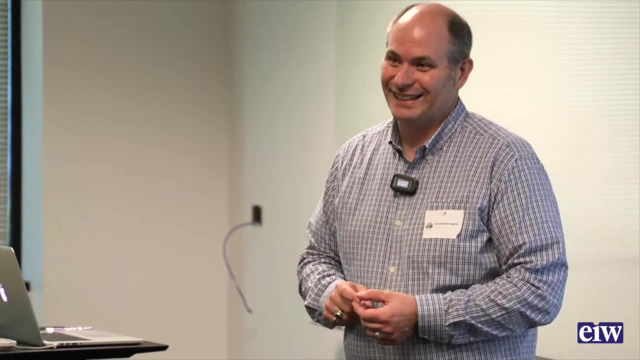 every dollar that I put in to that job to mitigate risk, maybe one more dollar that's going to push me over the top of the low bidder. I mean at that level where you guys are at Hoffman right, do you guys is? it sounds like it's an. 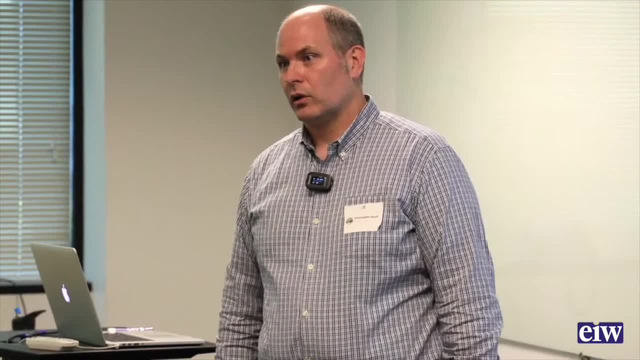 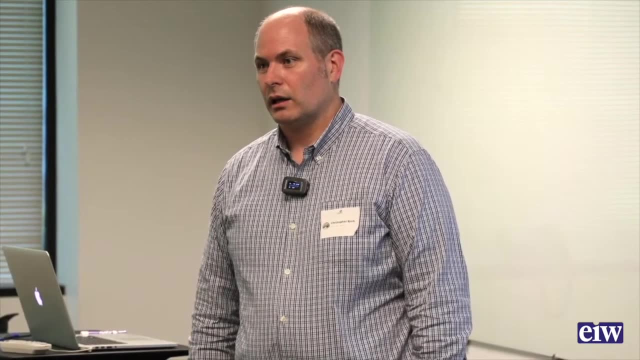 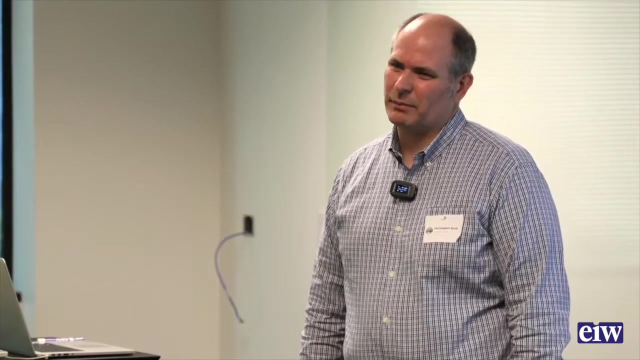 per estimator kind of decision is there like a sort of standardized way to manage risk as a factor 1.2 on just about everything, or 1.1, you know, I've seen some of that in the past. I don't subscribe to that theory because I think that 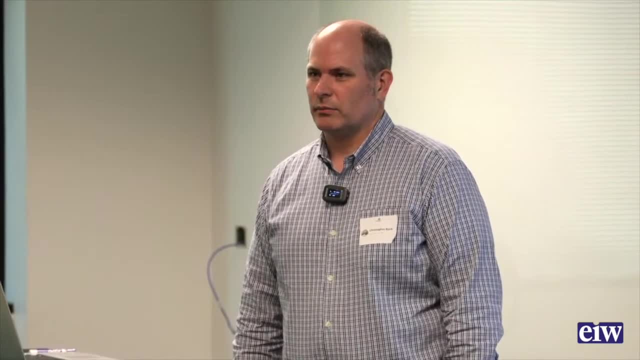 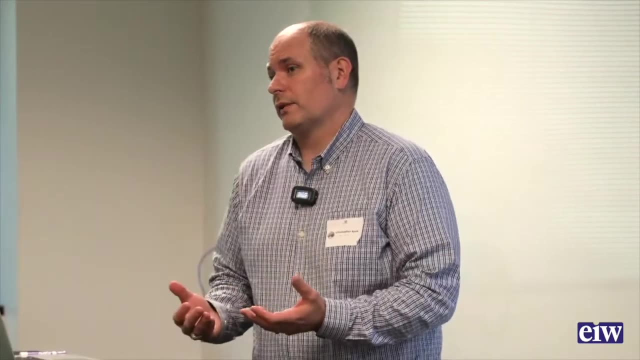 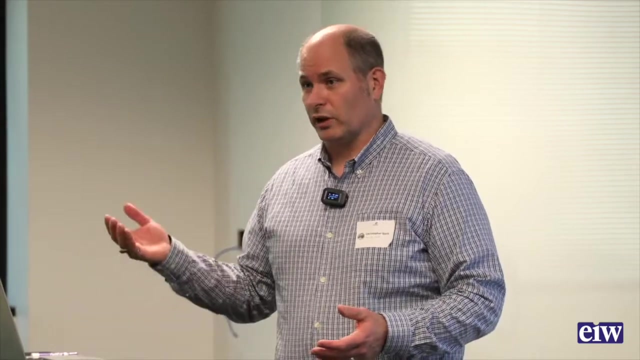 risk is a business decision, and so what you want to do, though, is you want to review, so what we will do often times is: I'll send out my estimate and I'll review it with the- maybe the junior- estimator who's done the quantities or has done some of the pricing. 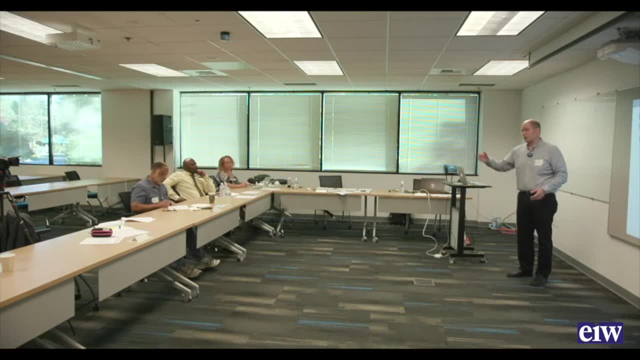 for it and I'll review that. I'll have an executive look at it, I'll have the project manager look at it. sometimes I'll even bring the superintendent in and have them look at it as well, because they might look at the man at the hours and say: 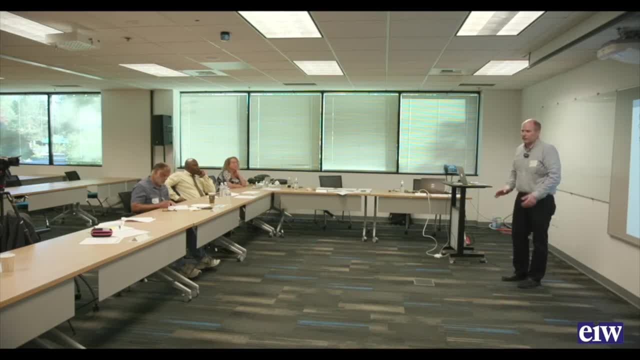 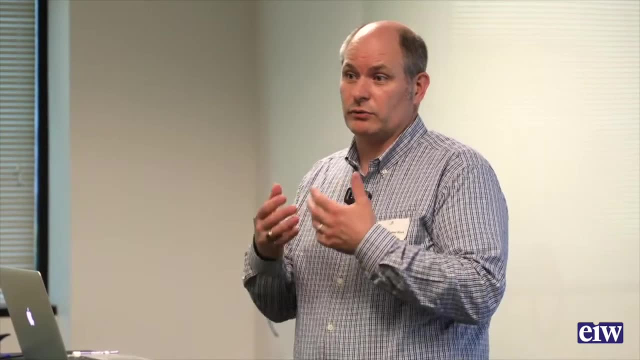 you're way off, you're in left field. it's going to take you twice as much as that, and so I need to know that, because if the superintendent, who's out there going to be running the work, thinks that it's going to take twice as many hours as what I've estimated, 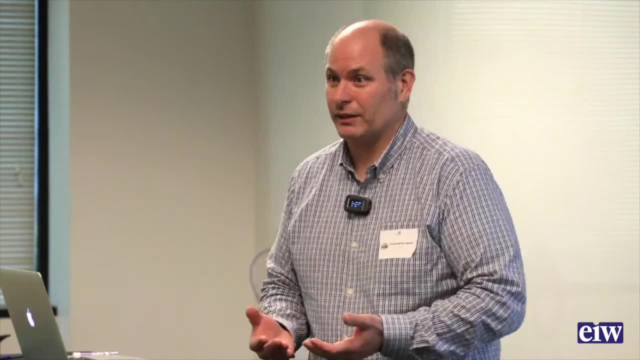 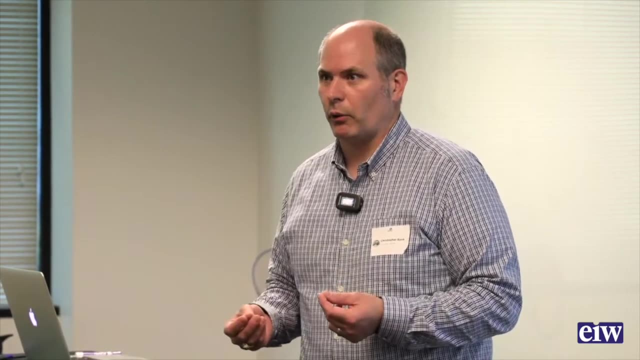 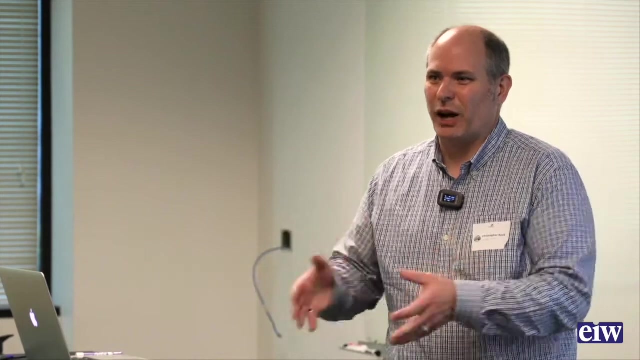 and I'm looking at historical data on what we've actually done. I need to know why he or she thinks that, because it's an important knowledge on making sure that we've got the right number. but so that's what I say, and I think every job is different. 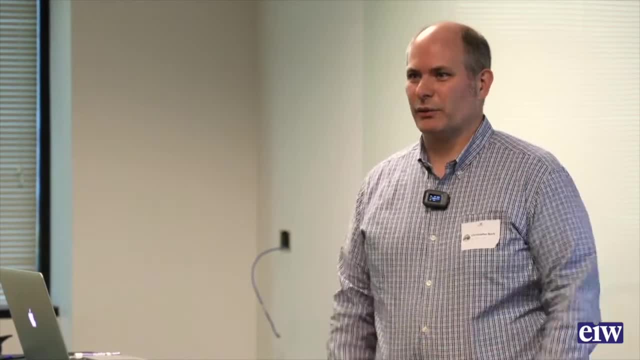 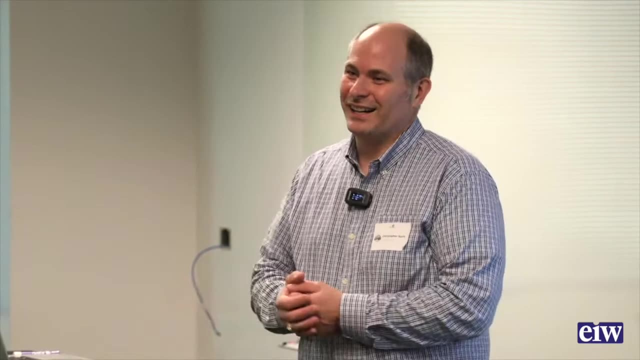 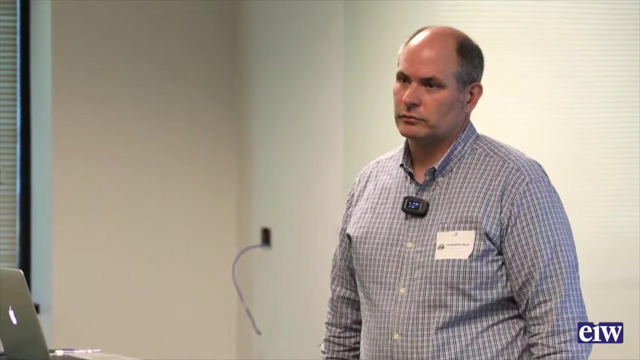 some jobs have a high degree of risk. you know you take the space, needle renovations. high degree of risk, well, even beyond risk, just like unforeseen, like okay, you forgot the. what do you call the wall? the footers on the wall account for that. you know, did that ever occur? 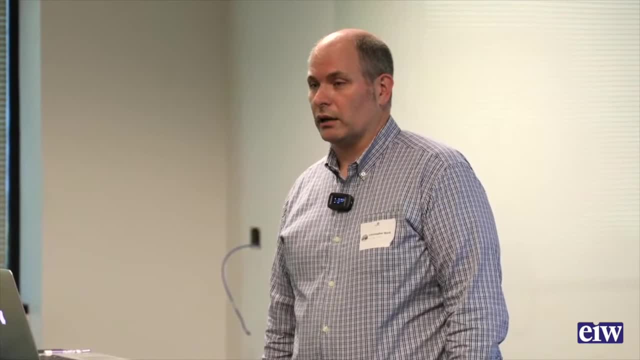 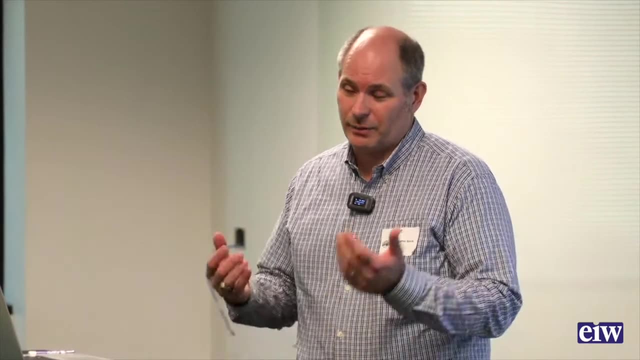 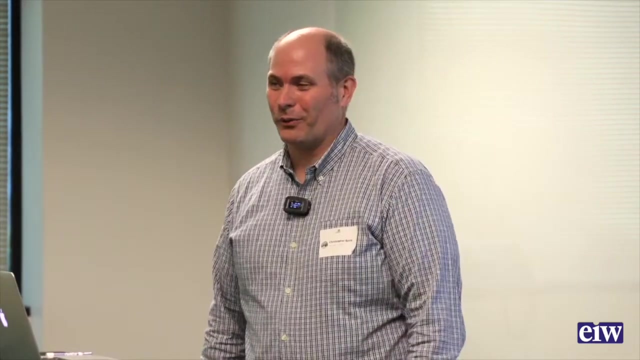 for you guys where you guys just yeah, oh yeah, you guys just take a hit to profit on it. yeah, well, that. and yeah, if it's something that's shown on the drawings and you just missed it, yeah, it's a hit on profit, but hopefully you know. 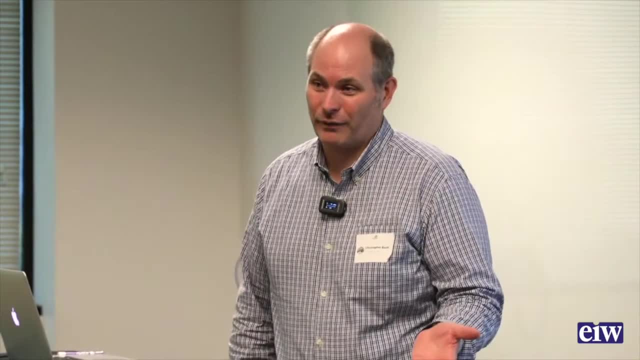 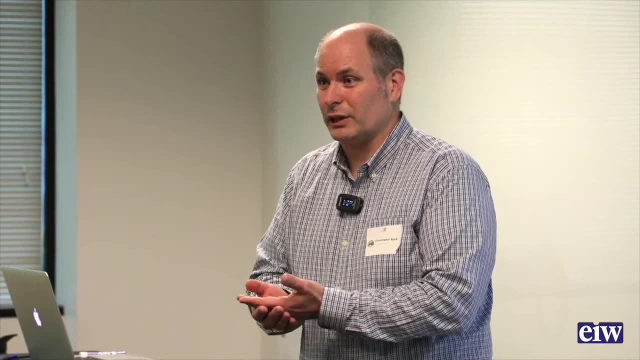 oftentimes what I've found is that sometimes those things that happen that are hits on profits, you might have other areas where you have gains on profit and so they can, so they'll equal them out. you know an example of that might be. you know, as a general contractor I may put together an estimate. 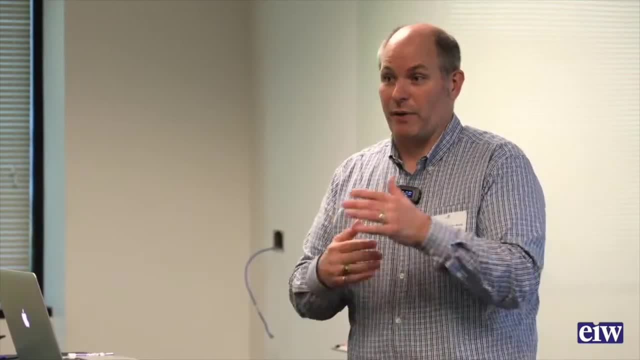 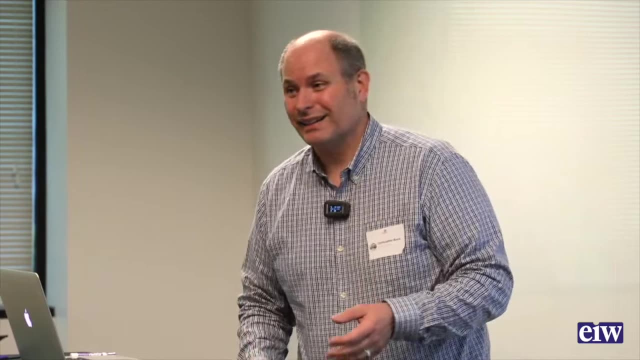 and I've got different bid packages and scopes of work, but I don't have actual bids yet, so it's an estimate. so I, when I go in, I expect some of those bids to come in over my estimate and I expect some of those bids to come in under my estimate. 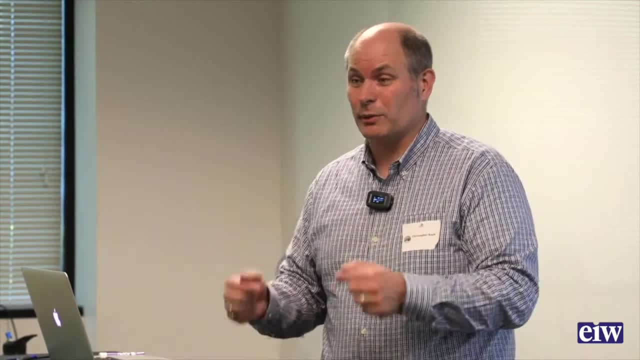 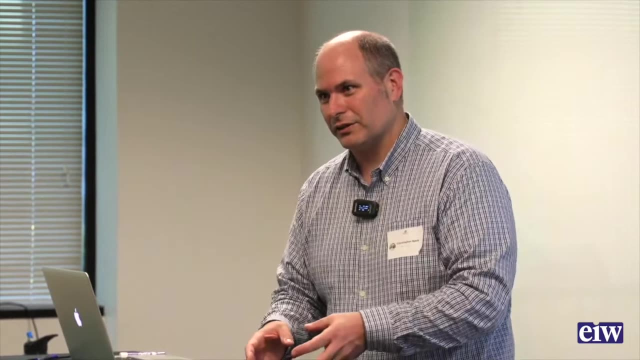 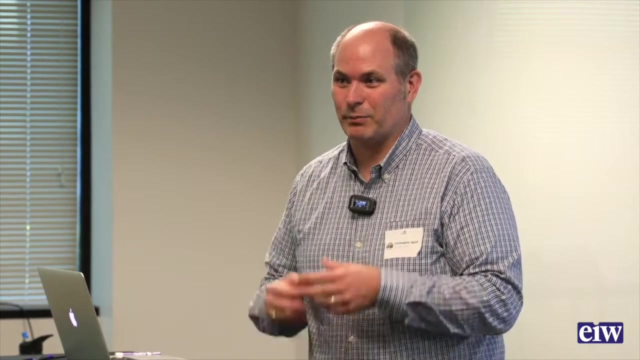 but I know that overall that on that project it should come in really close to my estimate. so just when you translate that into a more detailed work- and I understand this because in previous things that I've done with the company I've actually been the project manager for our 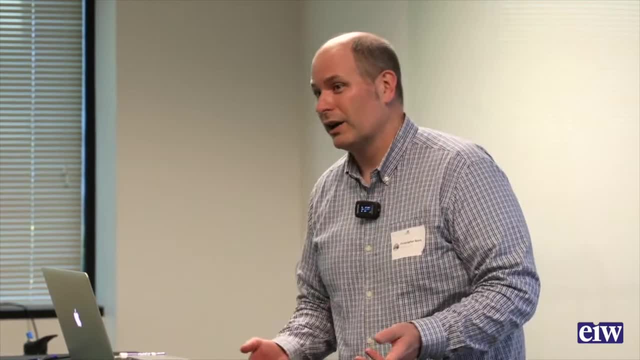 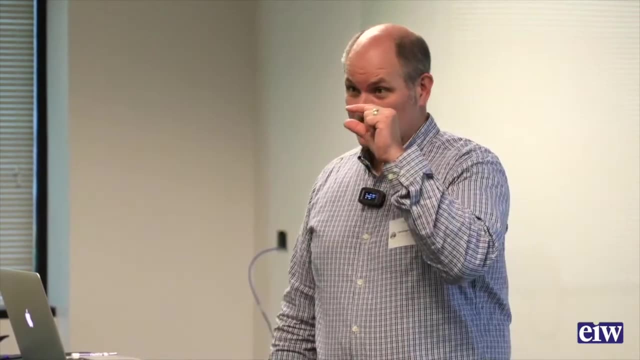 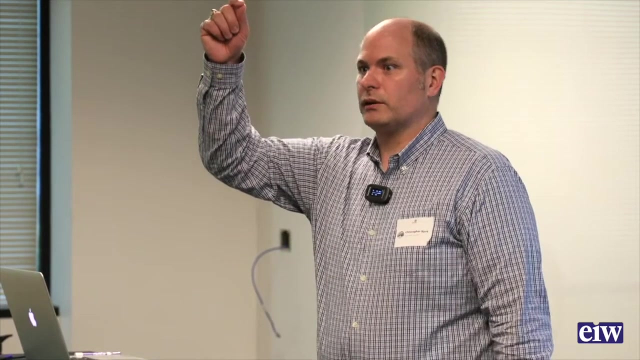 subsidiary that does the concrete work, self-performed concrete work on semiconductor plants. so I've looked at those details where we were looking at a detailed minutia of estimates and cost codes that we're tracking our costs on, and some of them are going to be we're going to have 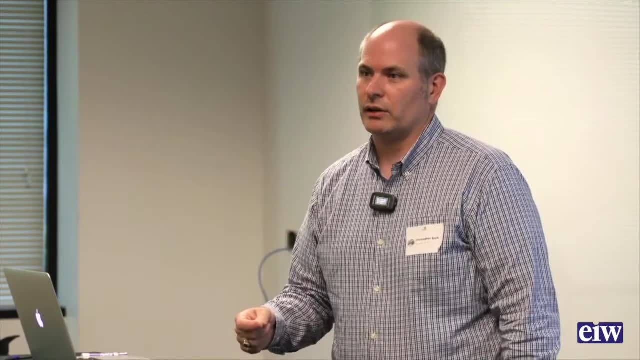 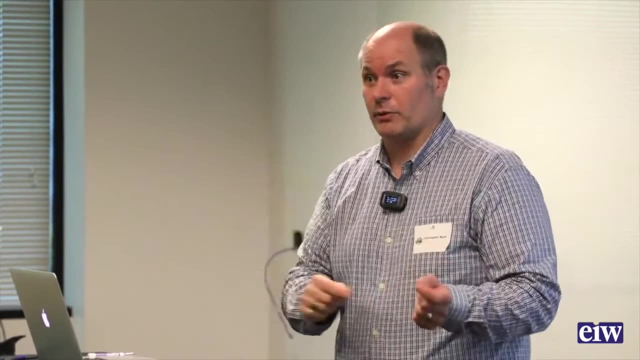 exceed our hours on some of them. we're going to beat our hours on, but ultimately I'm looking at where those are, because if they're large numbers, I want to know why. I'm trying to make sure that my estimates are better next time, but I'm also going to be 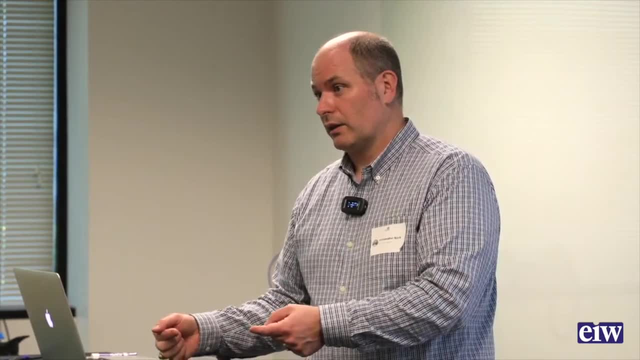 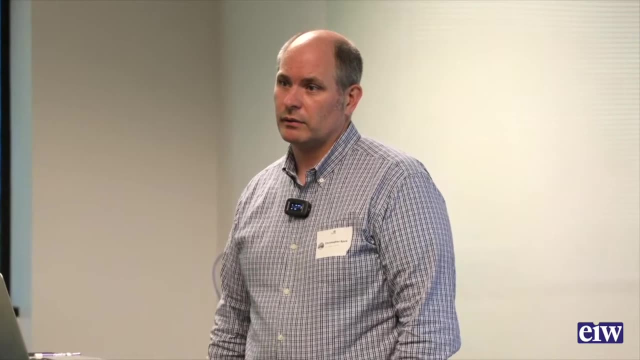 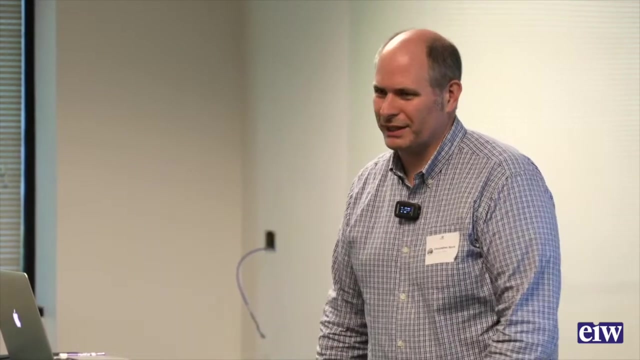 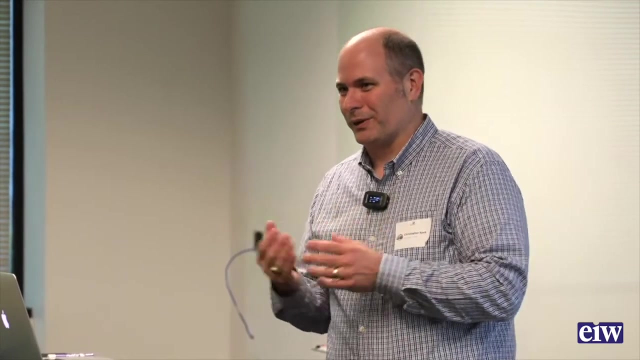 looking at that bottom line to make sure that that bottom line is evening out and we're still tracking where we need to track. you know one thing I will say about being an estimator, and this is a quote that former head of Hoffman said about one of our head estimators. 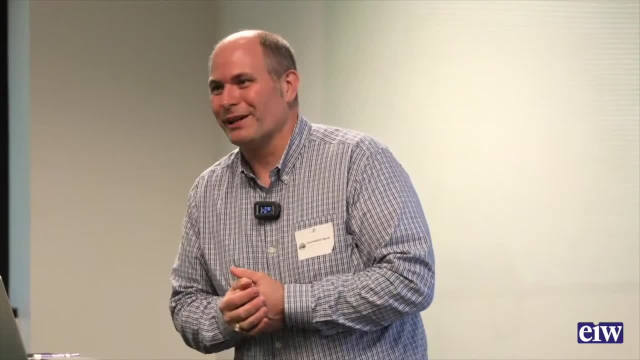 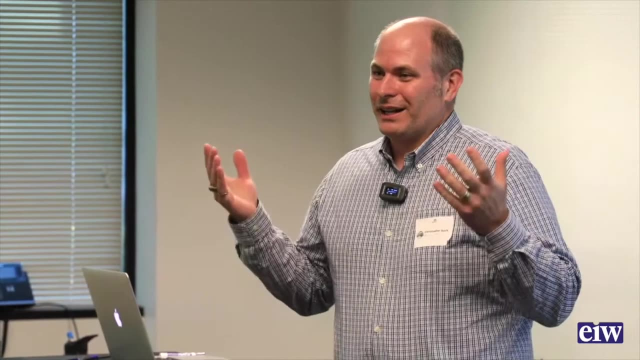 I don't understand why anyone would want to be an estimator, because we're never right. we're either too high or too low, and that's it goes with the territory that you have to understand that what you're doing. we may have a better knowledge of what things are going to cost. 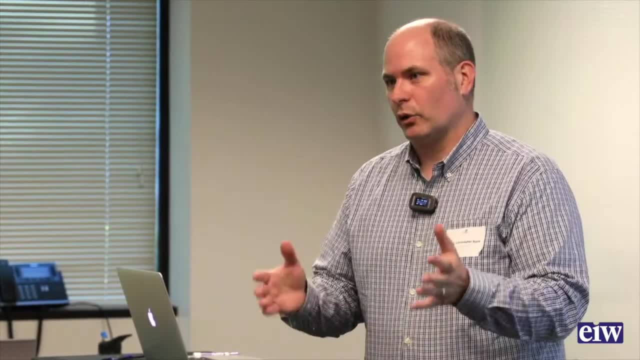 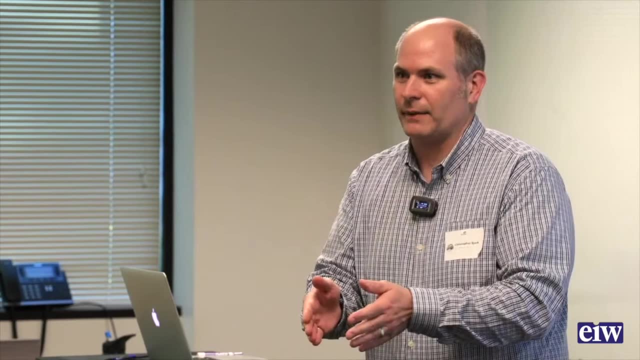 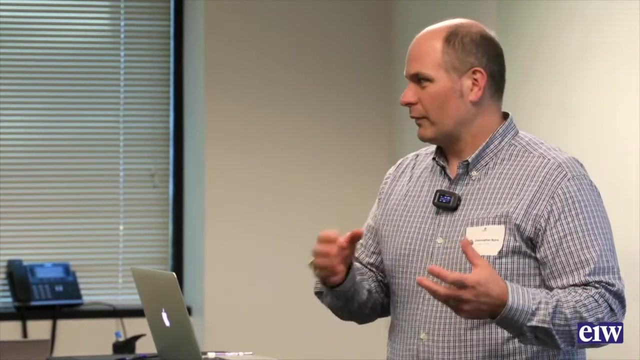 but we're still estimating and so what we are trying to do is to get that number as close to the number that we think is right that we can. and then we think and use that art of estimating the experience to, you know, cover some of that other. 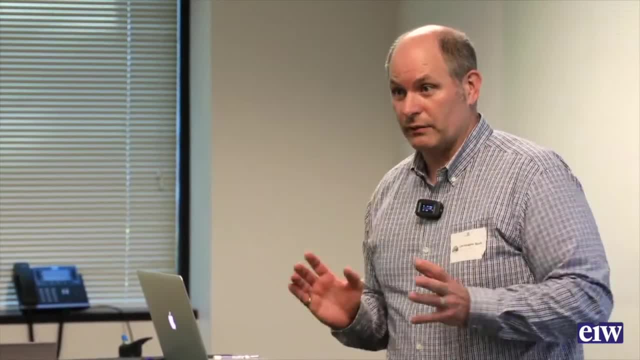 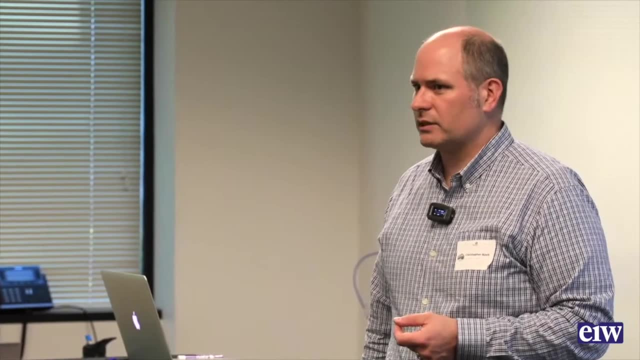 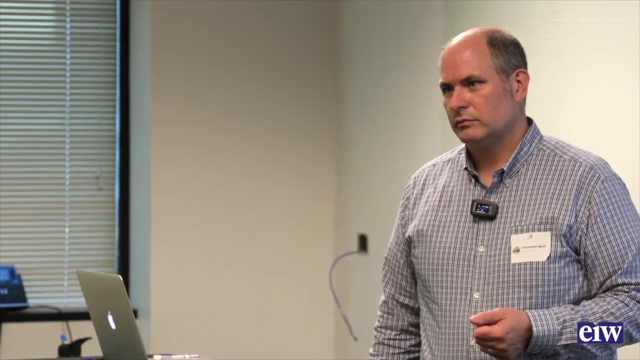 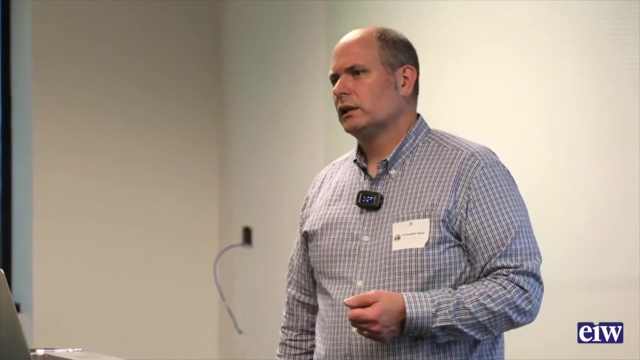 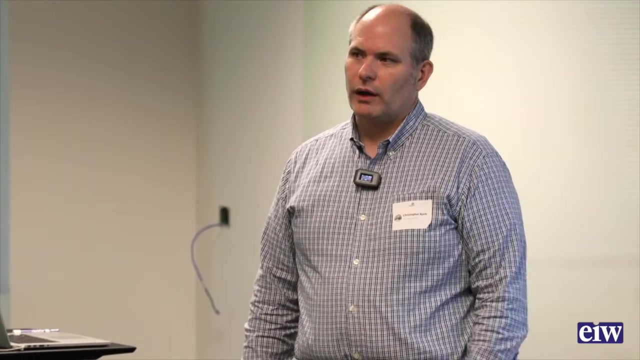 those risk factors to make sure that the company feels comfortable with where that estimate is at. yeah, there's some consensus involved in any kind of risk mitigation, or you might want to like cut a little of what you can just to secure. well, that's always a business decision that you get. 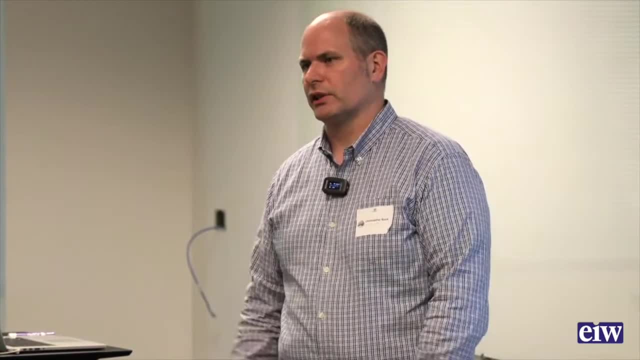 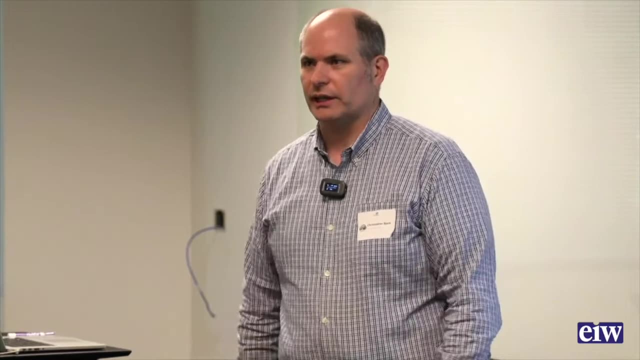 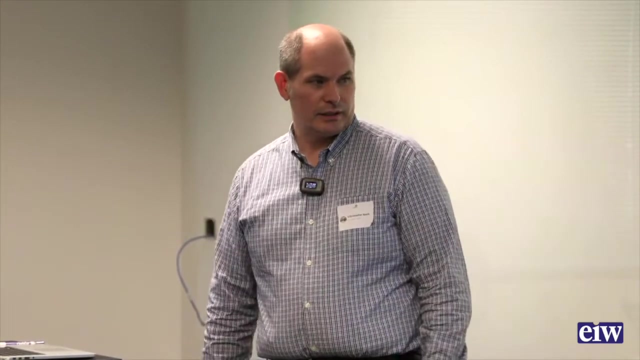 into when you go after a project. you know when you put your fee percentage on, what your fee percentage is is what you're willing to do the work for, for the risk that you're taking. we got people online too, Ryan. all good questions and I think you know part of what I wanted. 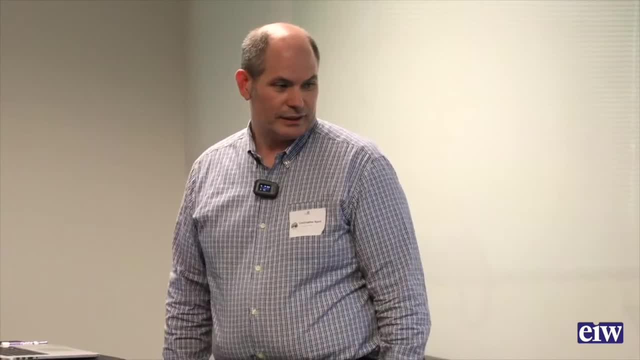 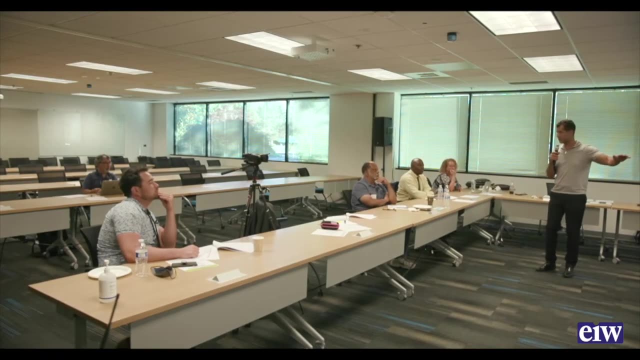 to address before we moved on to the next slide- and I was going to actually put Shelton on the spot right here, and you know what we were talking about- is you know? it's one thing to say. it's going to take a certain amount of time to do. 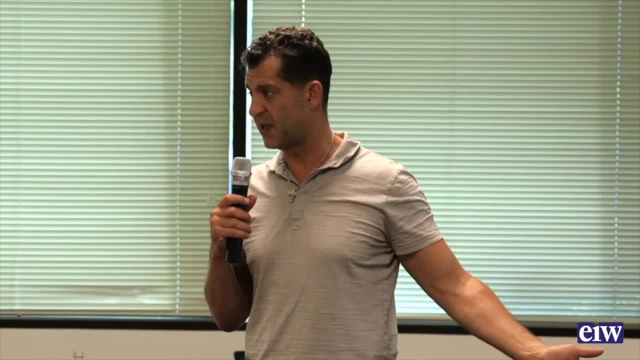 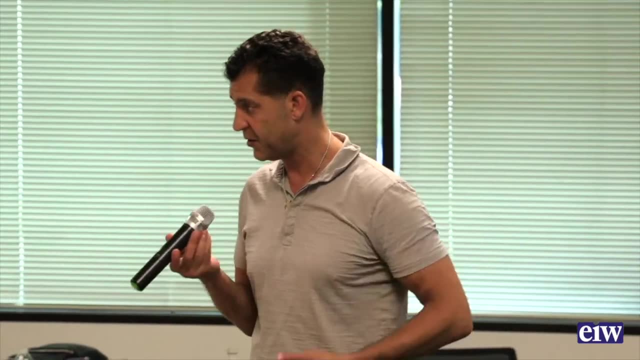 something. but then there's impacts that impact productivity and I just kind of wanted to get a just a quick comment on things that impact productivity in your line of work that could impact the labor rate. one of the things that definitely is an impact is who you're. 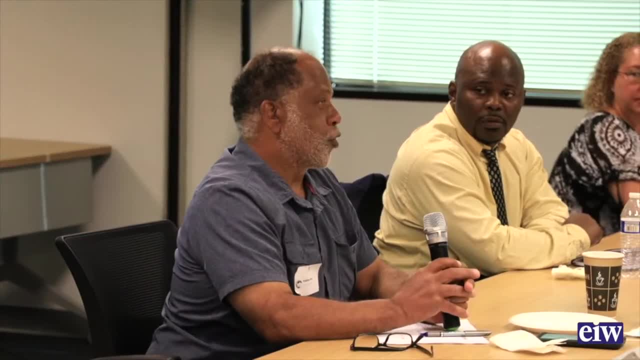 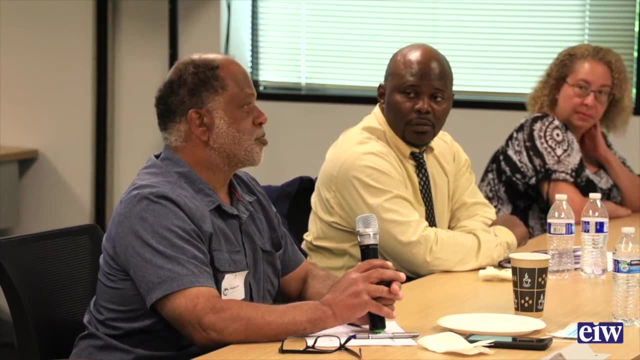 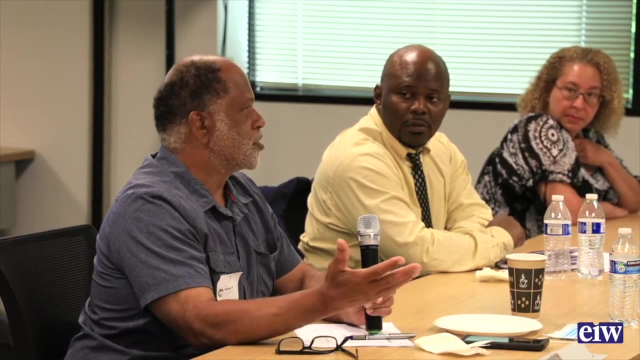 working for. be very, very careful who you're working for and you know how they run their projects. some general contractors you can do very well on and others you're going to lose your shorts because they're not organized or the state trades are stacked or the way the job flows. just 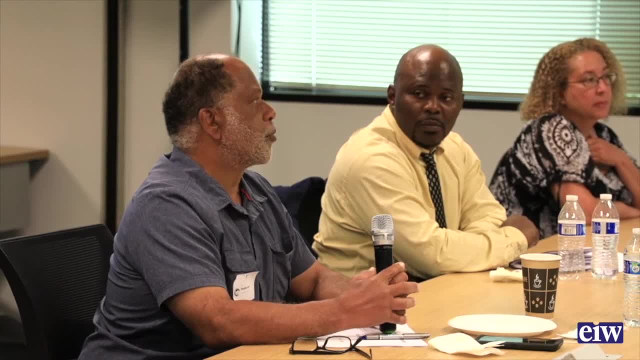 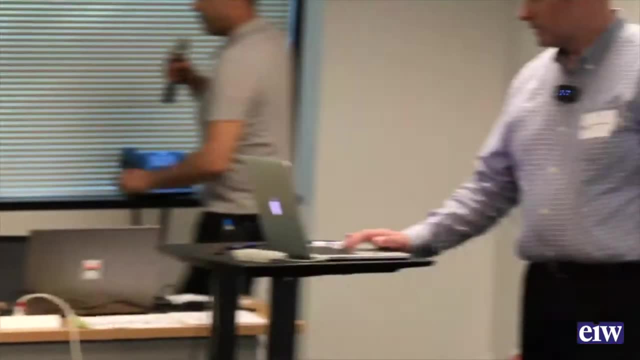 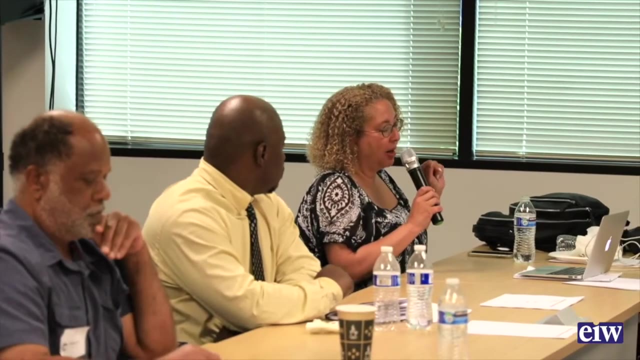 doesn't allow you to make money, so just knowing who you're working with is very important. go ahead, and then we're going to have some comments online, and so if there are some questions, please let us know as they come. excuse me, everyone online now would be a really good time for. 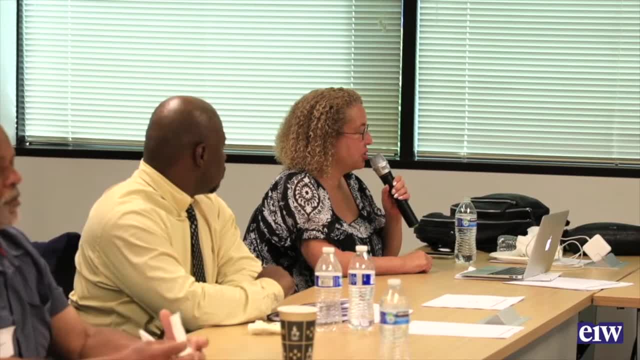 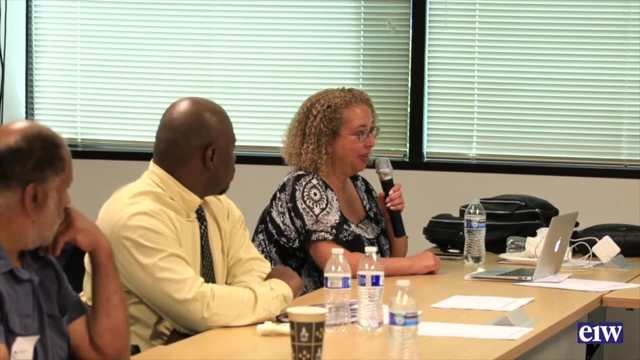 you to go to the Q&A tool and put in some questions. there are no questions open in the Q&A tool and now that we seem to have the sound and pictures moving together and we are in this take off, would you please put any questions that you have into the? 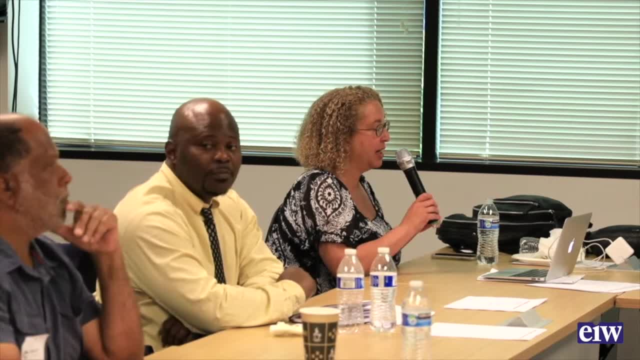 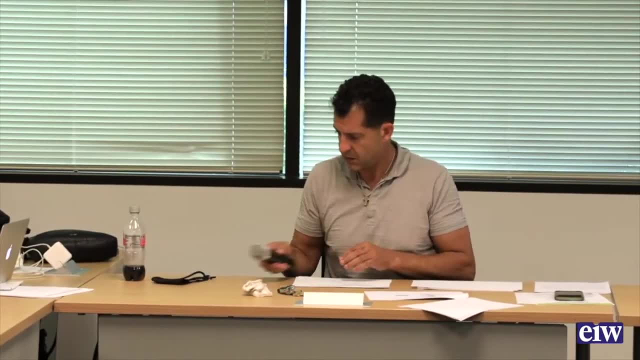 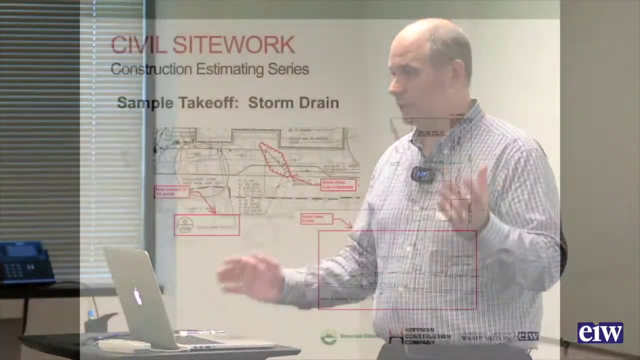 Q&A tool that you'll find on your pop up bar at the bottom of your screen and we will get to them. ask your questions now. thank you, okay, so we'll get through. go through this a little bit quicker here. storm drain, so storm drain. we talked about lineal foot of. 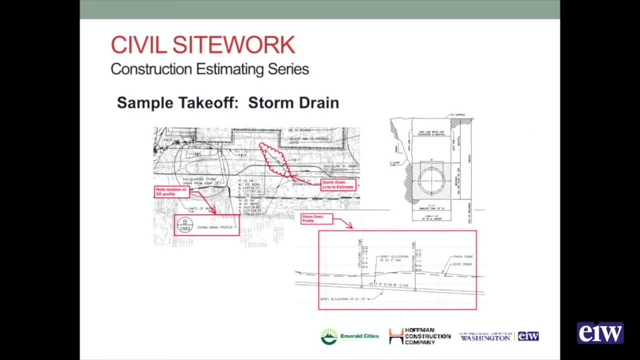 pipe. so you've got a plan view, you've got a profile. now, when you're looking at profiles and you're looking if you're going to scale something off of a profile, you need to understand that most profiles have a different vertical scale from the horizontal scale. 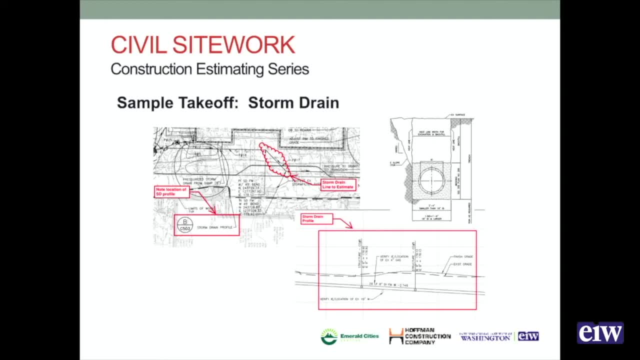 so, and that's just in order to make things look more cleaner on the in the profile. but the profiles also usually tell you what lineal footage is to actually use, so that's really nice. so this, this storm drain. we're looking at this section from here to here it says 29 lineal feet. 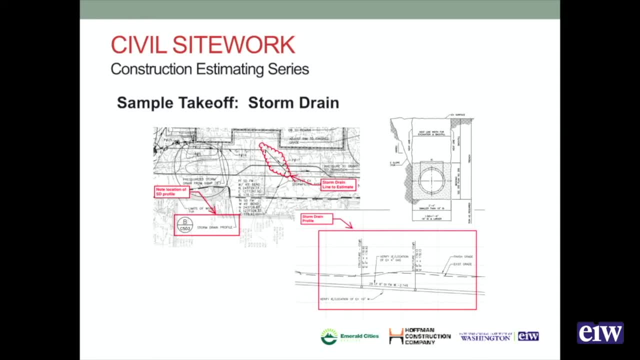 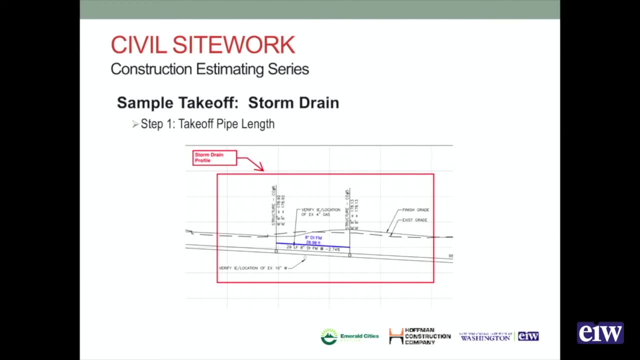 we've also got a trench section right there on what this trench needs to look like. so taking off the 8 inch ductile iron force main and force main just means that it's a pumped storm drain. so instead of water this flowing downhill, it's flowing. 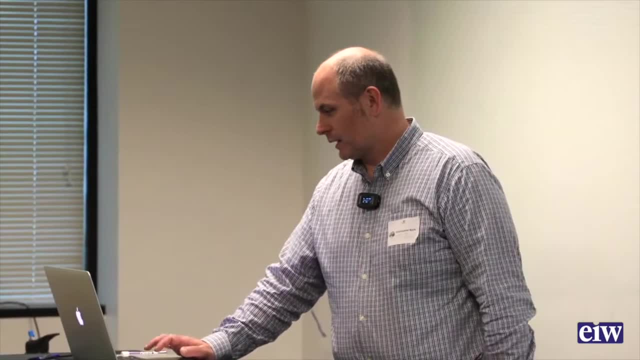 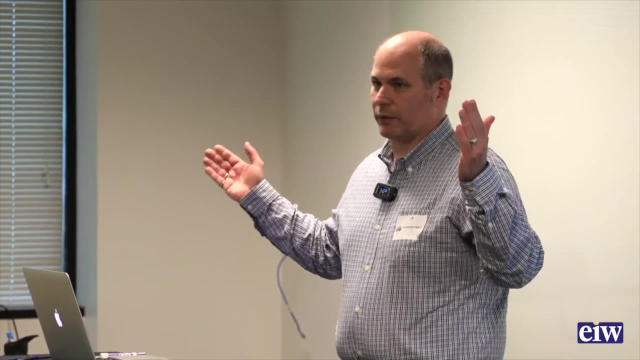 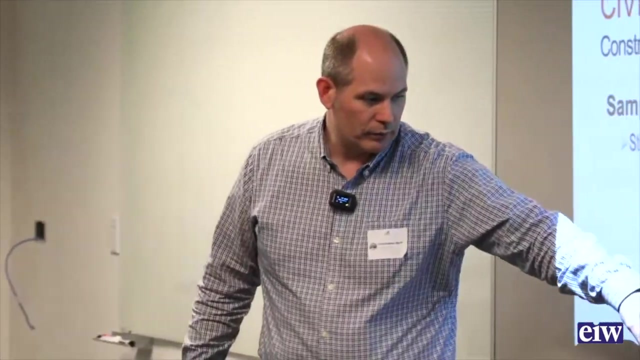 uphill because it needs to go uphill to get to where it needs to go. then we need to get our information from the trenching thing. so we have two points. they're both going to have different starting elevations and elevations and existing elevations. so if we look at the first point, we compute it out, it's a depth of 3.92 feet, the other side's 5.21 feet, taking those averages, and then we also know that the bedding depth from the dimensions is going to: that's going to be a foot and a half. 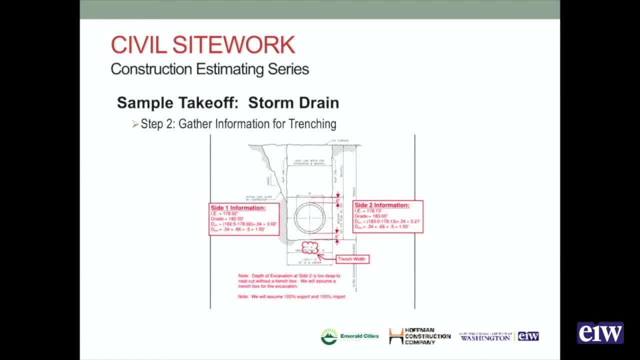 those are key information, but what we also need to know is that at 5 feet, we cannot just let the soil stand straight up, so we would need to either side slope it or use a trench box for this exercise. I'm going to say: we're going to use a trench box. 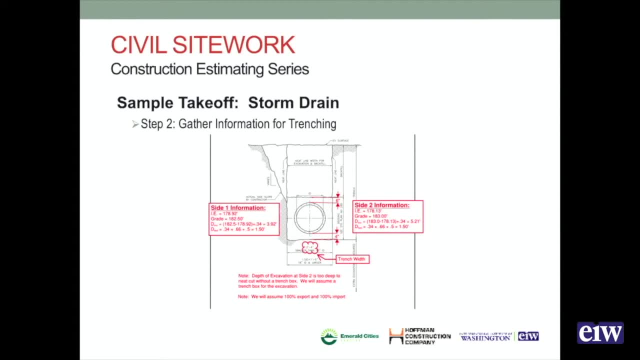 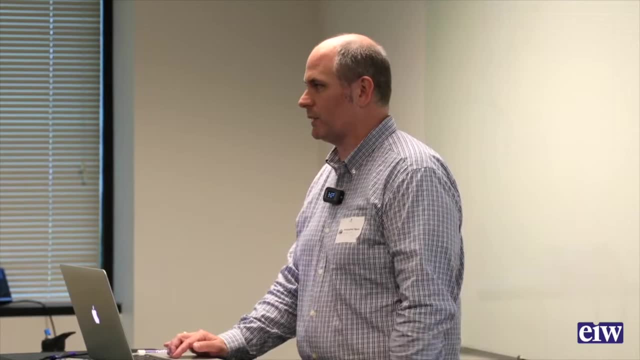 just so that you kind of see how that all puts together. we will also assume 100% export and 100% import, so everything we dig out has to go off site and everything that comes back in we need to bring pay to bring it back in. 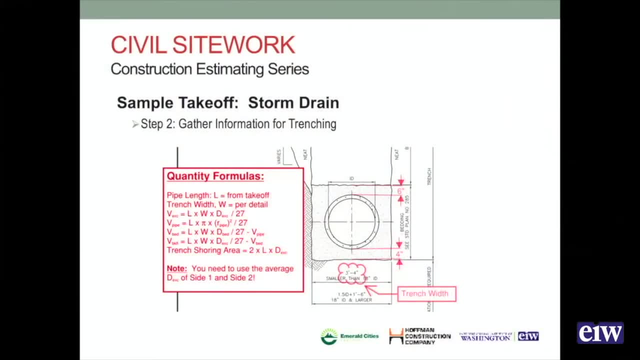 so quantity formulas: your pipe length, you need to know it's the length from your take off. the trench width is, per your detail, 3 foot 4 inches. the volume of excavation is going to be that overall length, average length times the average depth. so average one. 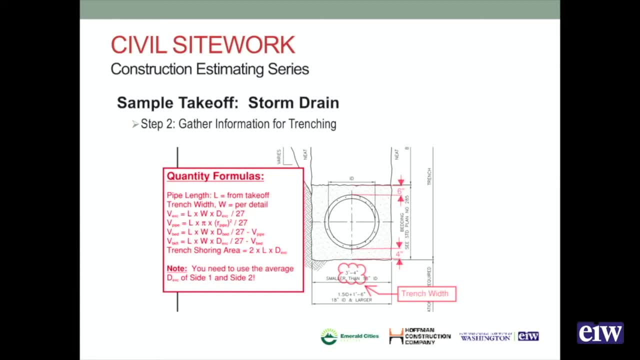 side and the other side. so the 3.92 and the 5.21. average those together and figure out what that depth is. I believe it's about 4.57 feet. and there's your depth. you've got a width, you've got length. 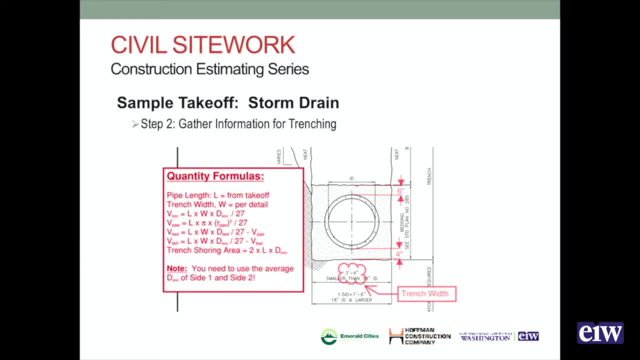 times width, times depth. you've got a volume. then we need to compute the bedding. so that's what's going back in. so the bedding, we know that it's 3 foot 4 wide times the length, times a foot and a half deep, less the volume of that pipe. 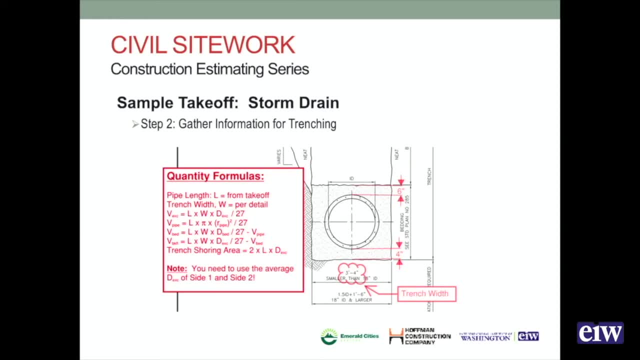 so we need to compute the volume of the pipe, which is the length of it times the cross sectional area of it. that's pi r squared, so it's an 8 inch pipe. radius is 4 inches, so pi is 3.14. compute that all together. 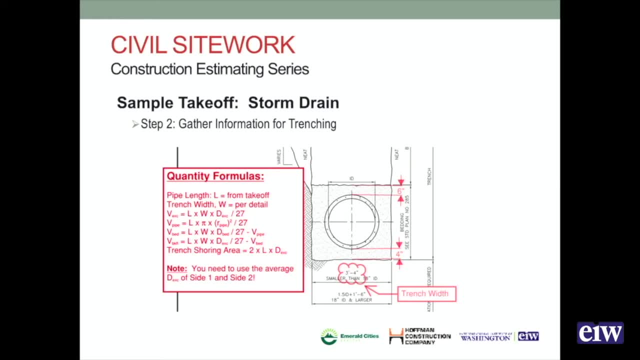 and you get a really small number, because an 8 inch pipe isn't, isn't very large, but then the volume of the backfill is going to be the volume of excavation, what you took out less what you put back in, so it's the volume of the backfill. plus the volume of the pipe, because remember for your volume of your backfill you took out what the volume of the pipe was, so you need to add that back in when you compute the rest of the backfill. for that your trench shoring, so your trench box is going to. 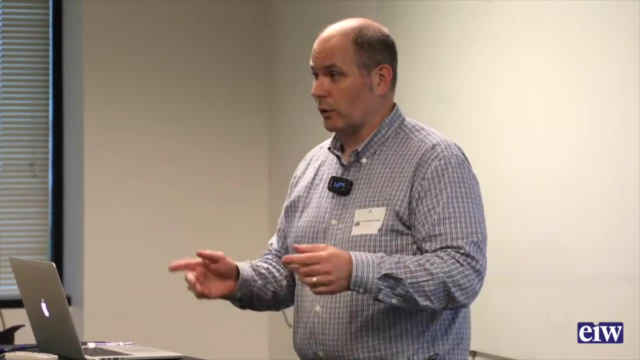 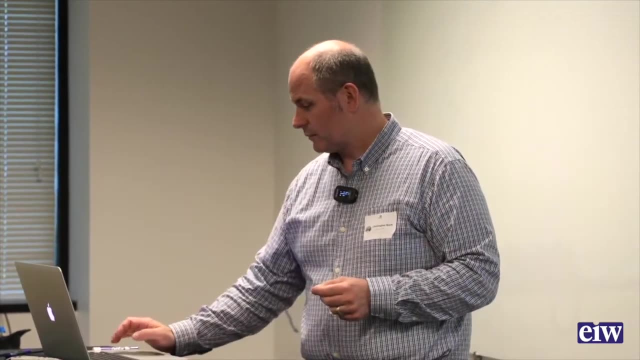 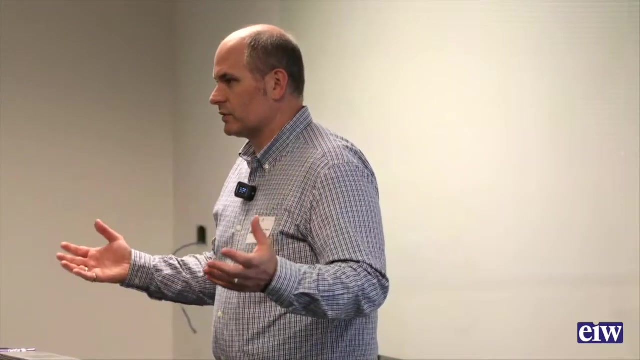 be a square footage of shored area. so it's the length of the excavation times, the average depth times 2, because you'll have it on both sides. so here's an excel spreadsheet that I've worked at to compute all this stuff up, all those formulas I just talked about. 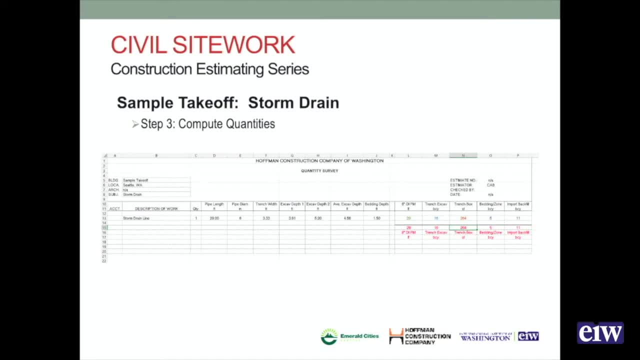 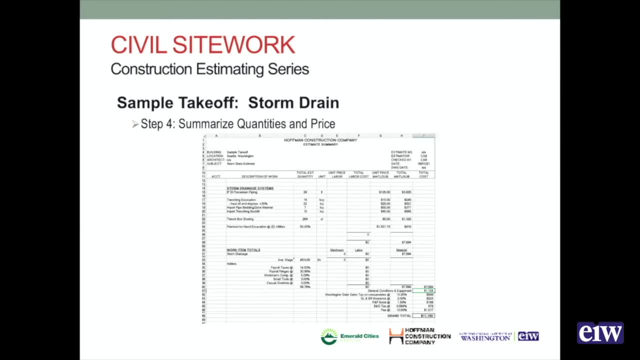 are inside those computations to make sure that you are computing things right, and it gives you the quantities that you need to know to price out the work. you price out the work. you've got the force main: 29 lineal feet times 125 dollars a lineal foot. 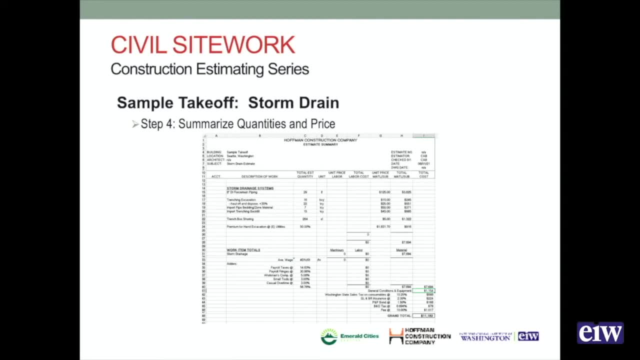 then we've got the trenching excavation and we figured your bank yards for the excavation. we figured converted that to truck yards adding 35% for the haul off of that excavated material. then we figured importing on the bedding and the trenching, the general trenching backfill. 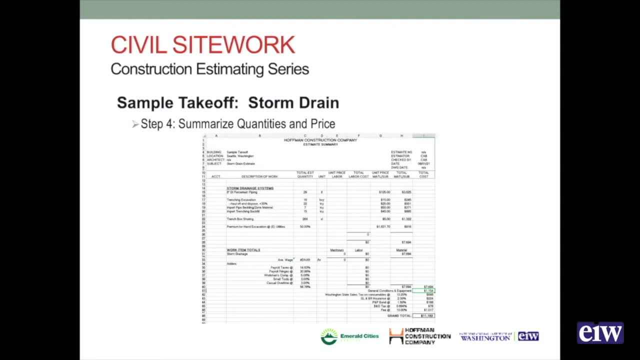 and it figured those at truck yards as well. so the neat volume that we did times the 35% and then we added in 5 dollars a square foot for the trench box shoring to get us a number. but one thing, if you go back on 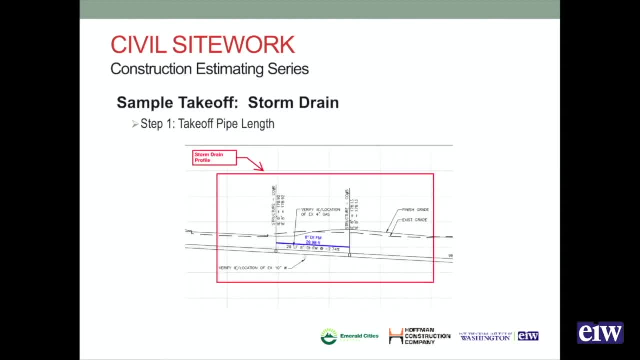 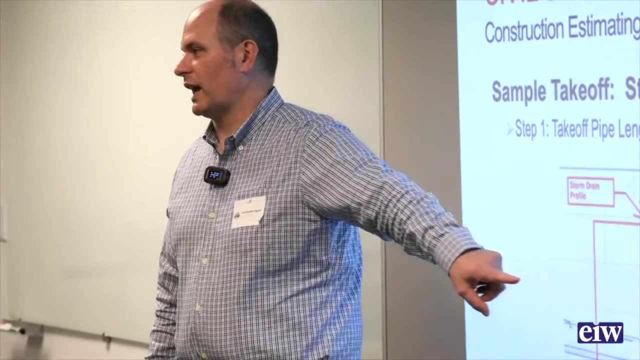 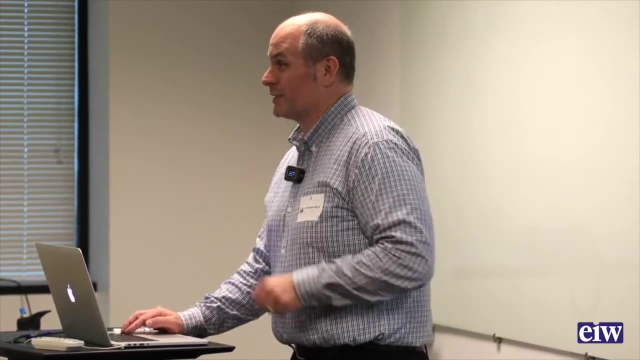 the drawings on this section cut right here. there's a note here. it says: verify invert elevation location of existing 4 inch gas line. that's a note that you need to know, because if you've got a 4 inch gas line, you're not using a piece of. machinery to excavate in that area, because you don't want to hit that gas line, and a 4 inch gas line is a larger gas line. so we've added what I've done here is I've added a premium of 50% of the cost. 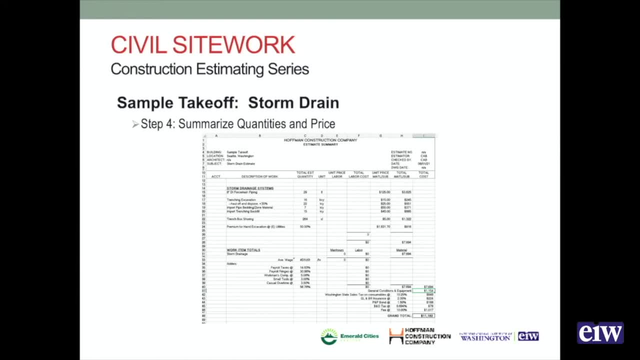 of excavation to account for where I'm going to need to hand excavate. so I'll save some money because I can have the backhoe going off and working someplace else, but the labor to excavate that is going to be less productive when I have a. 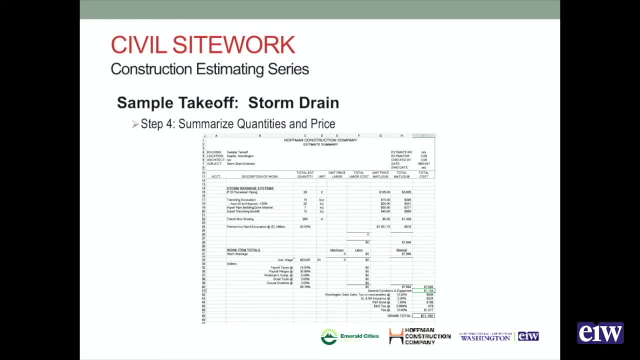 worker in there with a shovel. you take that. I've priced this out as if I'm subcontracting the work. so these are subcontracted numbers put on markups as far as my taxes, my fees, my insurance requirements, how I'm going to staff to manage the project. 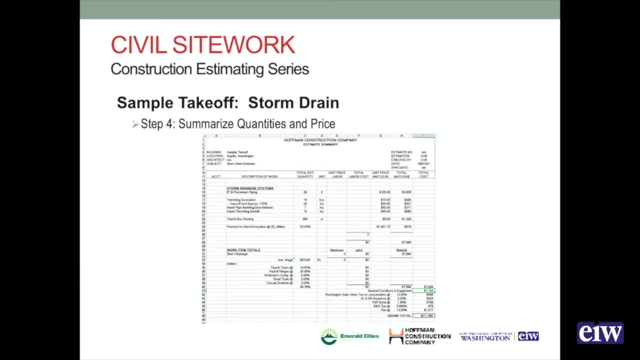 and we have a overall price of about $11,000 unit prices that you have for this sample. are they fairly current? they're in the right range of current. I mean, in this market right now, current is can be a little bit of a guessing game, depending on what. 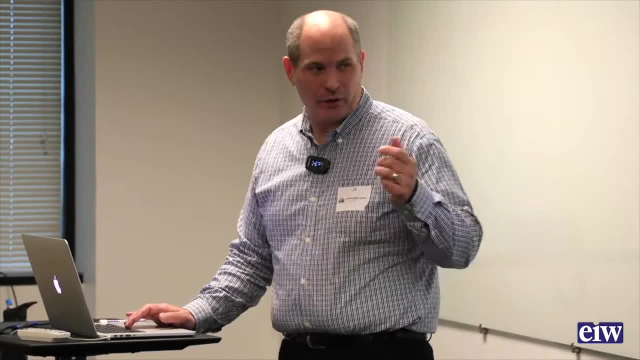 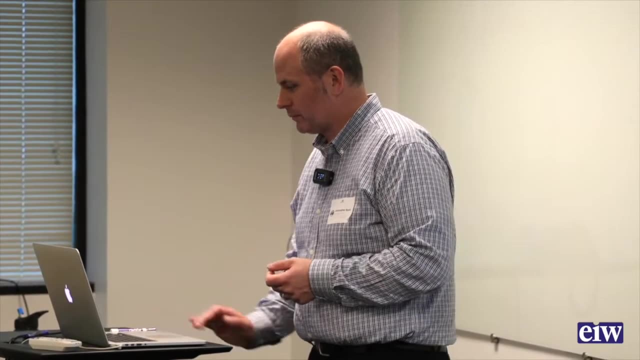 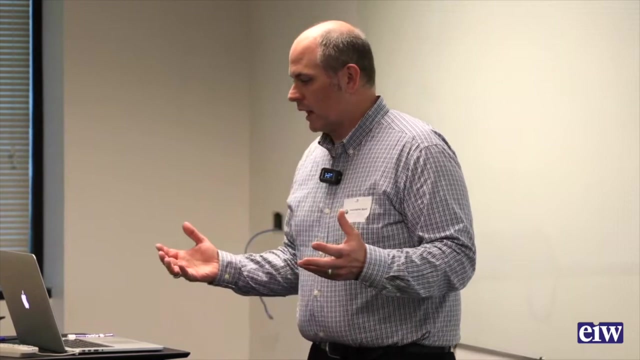 material you're talking about, but yeah, I've used some past projects that I've worked on and made sure that the units are fairly close. last thing we're going to talk about is asphalt paving. asphalt paving: we're going to look at an area. this is off of our Wazoo Tri-Cities job. 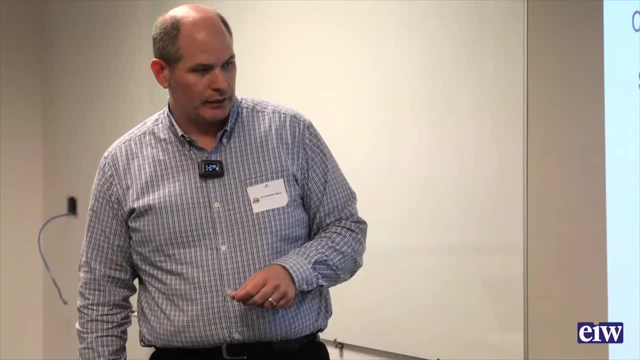 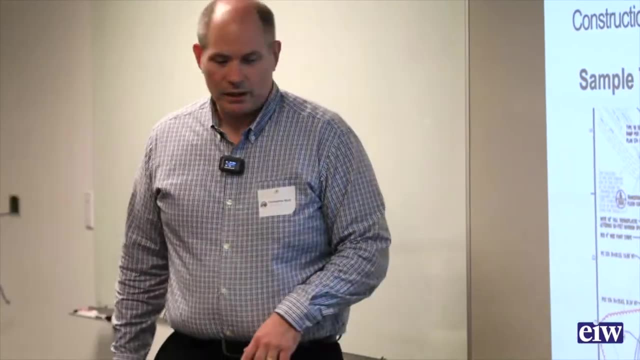 we've got a service lane that comes in, with a big turn around at the end of it. so we've got our paving section right through here. we've got our what that section looks like so we can go through and we can take off the asphalt paving. 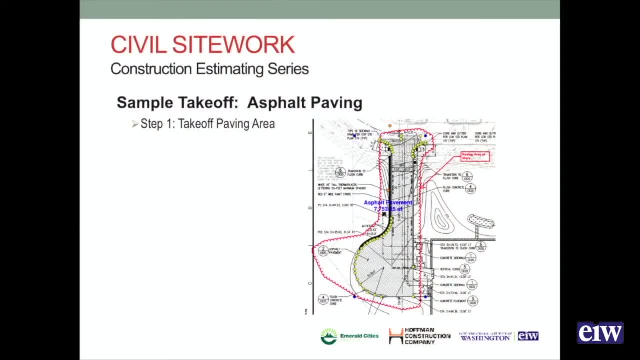 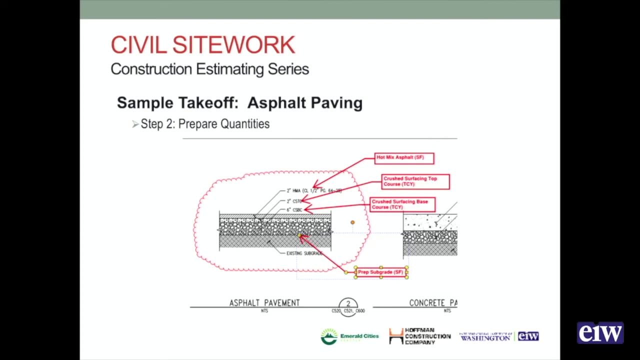 area about 70, a little over 7,000 square feet. we're not worrying about the curb, so we're just looking at the asphalt here. but what we do need to know is what that section is. what does that area get us? and that gets us. 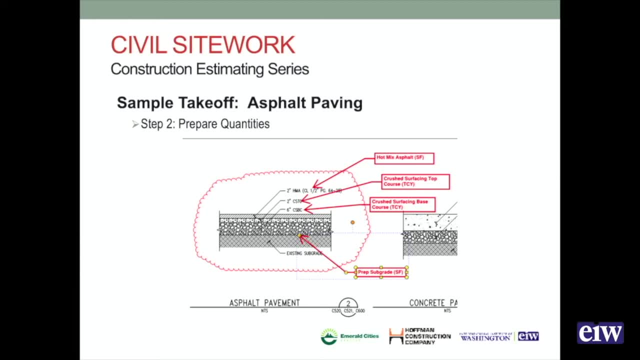 2 inches of hot mix asphalt. it gets us 2 inches of the top course, which we need to price that out in cubic yards. it also gets the 6 inches of the base course which we need to also need to price out in cubic yards and we also need to prep that subgrade. 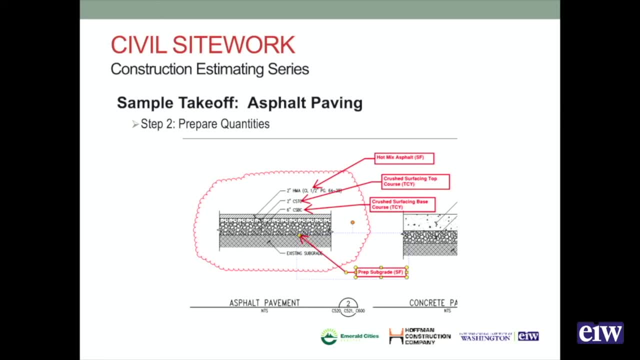 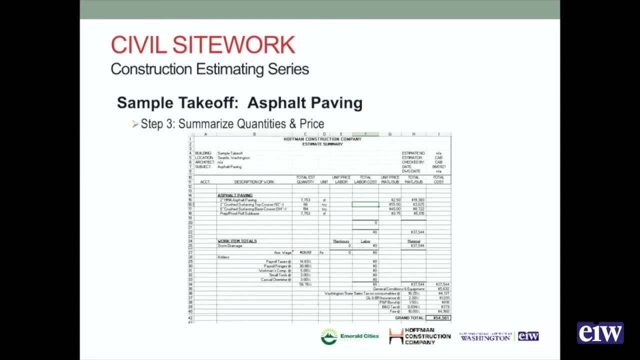 to make sure that we account for what work we need to do to prep or proof roll that subgrade, to make sure that the subgrade is in the right condition. so for something like this, I would actually just do all those formulas right in the summary, because I've got an area. 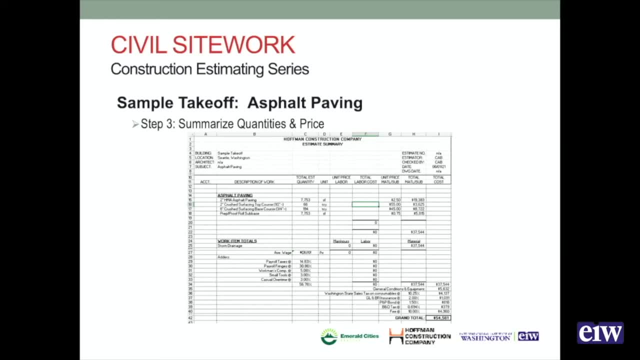 and then I can compute everything right off that one area, so 77,000 square feet of, or 7,700 square feet of, asphalt paving, and you've got the truck yards and the square footages that follow with that again priced out as if I'm hiring a subcontractor. 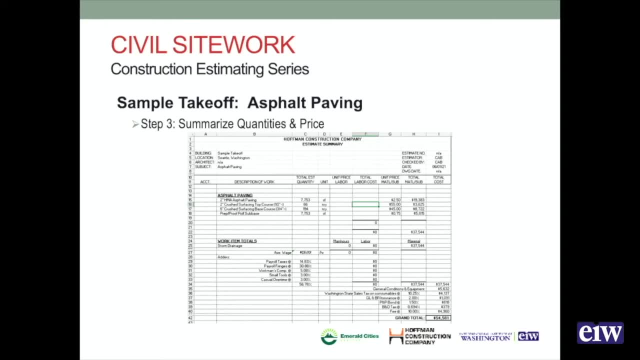 to do that work. mark it up, get your taxes and fees etc on it and you come up with a 54,000, a little over 54,000 dollars to do the work and that's really the sample take offs. we have the last section. we have. 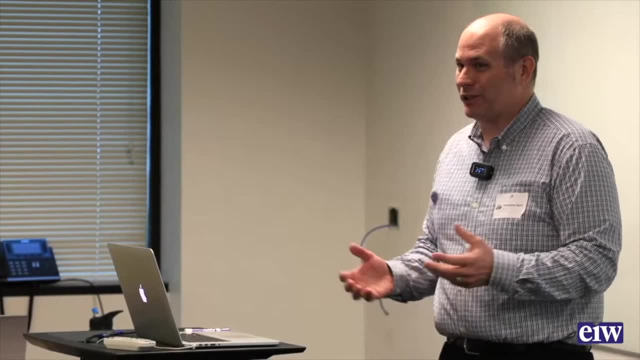 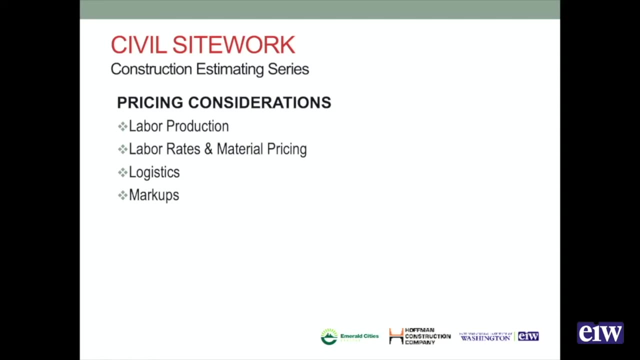 and we already started getting into this is the pricing considerations. what do you need to think about when you price, and that's labor production, labor rates, material pricing, it's logistics and markups, and we've talked about some of this, so I'll be able to go. 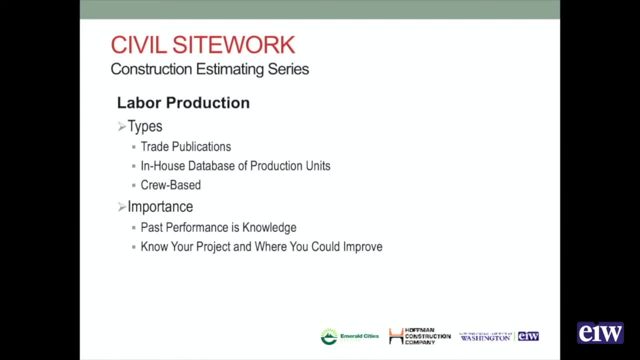 through it a little bit quicker here. labor production is hours per unit. where can you get that information? you can get that in a trade publication and RS means will have productivity units in there. if I run into something where I need to price something out in labor and materials, 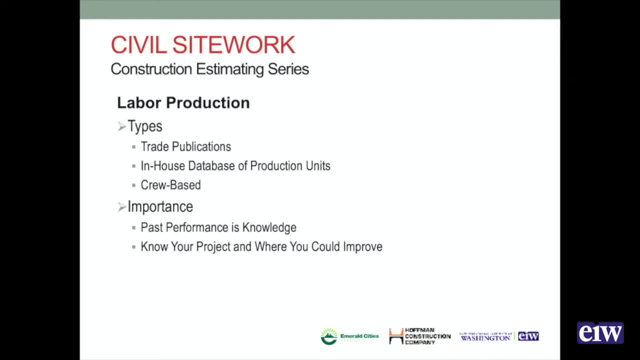 and I don't necessarily have a good historical productivity unit to use. I'll go to RS means because the productivity units are fairly reasonable to use as a good starting point until I have better information. there's a local publication called the guide which has information similar to that, except it's local to. 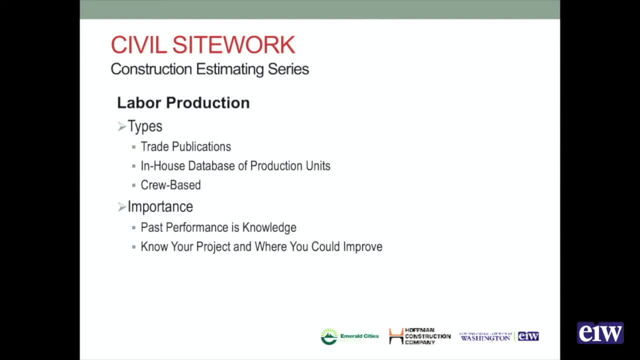 the northwest, but the best place where you can have is in house productivity units. and I will say this: if you are not tracking what you are actually putting in place in the field, not on just an overall job base, but how many hours per square foot of plywood- 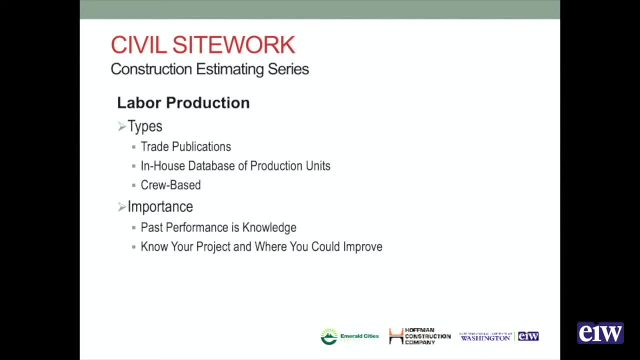 when I'm putting in plywood or how many hours per cubic yard of gravel fill when I'm compacting it. if you're not tracking that, you should be, because that gets you that historical cost information so that you know what your crews can do out in the field. 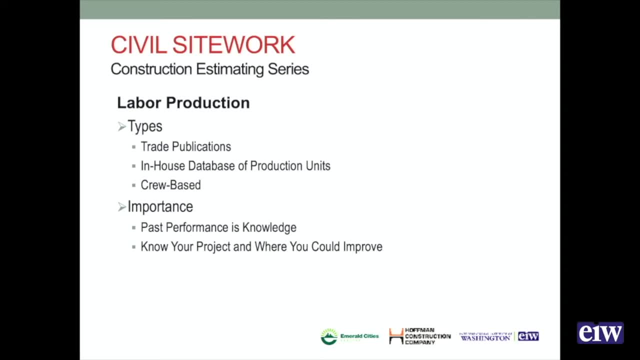 and then you couple that with your knowledge of the project and the challenges you ran into and the efficiencies you gained in that, you can start looking at those historical units and saying, okay, I know I can do better than that here. here I might need to increase this unit. 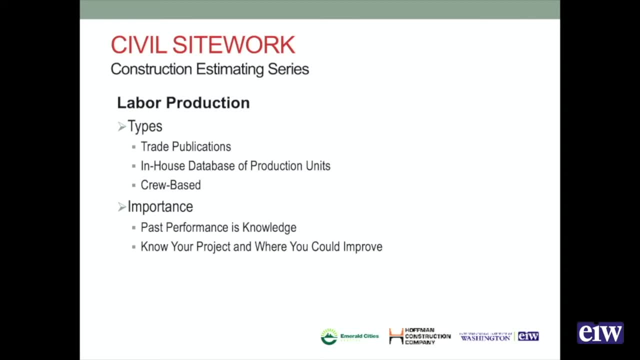 a little bit, because I know I may run into some problems here. or at least historically I have. that gets you that information and it's really important because the past knowledge really can help guide what we look at in the future. plus, when you are out in the 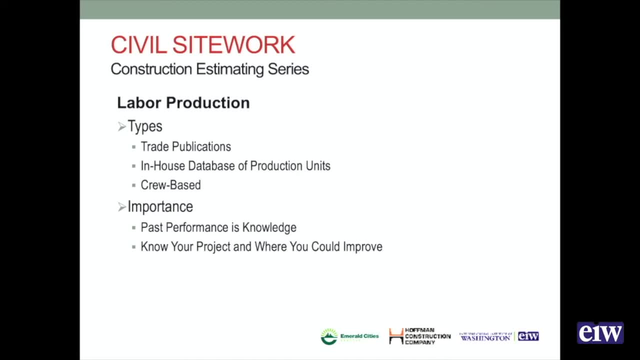 field tracking this labor. you can track how you're doing against your estimate and that way you can understand if you need a course correction in how the job is being run earlier than towards the end of the job, when it might be too late to salvage it absolutely, and that's important to know. 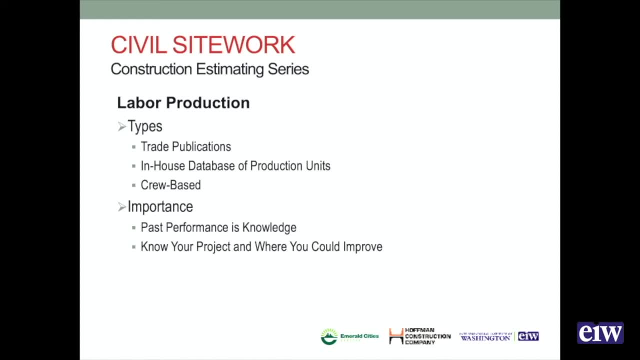 that goes into how busy the market is and what kind of a crew am I going to be using? doing crew based estimating, too, is a good check. some companies will say, hey, instead of estimating by productivity unit. I know that I've got a. my excavation crew is two laborers. 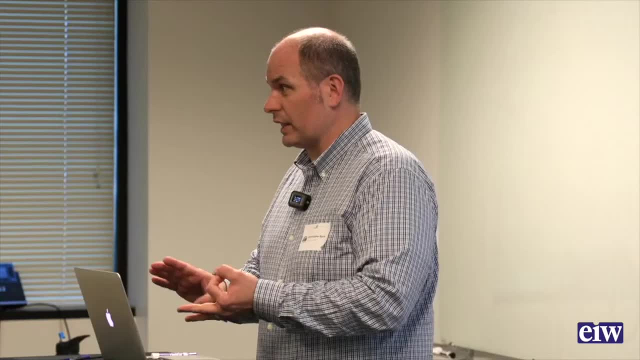 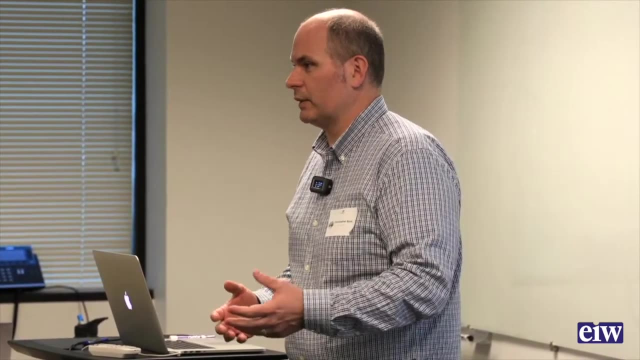 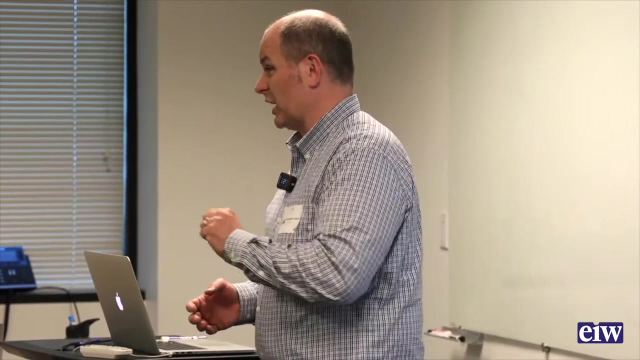 and an operator and they can put in 100 lineal feet of pipe per day and that's so. I've got how many lineal feet of pipe and that's going to turn into how many hours that I need on the labor side. I've used it as actually a back check. 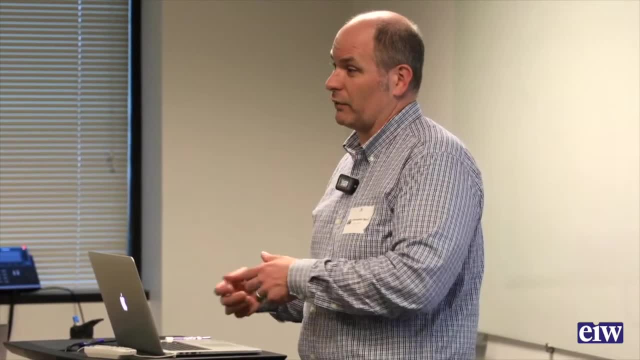 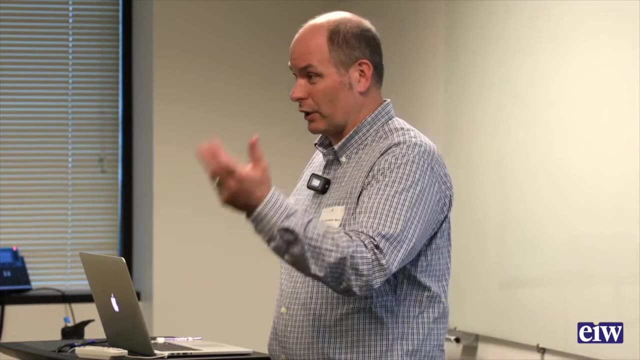 a great back check. so I'll sit down with using like for concrete estimating. I'll go through with our productivity units. I'll sit down with the superintendent who's been out there running the work and we'll do the same estimate, except from his perspective on what. 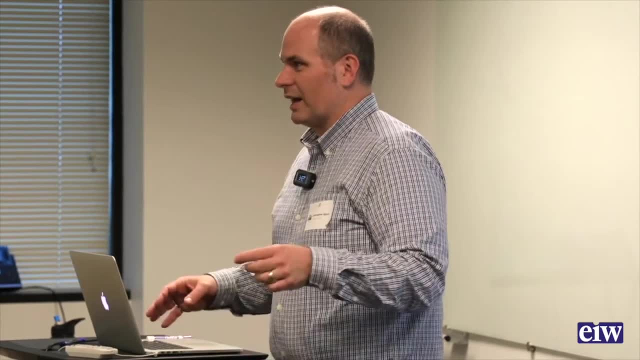 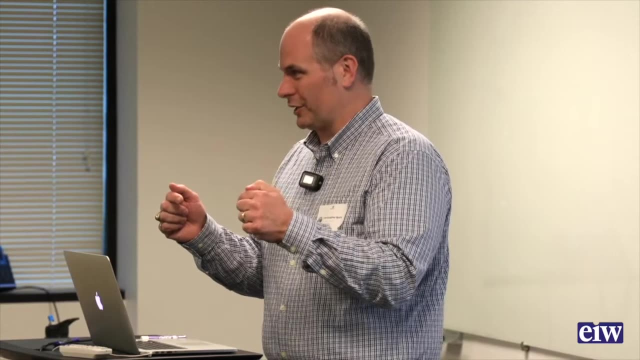 crews, what size crews and what durations he's going to use. and that's great because that is a back check. if you come up with two numbers that are close to each other, you know you're looking at the same job. if you come out with two numbers that are far apart from each other, 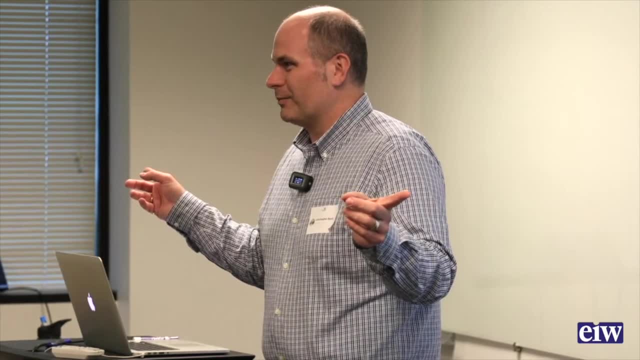 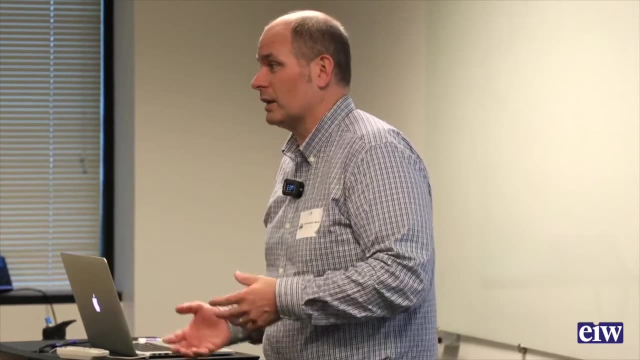 let's talk about what's the difference, because there may be just a disconnect on how you're looking at the job and I, when I've done this with superintendents, sometimes they're right, sometimes I'm right because we have come at it looking at two different ways. but once you get, 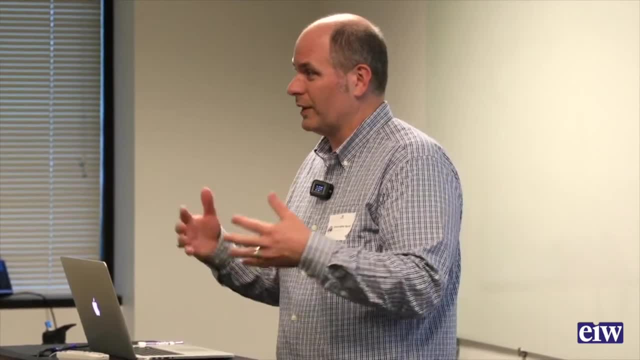 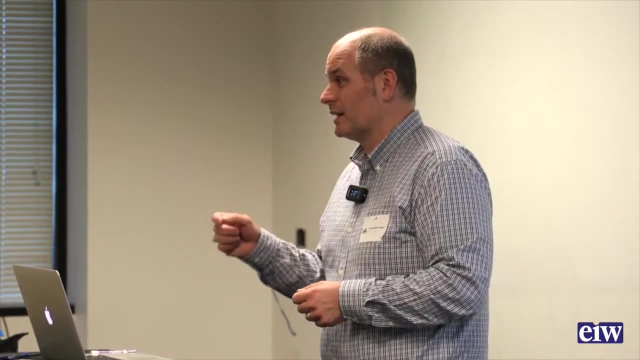 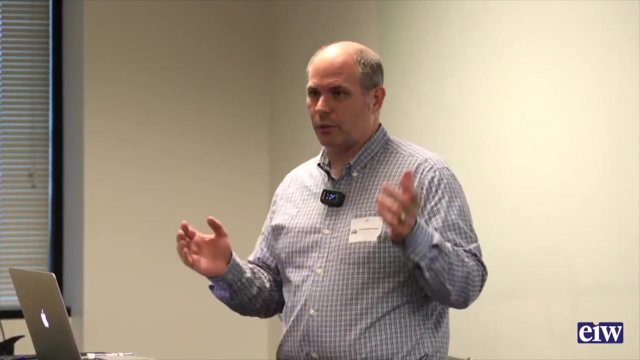 to that the closeness of both agreeing on the estimate. that way you know you have an accurate estimate because you're both looking at the same project two different ways and coming up with close to the same number labor rates. so are you a union shop or are you an open shop? what's your base wage? 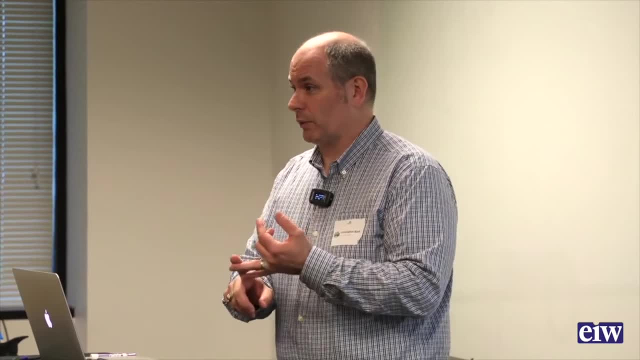 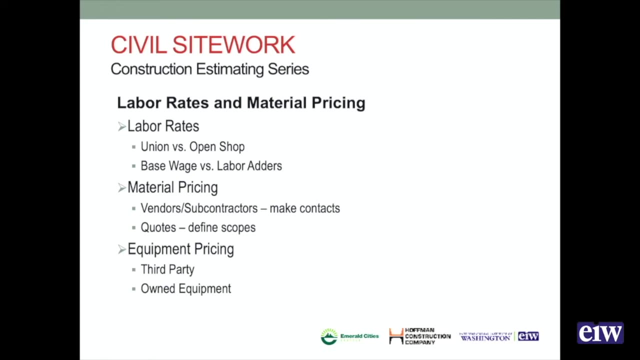 what are your labor, that's, your payroll tax, your payroll fringes, workman's comp, insurance. you might have some scheduled overtime. you might have some allow something for some casual overtime. just knowing it, hey, I know that I'm going to have to work a crew, a couple. 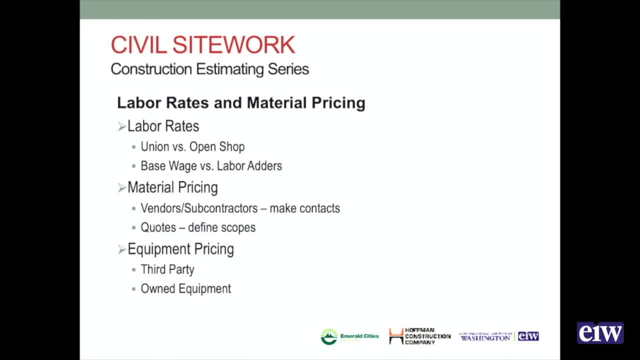 extra hours every so often, and that's going to be 3% of the labor cost, and so you need to factor that in into your wage rates. then there's the material pricing: talking with your vendors, your subcontractors, making sure, when you get quotes from that, making sure that they. 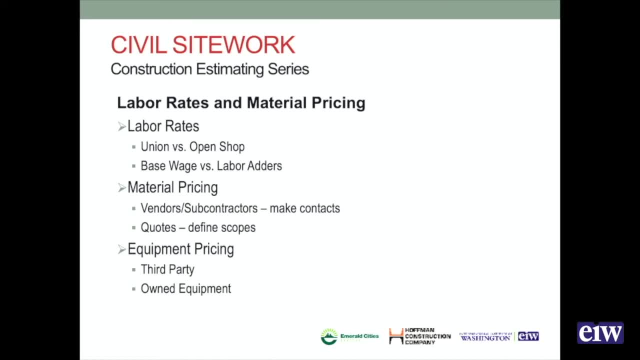 understand what you're looking for and you understand what they're going to give you, because undoubtedly they're going to exclude something that you need to plug a value in for and if you can work that out and have that good communication up front, then you have that pre-plugged and you're expecting it. 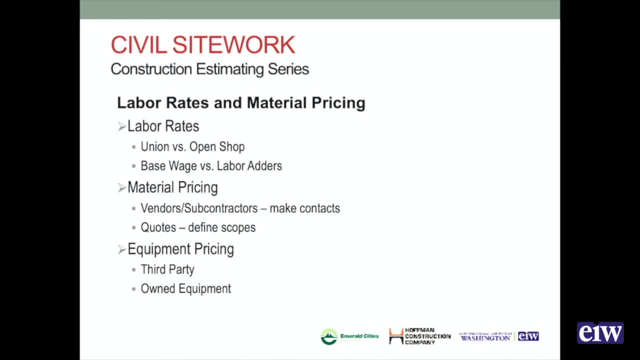 and you're not trying to figure it out on the fly, because that can be a little bit nerve wracking if you're bidding a job to suddenly, oh what's this going to cost? and if you bid jobs you've been there, but so just making sure that you have that. 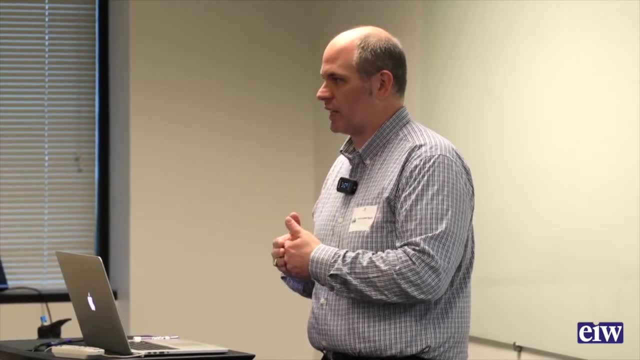 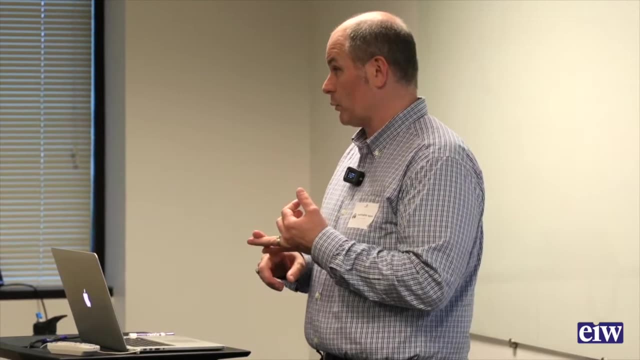 communication with your vendors and subs to make sure that you both understand what the expectation is: equipment pricing, you know. are you renting from a third party? are you renting from? do you have your own equipment that you're renting to yourself? is the project large enough and long enough? where it makes sense, 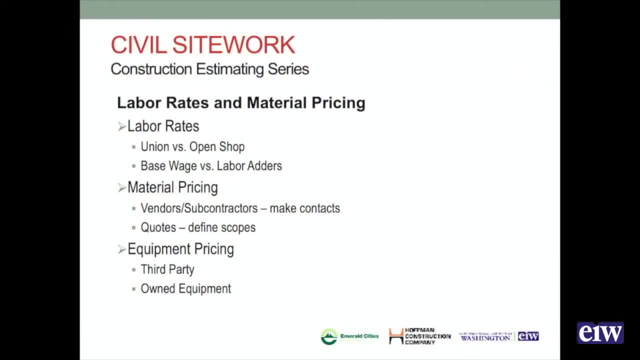 to buy the equipment as opposed to renting the equipment, which then you may have some maintenance costs after the fact. but you can then rent the equipment to yourself and you've paid for the equipment already. so that's might be another profit center if you're renting to yourself. 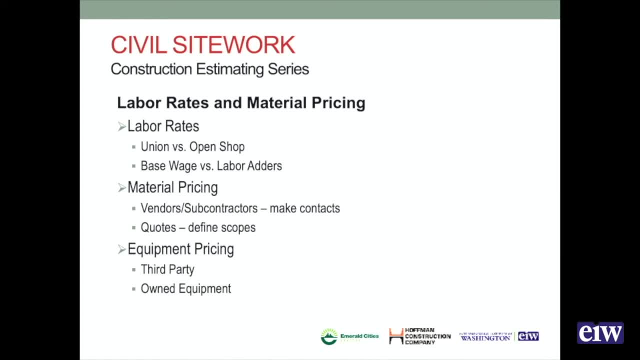 but you've got that added cost to make sure that you maintain and manage the upkeep on that equipment. then the next part of pricing is the art of estimating. it's the logistics schedule considerations. when is the work happening? is it happening two weeks from now? is it happening? 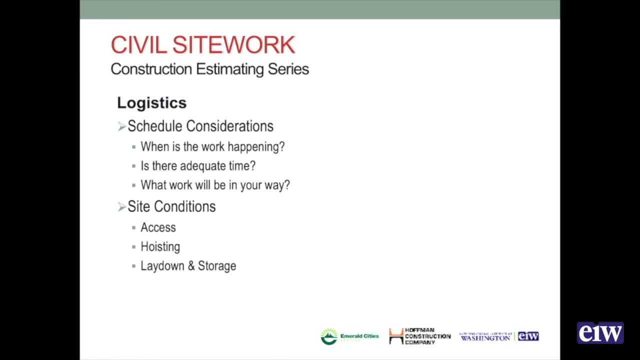 a year from now. if it's happening a year from now, you need to make sure that your wage rates are right, because in a year your wage rate is going to be higher, your material pricing may be higher and you need to factor that escalation in if you're going to take the risk on it. 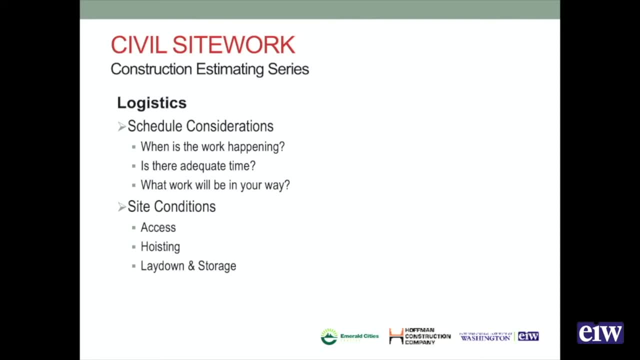 is there adequate time in the schedule? there may be a very good reason why a general contractor has allowed you to do two weeks worth of work in one week of time. there may be other schedule constraints. that that's the only way to get it done and you need to know that. hey, I'm going. 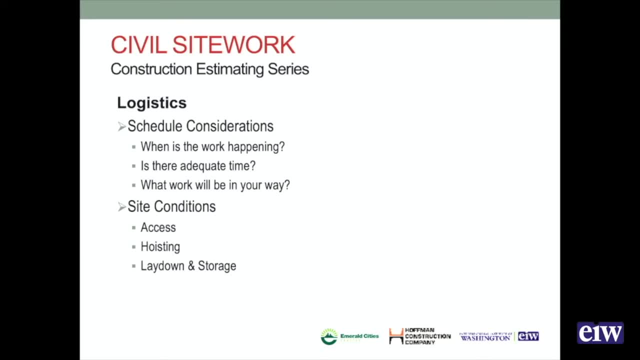 to have to double shift this to get that two weeks in. well, there's a cost impact to double shifting something. if that second shift is, you're going to pay them eight hours for seven and a half hours worth of work. if they're a union, if you're a union contractor. 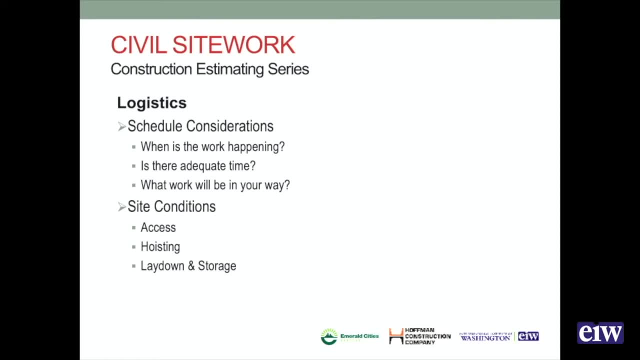 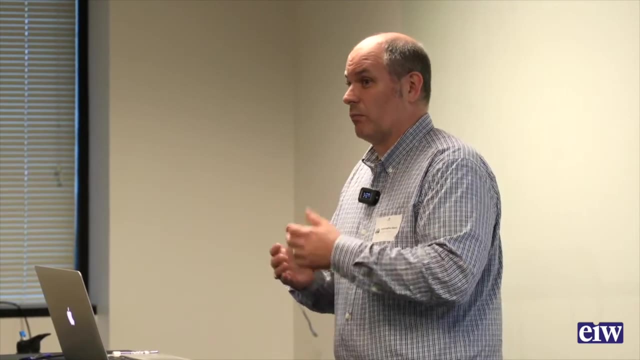 and you need to know, understand, how that's going to work and what work will be in your way. and that means looking at not just your scope of the schedule but the rest of the schedule too, because it may be very apparent in that schedule that say what's. 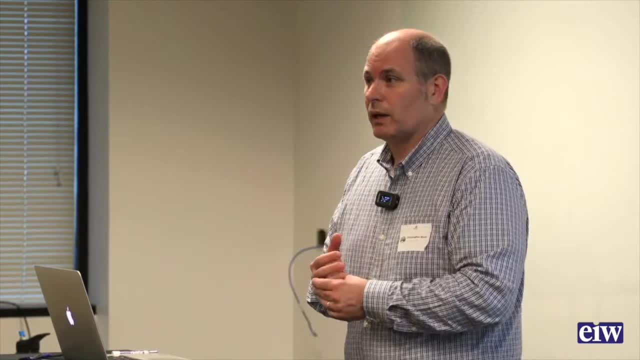 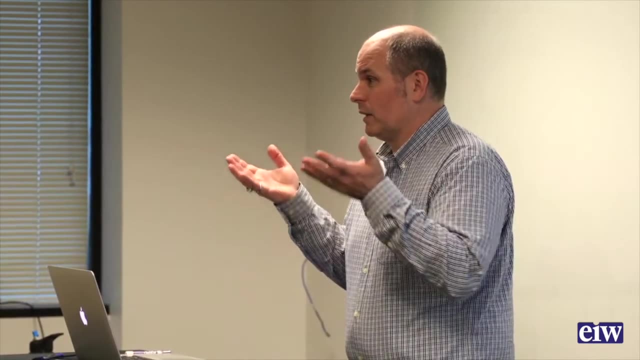 you know an example from the UW light rail station where, the way that we constructed the project, we actually had to put the escalators in before we finished the concrete work, so, as we were building slabs, we had to shore around the escalators that were already set. 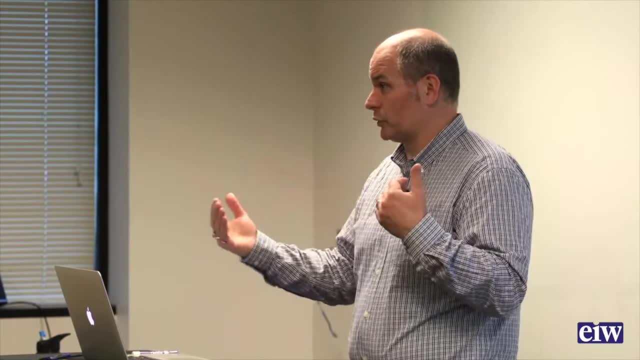 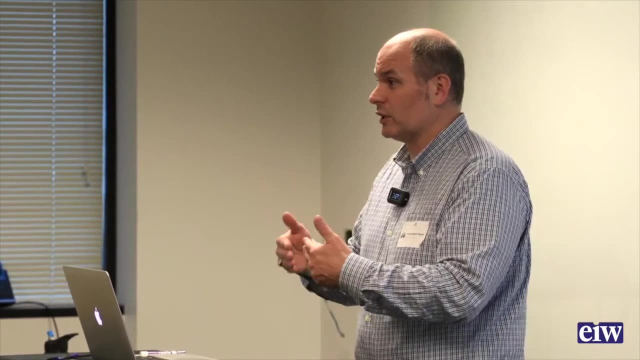 in place and make sure that those were protected and shored against it, which altered our shoring pattern, because we obviously couldn't put shoring towers right where the escalator was. it's a key thing. you need to understand what your points of access are. what work is going to be in your 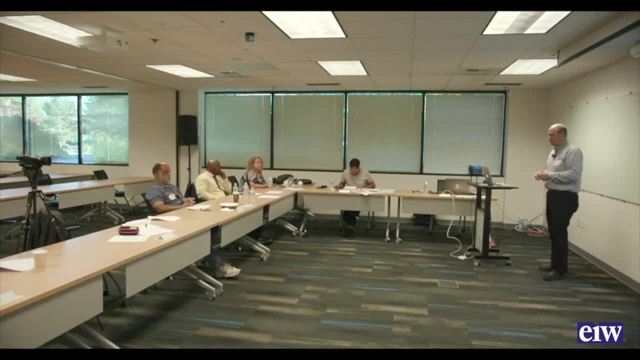 way so that you can price it effectively. things like hoisting, you know who's providing it. those are things to understand too, where your lay down and storage are. do you have lay down on site or do you need to have a warehouse, maybe to store pipe, and that's a cost if you. 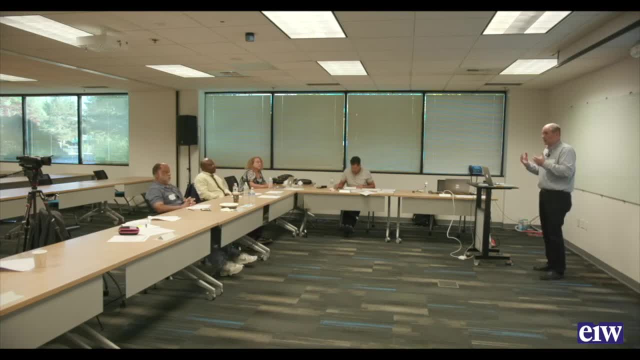 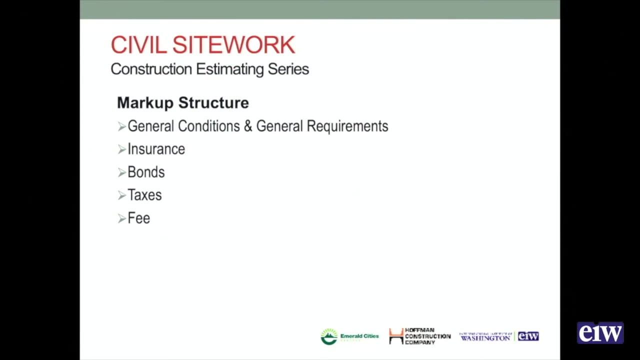 don't have it in your own own yard, you may have to rent some place to store materials. and finally, the markup structure, and I'm going to just touch briefly on this, because this is really. this is a whole other session to talk about markup structures and we are planning on doing something. 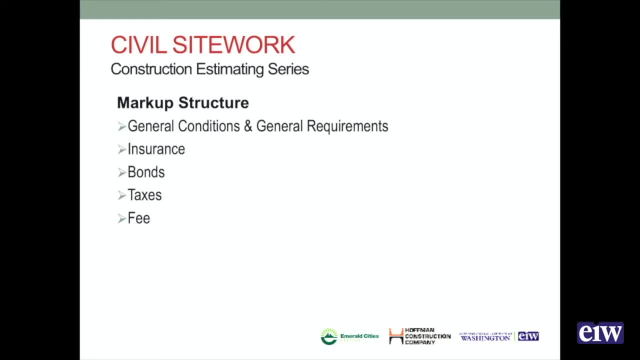 about this and using a structure of this, but that's your general condition. how are you staffing the project? project manager, superintendent, nonproductive foreman, superintendents? you know general requirements, your trailers, you know the labor you have. that's not really doing any. you know actual, direct 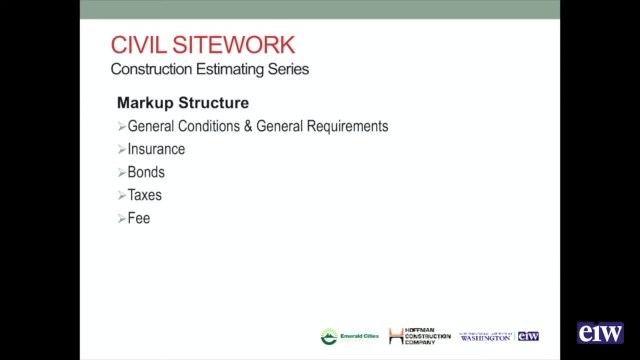 work, but it's helping make sure everything's clean around the site and your work area is clean. insurances: your general liability, your insurance, your workman's comp insurance, your builder, if you have builders risk insurance. if you're doing something- design, build, your- you might have to carry errors and emissions. 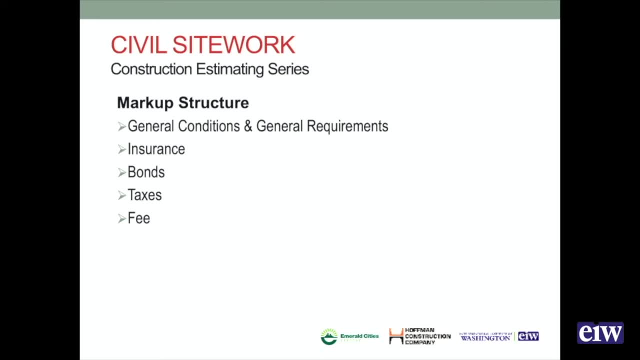 insurance for the design work bonds. do you need to carry a bond? do you need to carry bonds for your third tier subcontractors? you need to understand that what those costs are taxes and then obviously, your fee. so what are you willing to do it for? and that's. 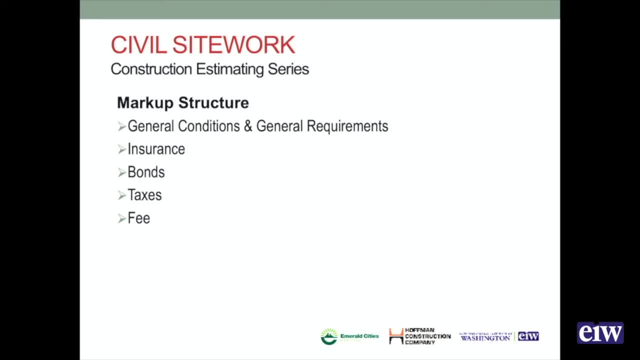 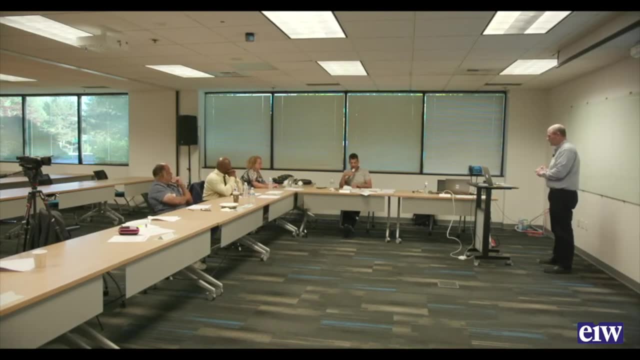 you know we've already had a large discussion about fee there, so with that, that's the wrap up. so talk about questions. yeah, really quick. before we start to get into the questions, go back on the markup structure. you know uninsurance. you know most of us as business. 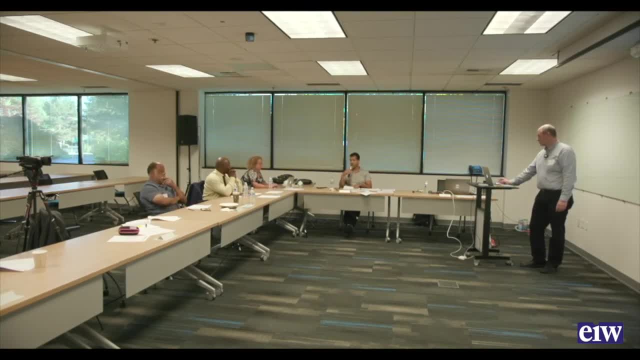 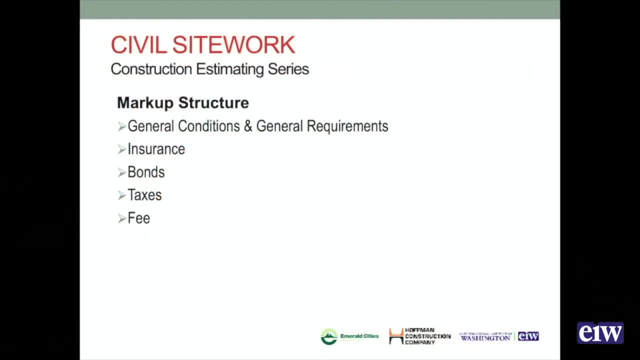 owners, you know, have general liability. some of us have even professional liability. what you also need to understand is that your labor, bless you, has markups and sometimes you know that can be, you know something that it's a cost to your labor and so if, for instance, 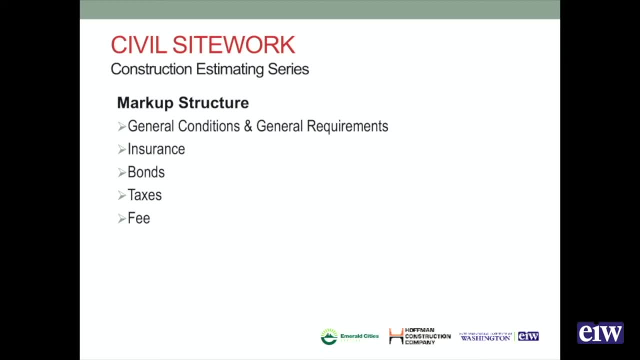 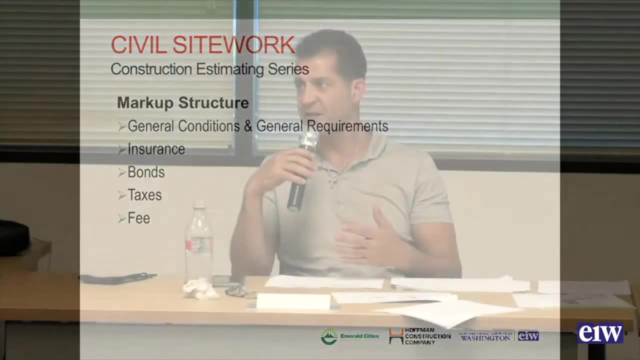 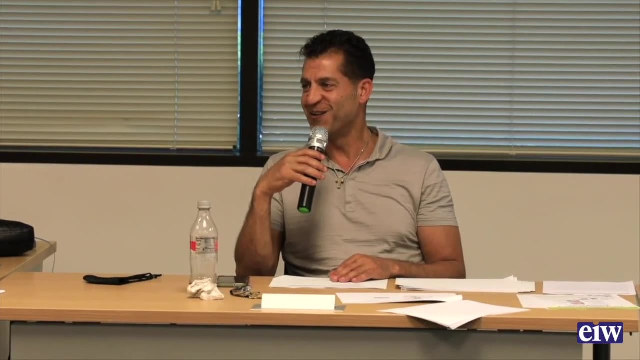 you thought you were going to have 200,000 in payroll and you had 500,000 in payroll. guess what? your insurance company that is, you know, providing, you know, that umbrella for you will, you know, bless you with some additional fees as it relates to your next year. 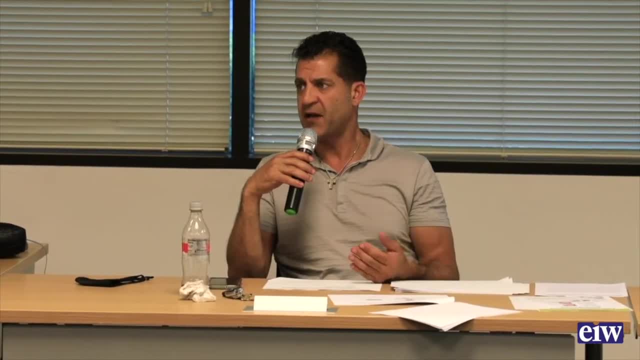 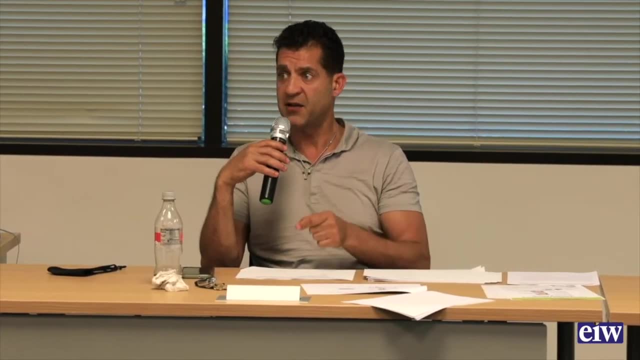 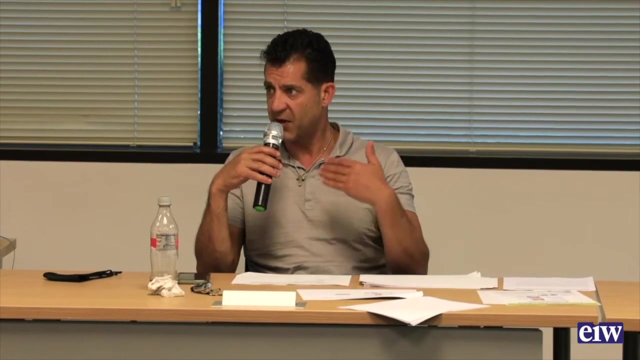 premium and so forth, so you always want to be aware of that. also, in labor and industries, that's something that you know. sometimes folks aren't not necessarily taken into consideration whether you doing the work inside or outside. what craft is actually performing that? and so you want to make sure. 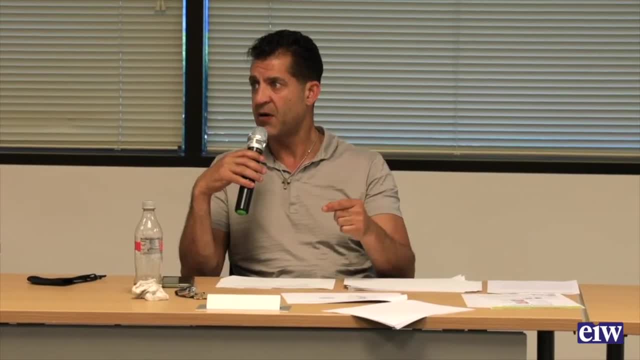 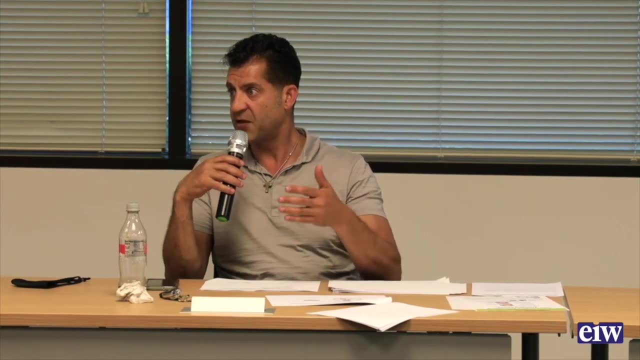 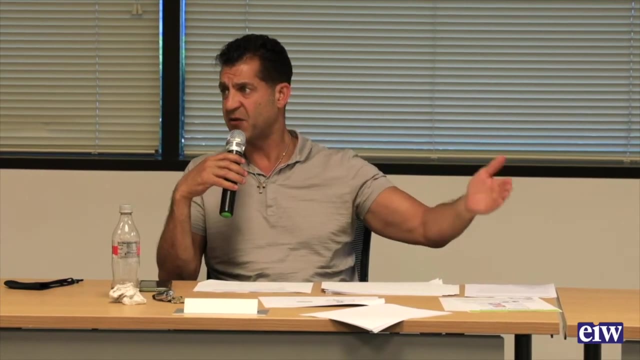 that you've incorporated that into your labor and sometimes you know if you're a member of a trade union. there may be other. you know costs that you want to make sure that you have them included and, like for instance with Hoffman, they have some of their projects. major government. 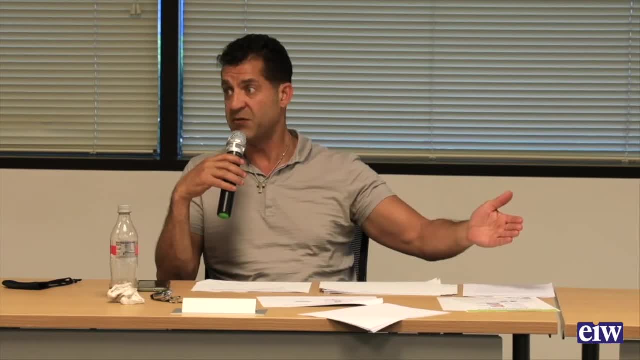 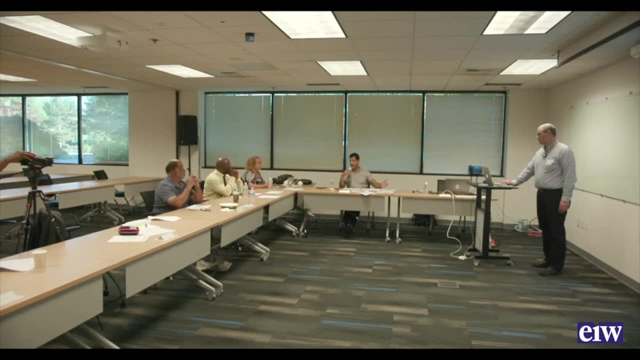 projects. they take years to deliver these projects, and so parking for a journeyman trades person every day in downtown Seattle, for instance, can be, you know, 20, 30 dollars a day, right, and so that's a real cost. and so what I want to just make 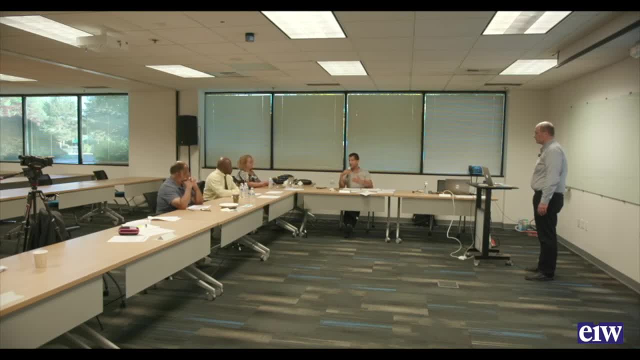 a point is: make sure folks understand and appreciate the cost that it takes to get an individual on your job. we have some questions and I know our participants also have some questions, so I want to start with those folks that are online because they haven't had an 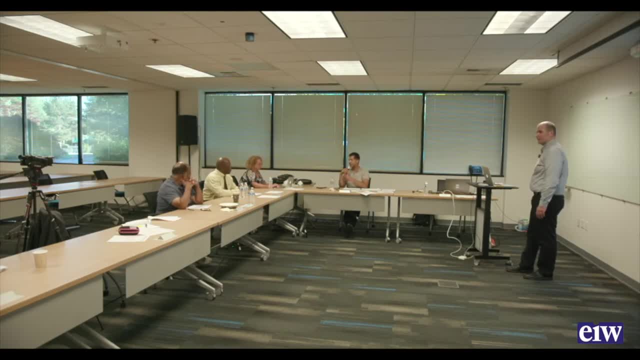 opportunity. all right, well, I'm going to pass the microphone to our participants and see if there's any other thoughts or questions that they may have, and thank you very much, Ryan, for the great questions. I have no questions, not actually. this is your chance if you have any. 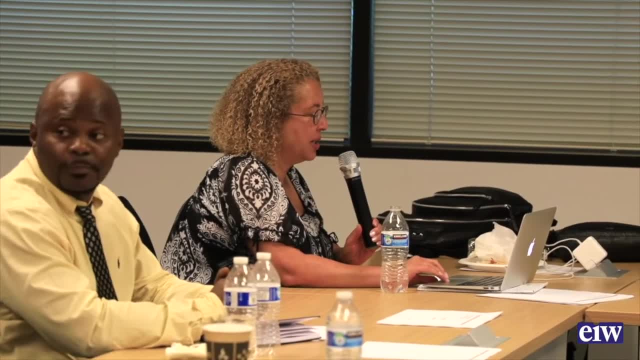 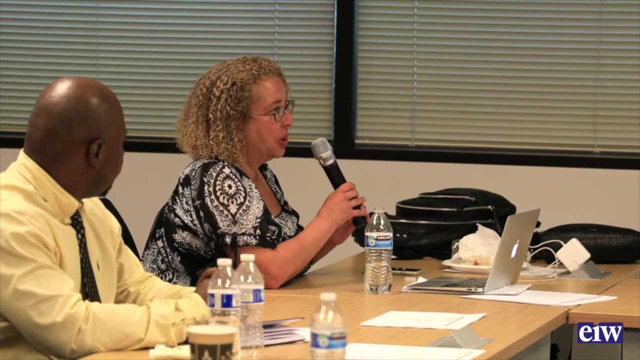 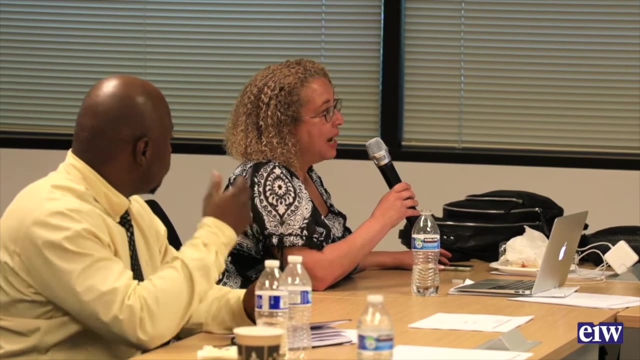 questions. we would like to hear your questions and clearly we had a few little technical difficulties and what we're going to do is send everyone the slide show and we can make Dan Seidel available to gather questions, answer questions and, if they need to be addressed to Chris Bjork. 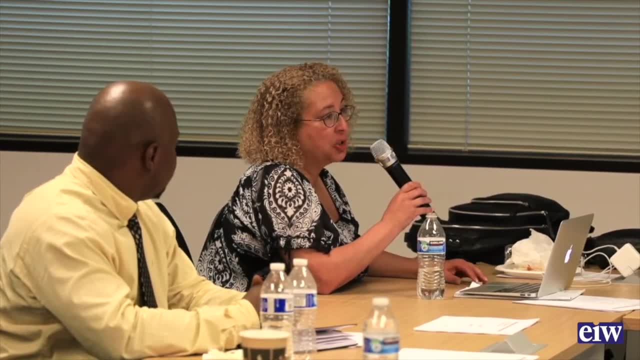 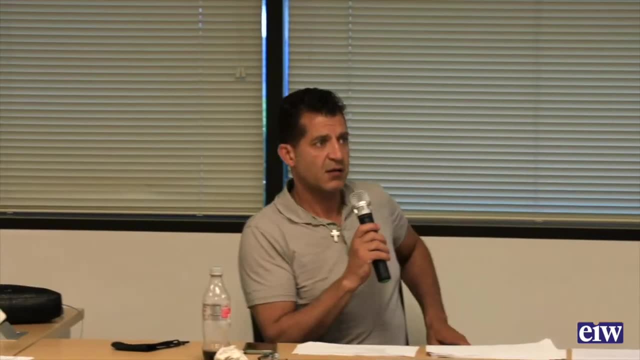 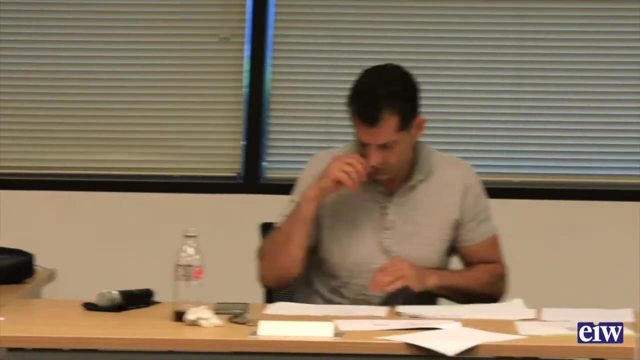 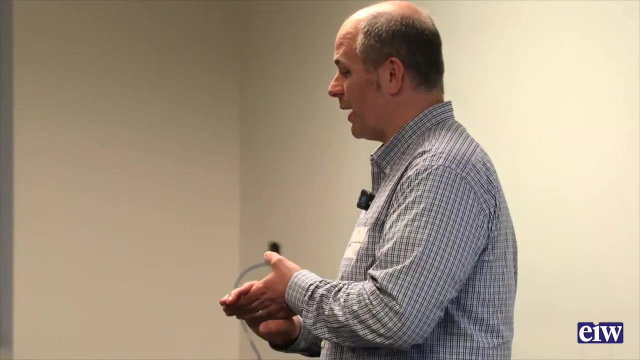 our instructor or others with specialties. we will make sure those connections occur. yeah, so just wrap up quick here. conclusion: what we covered: we covered civil sky work scopes. we covered take off methods. we covered pricing considerations. now one thing I would say: there's application to new items, so 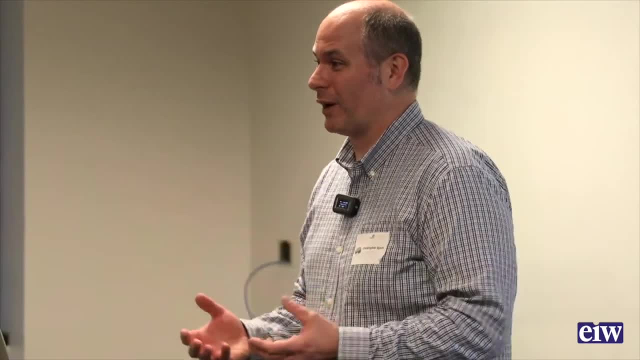 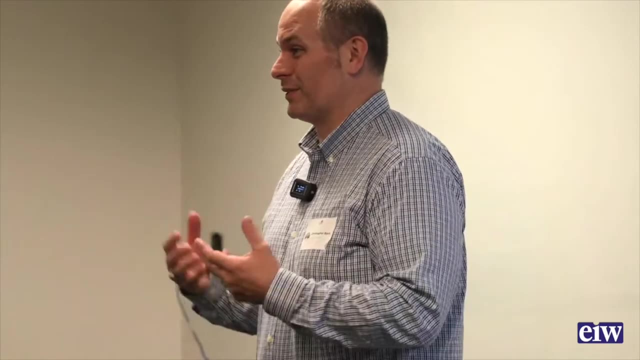 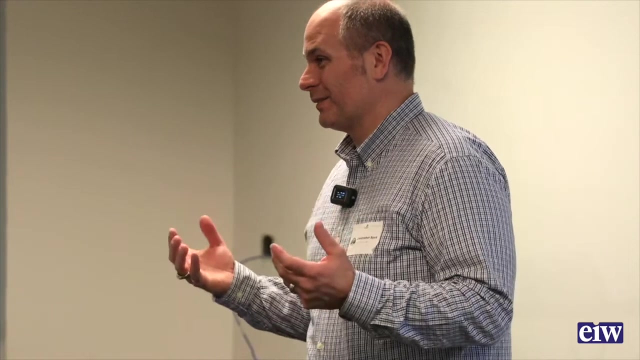 what the methods of taking off, what we take off, apply to. whatever you take off and whatever you estimate, because you will always find something that you've never seen before when you estimate. I've worked in, you know 20 plus years and suddenly we're renovating. 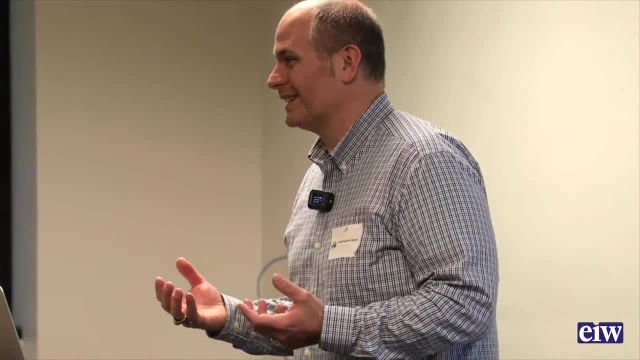 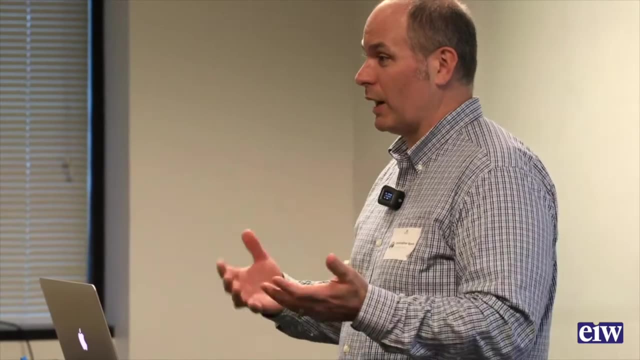 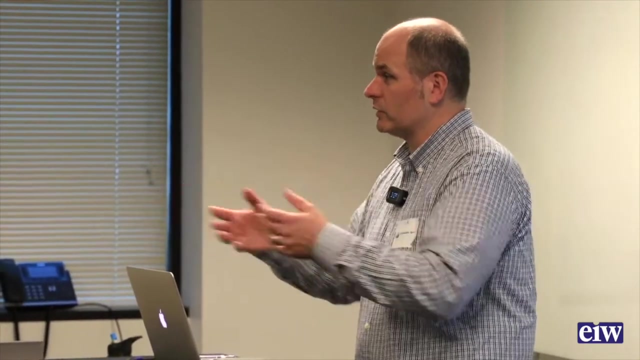 the space needle. it's not something you really see very often. it's kind of a once in a lifetime type project. but everything I learned- I knew how to do, how to quantify, how to price, how to look at the logistics involved in it is how I used to do. 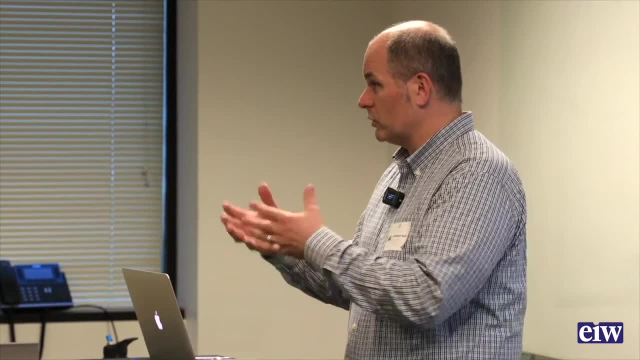 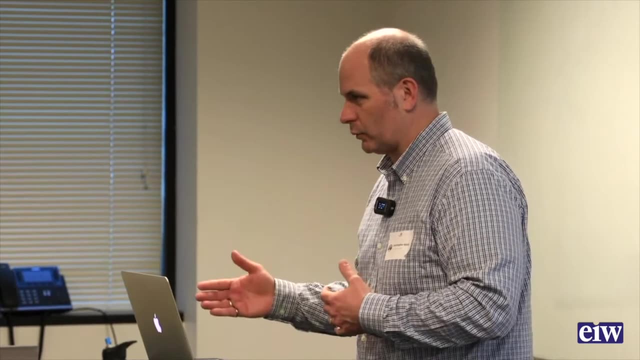 the estimate and you take what you know and apply it to what's new and it's the same methodology and the same thought and that will get you through, so that you can use this no matter what comes your way. whatever you have to estimate, it's you know, knowing what units you are. 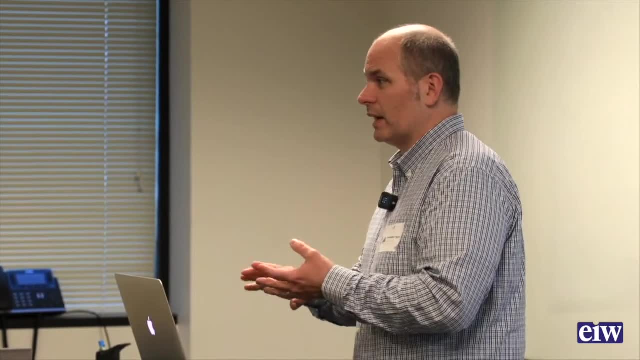 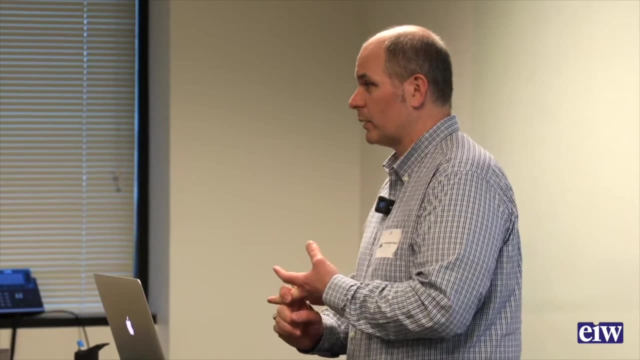 what you need it's: how much of something do you have, and then how much is it going to cost me to put it in place, and whether I need a quote from a vendor or subcontractor or I'm going to do something myself and install it myself. 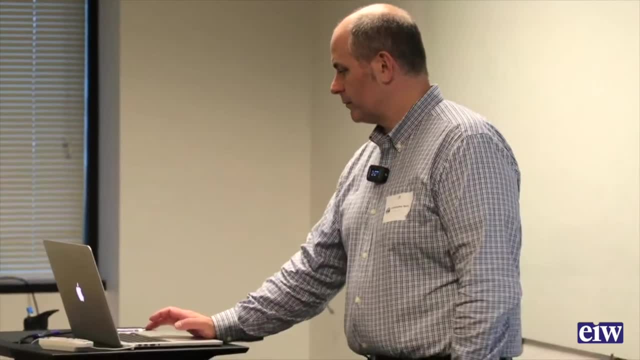 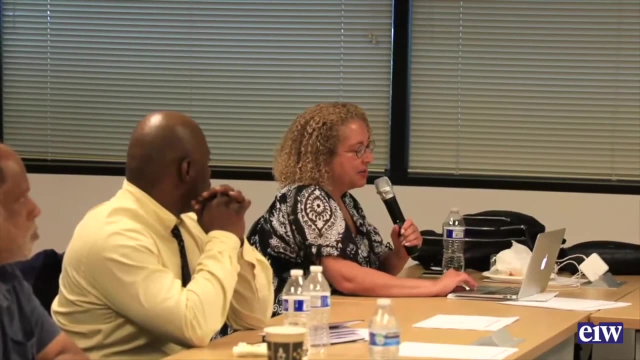 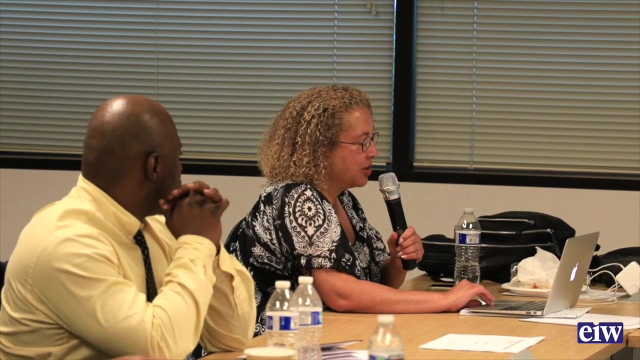 you understand where to get that information. We have a question, and I think I just got a question via text as well. Mayor Mata, this is Roslyn. I'm going to allow you to ask your question verbally, so be prepared to ask your question when I turn this on. 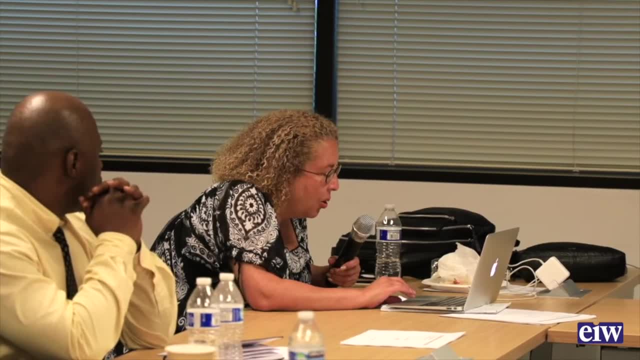 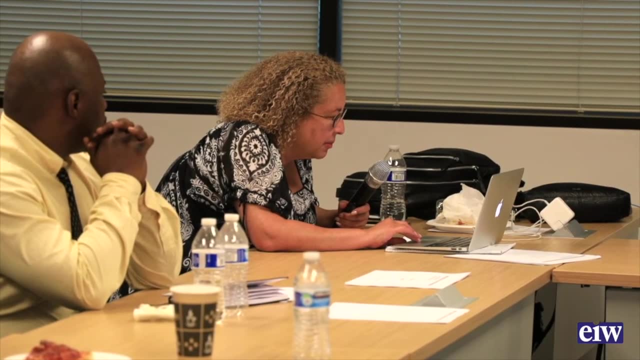 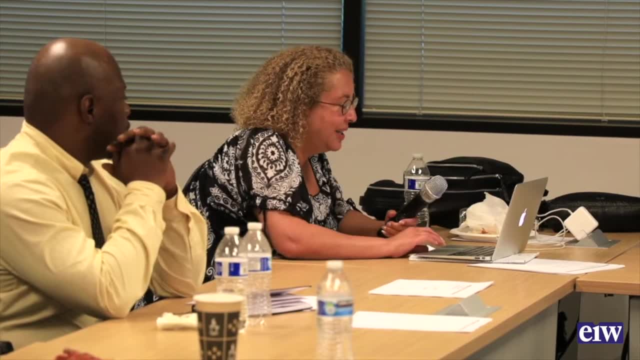 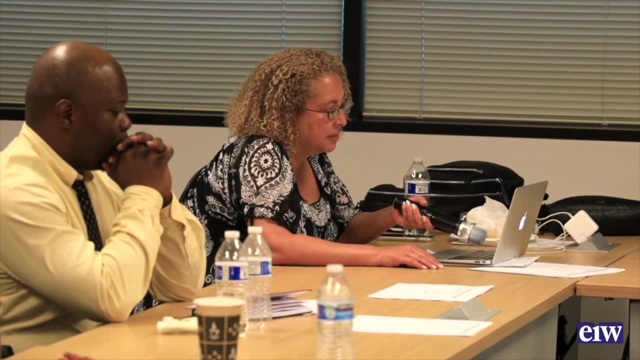 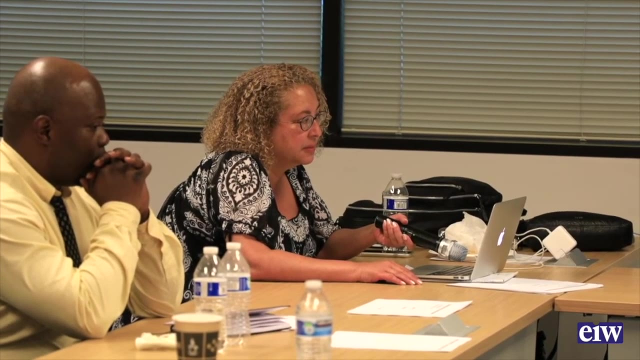 Can you hear me? Yes, Perfect, thank you very much. First of all, I don't have a question, it's more of a statement. I want to thank Hoffman for really five years ago I was sitting where other people are sitting there today to talk about estimating, to look at. 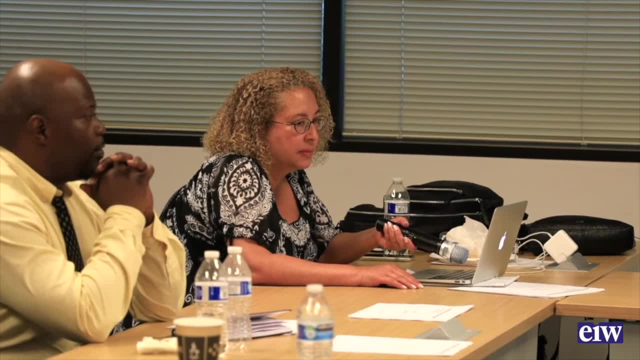 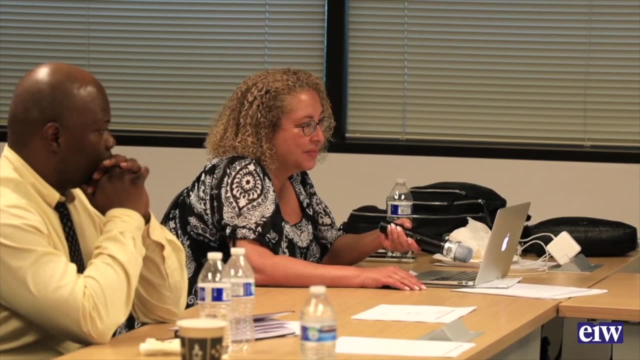 you know what it looks like to estimate a job, and I was sitting right there and five years later actually- and I'm happy to announce this publicly- but secured a contract with Hoffman for over $700,000, and these classes that you're going through are very important. 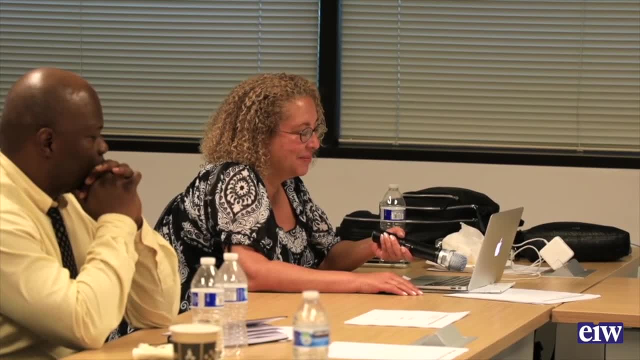 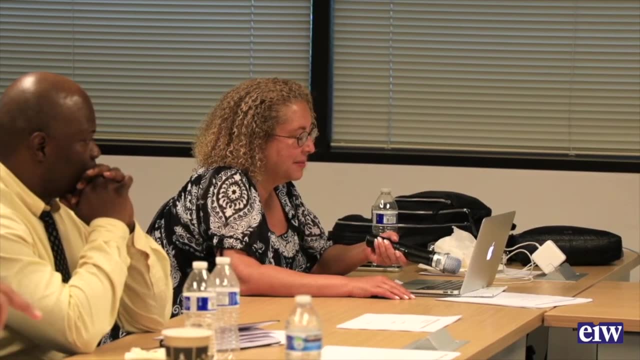 some of it may be over your head, and it was over my head five years ago, to be quite honest, and I never thought I'd get it right. it's not necessarily about getting it right, it's about understanding it. that's why you end up hiring professionals with your company. 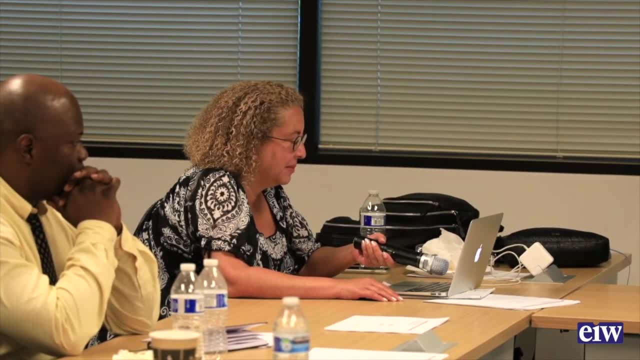 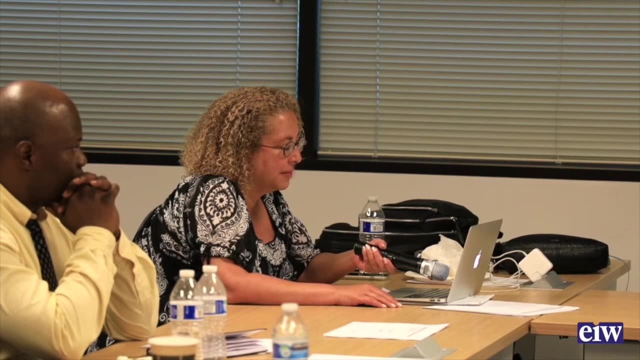 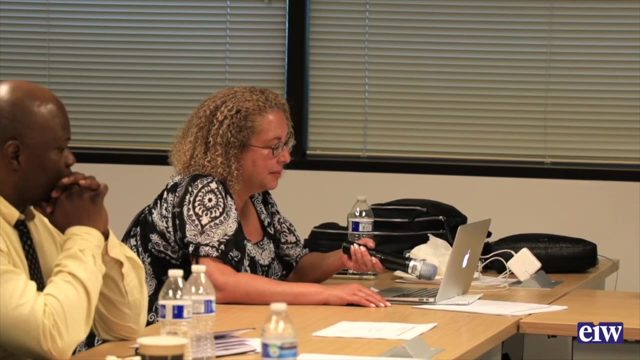 when you first start out, these are very important for you to really focus, look at, break it down, and I'm grateful that general contractors are taking the time and that we have organizations like the institute and Emerald Green to make sure that we are getting the training. so thank you very much. 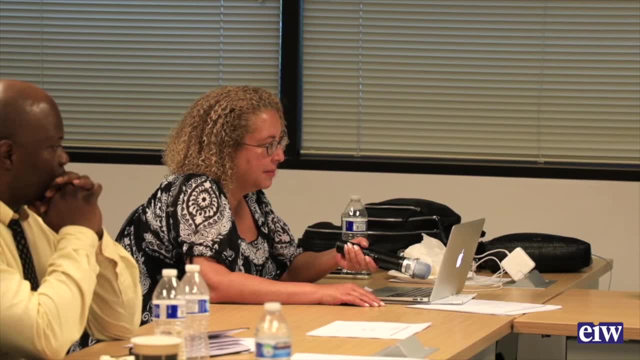 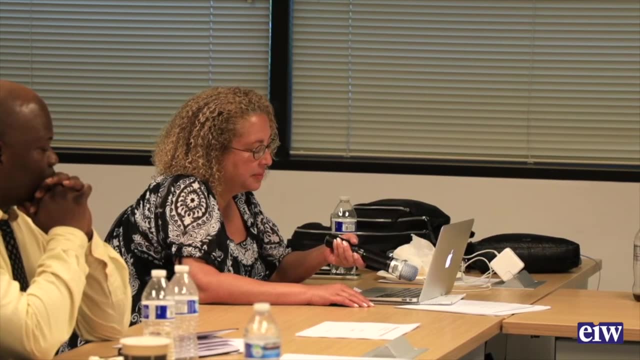 I look forward to sharing your training with my former superintendents and making sure that they're out participating in this class. so very happy to have participated today. thank you so much, and I also want to thank Hoffman and their leadership for continuing to push forward. 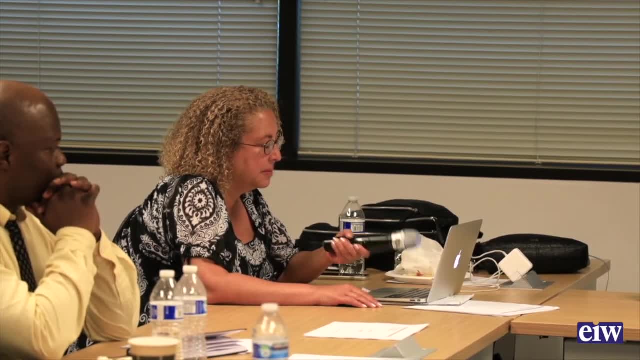 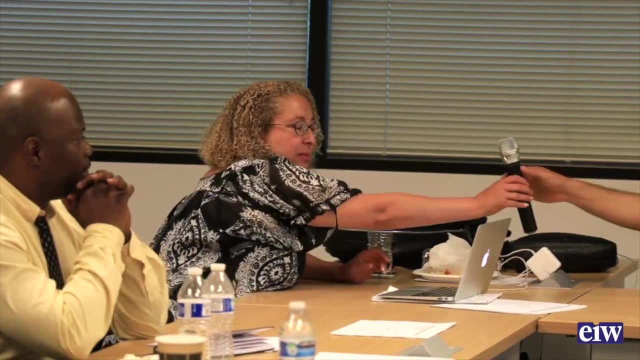 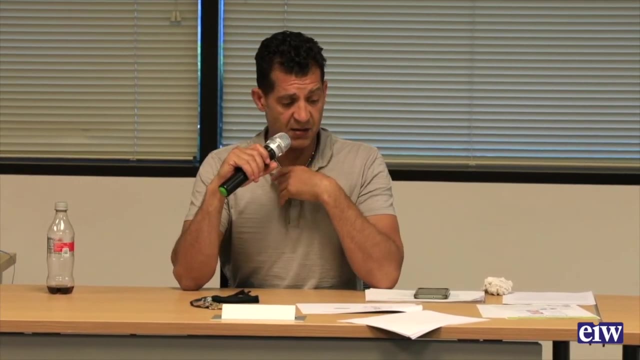 and helping us exceed and try to scale up. thank you very much. Thank you, Mayor Mata, and thank you also for stopping in in person earlier. Yes, and I just have to echo: Jimmy has. Mayor Mata, excuse me- has just been a wonderful addition to this body and in fact, Hoffman has. 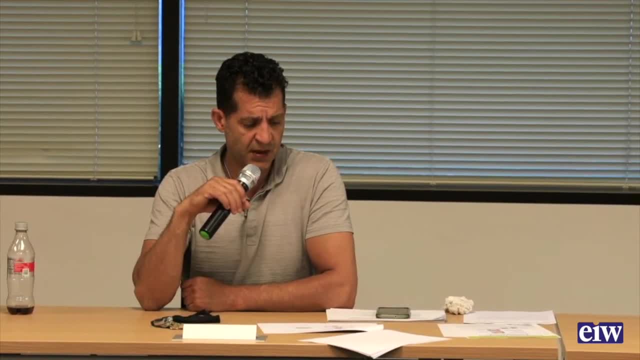 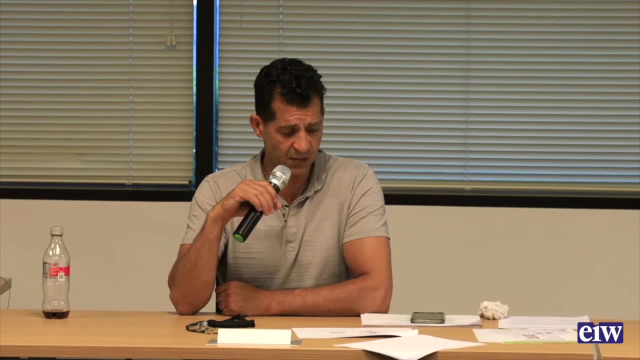 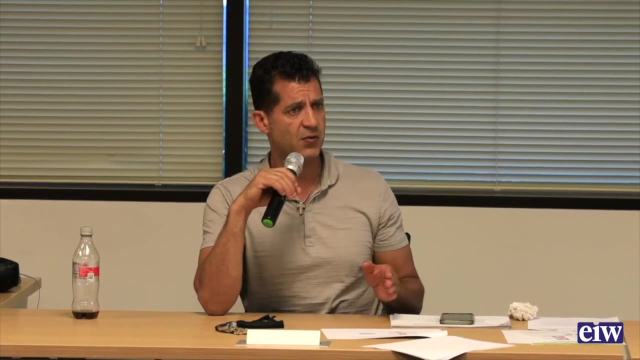 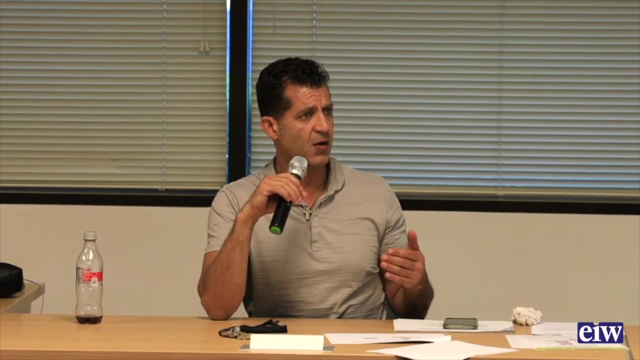 really taken an effort to embrace AHORA construction and actually looking at mentoring- yet a third firm- and so we couldn't be more proud. earlier in the presentation, you had showed some spreadsheets that you had already populated, and there are some folks that want to know if you would. 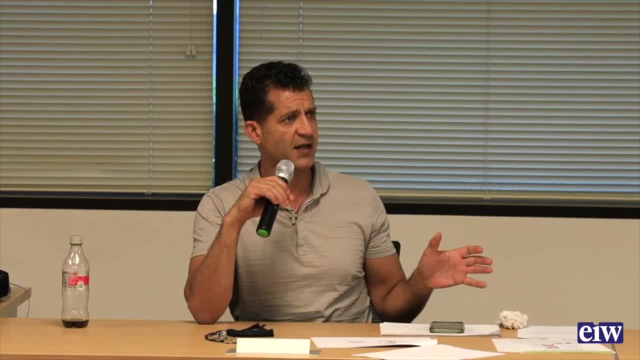 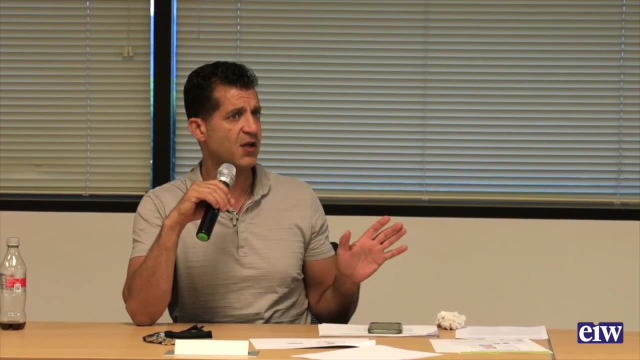 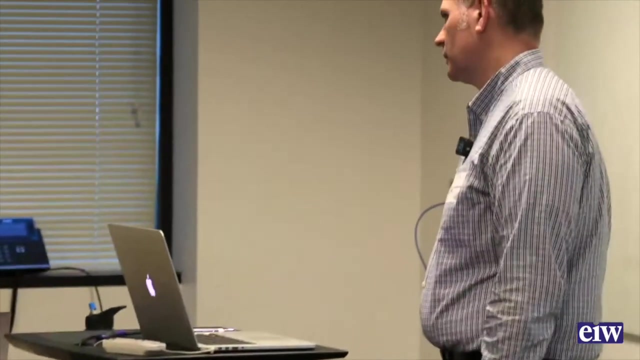 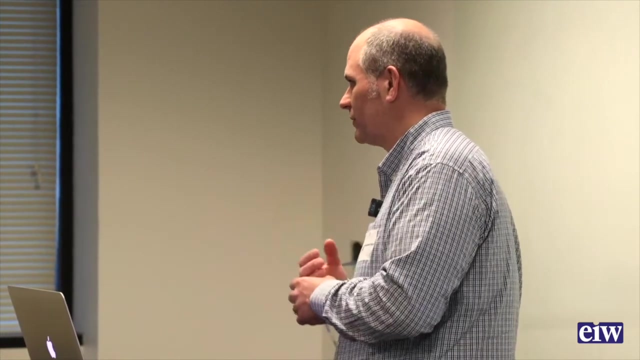 have any challenges or problems, providing some templates that folks could utilize that wouldn't jeopardize any competitive advantage that you know Hoffman has. I think that I could work something up. absolutely most of the stuff is just most of the items are, you know, just general formulas. so 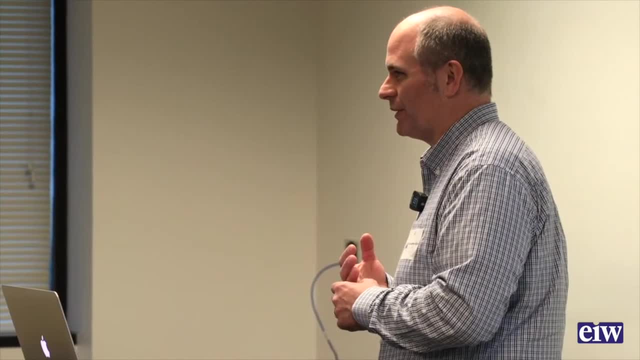 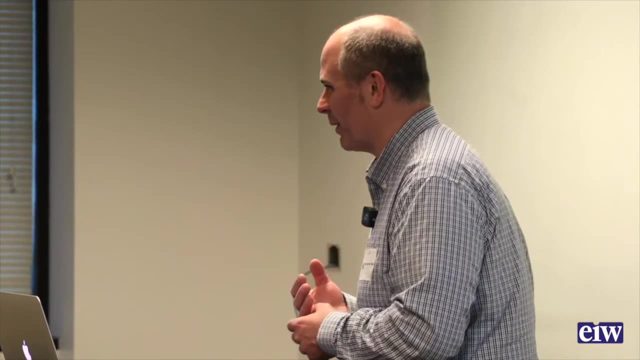 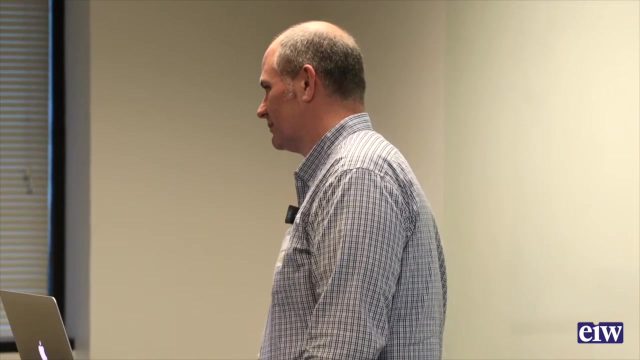 I have some of those templates. how you take off quantities isn't proprietary, it's the productivity units and proprietary sure? well, whatever you would be able to provide us, it would be a great resource. I know that the folks on the call and here would find this tremendously valuable. 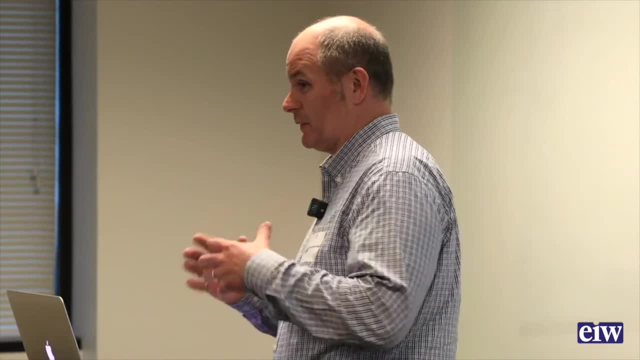 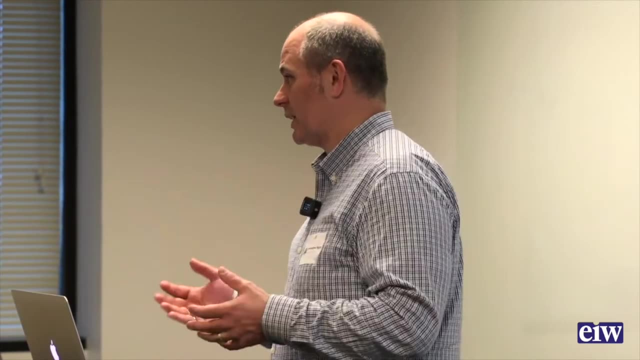 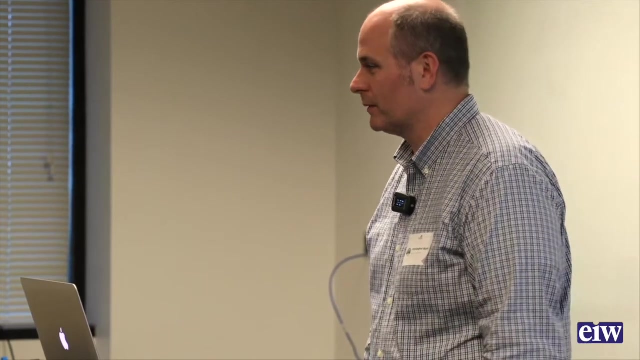 yeah, if people have specific templates that they're looking for- whether it's trenching, whether it's just a general take off- that would help me make sure that I get something that's useful and what will help people okay. so last thing is future opportunities at Hoffman. 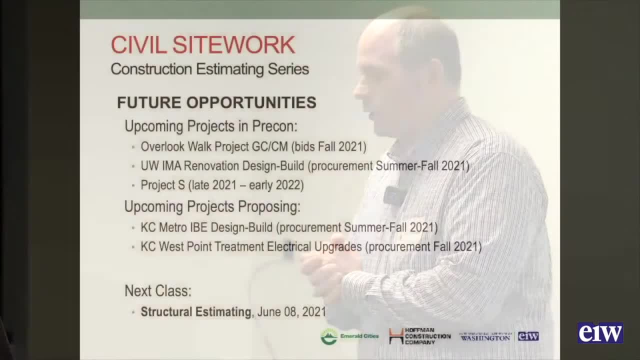 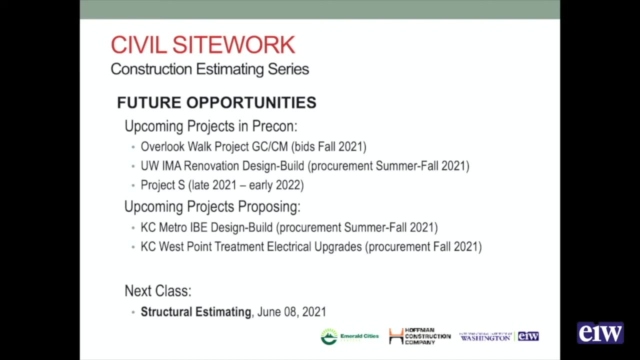 we always like to highlight what's coming up, so we've got the following projects that are in pre-construction: the overlook walk project, which is part of the waterfront redevelopment in downtown Seattle. cool project: it's a- basically it's a pedestrian bridge that will connect Pike Place Market with the. 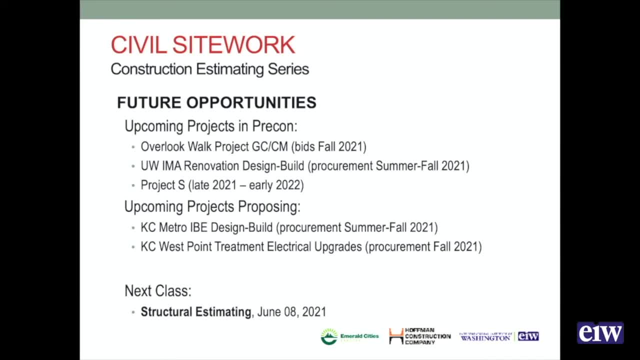 aquarium going over the new roads that they're building in replacement of where the viaduct used to be. that will start bidding in the fall of this year. we're also doing pool renovation at the IMA over at UW. that's a design build project that we're. 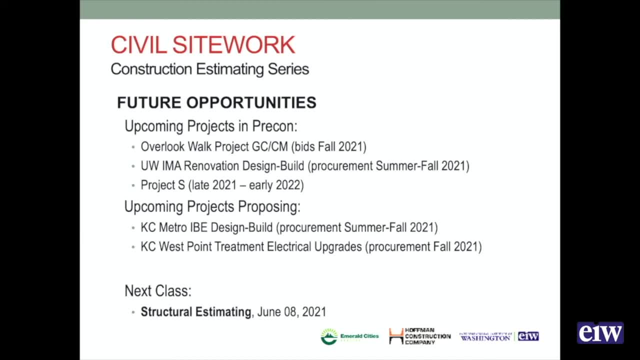 working on- and we will start that procurement process this summer and into the fall- and project S, which is a developer office building in Soto that is projected to start bidding out work late this year and early next year. other projects that we are currently proposing on but our design build. 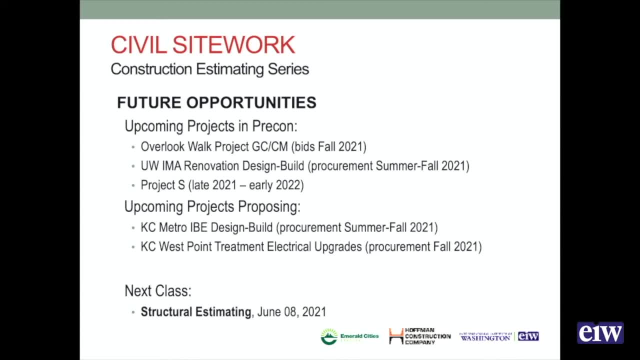 projects. so they're traditional design builds. so we have to actually provide a price that we'll be soliciting for quotes and bids and that's part of that process. the King County Metro: it's the interim bus electrification project where they're looking at how you 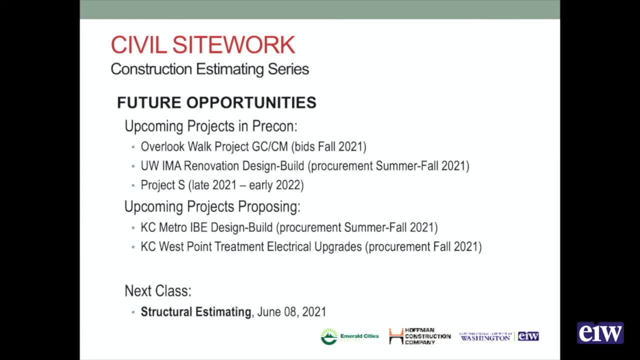 go to all electric buses that will be start procurement this summer and into the fall and then also out at West Point Treatment Plant. there's some electrical upgrades that they're going to be doing to improve the plant. we'll start looking at procurement in this fall as well. 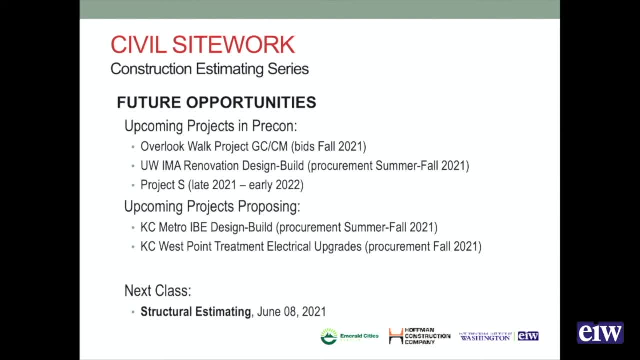 and then finally, next class, one week from today, right back here we'll be talking about structural estimating, so that's we'll be taking a more deep dive into concrete and steel. we'll also be talking about other systems as well, and how you estimate that and those systems. 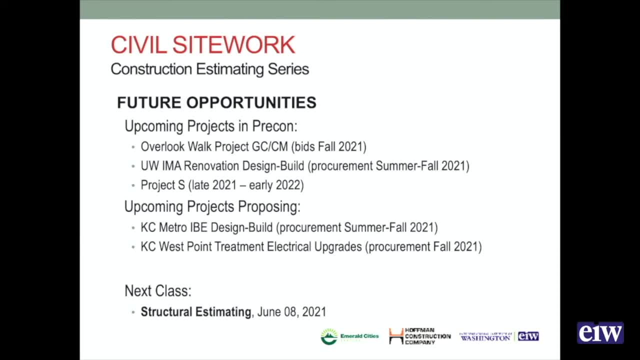 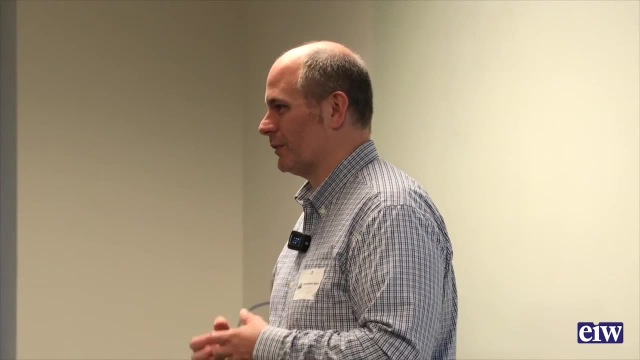 certainly structural- is near and dear to my heart because I've looking at concrete and managing some concrete projects, some pretty large concrete projects, and working with our crews to manage that work. so making sure that those costs are right is always been something that's very important for me to do. 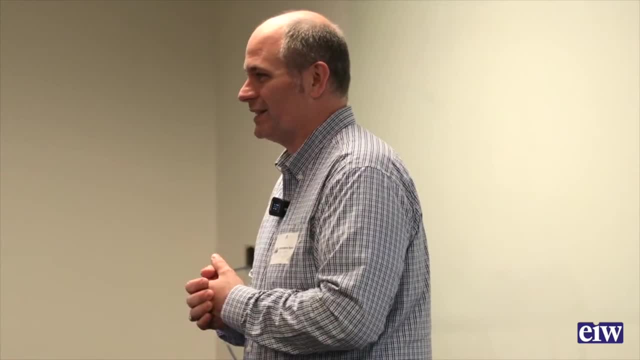 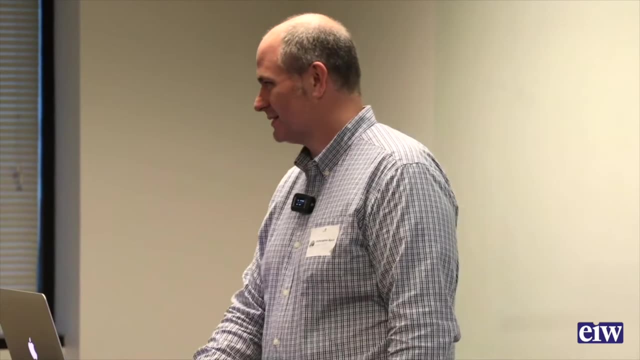 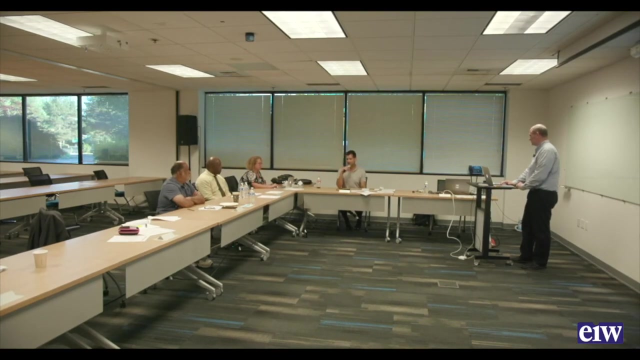 so I hope that if that gets your attention and gets your interest, come back and join us next week. we're really excited. the structural- you get to the meat of the operations, you know, and when you're working in construction there's obviously a lot of different sections within. 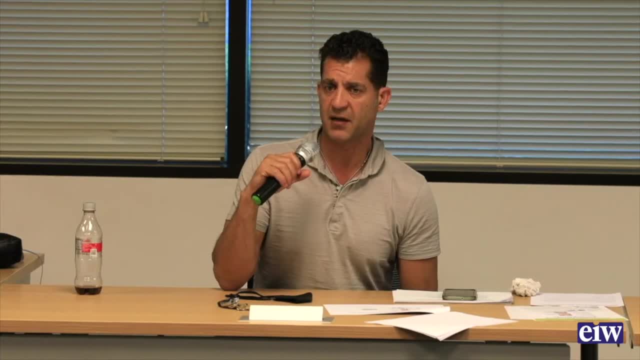 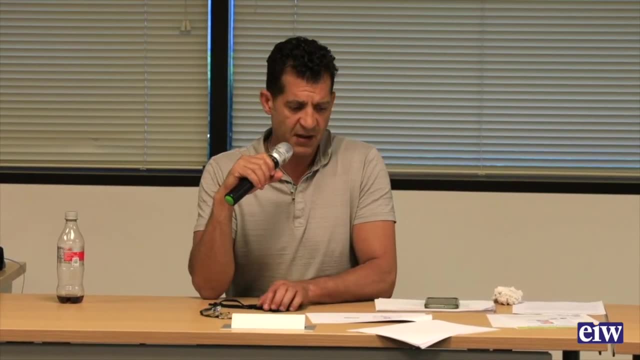 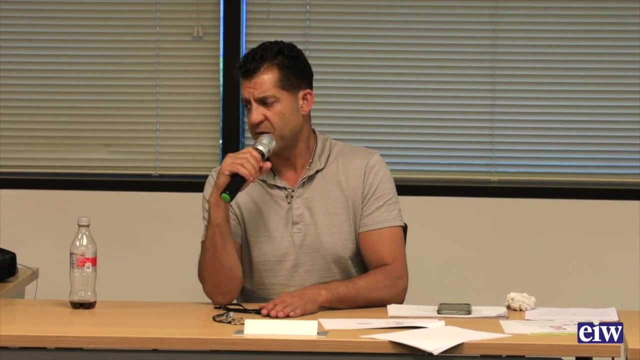 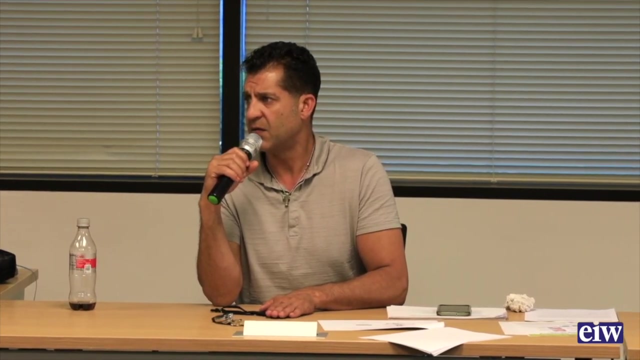 the plans and when Chris and I and Dave were talking about developing this series, we really wanted to develop, I guess, an enhanced series that would provide exposure to those trade segments that can really move the dial, and so you know there's a lot of people that can paint. 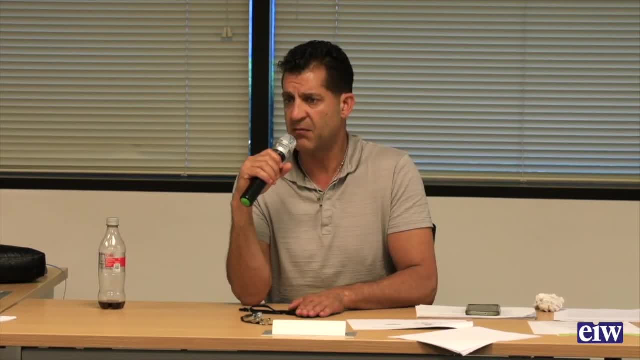 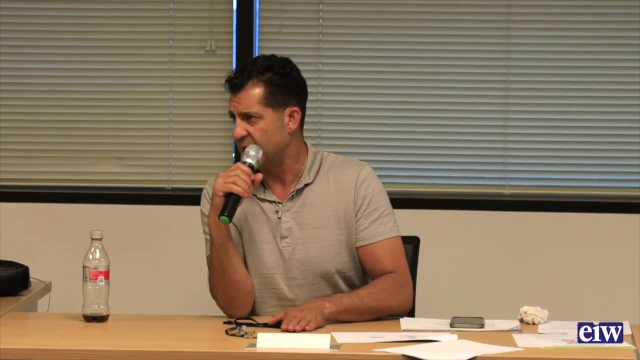 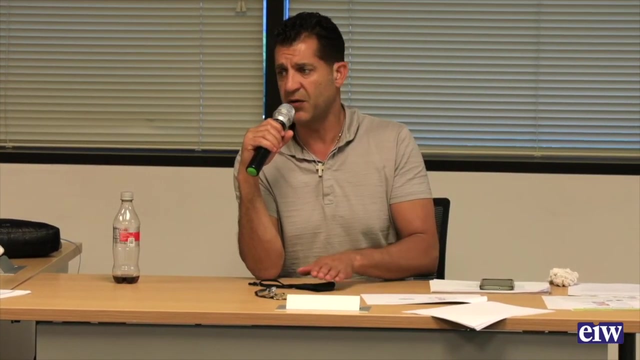 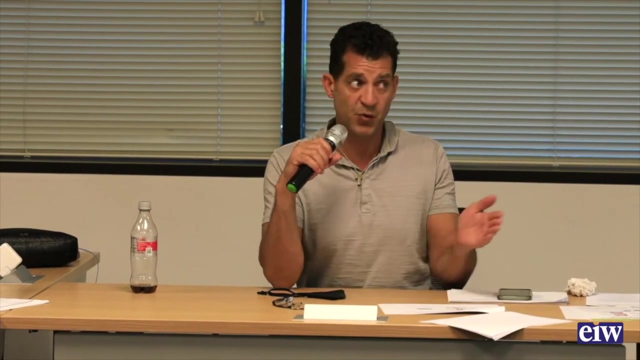 and we're gonna, you know, provide, you know, some some architectural um, sequencing, um, and information on that. but when it comes to those larger dial, moving, you know, in those large mega projects, it's typically those projects, you know, or those trades that involve moving a lot of dirt. 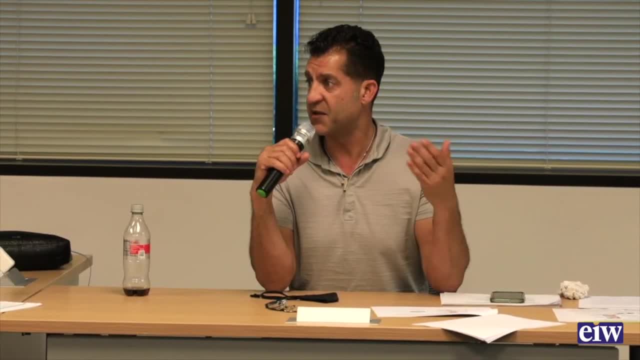 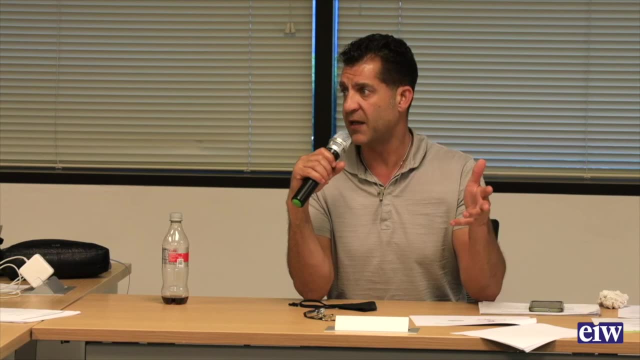 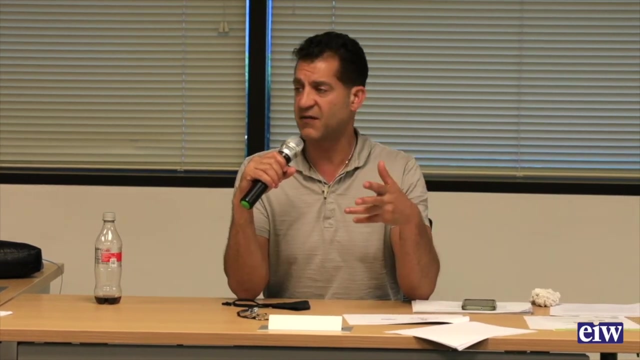 like we just discovered, covered today. there's the structural, you know, the steel and the concrete members and other members that are, you know, making it possible for whatever structure to exist. there's big dollars in those. and then you look into the finishes and the architectural and that's where you 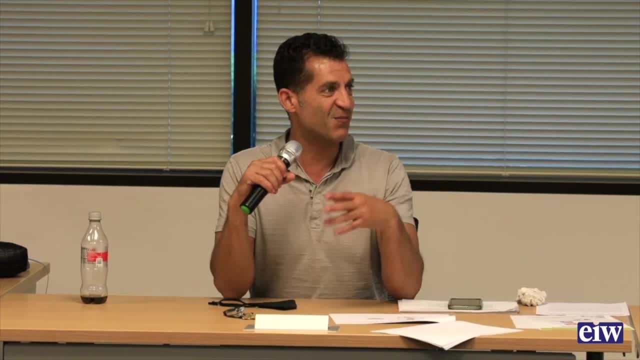 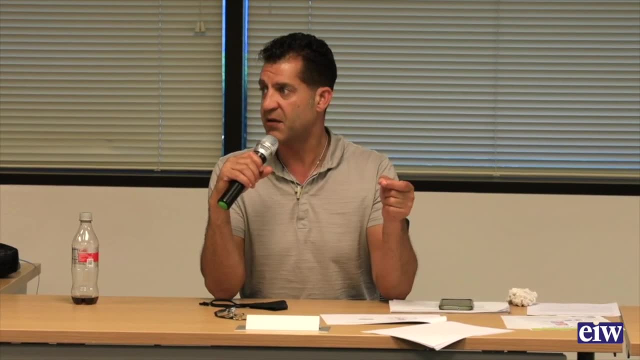 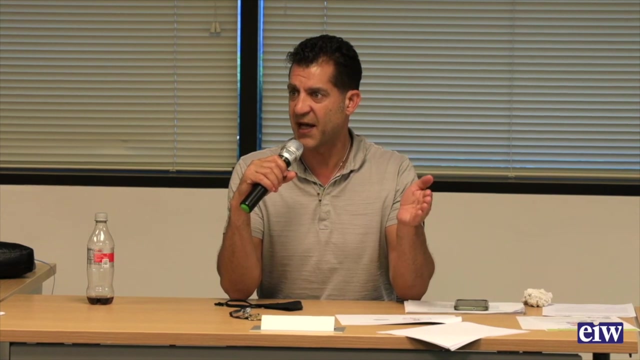 see some of the smaller trades, but we wanted to really start on the big side and we also wanted to focus on those areas where Hoffman is really looking to develop uh trade partners and that is in these areas that can really help move the dial. and when I say move the dial, I mean 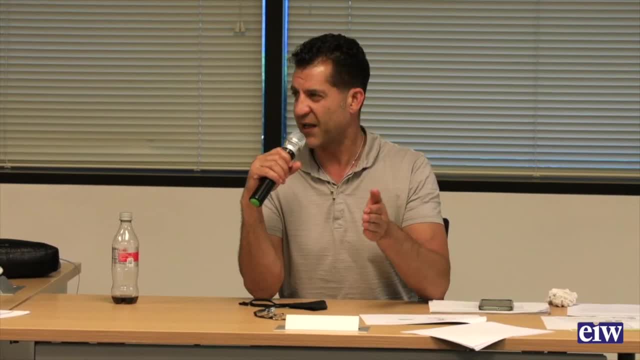 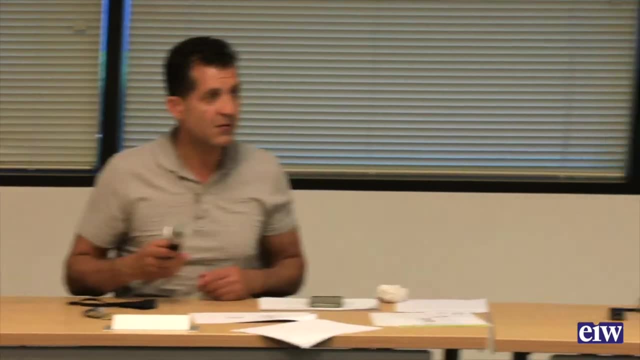 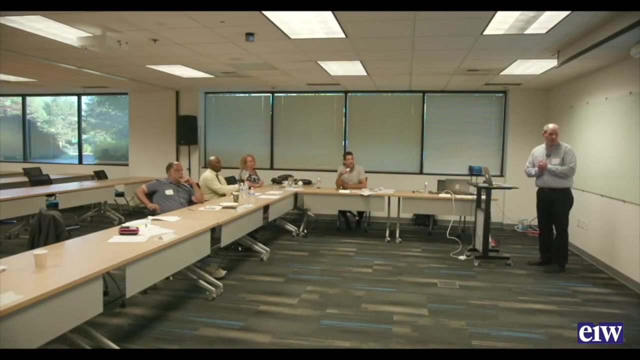 include small, diverse firms like ours in these projects that can really help us grow and expand. sorry is that the last slide, uh, the last slide has contact information on it, so there's my email, there's Dan's email, there's Rosalind's email. um, if you have questions, feel free. 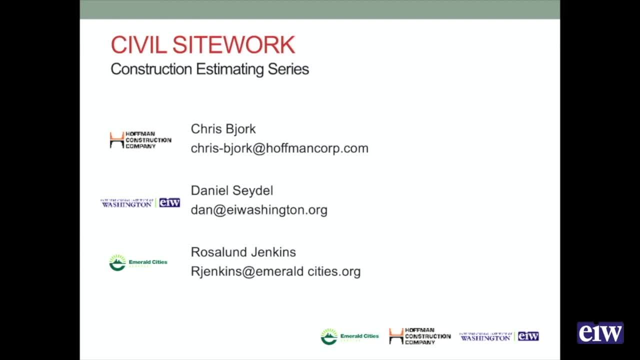 to email me. we said we will provide the slideshow as well. um, and you know, this was designed so that you would be able to get that slideshow at the end. that's why we did the snapshots of the actual takeoffs, so that you can see that systematic approach. 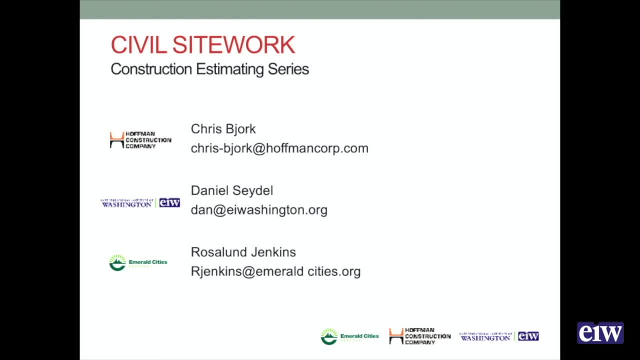 um, on how to take off those various scopes of work, um, but if you have questions, if you have requests on other, you want to talk about some of the things that we didn't necessarily dive into. feel free, um, if you have questions on landscaping or shoring or whatever it is. 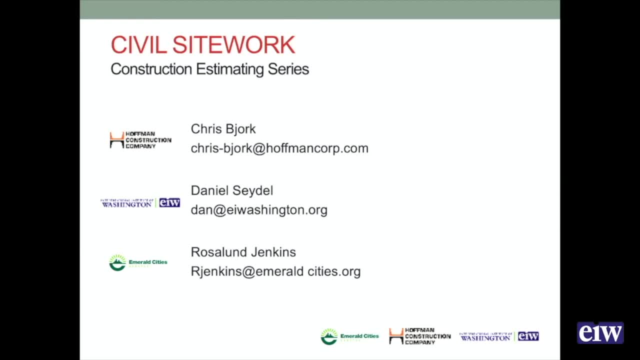 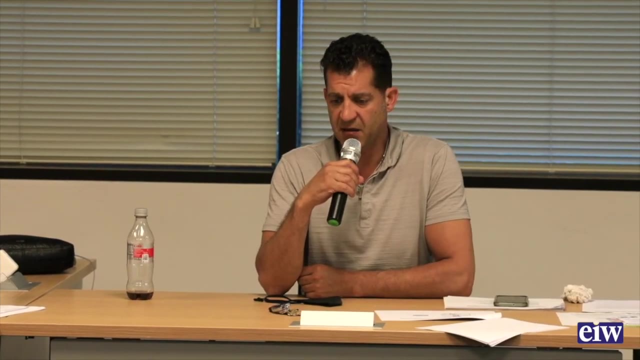 feel free to email me with the questions and we can talk and I can try to help you in any way. I can thank you. thank you, and again, we are so tremendously grateful for Hoffman Construction and those of you that are online and and tired of being uh. 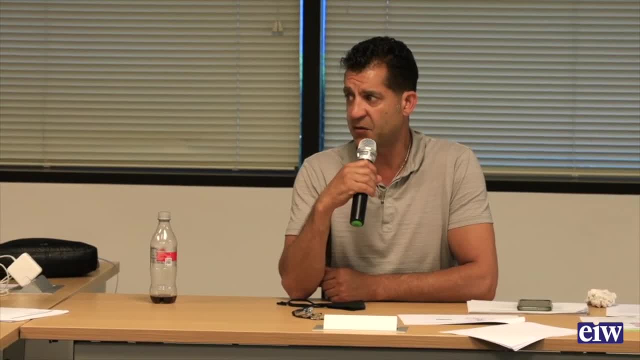 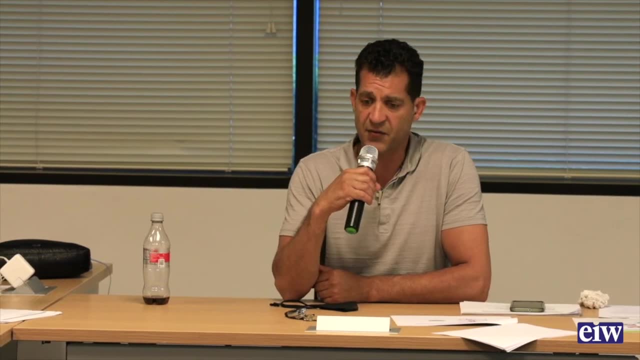 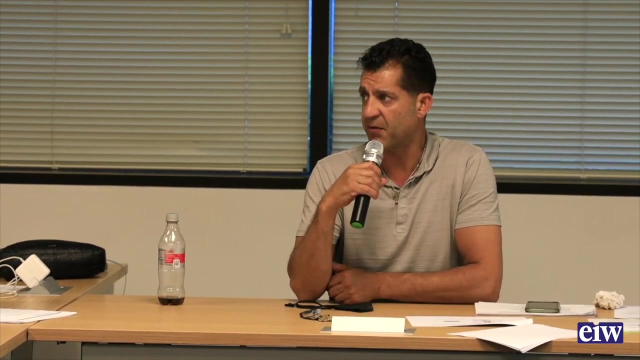 cooped up at home. you're welcome to come down, uh, to our next class, face to face. we'd love to see your faces, those of you in Washington State. um, we are going through the, the COVID practices here. uh, temperatures are taken and uh the the proper. 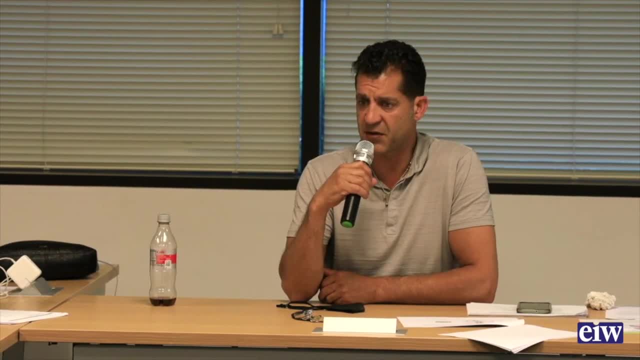 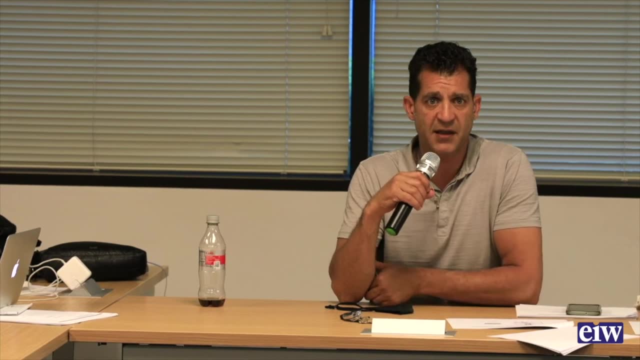 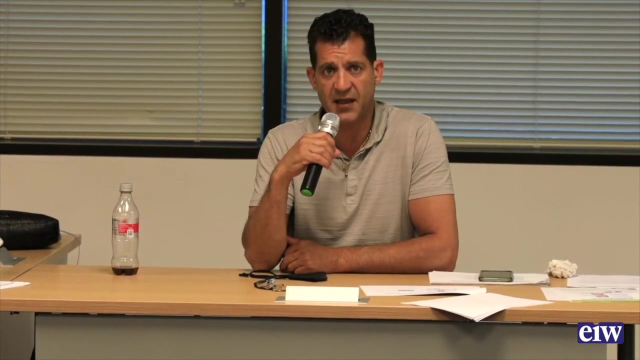 questions are addressed, and so we feel pretty safe. we do encourage those folks that uh are eligible to take their shots, uh, so they can remove their masks and have fun like the rest of us. um, but again, we just appreciate all of you that participated today. uh, this uh class, along with 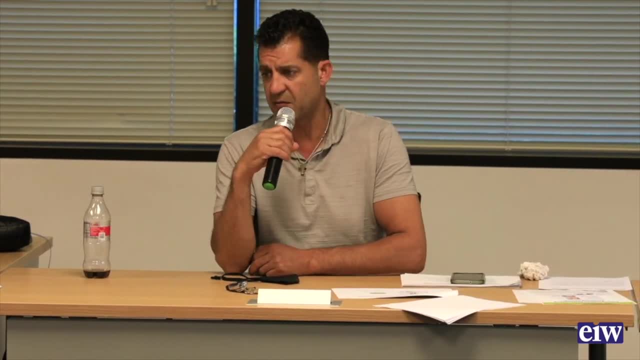 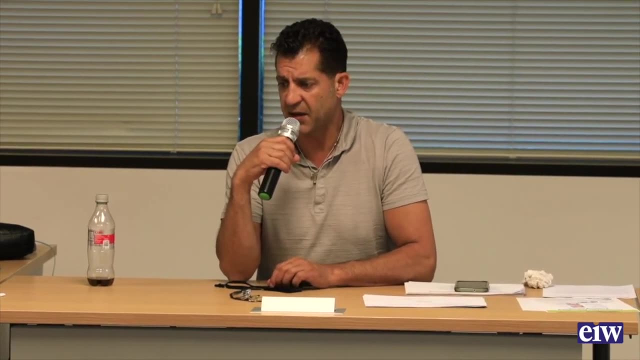 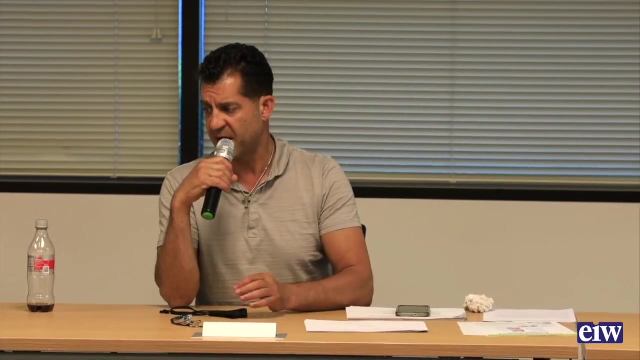 the uh the other two classes uh will also be a resource that we will share um, but those of you that are present are gonna get uh the benefit of asking uh direct questions to a very talented uh senior estimator. chief estimator for Hoffman Construction, Chris Bork Bjork. let's get a round of applause. and uh say goodnight.